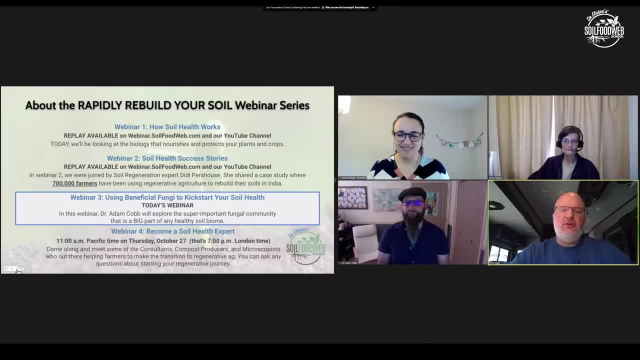 So let's talk about the webinar series. Like I mentioned, this is webinar three, which is using beneficial fungi to kickstart your soil health, And then we have another webinar coming up, webinar four, which is Become a Soil Health Expert. 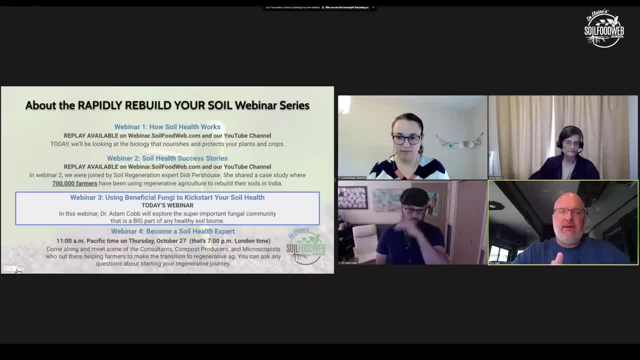 And that's going to be on Thursday, the 27th, And that's going to be talking with people like myself- consultants and compost producers and people who are running labs and so forth- And it's a great place to be able to ask all the questions about our experiences in doing this type of work. 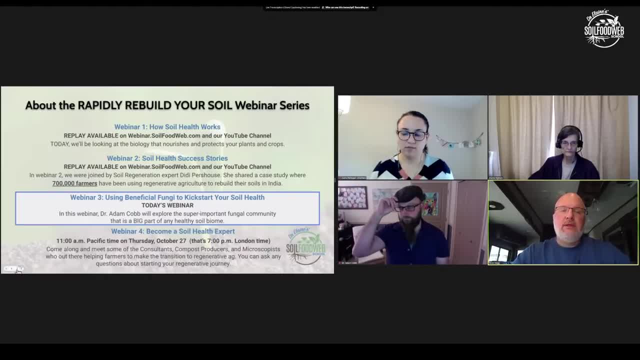 And then also, just as a reminder, we had webinar one, which was how soil health works, And then webinar two, Soil Health Success Stories. Those are recorded, So definitely, if you haven't watched those two, go back and watch those as well. 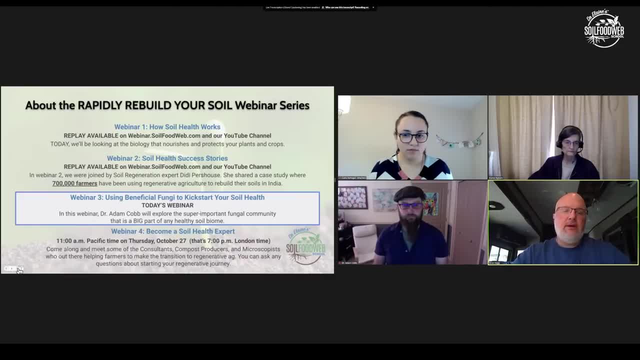 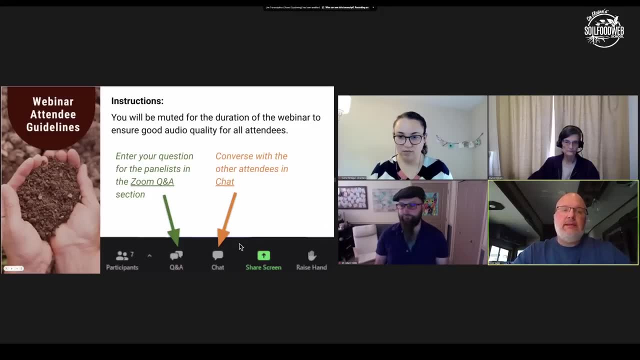 There's a lot of great information that were in those two webinars. All right, Next slide And just some housekeeping issues. here. We want to make sure that all the attendees are going to be in muted mode. There's just so many of you. 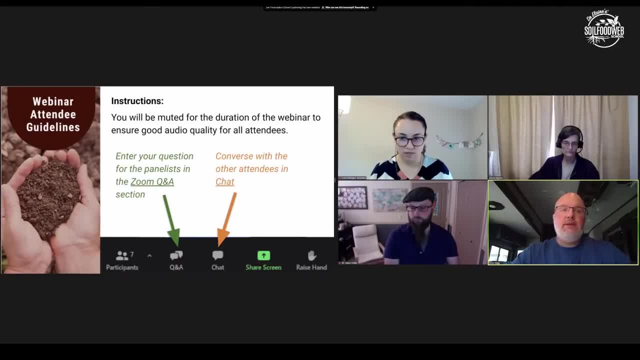 And we just want to make sure we cut down on any kind of background noise. But we definitely want to hear from you. So if you want to ask questions of the panelists and we'll have a Q&A section at the end of today's webinar- 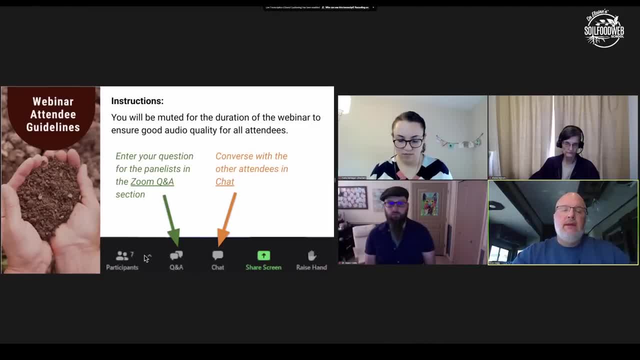 Go ahead and click on the Q&A Again. it's at the bottom of your screen And that will be for questions that you want panelists to be able to answer during the webinar. And then there's also the chat button, which usually is very heavily attended. 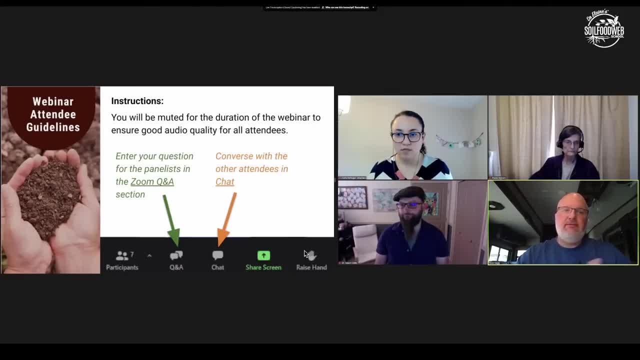 And those of you that are already chatting on there and told us where you came from. you already know where the chat button's at, But this is where you can have an ongoing dialogue with your fellow attendees, So just remember: if you want a question, though, to be answered by the panelists, don't put it in the chat window. 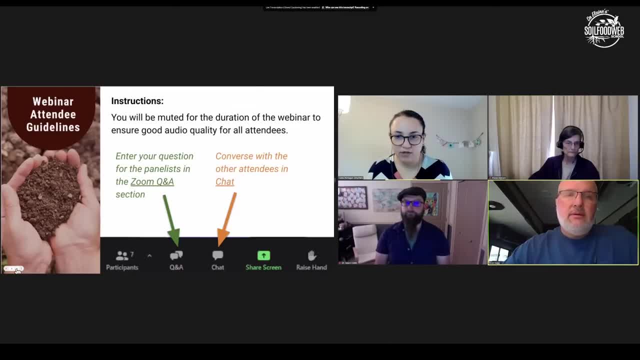 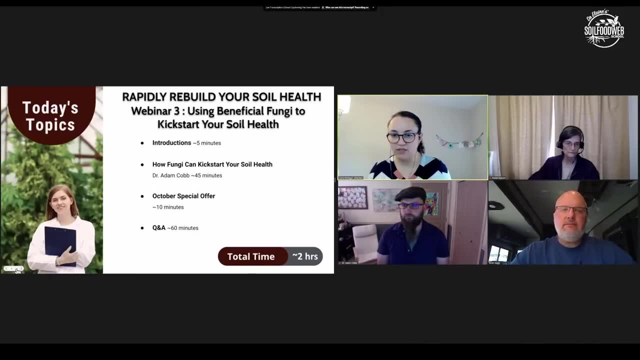 Put it in the Q&A section. All right, Brian, can I interrupt you for a second? Sure, We have a lot of questions. Some folks think that slides are a bit fuzzy, So, Adam, should we try to share again please? 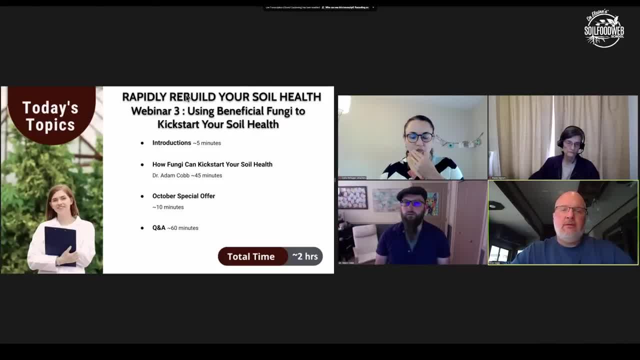 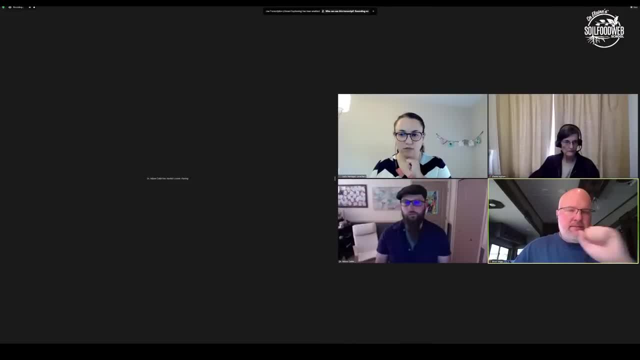 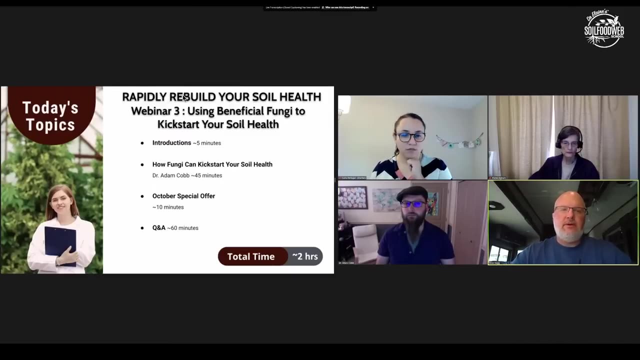 Adam can stop sharing and reshare. Is that a little better? It looks okay on my part. How about you panelists Looking all right? For me it looks fine as well. Let me try A lot of much better in the chat. 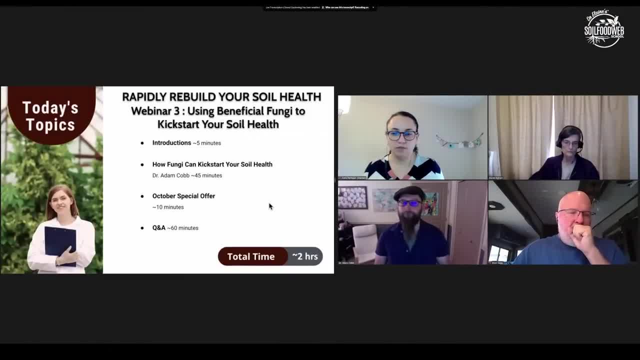 Adam, be sure to optimize your video. Yep, Okay, All right, So let's talk about what we're going to discuss in today's webinar. So we're going to do some introductions. just talk and let the panelists introduce themselves. 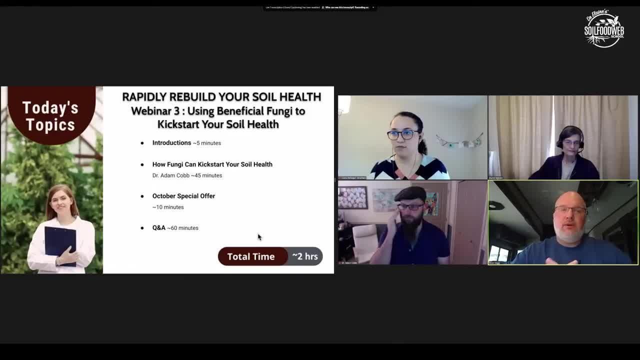 And then Dr Adam Cobb is going to go through how fungi can kickstart your soil health, And then we'll have a brief discussion or video talking about our October special, the promotion that we're actually running this month, And then our Q&A. 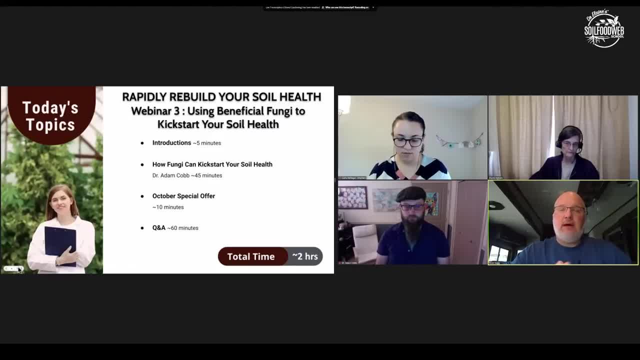 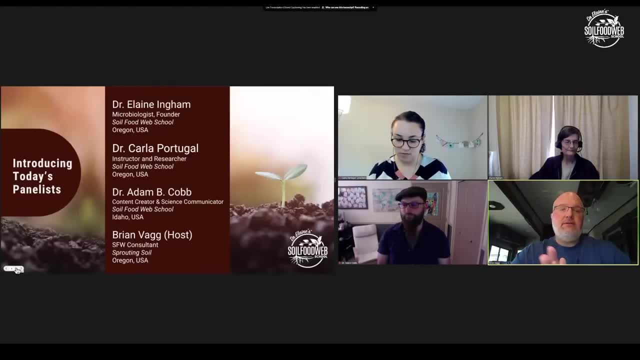 It's going to be about 60 minutes a night, So we're looking at about a total time of about two hours for today's webinar. Okay, Next slide. There we go. So let's have the panelists introduce themselves. 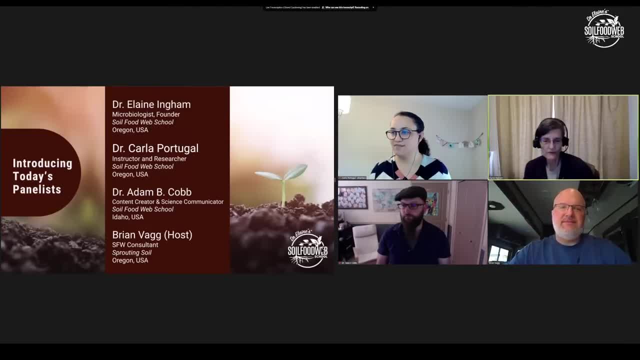 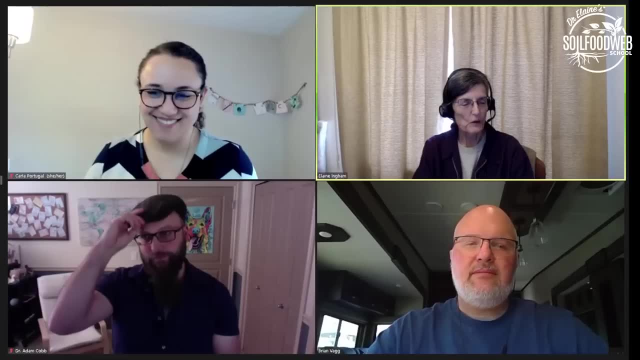 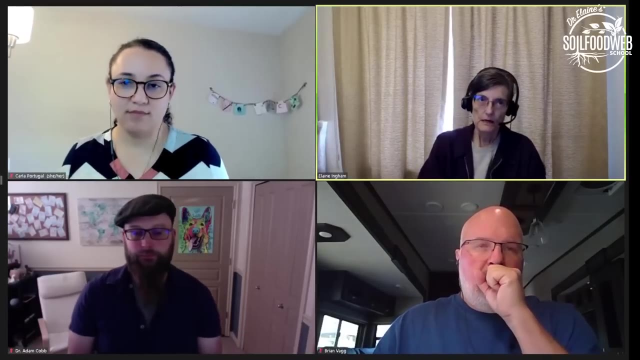 So Dr Elaine Ingham take it away. Okay, Thank you. I'm Dr Elaine Ingham. I'm the founder, or one of the founders, of the Soil Food Web School. I have worked in the area of soil microbiology for about 45 years. 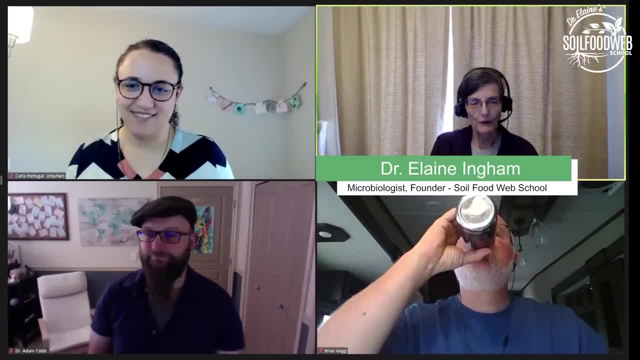 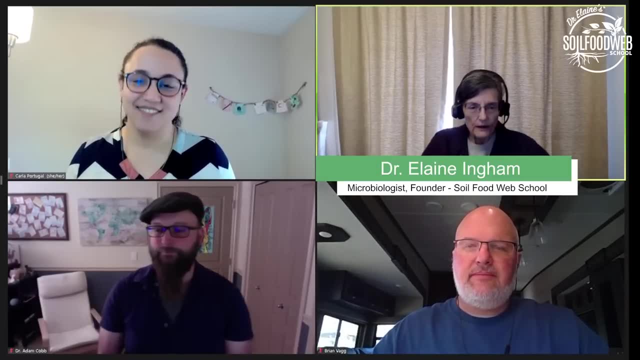 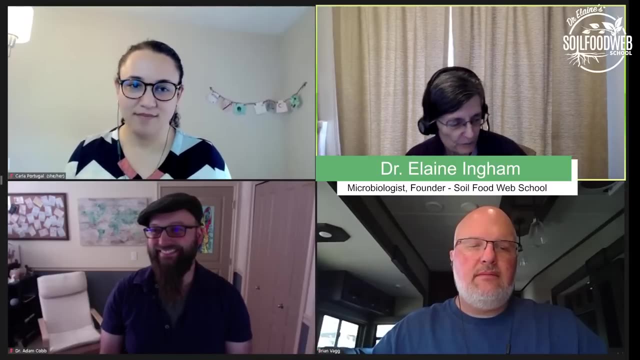 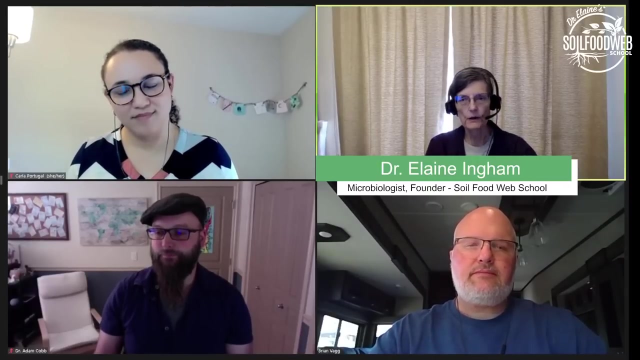 And know a little bit about what actually goes on in the soil. and that's kind of the fun of this is: you learn more all the time and you have to fit it into the picture puzzle and it's a three dimensional or maybe even four dimensional cross jigsaw puzzle of what belongs where and how do they all interact with each other and what happens when it's cold or hot or wet or dry. 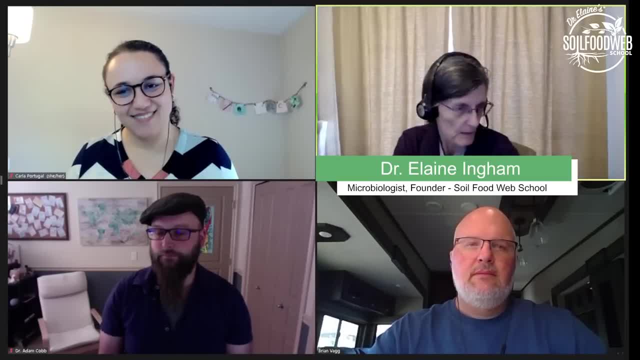 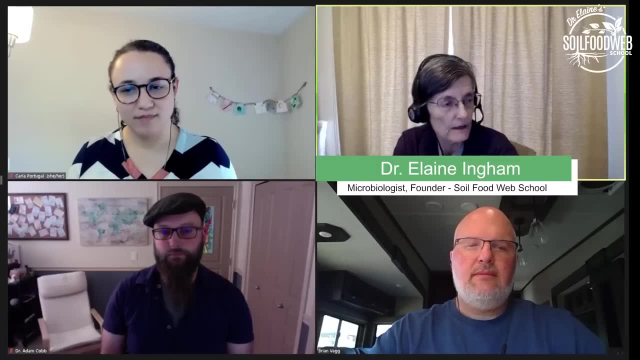 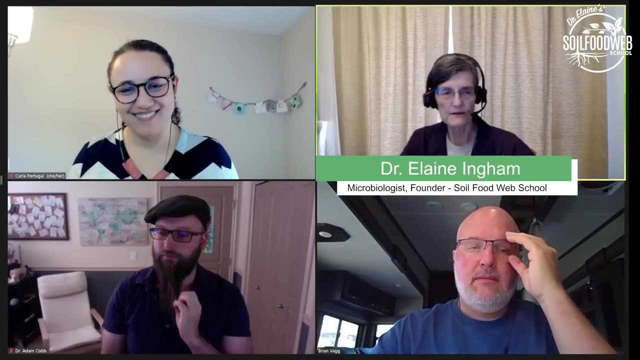 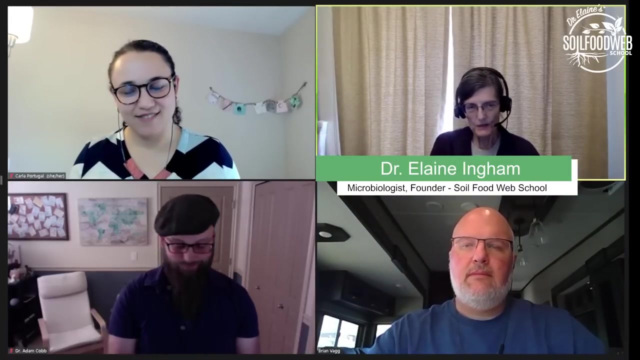 So these are the things we're going to be talking about, We're going to be picking up on in all of the courses and the classes so you understand how to manage your property to be able to grow really good, flavorful food that's got the nutrients in it, that has the help from all of the microorganisms. we suppress diseases, we suppress weeds- the whole dammit that we teach you about. 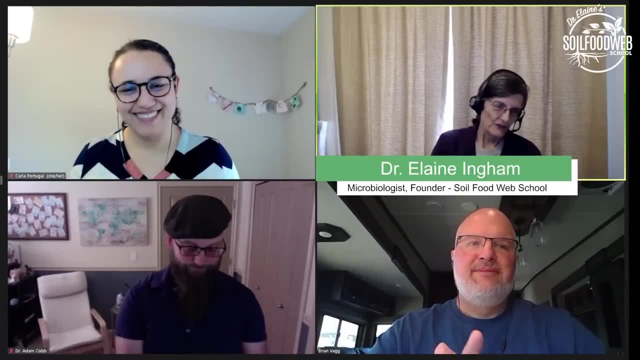 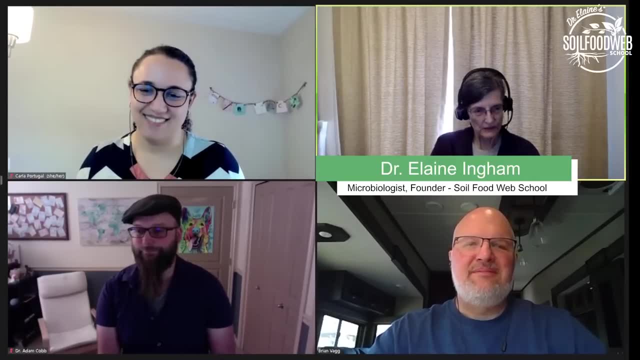 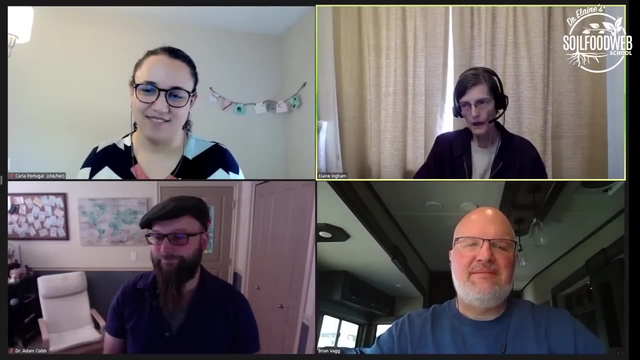 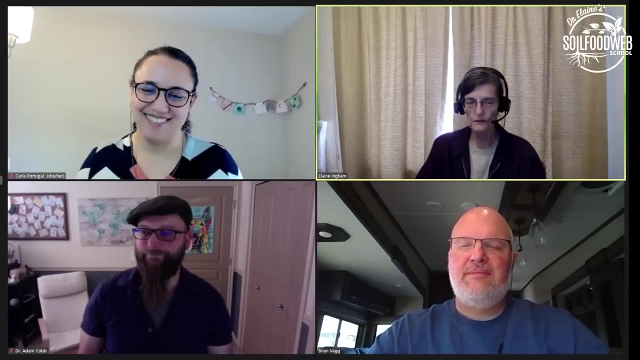 So we're looking forward to seeing you here in the future In Corvallis and learning the information you need to have to be successful- and typically we are quite successful at getting people converted from their dirt, get it converted into soil, If you follow the directions. it's really important to add the right biology at the right time. 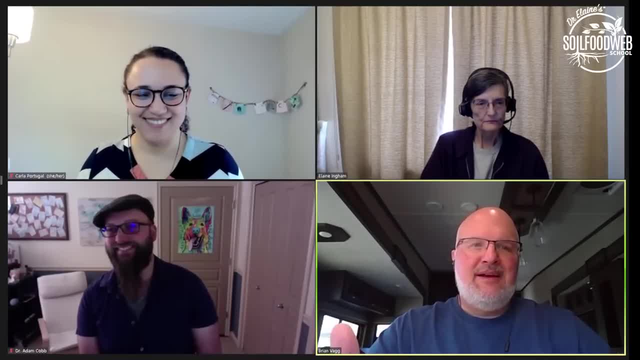 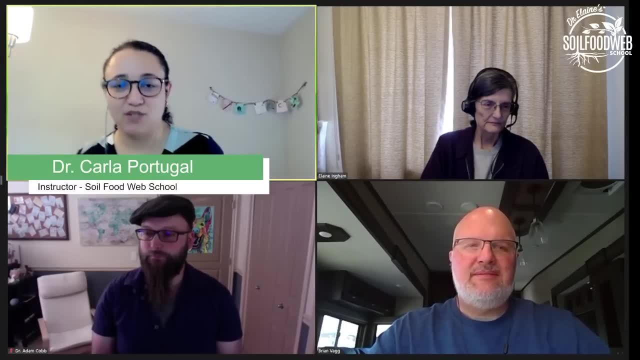 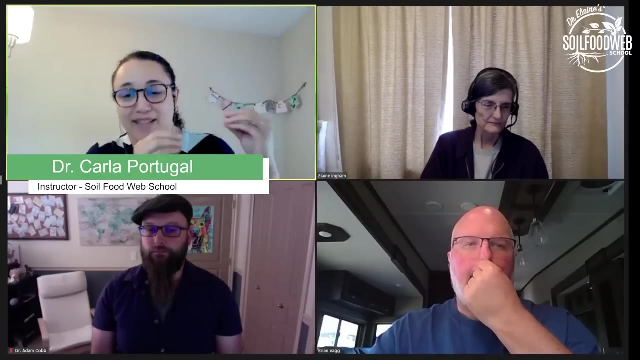 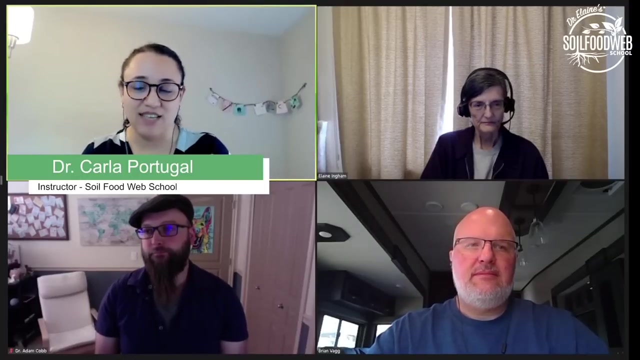 Okay, Thanks, Elaine And Dr Carla Portugal. Hello everyone, Welcome. I'm have a pleasure to be instructor and research at the school. I'm environmental scientist and I love to be this bridge to connect all the knowledge that we have and continuing on this journey, like Dr Elaine said, and help guide you guys on this path, on this beautiful path. 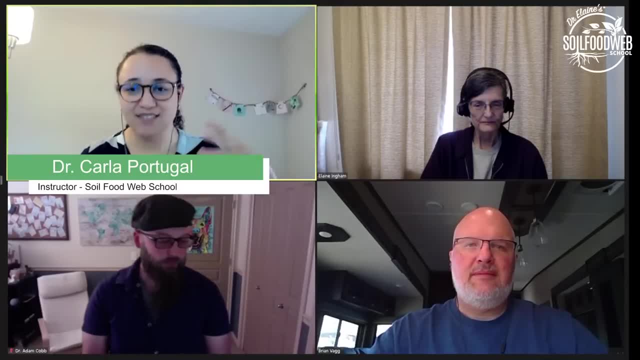 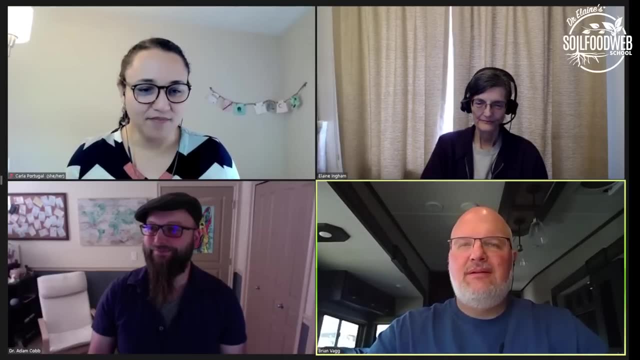 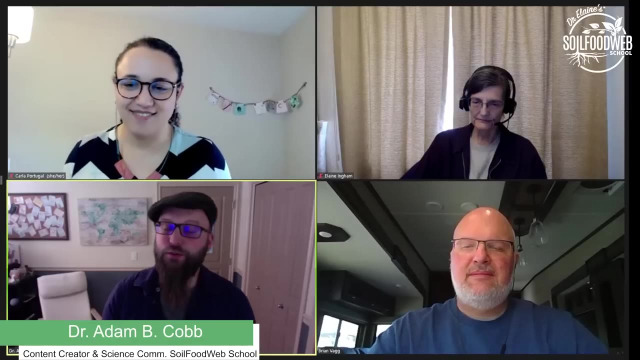 So thank you everyone to be here and hope to see you guys coming to our courses. Thanks, Carla And Dr Adam Cobb. Thanks, Brian. So those who have seen me on some other webinars will know that I'm just a fool for fungi. 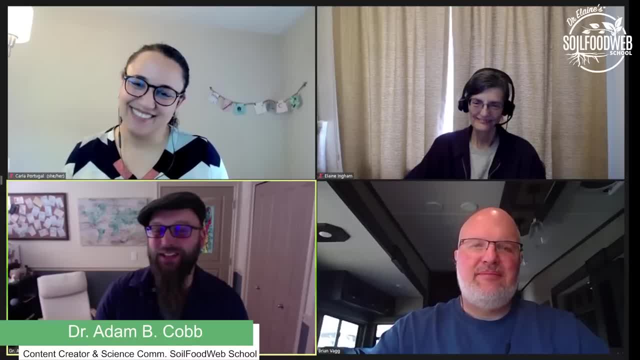 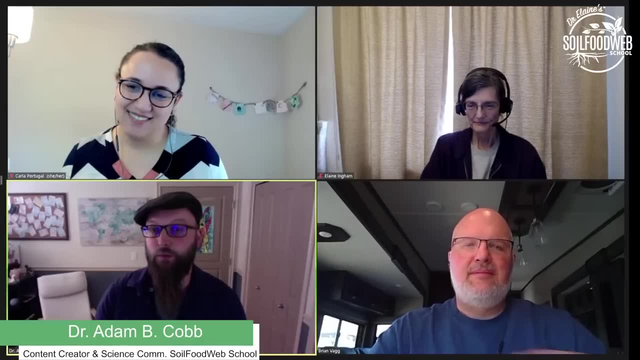 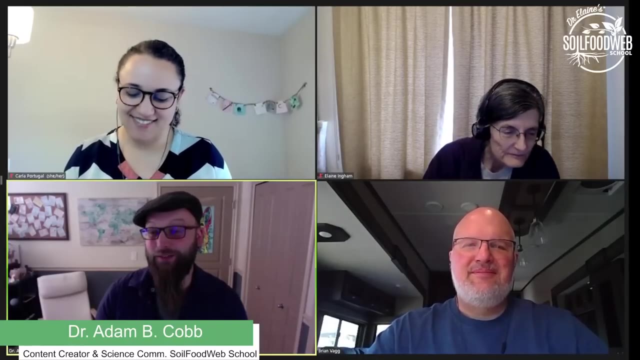 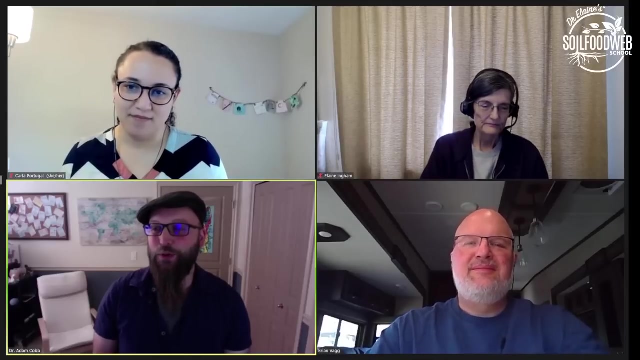 I just love them. And yet I've come here to the soil food web school and been involved in content creation and communicating the science of what we're doing here And I'm falling for all the organisms Now. And there's there. In fact, earlier today we had a microscope session with the staff, and just to see all these beautiful creatures in the soil and what they're doing is exciting. but I'm excited today to speak about fungi, which were my first love in the soil. 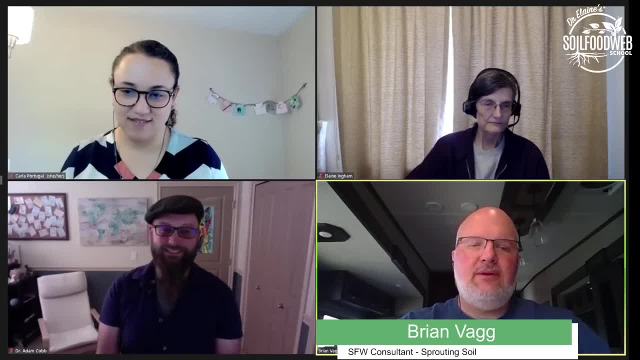 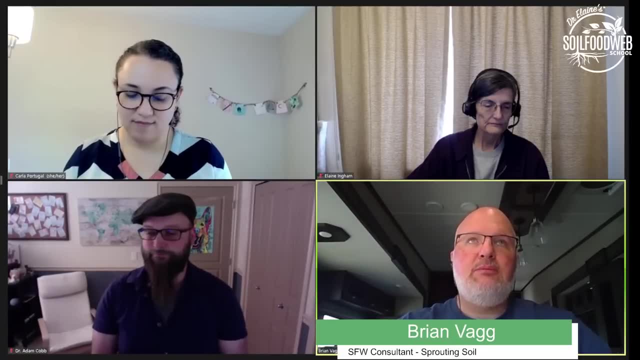 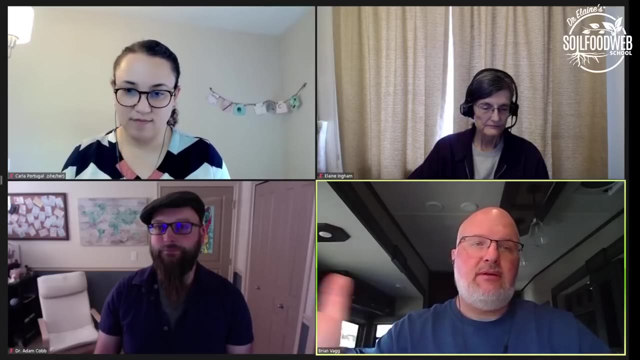 Thanks, Adam. And then I'm Brian bank. I am a social web consultant. I have a company called sprouting soil and I'm based out of Oregon. Yeah, I basically help people make those conversions and I have clients that span the gamut from residential yards all the way to very, very large scale agriculture, very large ecosystem restoration projects. 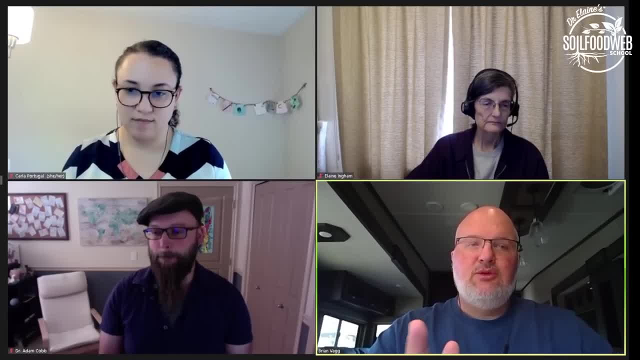 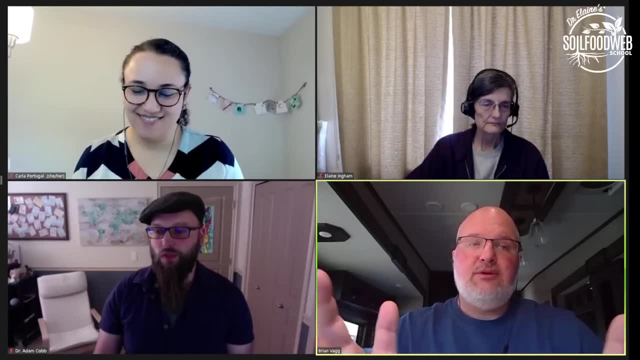 And it's amazing how you can apply these principles to any growing system. It really doesn't matter what you're trying to grow, the principles will align because we need so biology. So all right, And I think at this point, Adam. 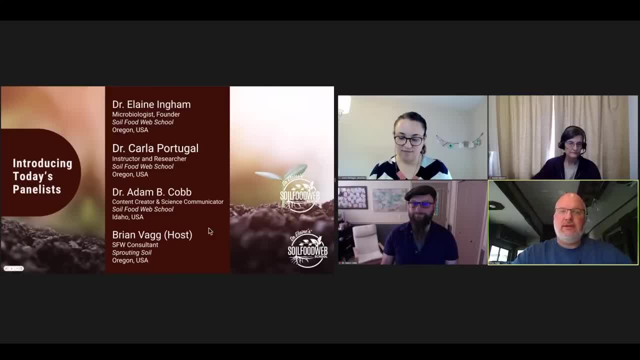 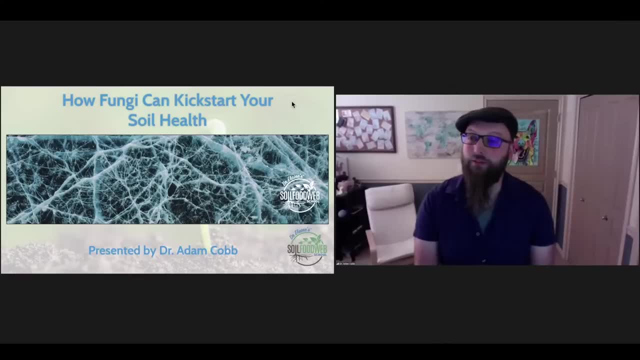 We're going to hand this over to you and I think you're going to take this away for us, right? Yeah, thank you very much. So, as promised, we'll we'll talk a bit about fungi today, and I want to remind everybody listening that fungi are one group, one very important group in the soul food web, and we'll have a chance to talk about some of the other players. 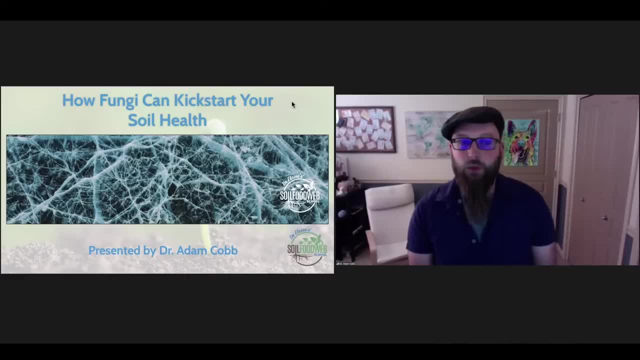 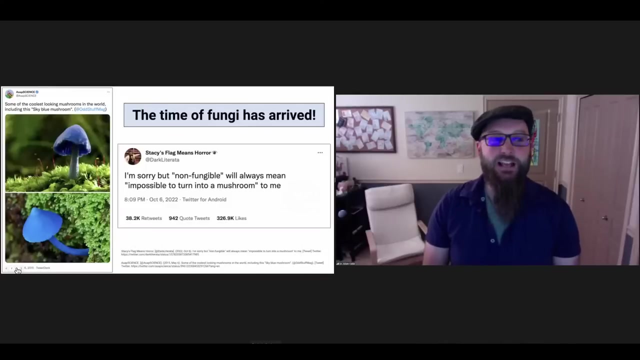 as well how they interact with fungi. But when you're talking about a soil that's been severely degraded, Especially, maybe over tilled, Overgraze, managed in the wrong way for years, Fungi, because of the fact that they create structure in the soil, are an organism that we find is absolutely critical, a critical player, And so I just I'm excited to get to share a little bit about that, including 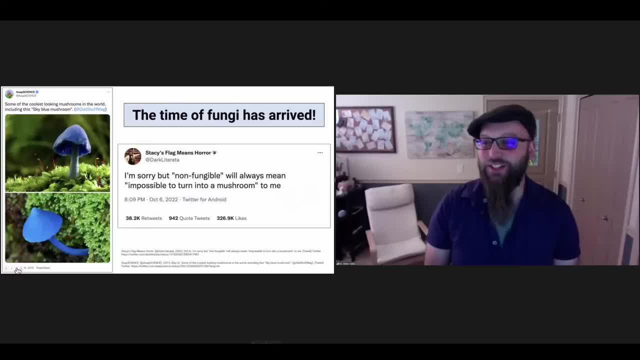 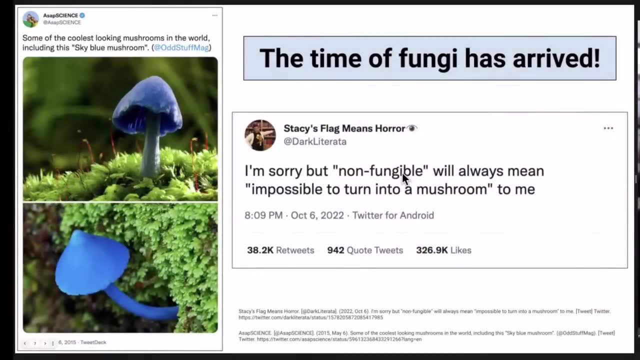 I'm excited to say that That now is the Time of the fungi. We are seeing popular science tweets or even seeing jokes. I don't know if anybody gets this cryptocurrency joke, but I is too good not to share. And it's true. actually, non fungible will always mean impossible to turn into a mushroom, since non fungible is non physical And since most of the rest of the world could turn into a mushroom given enough time, even you. 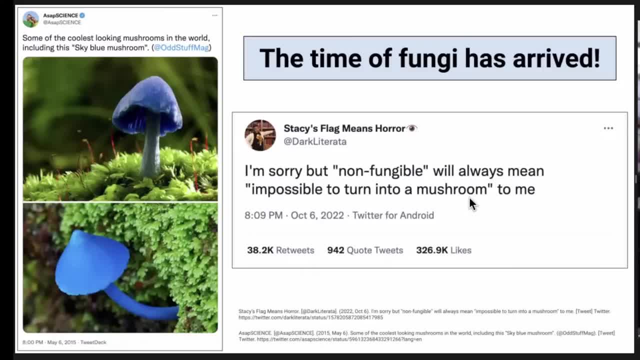 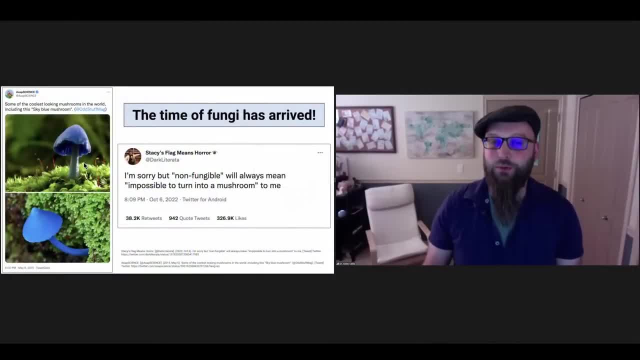 Even me we could. we could turn into mushroom someday. I think it's pretty great that people are talking about it, that we're sharing you know, all of the wonderful, beautiful fungi that are in the world. The internet is a great place for that. 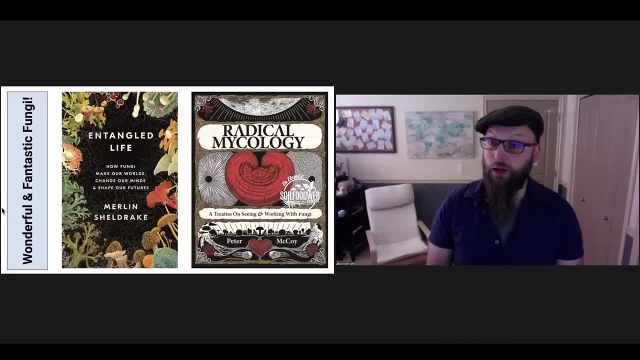 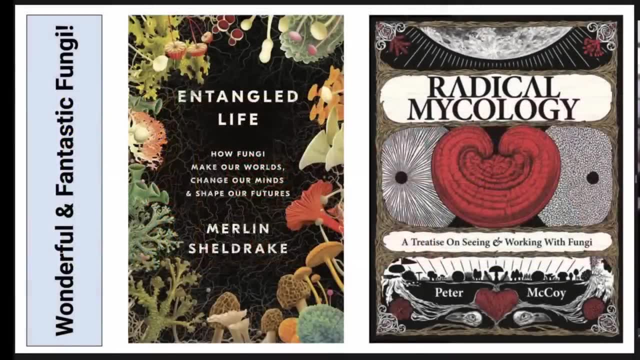 I'm. Also there are books, So these are two gentlemen that we have had here at the soul food web school is speakers and panelists in our recent soil summit, Merlin Sheldrake and Peter McCoy- And many of us here at the school just got back from. Peter McCoy is special radical mycology convergence, which was a great opportunity to connect with people and just appreciate all the things that fungi can offer us, because they are wonderful. 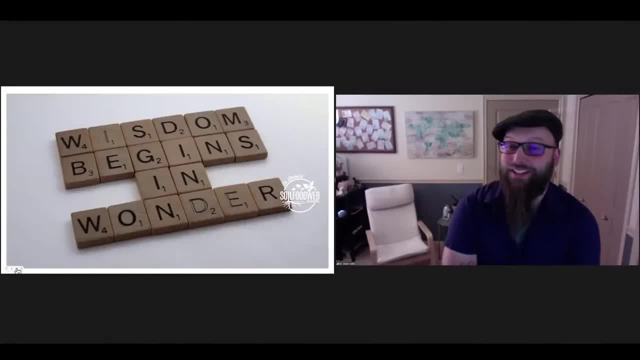 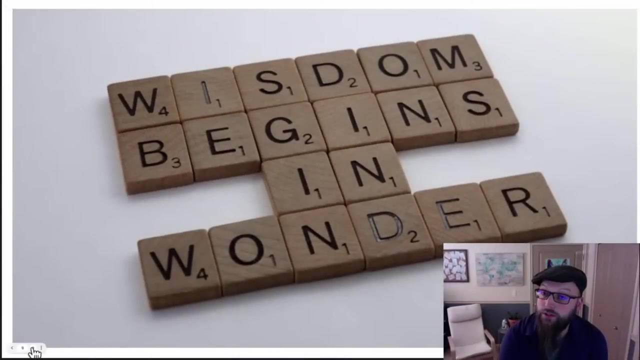 and fantastic And, in fact, when we're talking about the con in the context of soil health, One thing that is pretty magical to me to think about is that learning to have a relationship with the fungi and soil, learning how to help support what they need so that they can help support us and the process of regenerating soils. 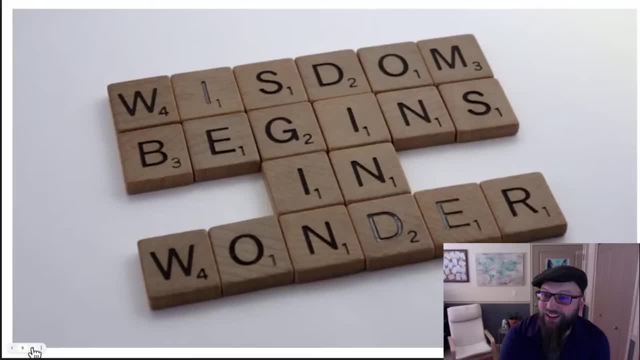 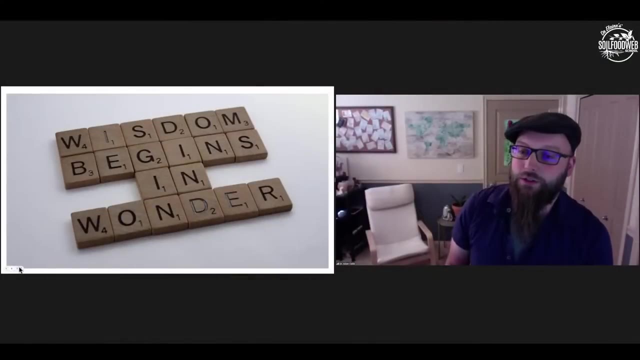 We literally get to tap into the wisdom of the fungi that goes back over a billion years of evolutionary history. They have been here doing their thing And it is so exciting to learn about their character and their features and all of the benefits that they provide to us, which they kind of give freely. 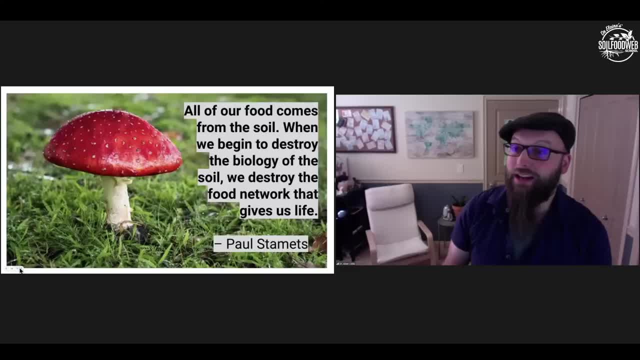 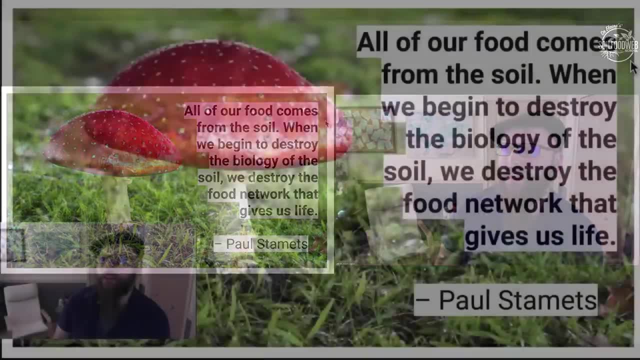 So I just want to want to start with that idea- And this is a quote you may have heard of Paul Stamets because he's quite famous in the fungal world- but I thought that this really fit with some soil food web. But I thought that this really fit with some soil food web. 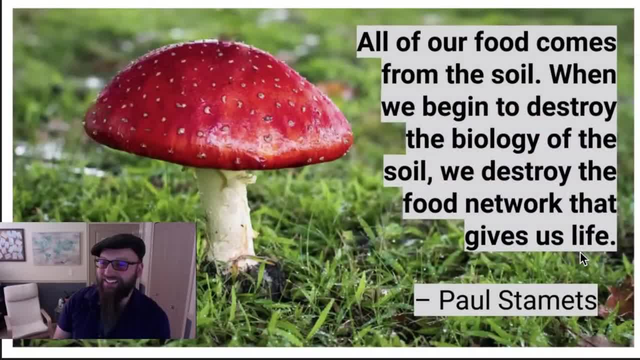 But I thought that this really fit with some soil food web And I think that's a really good approach as well, because he says: all of our food comes from the soil. When we begin to destroy the biology of the soil, we destroy the food network that gives us life. 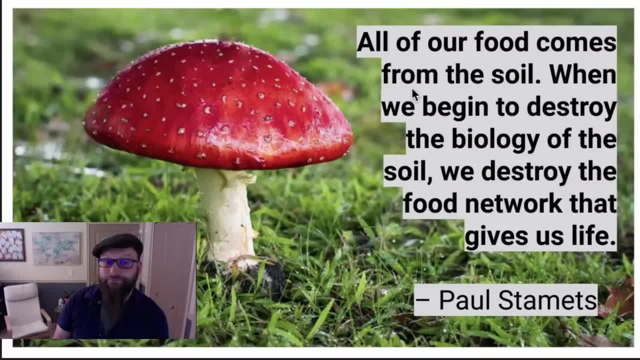 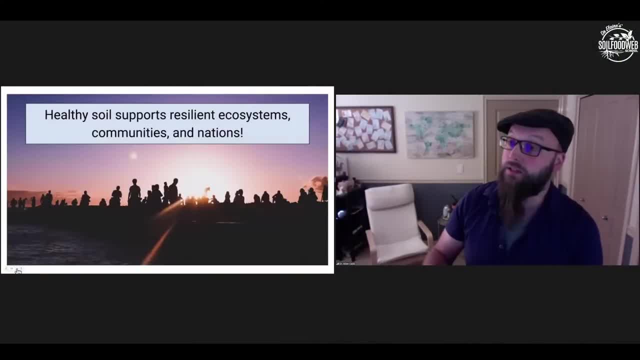 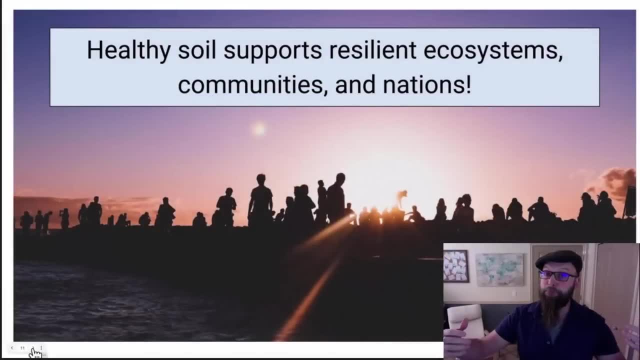 And so this is something. This is just a starting point to orient us to the, to the whole, the whole talk today. Because, as I mentioned in webinar number one, healthy soils support resilient ecosystems. Because, as I mentioned in webinar number one, healthy soils support resilient ecosystems. 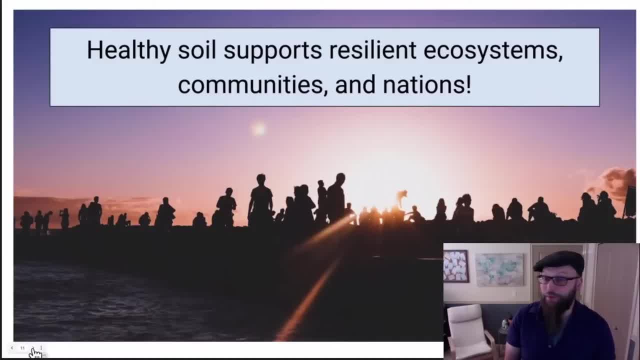 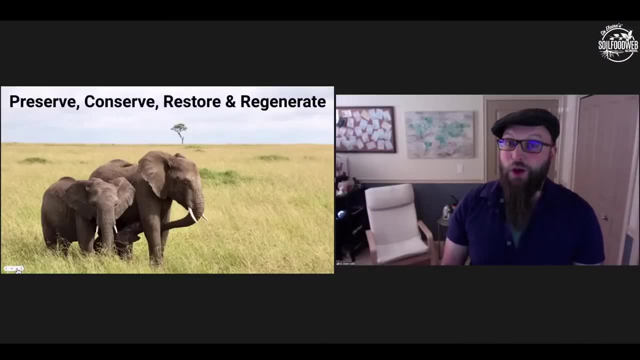 Human and animal and plant communities and, ultimately, nations right. I love to share the quote from us President FDR, who said: the nation that destroys its soils destroys itself. So this to me, I was I was looking for. You know it's sometimes it's hard to visualize what's going on in the soil. 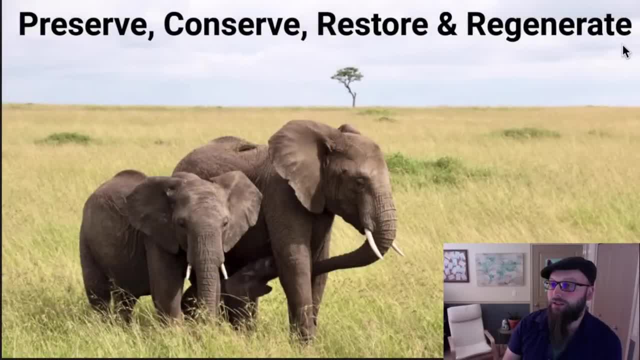 But let's think about the fact that what we see, But let's think about the fact that what we see, the fact that what we see more easily, even the large creatures like the elephants, are really there because of what's going on in the soil. elephants are eating vegetation and those plants. 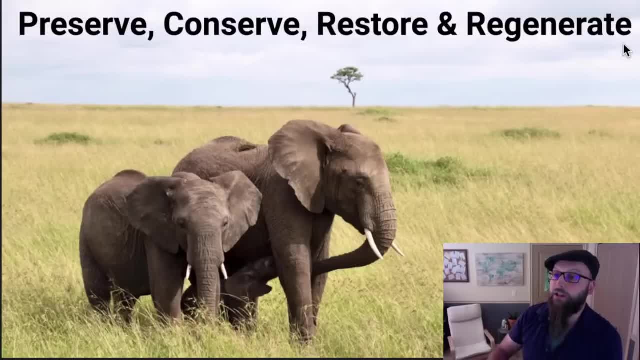 are dependent on the microorganisms that they're in community with right. and so, if our goal is to see things like the preservation of lands around the world, that we can have a safe refuge for the biodiverse life that we share this planet with, if we, if we're talking about the conservation, because 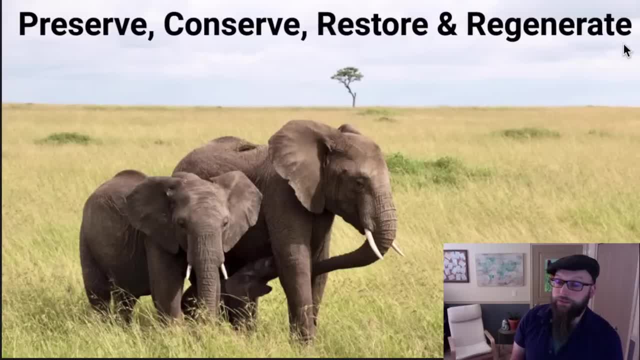 the use of the resources that we do access, like forestry, because we need those products for our, for our human needs to be met. and if we talk about farming, ranching, food production or the production of cotton- which i'm wearing right now- right, it ultimately goes back to the soil. 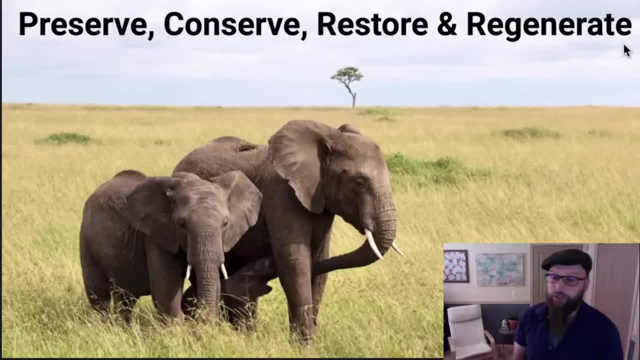 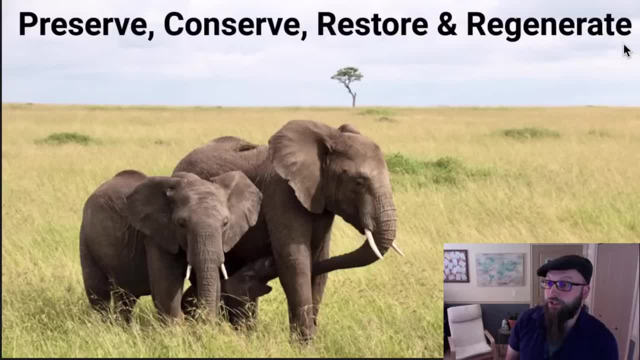 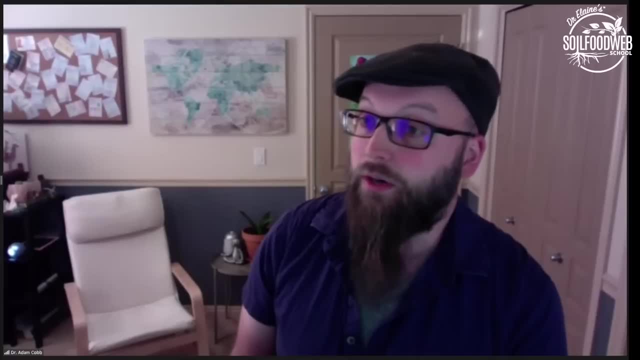 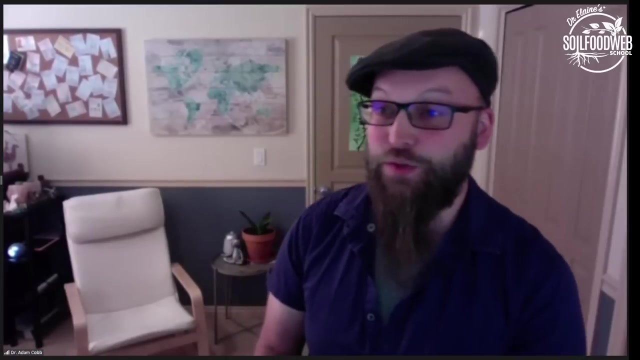 a lot of hope that in the restoration of these organisms and their and their ecosystems, with the regeneration of the functions of the soil, that we can actually reverse a lot of the damage that human society has accidentally or negligently or intentionally done to our biosphere. and i don't really want to live in in a world that doesn't have elephants in it. 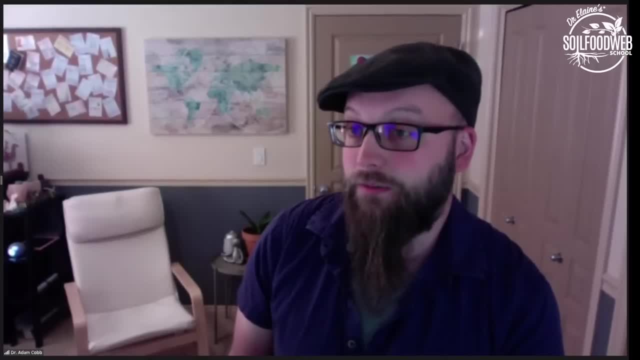 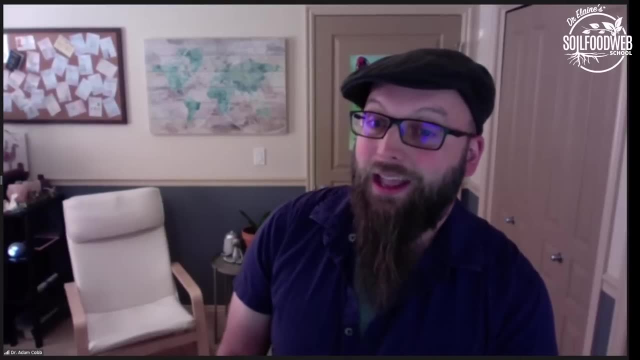 biosphere, and i don't really want to live in in a world that doesn't have elephants in it, and they're very threatened by climate change and many of the other ecosystem disruptions that they're facing, and so let's remember that to have them, we have to have thriving soil microorganisms. 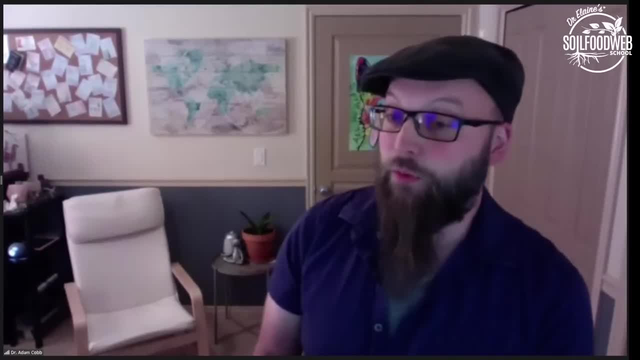 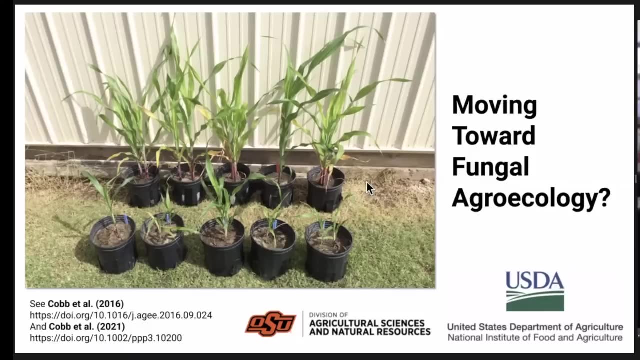 i would also say this is personal for me and i've shared this before, but some of the research that i've done this is with grain sorghum and just one subset of soil fungi, the arbuscular mycorrhizal fungi. i found that there these plants are much more productive when they have that full suite. 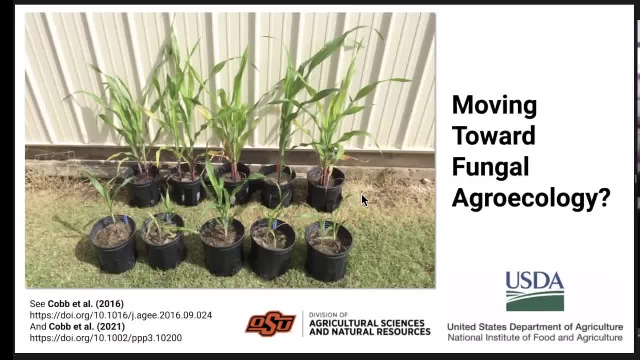 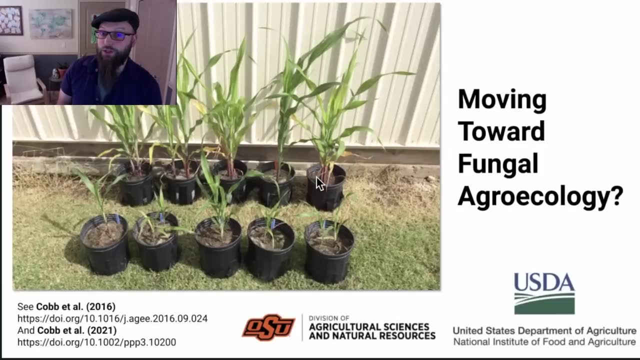 of soil microorganisms. so the only difference between these pots in the front and these ones in the back was the arbuscular mycorrhizal fungi. we, we removed it from the soils here but left it in the soils back there, and so that difference of growth, you know, sometimes we, we could calculate that it's like 600. 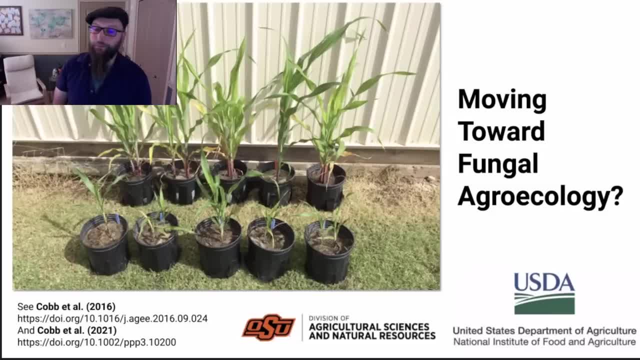 percent more productive. but the plant is because of its relationship with a beneficial fungi- and i have links to a couple of papers where i've explored this- mostly with sorghum and and some other grasses, but also alfalfa. we saw a similar thing, but again i would, i would remind us that fungi 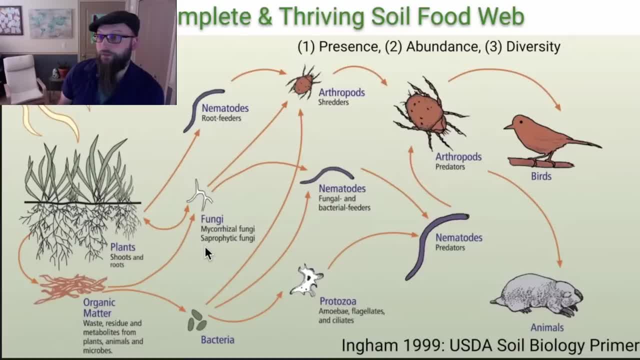 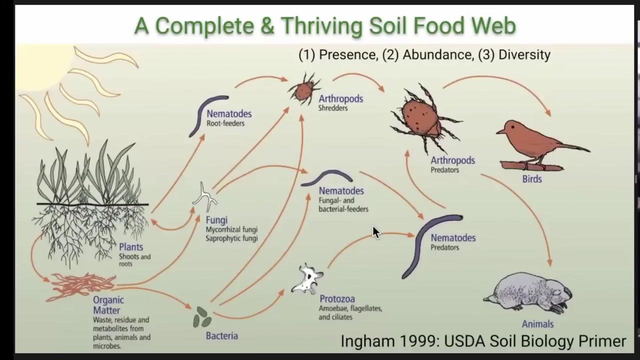 are one component of a complete and thriving soil food web and that if we have the, the idea here, one of the central ideas, is that if we have anything missing- the protozoa, key bacteria, the micro arthropods, various um groups of of nematodes- that something will be disrupted. 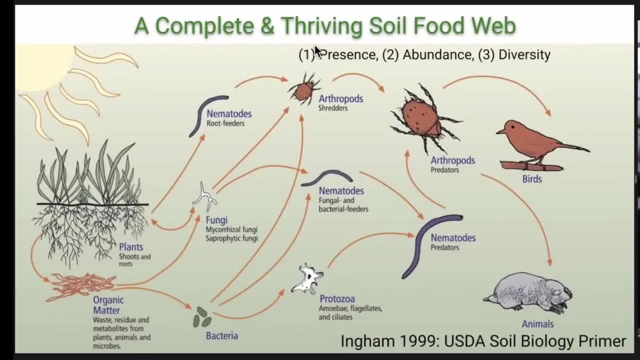 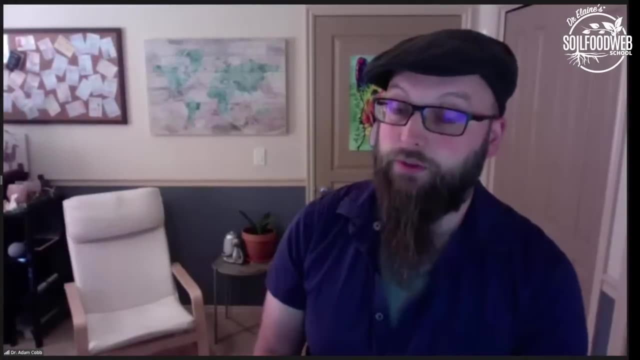 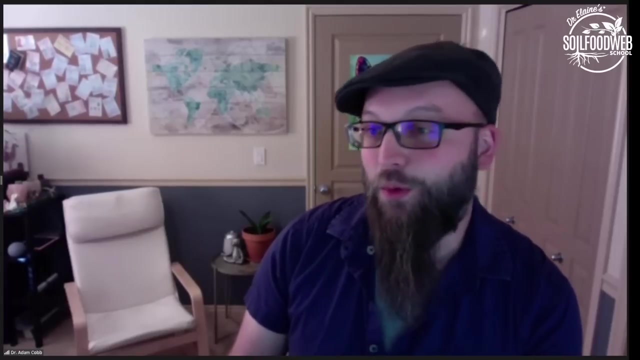 in how these these systems come together. we need the presence of every functional group. we need the abundance- sufficient abundance- and we need diversity. these are really the the supporting aspects of of a thriving soil food web. so again today we're going to talk about fungi, but they are not the only player in the soil. 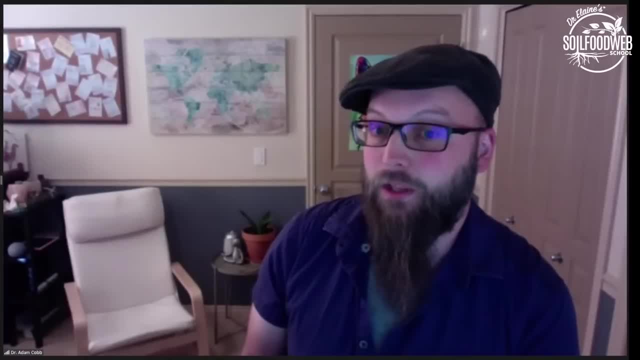 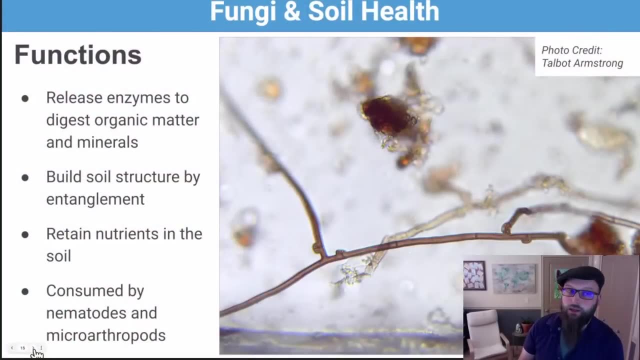 they do provide some very important um they. they fill a role that nothing else fills. in the soil. they have their own special contribution that they make. fungi are some of the world's most effective digesters. they produce enzymes that are very good at breaking down organic matter and sand, silt and clay minerals. 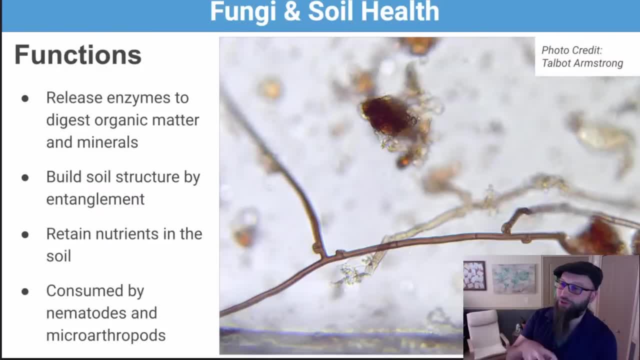 was it? dr lane said once that the nutrients can be in jail in the soil, in the fungi, along with bacteria, bacteria. but the fungi can be very good at getting those nutrients out of jail, out of the soil mineral complex, and then they incorporate those into their body. so as they grow, as they get the 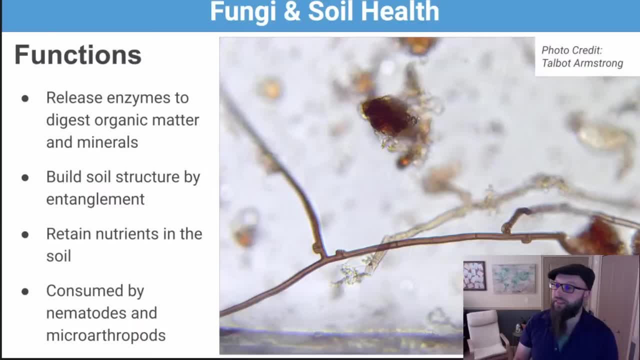 nutrition that they need. they grow and they entangle everything in the soil. they they grab little crumbs of soil we call micro aggregates and they stick them together into larger crumbs that we call macro aggregates. they add all of this structure. it's sort of like if the plant 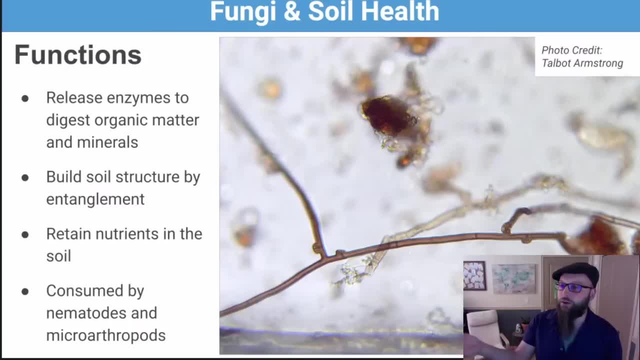 root were the highway, then the fungi you could think of as the side roads. right they're going into different, they're going deeper into the soil system. they're going at a finer scale than the roots and the bacteria and other organisms sometimes hitch a ride on the fungal roadway. 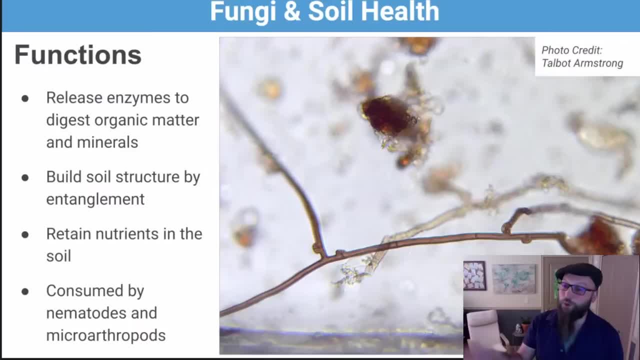 we see that they proliferate, they, they grow much more abundantly near those hyphae and because, uh, of the structures that fungi make and the, the entanglement that i spoke of, there's a lot of nutrient retention. there's a lot of carbon retention, when we talk about trying to draw down some of the extra carbon we have in. 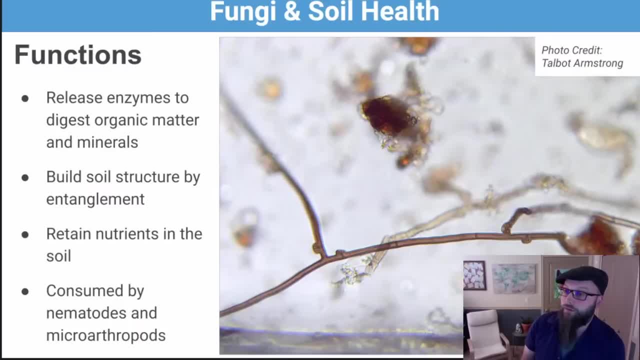 our atmosphere. fungi are a huge part of that of creating a stable, longer-term storage for carbon, but we don't necessarily want them to lock up those nutrients forever, which is why we need things like fungal feeding, nematodes and micro arthropods that will come along and say, hmm, i want some of that. 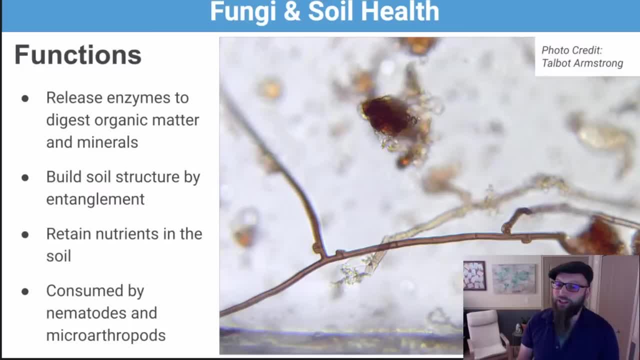 delicious juice inside of that fungi and they'll. they'll pierce the fungal cell walls or they'll shred them and they'll get at that those nutrients. but a lot of those nutrients get released so that the roots of the plants absorb them as well. this is the same thing that 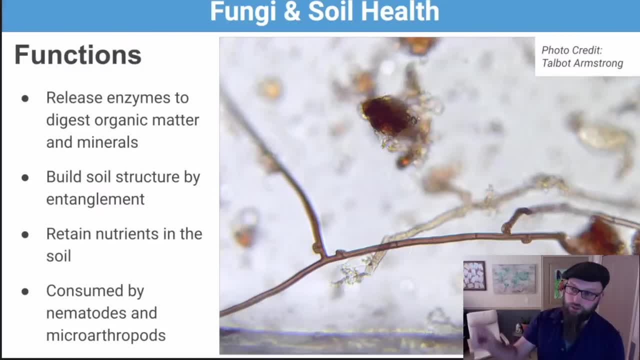 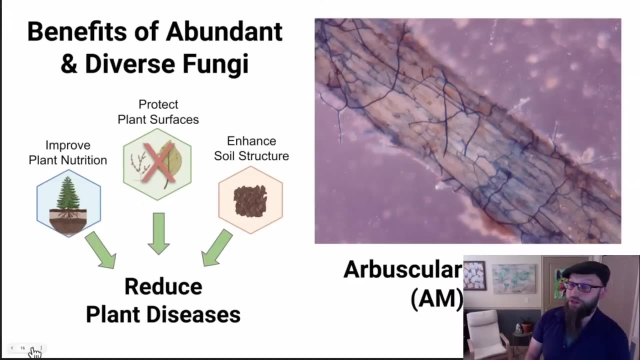 bacteria and protozoa and other things, is these relationships, this dynamic system where there's just a constant turnover and trickle of nutrients in the system so that the plant is fully nourished. The other ways that we talk about fungi here at the school is we like to highlight that. 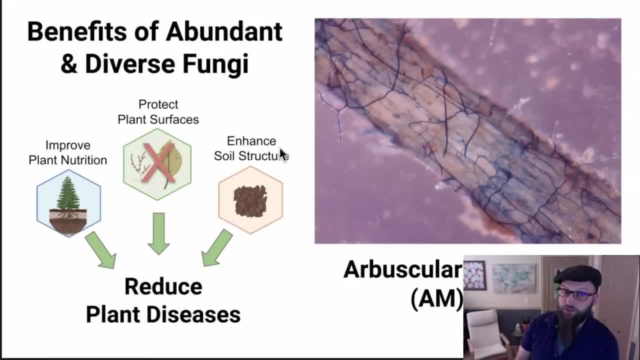 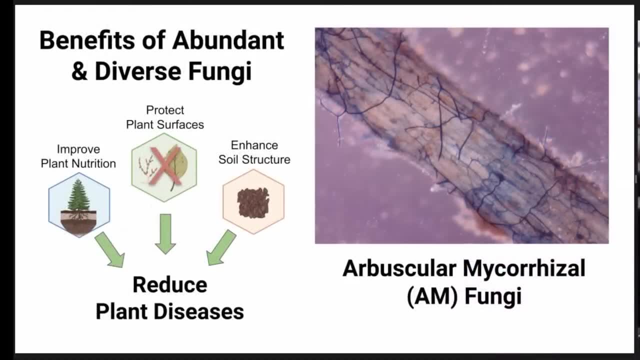 in addition to the soil structure enhancement that I mentioned, we can also put beneficial fungi on the leaf surfaces of plants as well, as they can crowd into the roots. This is a picture I took of some arbuscular mycorrhizal fungi, and they can armor those. 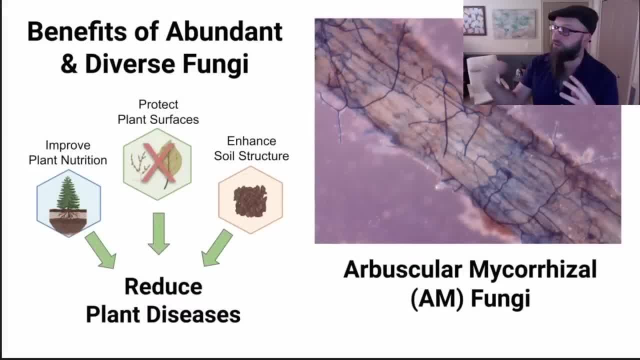 surfaces of the plants so that potential pathogenic organisms have nowhere to land and start attacking the plant, And then By improving the plant nutrition. it's sort of like when the human body is well nourished, the immune system of the plant is functioning well. so there's 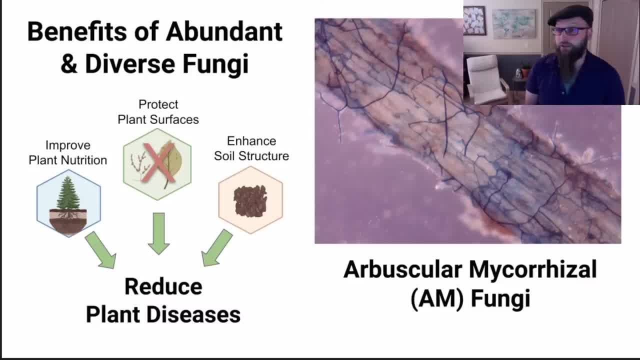 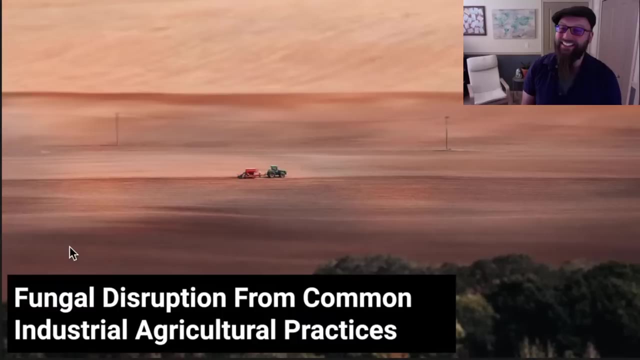 it's incredible benefit of having diverse and abundant fungi in the system. they they tend to regulate the system. they make the environment such that no one pathogen starts breeding out of control and and causing a problem. The downside of this Is that all of these benefits can be lost in industrial agriculture because things like tillage, heavy tillage of the soil- disrupt the fungal networks. right, think of if those fungi are sort of like long straws or tubes, then what happens when you chop those up and they bleed out and they die in the soil. 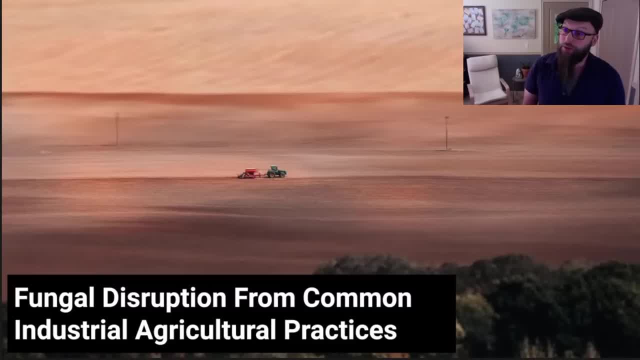 A lot of the agrochemicals that we use, The biocides, the synthetic fertilizers- those can disrupt the fungi in the soil. we see a big shift where Maybe we had 40,000 species of fungi and then if you do something like fertilize with a lot of nitrogen, that cuts down to 5000 species of fungi. right. these are some some studies that are out there that show agricultural practices that are commonly used can select for a less diverse 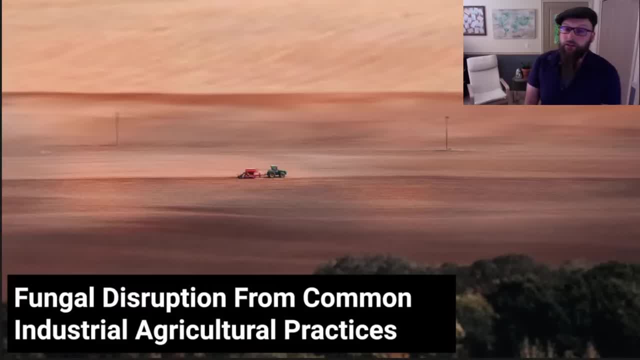 plant Fungi And then leading a field fallow is a huge problem. I passed a cornfield near my house the other day. he cut that corn for silage, He tilled right away and then the field is left naked, baking in the sun, and I can just hear all the microorganisms screaming. they're dying breaths. 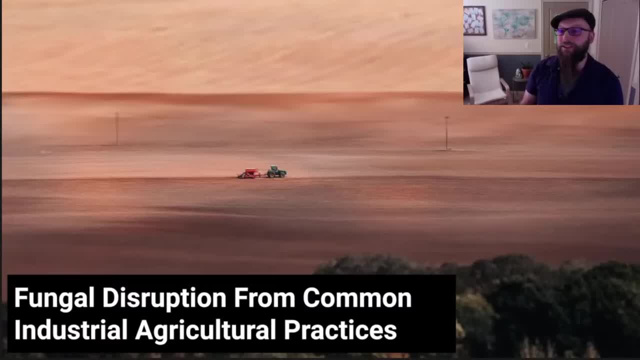 When I pass that field, because they've opened it up to the sun, The sunlight to the heat, there's not as much organic residue for things to eat. maybe the bacteria are kind of happy for a while at least, but the fungi are really suffering. in those situations we need living plants covering the soil year round to feed these, these diverse organisms. 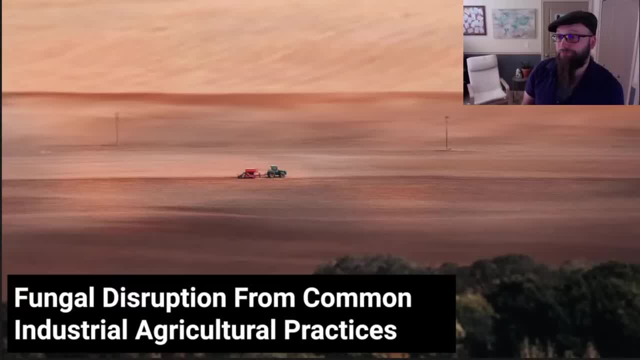 And monoculture. there's another huge problem: When he planted only corn that farmer, When he planted only corn that farmer, When he planted only corn that farmer, that corn might be feeding A few specific kinds of microorganism, but they're not producing all of the different hormones and exudates and growth factors and proteins and enzymes in the soil. 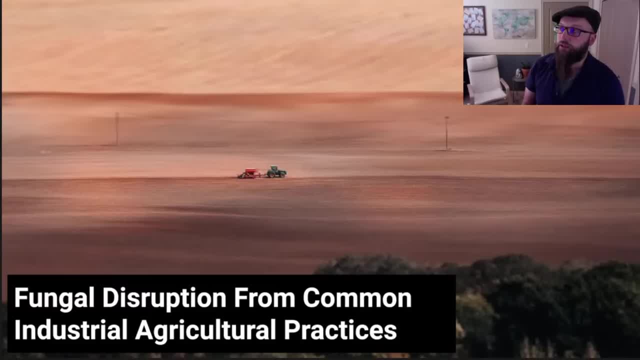 That you would see in a natural setting. right, if you go to a grassland, you would find maybe 16 species of plant every meter, every square meter, and those are all feeding different organisms. They're all producing different compounds, but the corn is producing one suite of foods. 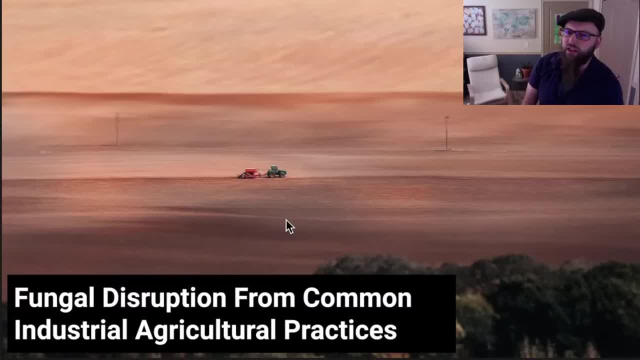 So these are, you know, just a few examples there and I know, Dr lane, that you- we talked about this yesterday- you may have had a few more examples, especially related to weeds. yeah, we've done a fair amount of work on what happens with the weeds. 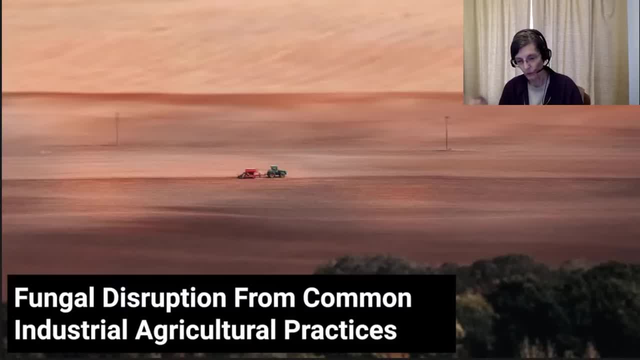 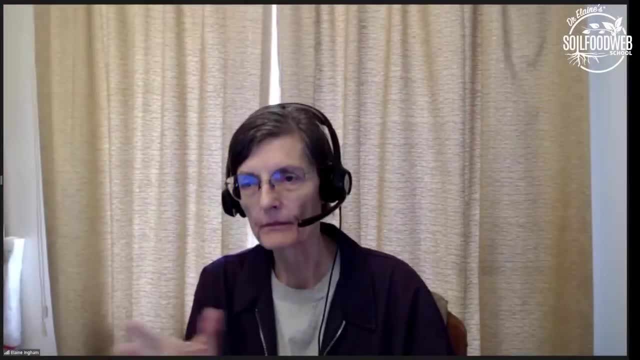 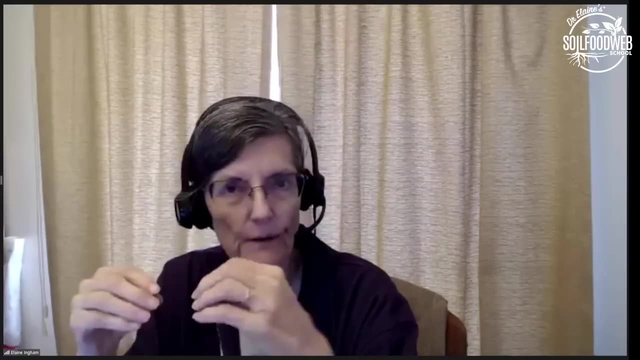 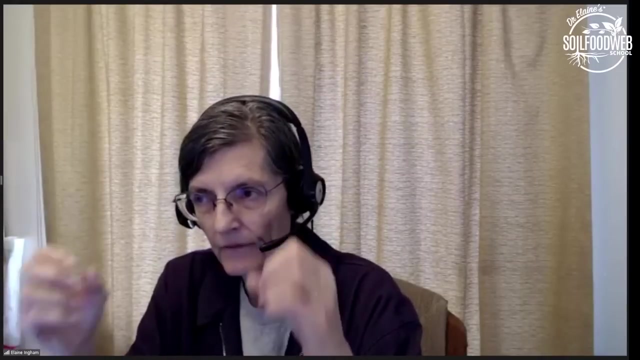 You first have to. when we're talking weeds, We have to define what a weed actually is. it isn't. the definition is not what nursery men or you know people in even the nrcs for, for example. they're saying that weeds are the plants that you don't want. well, so that with that definition, you're telling me that every plant on this planet is a weed. 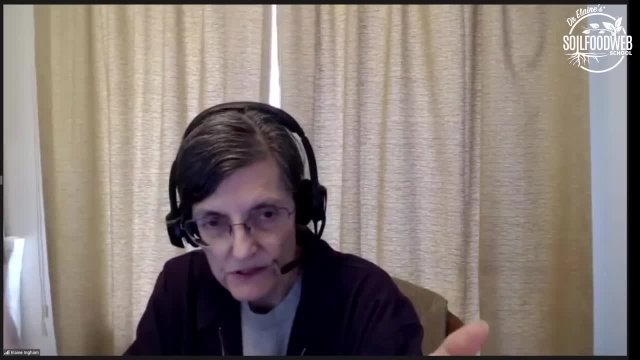 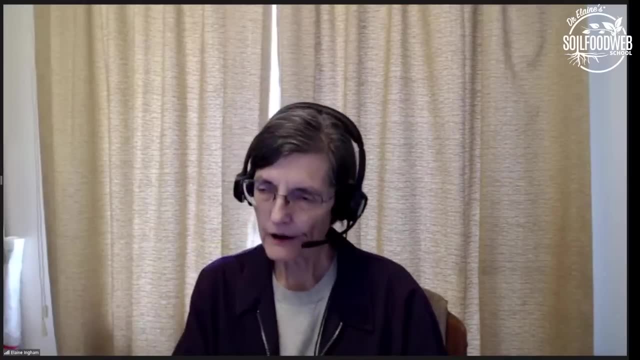 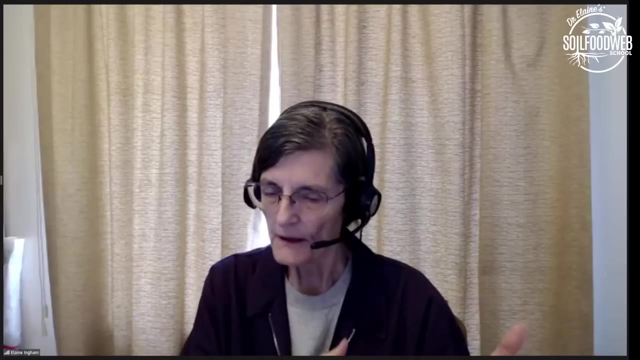 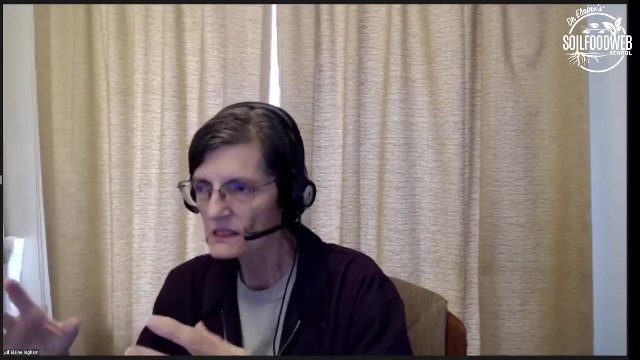 And so what uses that definition? it's totally pointless. let's go to the ecological definition of weeds, where it's our selected plants. but to you, what do I mean are selected? when you understand succession And you look at very rapidly growing plants that produce lots of offspring, lots of seeds, very rapidly they only put a small amount of their 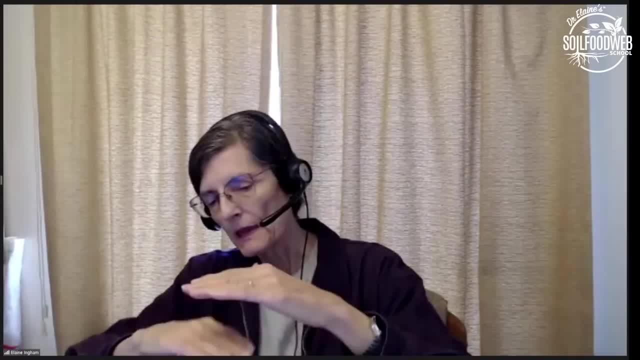 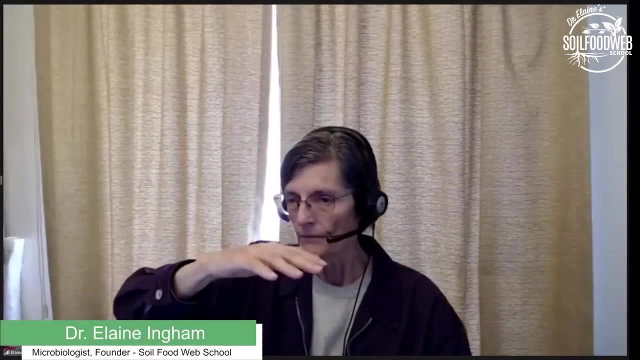 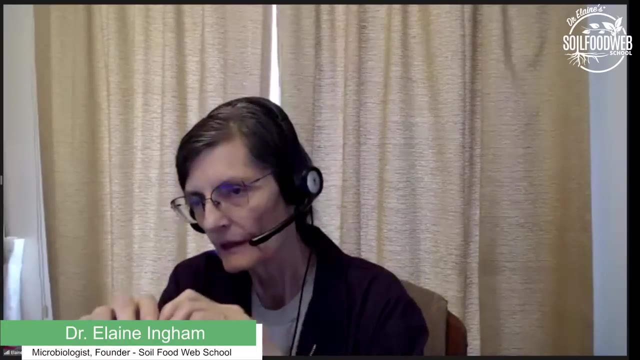 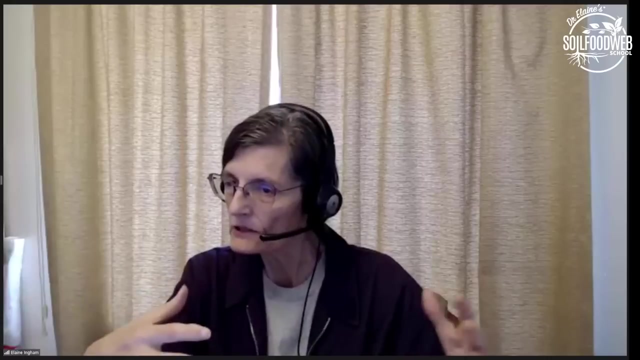 energy into the root system. So the roots may go down only an inch or two, even though you may have really good, healthy soil deeper. Those plants, the weeds, the true weeds- only put down a very light layer of roots and they send their roots sideways and fight with all of your different plants that you might have planted in your lawn or in your vegetable garden, or in your orchard or whatever. 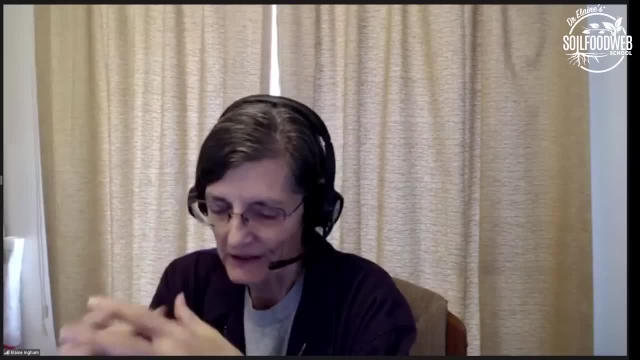 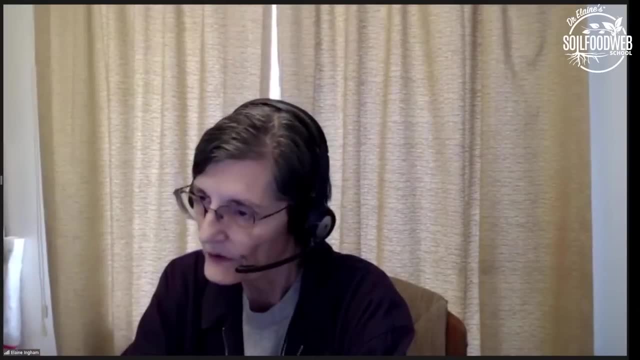 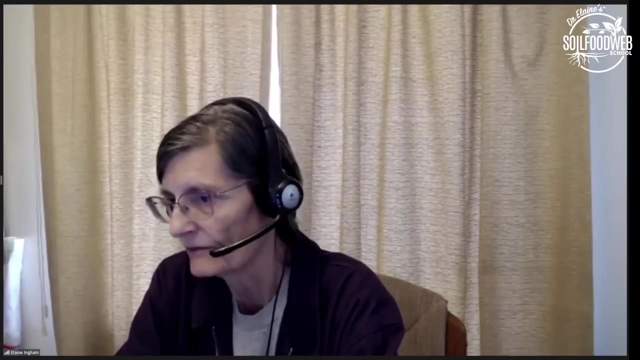 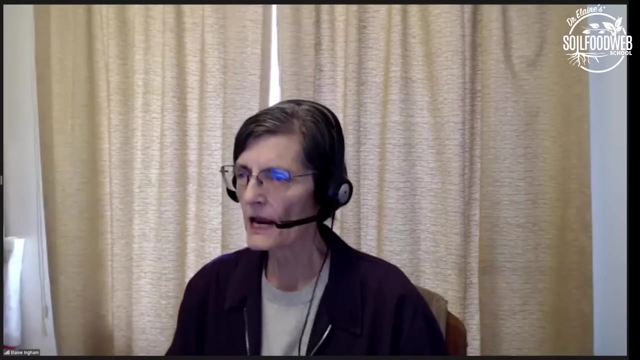 So they're very combative, if you think about it in one particular way. they grow very rapidly. they're going to suck up all the nutrients that those weeds will suck up all the nutrients that they possibly can and they win In competition with the plants you want to have growing, the crop plants. So how do you deal with those? well, how does mother nature change the soil such that at later stages in succession, 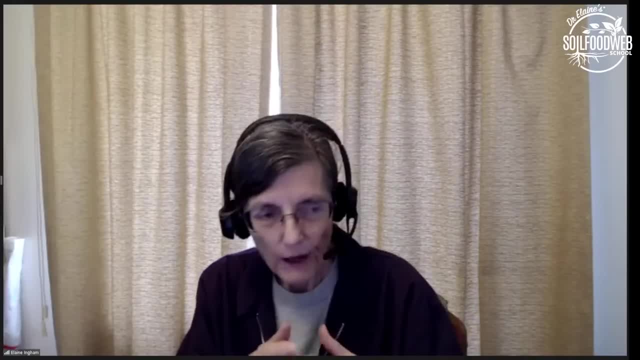 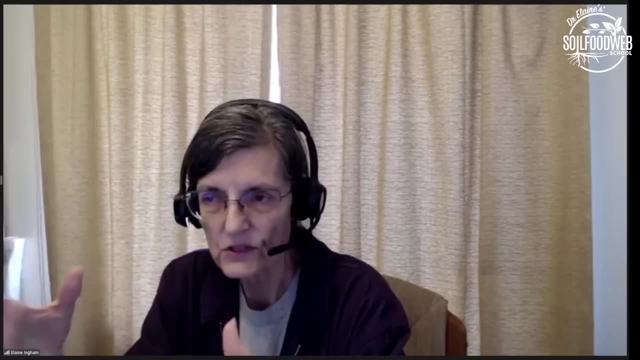 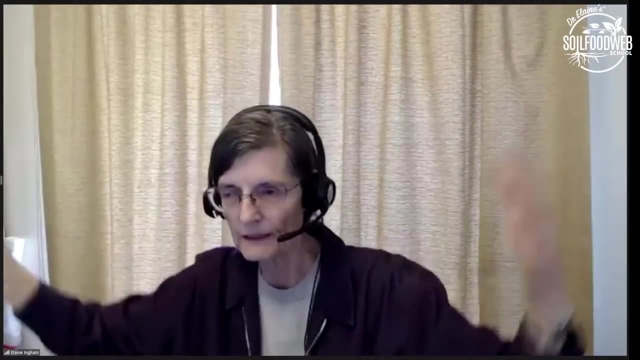 The weeds are not successful. if you've ever walked into a mature forest, there are very few weeds sit not going on the surface of that soil. you have all kinds of understory. you have the next layer, the next layer and then the overarching canopy. 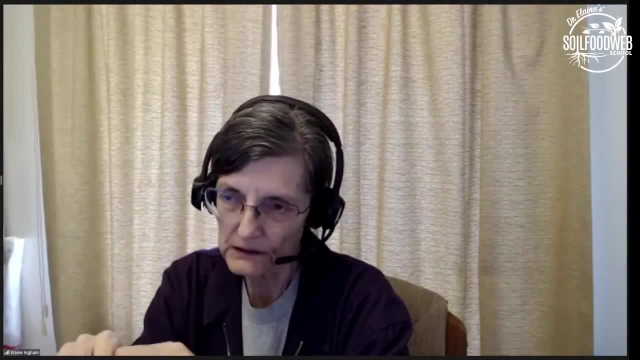 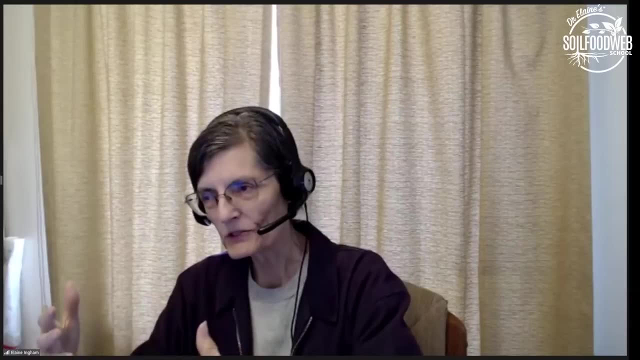 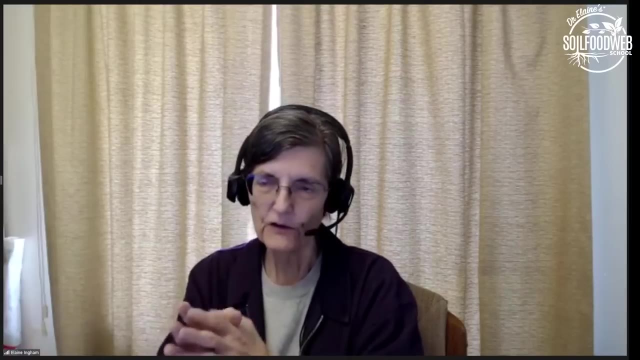 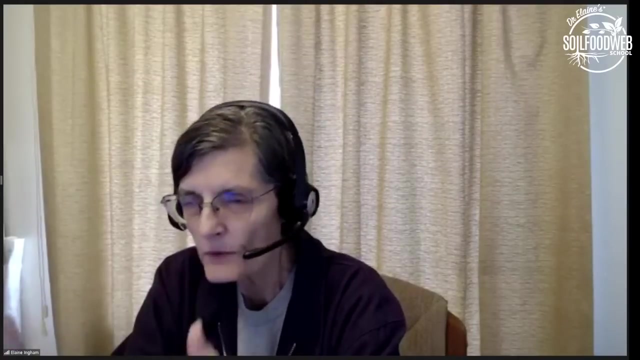 So what is nature doing specifically to control those weeds As a huge disturbance? Most of the biology is destroyed except for the fun for the bacteria, and we are left fungal lists in those early, severe, Contendant conditions where almost everything catastrophic, catastrophic, catastrophic disturbance. And so the only thing growing in that's all our bacteria eventually, and so bacteria in aerobic conditions will produce No three. they'll take all the NH four that is being released by the predators of the bacteria, and, as that NH four is released almost instantaneously, That NH four is converted into no three, and so that's the predominant form of nitrogen. in those early successional stages, where the weeds are so happy, almost nothing can beat them. Well, what's happened is that nitrate is what Weedy plants require. 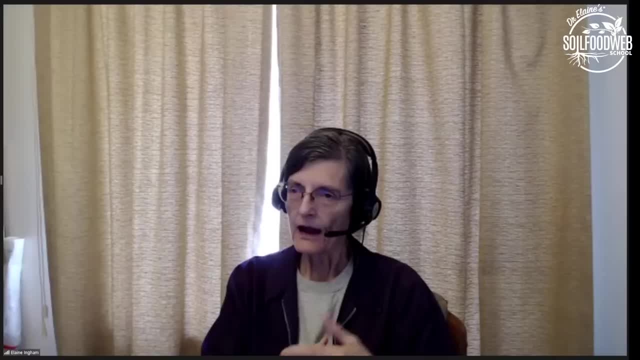 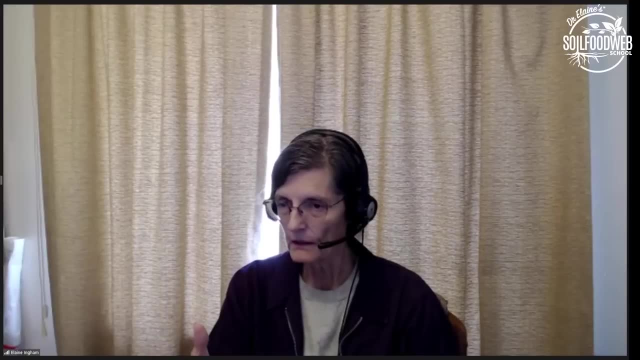 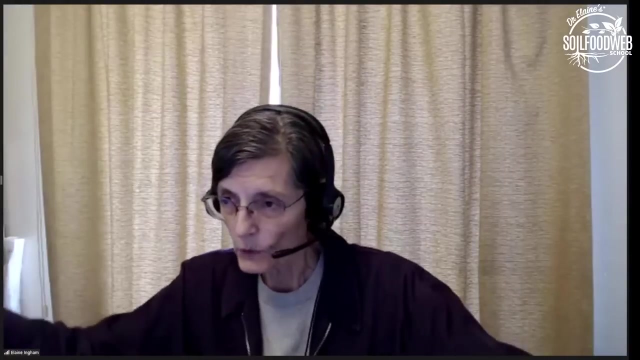 And so, as the bacteria are, start to share the scene with font of fungi. well, where the fungi coming from? and a severe catastrophe. They may have to come from hundreds of miles away or 20 miles away, and it's going to take time for those fungi to get there, but eventually they will arrive on. the scene, especially as plants start to grow, in those weeds is a lot of cellulose and that's the food that the fungi need. so as that component increases, then the fungi are going to start doing their job, And fungi are going to produce organic acids that drop the pH of the soil down to somewhere around. 66.5.. 66.9, somewhere in that range, and so now the nitrifying bacteria can't convert the NH four that's released with predator prey interactions. that NH four stays NH four, And the more NH four you have in your soil means that those weedy species, the thistles and the dandelions and all those things that you don't like growing. 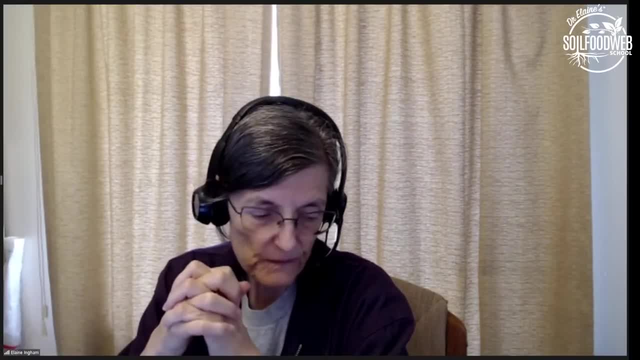 And so, as the fungi come from the soil, they're going to start doing their job. 66.1.. 66.2., 66.3., 66.4., 66.5., 66.6., 66.7.. 66.9.. 66.10., 66.11., 66.12., 66.13., 66.15., 66.16., 66.17., 66.18., 66.19., 66.20.. 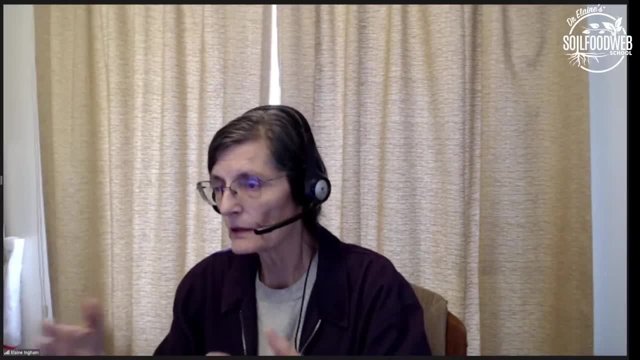 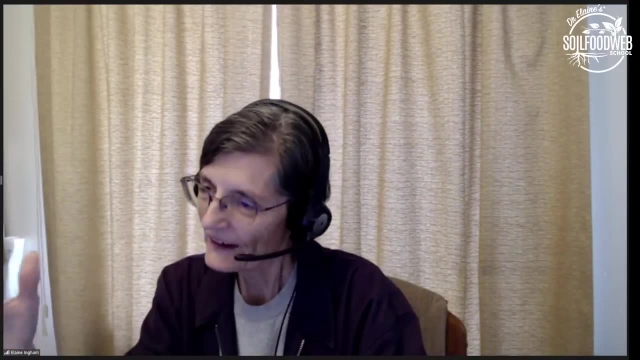 66.22., 66.24.. 66.25., 66.26., 66.27., 66.28., 66.29., 66.30., 66.33., 66.33.. We have to understand what we're doing when we have effects. 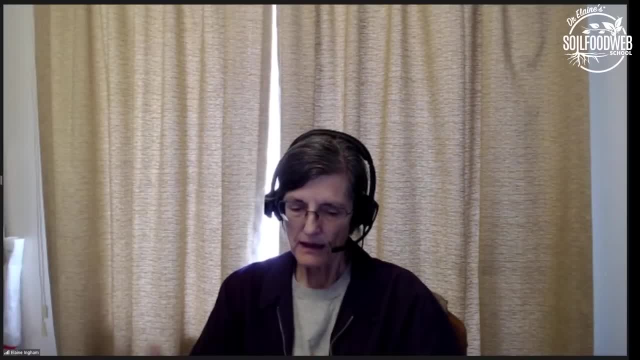 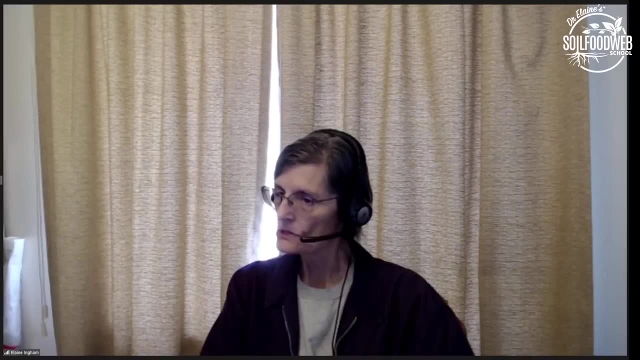 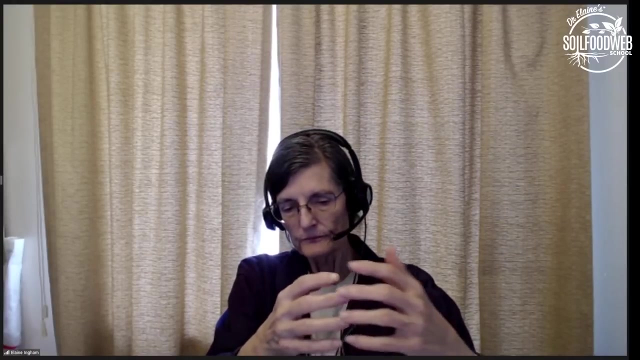 As soon as we go out and we start putting on fungi, the whole food web gets reestablished. We can watch the weeds disappear. It doesn't take long And we've done a number of studies where we have the original: the normal management of. 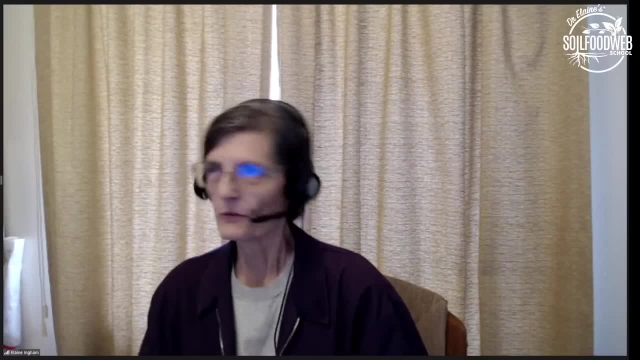 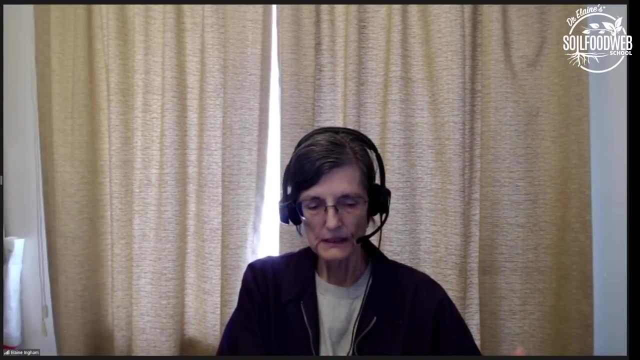 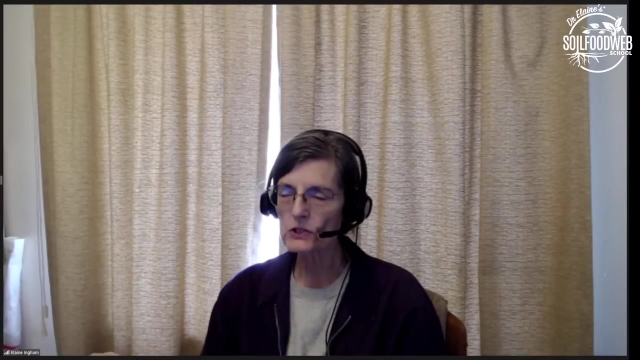 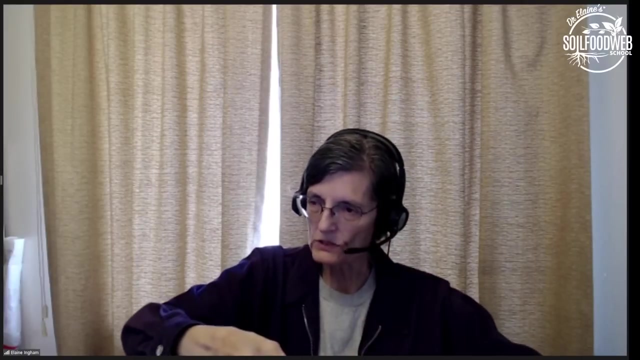 the toxic chemicals is the way I usually say it. so typical way of growing plants for the last 50 to 100 years. And then right next to that, we have plots where we have been putting on all of that biology And then we measure how long it takes to. you know, just a circle that we throw into. 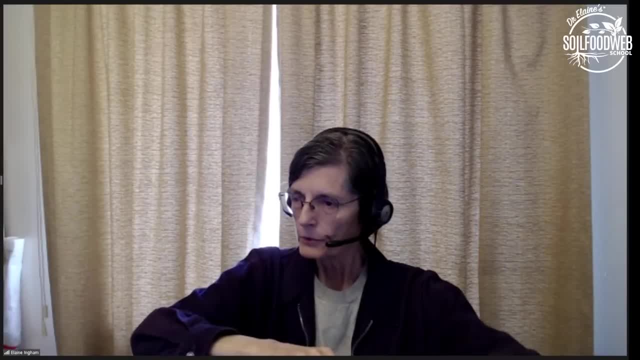 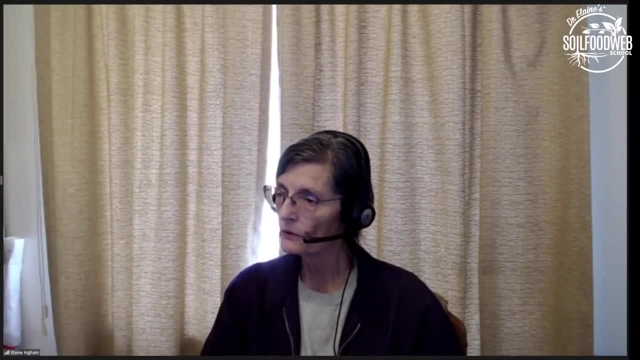 that plot And we'll go and pull out all of the weeds, The weeds in that place, And measure the time that it takes for you to pull those weeds As compared to where we're putting in the biology. we have the bacteria and the fungi. 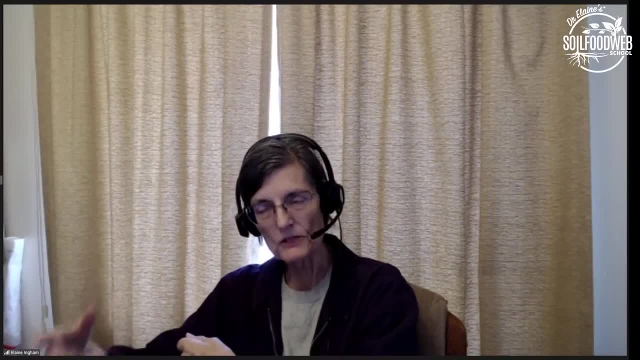 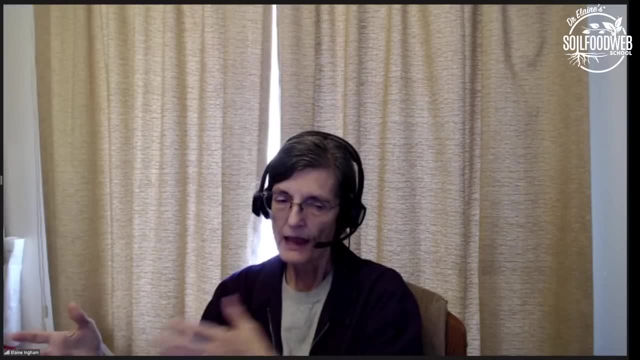 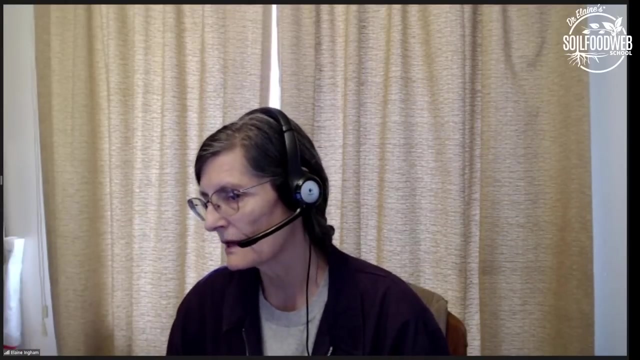 protozoa, nematodes, microarthropods, et cetera. And so we measure the same thing: How long does it take for you to pull all the weeds out, And how many weeds are there? And it's usually an order of magnitude: less time, less individuals. 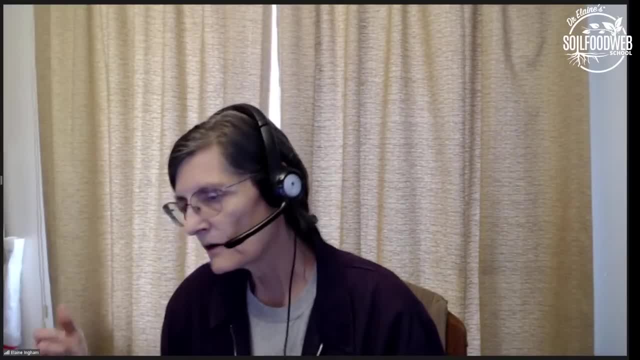 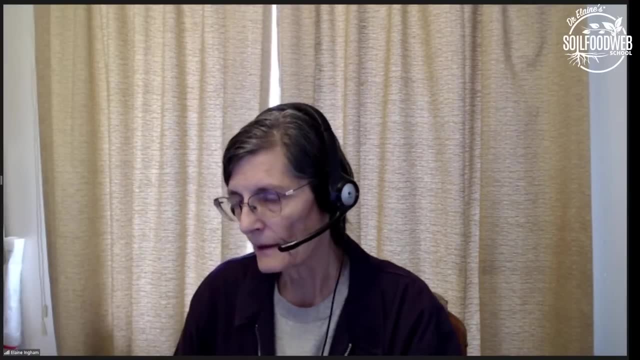 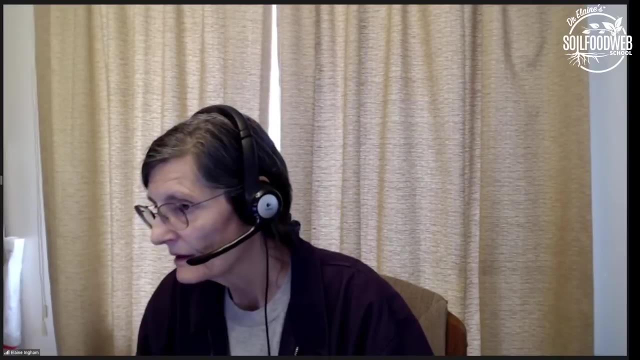 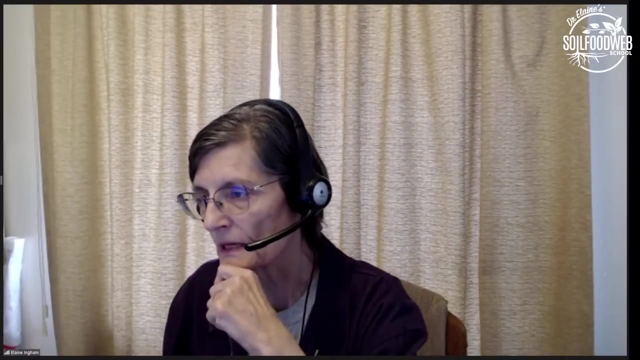 Of whatever weeds you've got in the system an order of magnitude less. You go from having to spend an hour in the chemical plots to only having to spend five or six minutes, perhaps a minute, to pull out all the weeds. That's how different those systems are going to be. 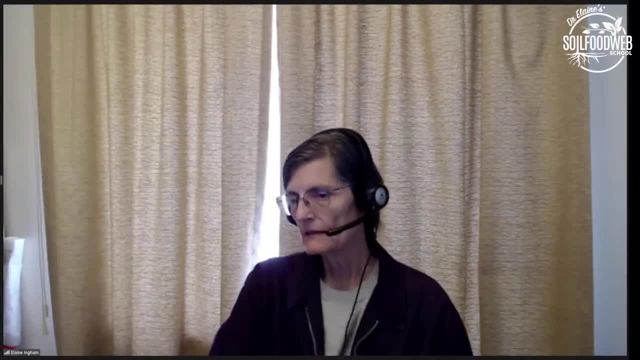 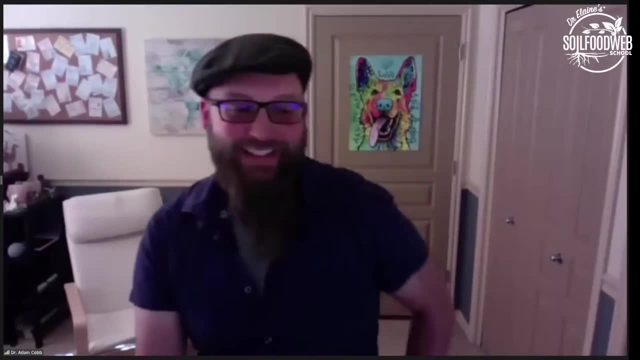 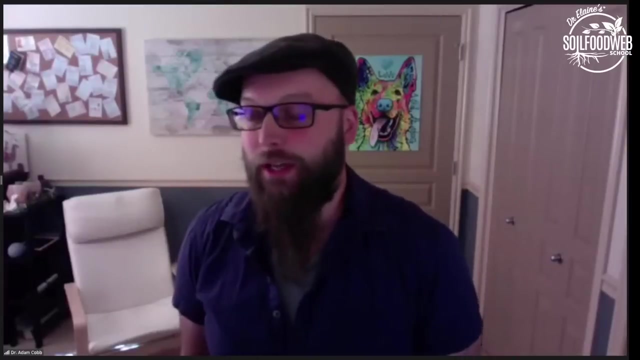 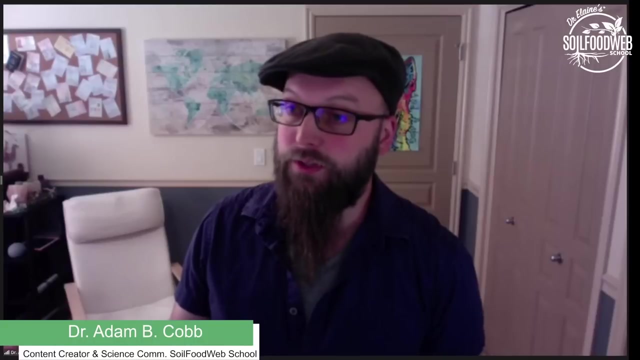 So understand what nature does And start using it to your advantage. Back over to you. Oh, thanks for that. Yeah, I love thinking about the way that this goes together with some of the things that I've seen in the world. So there was a time I was working to help reestablish some native plants in a formerly 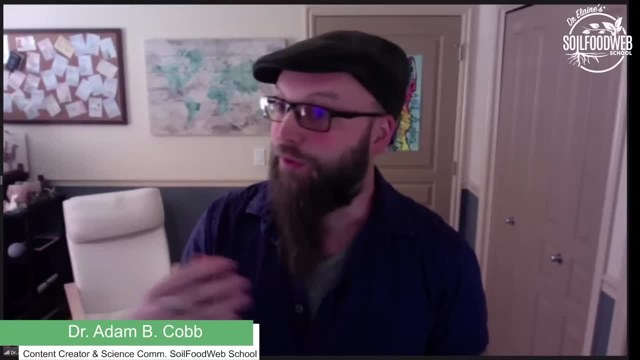 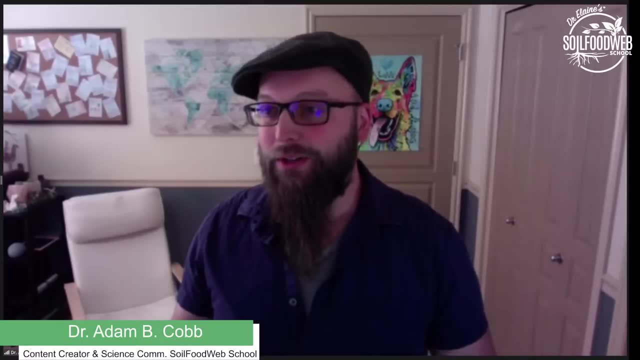 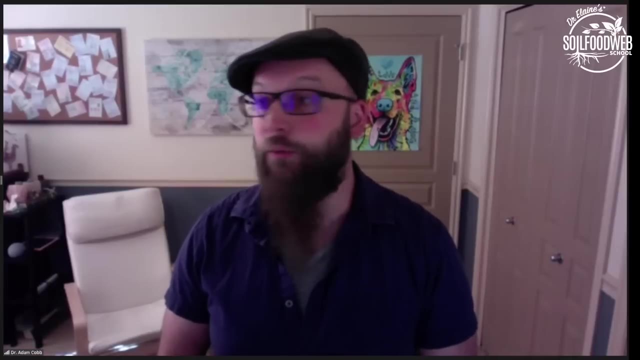 disturbed part of the prairie And in the first couple of years there was a lot of ragweed And annual sunflowers that popped up and really aggressive species, like you were saying, Quick reproducers. they got started before everything else in the season. And then, as we restored the arbuscular mycorrhizal fungi and brought in some nurse plants that had that relationship established, we saw those annual species kind of. you know, they didn't have the roots, Yeah, They didn't have the right context anymore. 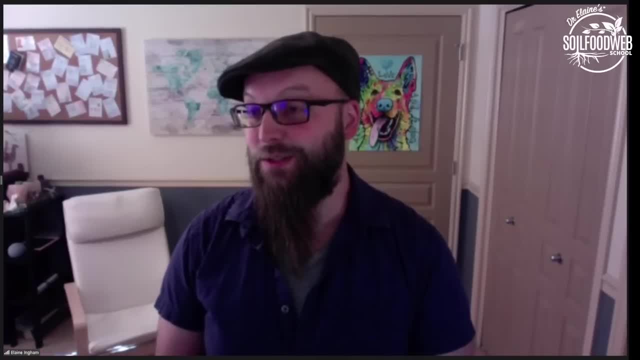 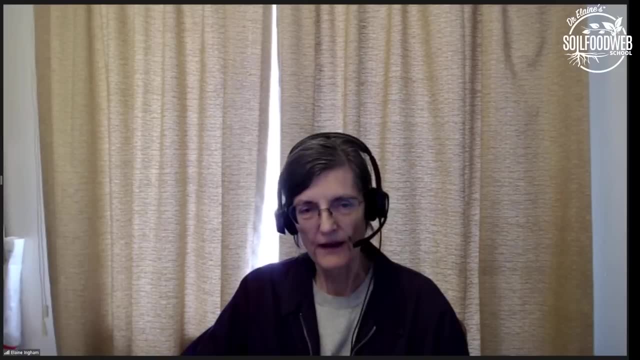 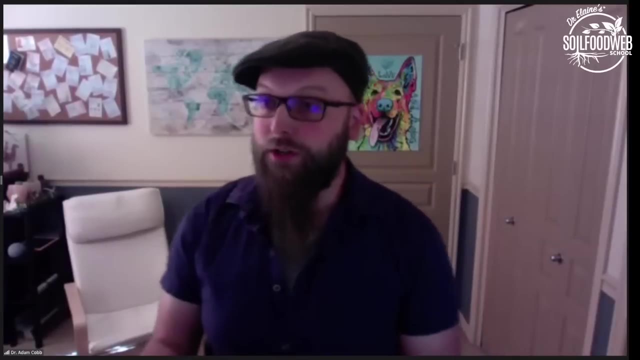 They didn't have the environment that they wanted. They can't get the nutrients that they need out of the ground because they're being outcompeted for that space, for those compounds, Exactly. It's really cool, Okay, so what Dr Elaine has primed for us is this thing: 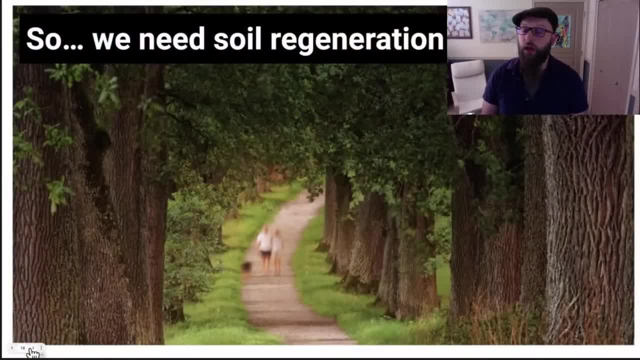 We have a pathway. She's discovered a pathway to help us get from here. If here is this really This really disturbed dirt that's from the typical, you know, poorly managed farmland all the way back to a beautiful soil ecosystem, right. 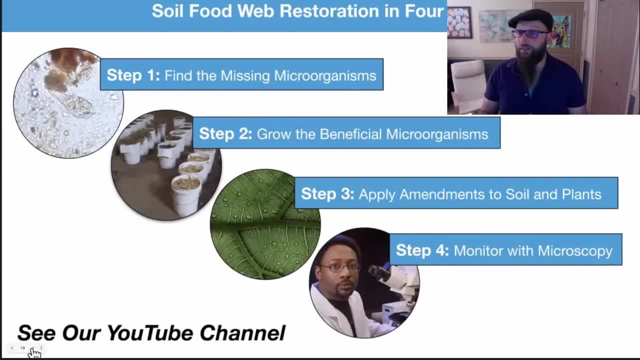 That regenerative process And this is the breakdown of that in just four steps. There's, especially from January, more details on these steps on our YouTube channel, But we're going in there and actually assessing what's missing From the soil food web. 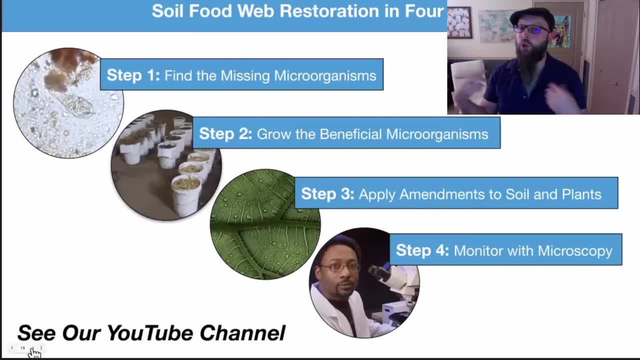 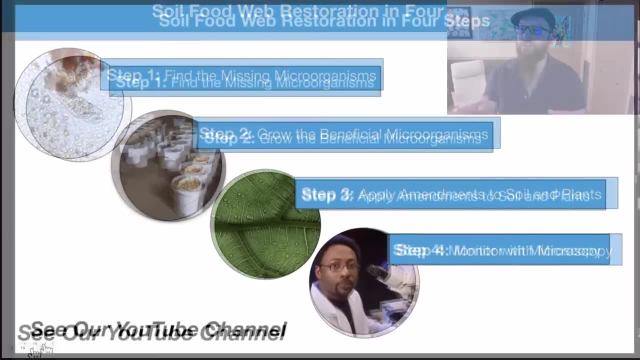 And then we're finding those missing microbes that are locally adapted. right. They're from local materials And through a specialized composting system, which is thermophilic aerobic composting, we make an inoculum. that's just. It's not even that the compost is adding that much nutrition, although it adds some. but 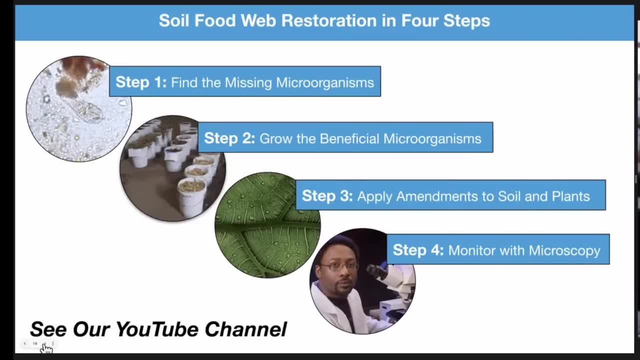 it's chock full of all of these diverse abundant nutrients. Yeah, Missing components of the soil food web. We can even take that compost and then make a tea or an extract with it, But in some form or fashion we apply that amendment like an inoculum to the soil. 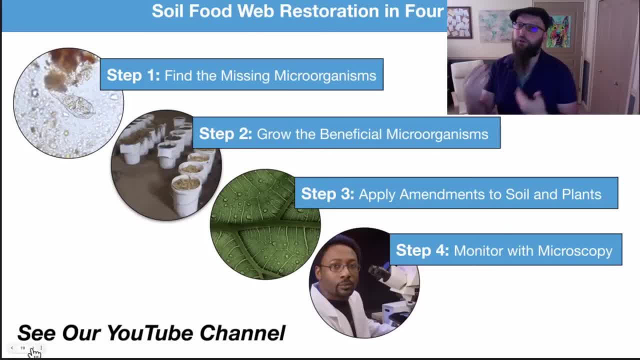 to the plant surfaces And then it reestablishes these missing microbes and these broken relationships. It gets the system back to health, right Back to where it's- The dynamics are positive, Yeah- And where there's all the functional players that we need. 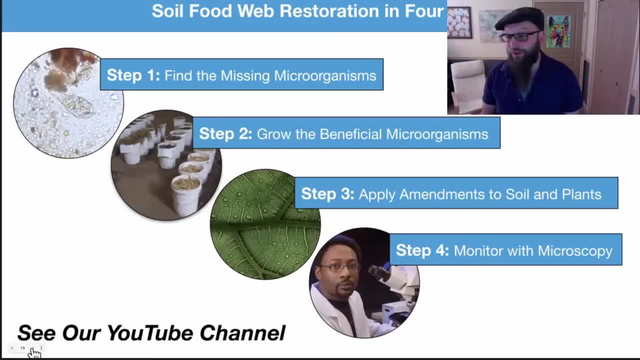 And the microorganisms do the trick and we really just monitor them. We use the microscope to say: I tried doing this agricultural practice. what effect did that have on the soil food web? I applied this product. what did that do to my microorganisms? 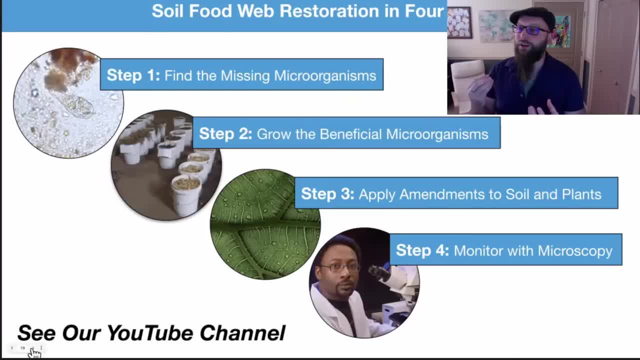 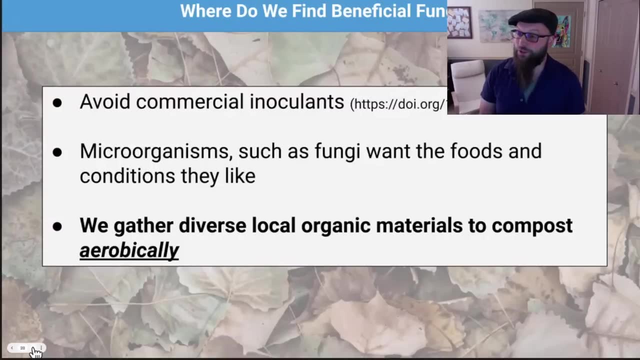 We're constantly going back and asking of the microorganisms be our indicator. Are we doing the right thing? Are we doing the wrong thing right in the soil systems? So there's more information on that out there. I always like to, when I talk about fungi, make a big deal about how we should avoid. 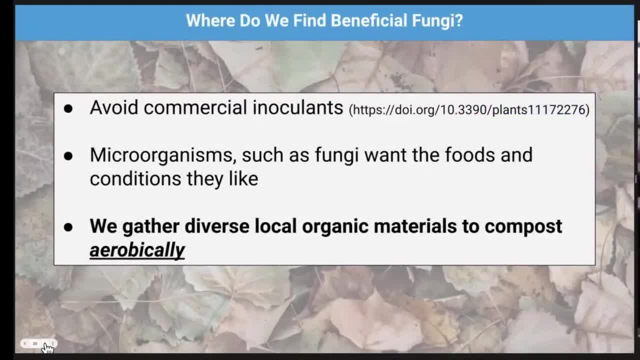 the snake oil. of many of the commercial inoculants on the market I only know of one or two that I would even try to experiment with, but this paper that came out recently. with Some of my colleagues and I we studied six commercial inoculum and we found in some 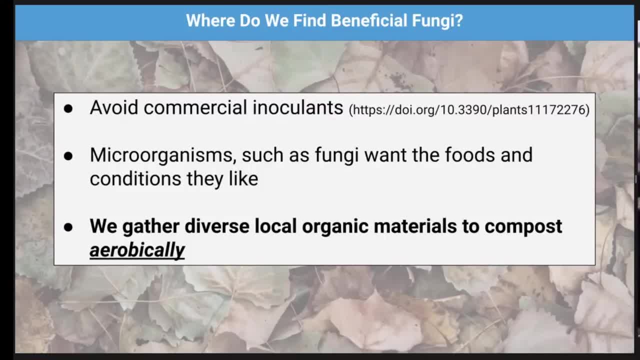 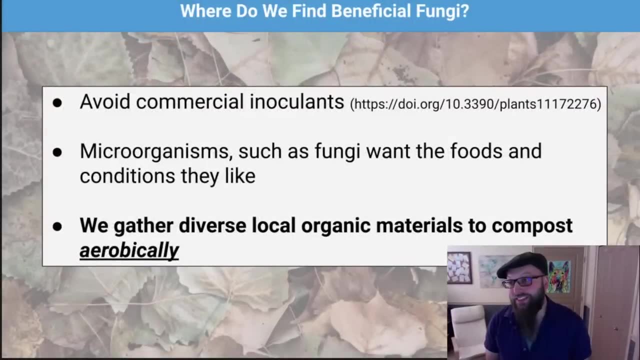 cases that they actually encouraged the growth of the invasive or weedy or the plants that we didn't want in a grassland system, And many of them had high levels of nitrogen and phosphorus in the carrier. So they said this is just a fungal inoculum, but actually there was fish meal or something. 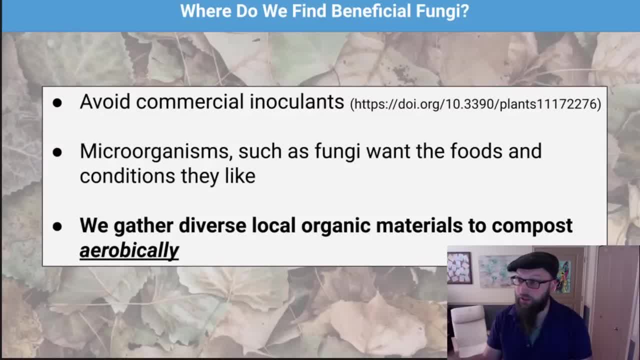 that was maybe even synthetic nitrogen added, And so we saw really high levels of nutrients which can actually further disrupt these relationships in nature. So we're looking for those microorganisms like the fungi. what do they want? They want foods that they like to eat. 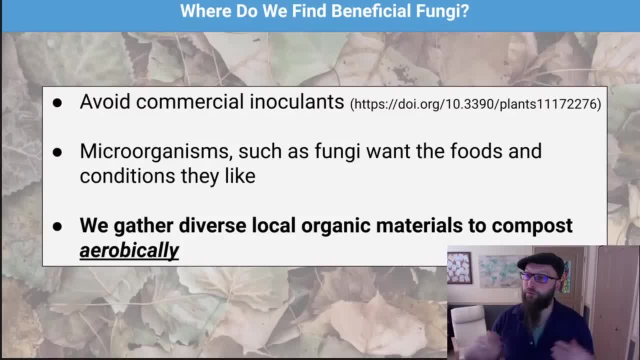 They want conditions that they like to grow in. We can go find these organisms in our local environment Instead of buying that commercial product that won't be very good. they're colonizing the surfaces or the roots of lots of plant materials around in our environment. 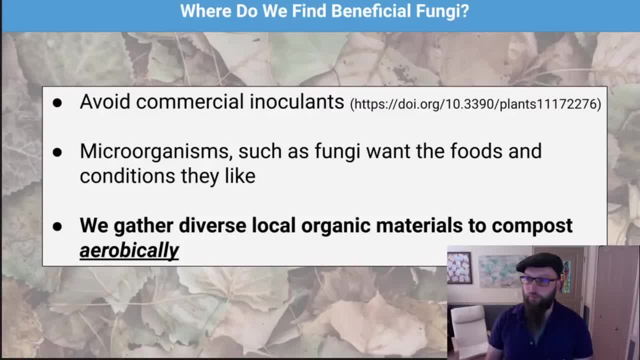 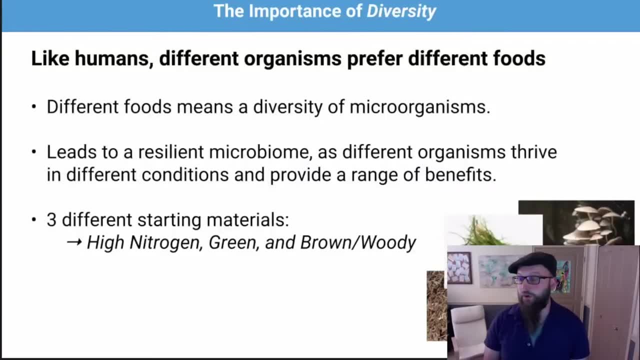 So we gather diverse local organic materials and we compost them aerobically, And this is a huge part. We introduced this in the foundation courses, But in our advanced programs here there's a lot of instruction and mentoring and people like Carla are working. 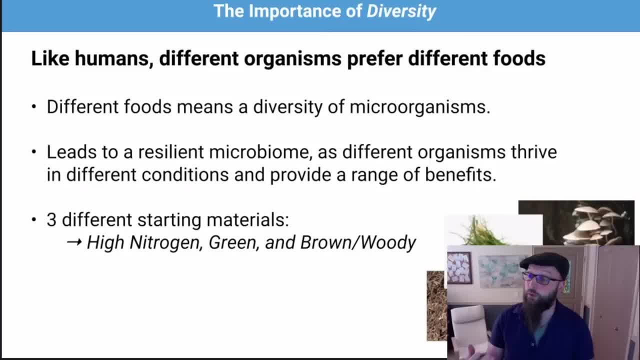 Hand in hand with people who are trying to figure out how do I do this composting thing correctly so that I get a really good inoculum at the end of it. So if we put a diversity of materials into a compost pile, that will help feed a diversity. 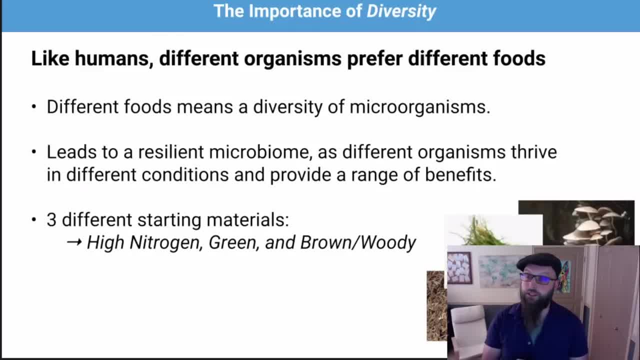 of microorganisms And that will help the entire ecology that we're adding back to the soil. the soil biology will be more Resilient, will provide more functions. So we have these three different starting materials that are really broad categories where we say we need some high nitrogen materials, we need some green materials. 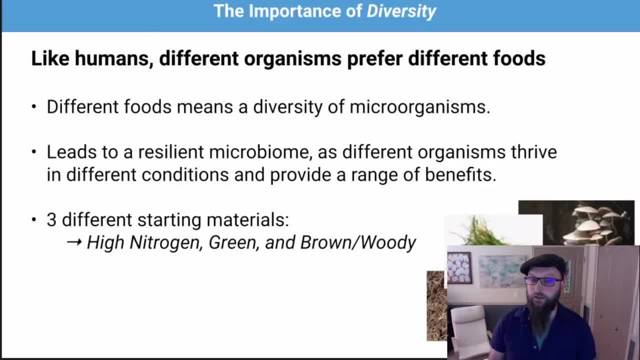 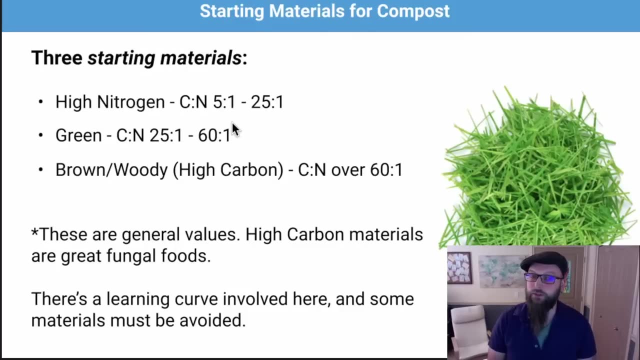 And we need some woody or brown materials. The woody and brown materials usually 50, 60% of our compost pile. Those are really good foods for fungi, And so What we're categorizing these different starting material groups is really based on their carbon. 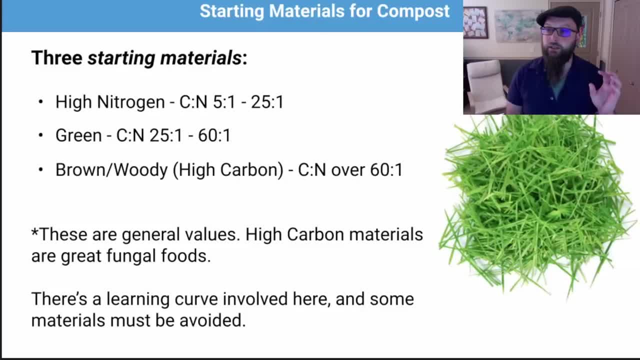 to nitrogen ratio. So for every atom of nitrogen, how many of carbon is there in that material? What's the comparison between the carbon and nitrogen And so high nitrogen materials we generally classify It's having about five carbons To every one nitrogen, all the way up to 25 carbon to every one nitrogen in the material. 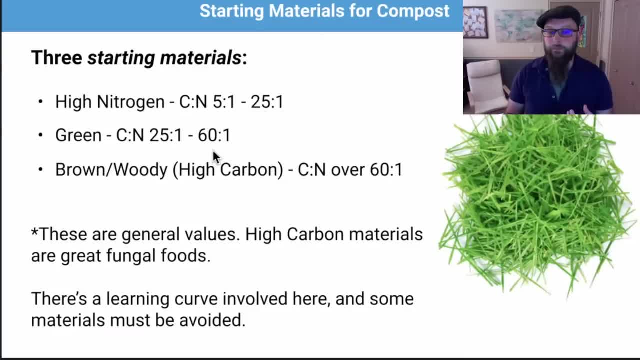 And then green materials. in addition to maybe being like fresher plant material- right In a lot of cases freshly cut, still full of all the juices- they tend to have a range that's a medium level of carbon to nitrogen. And then, as we get up into those brown and woody materials, 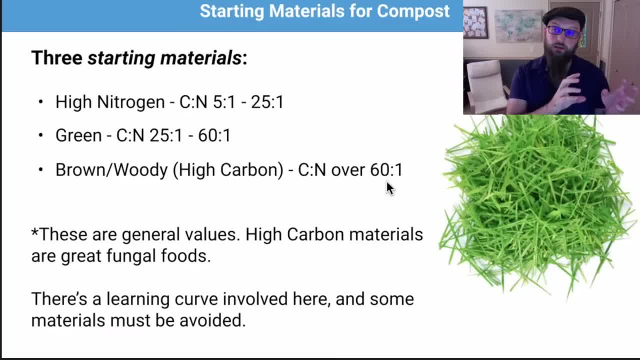 We're talking more than 60 carbons to every nitrogen. even up to you could do material that are hundreds of carbons to every one nitrogen- some of the hardwoods. So these are general values. You're going to have to poke around a lot on the internet to maybe come up with some. 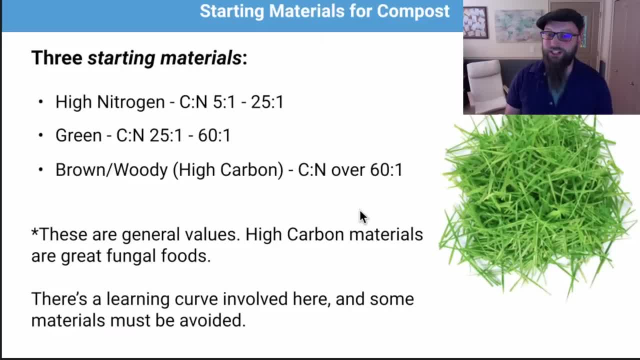 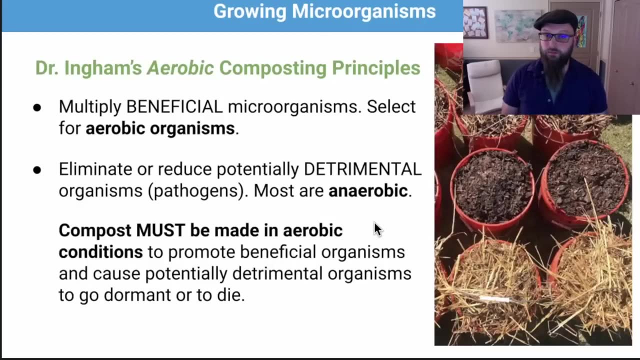 different ideas about what the carbon to nitrogen ratio is of the thing that you have, And this is a huge part of the mentoring that we offer as well. There's a learning curve here, But we're putting those materials into a system with the thermophilic aerobic compost. 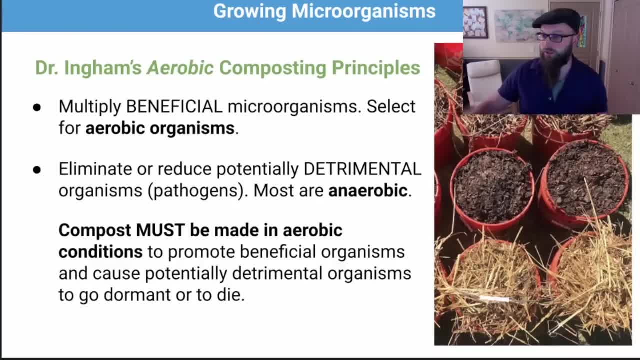 that helps filter out the anaerobic organisms that can cause disease. They don't have the environment that they like, So they shut down, they die, they go dormant, And it encourages these aerobic organisms that provide a lot of benefits to our plants. 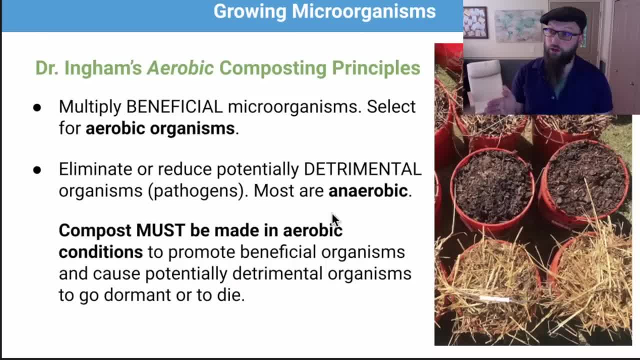 And it has to be thermophilic. Okay, Hot enough, long enough to do things like: kill the weed seeds, drive the detrimental organisms into dormancy. It takes a lot of care and effort to do compost this way, But on the other side you get an inoculum that is very valuable for regenerating soil. 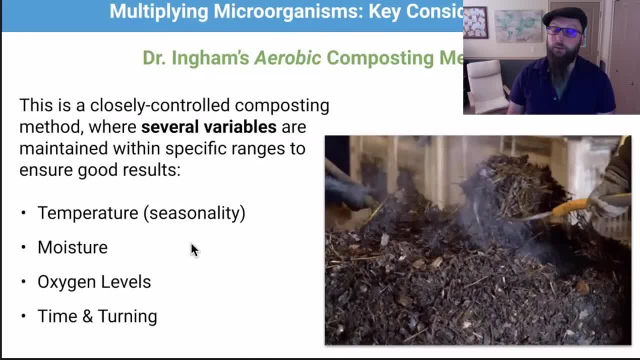 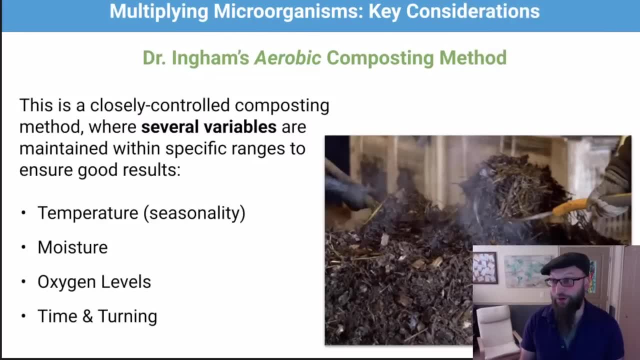 So not only are we controlling temperature, Okay, But we're controlling the moisture. This is a big one. A lot of people let their compost get too dry and they end up killing a lot of their beneficial organisms, The oxygen levels. we want to keep those oxygen levels high in the whole pile and not have 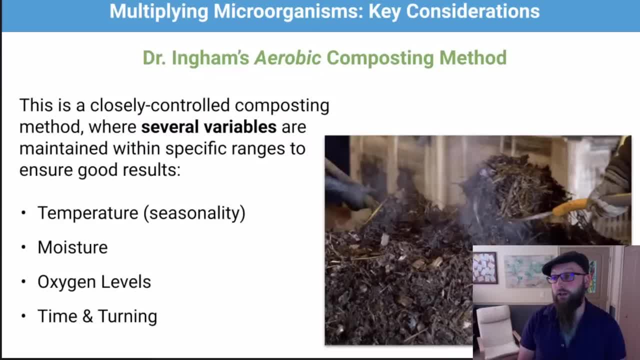 big chunks of the pile going anaerobic, which can be an environment for pathogens to enjoy those conditions. And then we need to have time and turning, So we need to make sure all parts of the pile Are hot enough, long enough in the hot center. 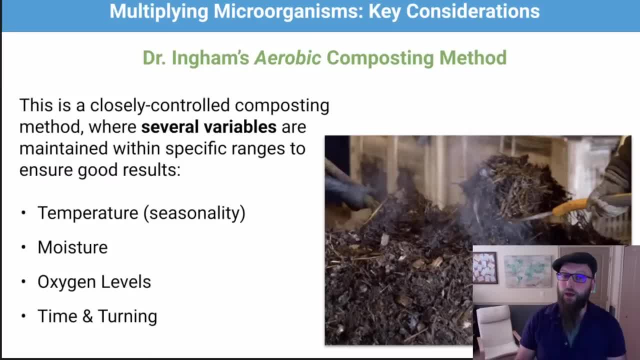 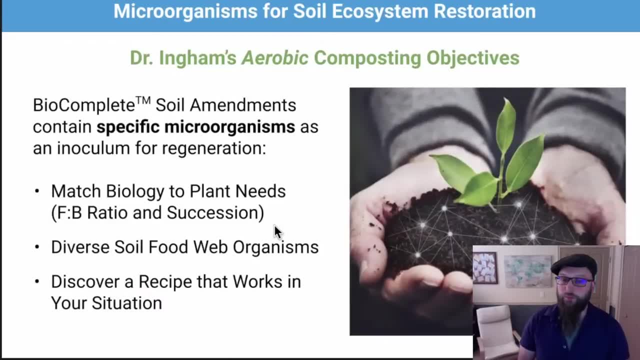 And then moved around so that all components of the compost pile spend time getting hot enough in the center. As a result of this, we get a diversity of organisms. We have to keep tinkering with recipes until we sort of find what works for each condition. 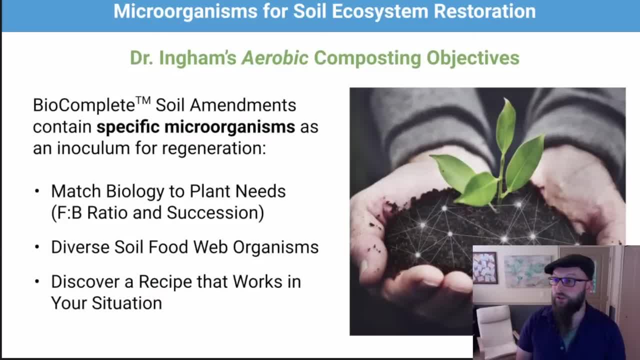 each area And you know one of the big principles, Okay, Okay, One of the big principles, as Dr Lane mentioned, is those early successional weedy plants. They're going to want a certain amount of bacteria to fungi in the soil. 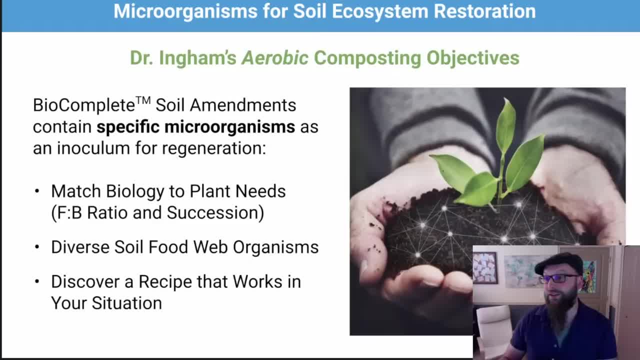 And many of our agricultural crops are going to want more like a one to one right. They're going to want about an equal amount of fungi to bacteria, And some of your shrubs and trees are going to want much more fungi than bacteria. 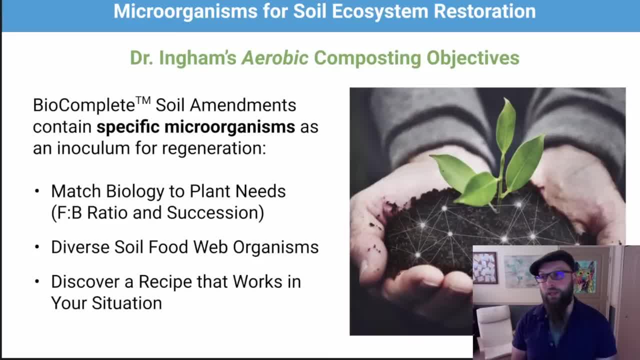 And so we have to sort of match the kind of Compost we're making to what we want to grow with it as well. So there's a lot of details, which is why we have these advanced programs here. People can be mentored in this. 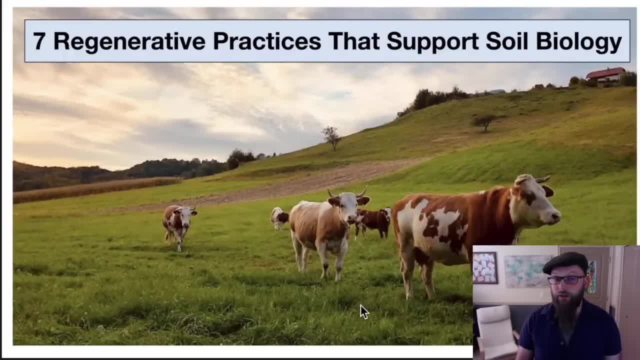 So this is my last few slides here. I think we have time before we get to the Q and a. Brian, don't let me cut me off if I am talking too long, but I just wanted to mention After we go through this process. 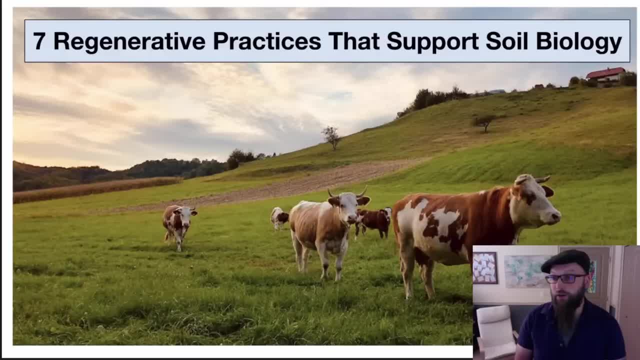 Okay Of trying to biologically restore the soil food web, We need to think through holistically how the whole system can either support those microorganisms or can harm them right. So we mentioned tillage earlier. If you're coming in with a rototiller every year into your garden, that's not really supporting. 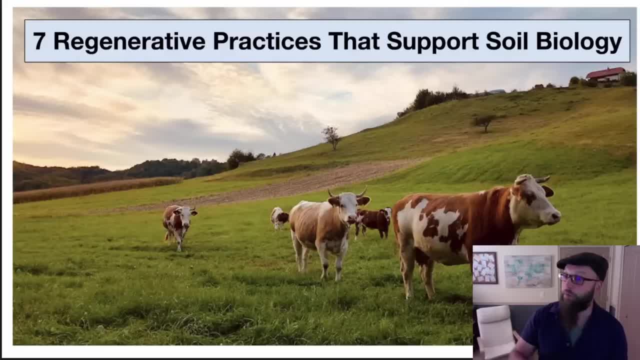 the microorganisms right, It's going to keep knocking those populations back, causing harm. And so these are seven regenerative practices that you know. this has sort of been out there in the scientific literature. in other we're getting inspired by other things that we're. 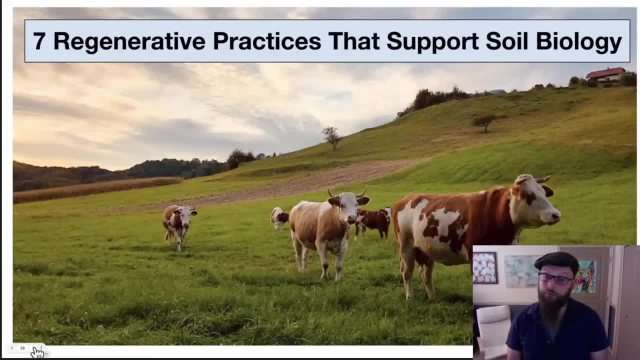 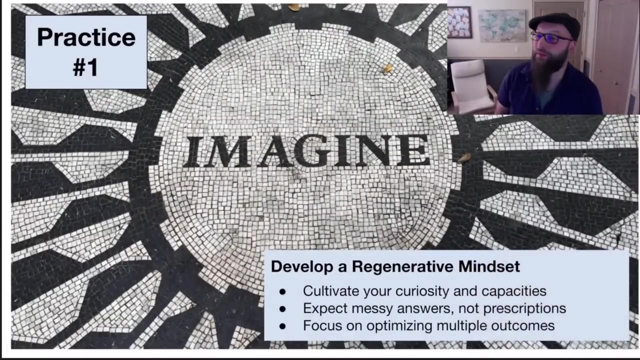 seeing in the regenerative ag movement and and filtering this through what's been tested on our end as well. These practices tend to be microorganism centric, Right They. They tend to enhance the soil food web And really the first thing, the first practice. it might not seem like a practical practice. 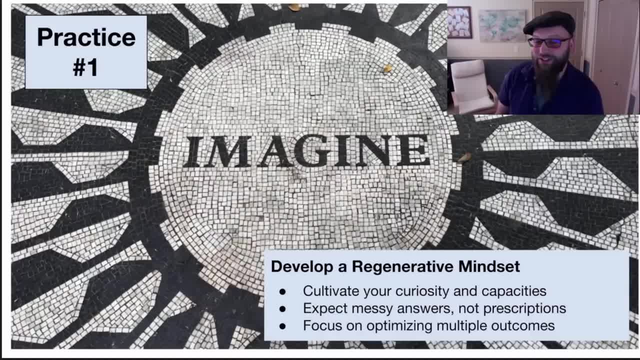 to you, but it is maybe the biggest challenge is we have to re, we have to develop a regenerative mindset, Those, those of us who are working, managing, stewarding any kind of land. It's about thinking through our relationship to that soil and to that land and to those. 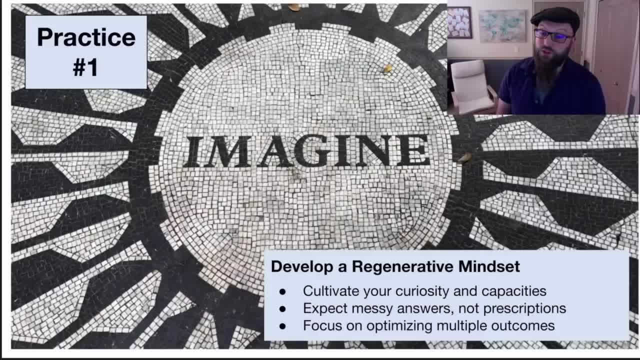 microorganisms and plants. So a lot of times people want us to just give them an answer and it's like there is no one answer. We need to teach you the principles. we need to teach you to use your, your eyes. You need to go and look at your soil, get your hands in your soil, smell it right. 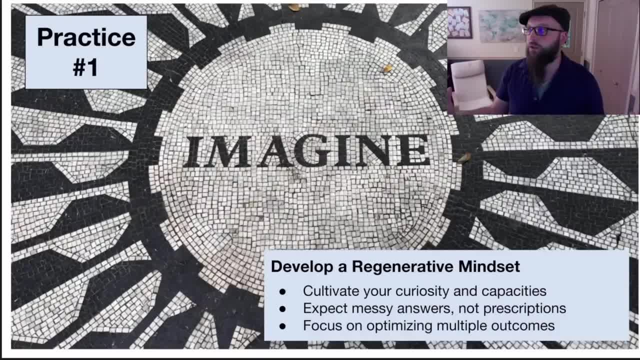 These are it's. it's taking a radical sort of self-motivation at play and recognizing that there's a lot of quick Answers, like chemicals that seem good in the short term and are not good in the long term. Right, So this is practice. 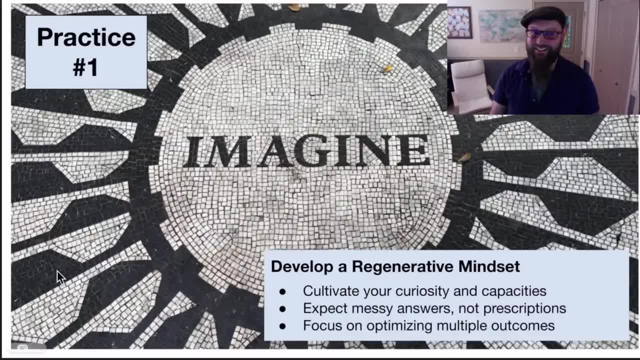 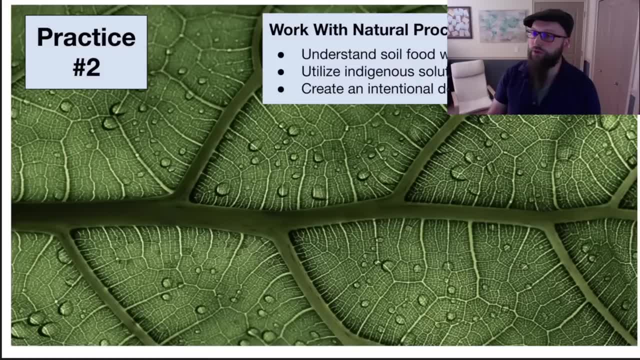 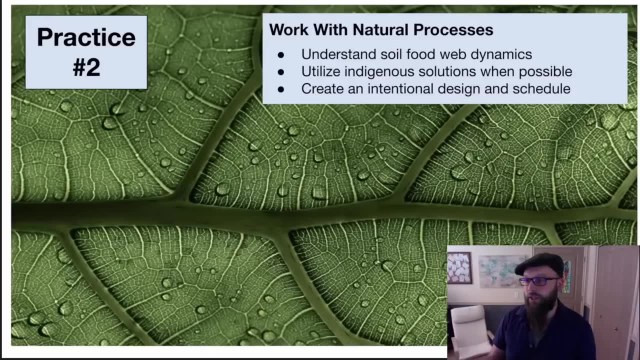 Number one our regenerative mindset, And part of that is that we understand that there are natural processes. Dr Elaine in the in the foundation courses she lays out the ecology of these organisms, how they interact with their environment, how the chemicals that they encounter. 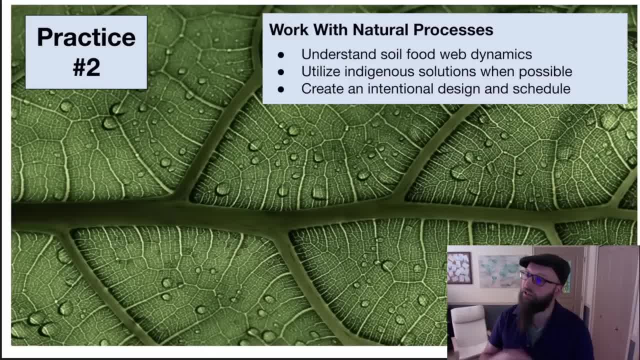 How the physical environment that they encounter influences what they do and how they interact with each other, And so we really have to- for lack of a better word. I'm trying to encourage you to fall in love with them right, To think of them as worthy of your time and energy, to understand those natural processes. 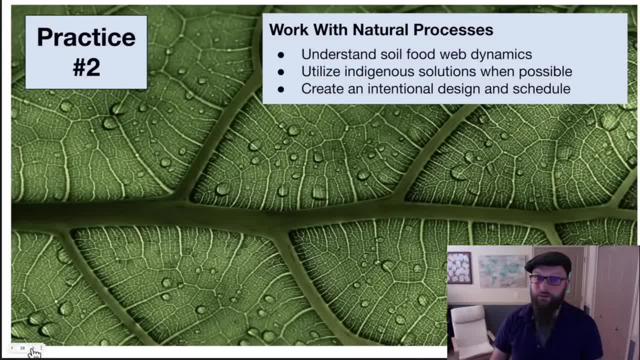 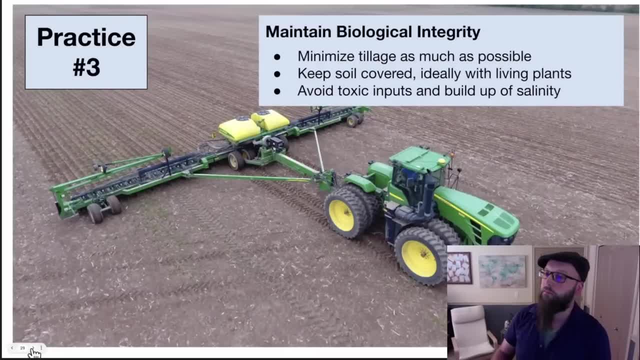 and those biological dynamics. And then part of that is- we've mentioned a few things. We've mentioned a few of these things before: maintaining the biological integrity, So minimizing biological disturbances like tillage, keeping that soil covered with living plants year round, avoiding those toxic inputs. 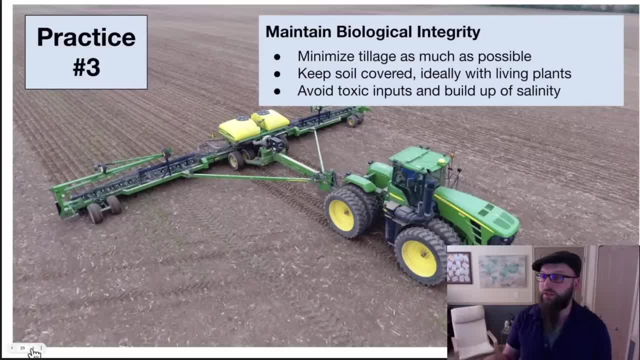 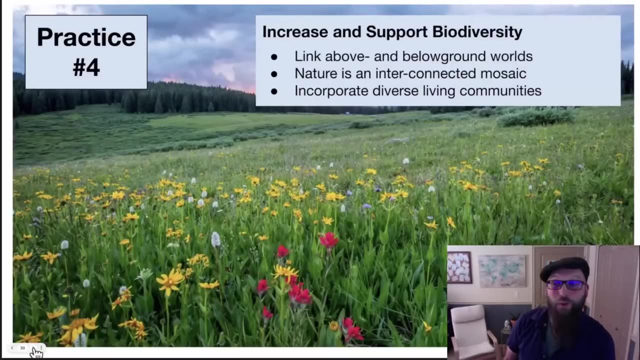 Salinity is a huge problem. There's lots of things that people use in soils that build up salinity- the level of salts, till the point that it becomes harmful to the organisms. So, understanding that biological integrity- Okay, Biodiversity- is almost always the right answer. 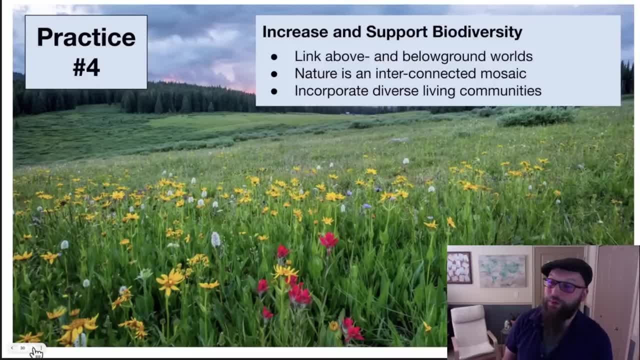 Get more plants in that system, more diverse plants. Make sure all of your organisms are there. You may have heard it said. as above so below, We tend to see a reflection that diverse soil microorganisms lead to plant diversity and plant diversity leads to soil microorganisms. 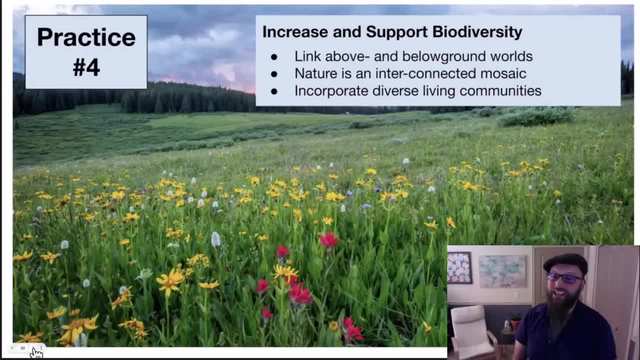 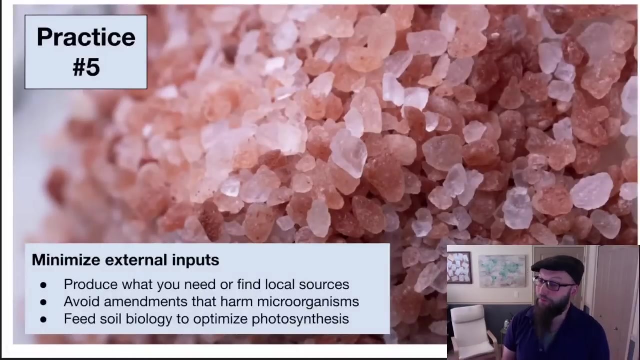 It goes back and forth right Between those two worlds. So incorporating animals into your system can be huge. They can help cycle nutrients more efficiently. There's a lot to go on here, but biodiversity is one of the most important. We say to minimize your external inputs other than maybe the compost, right. 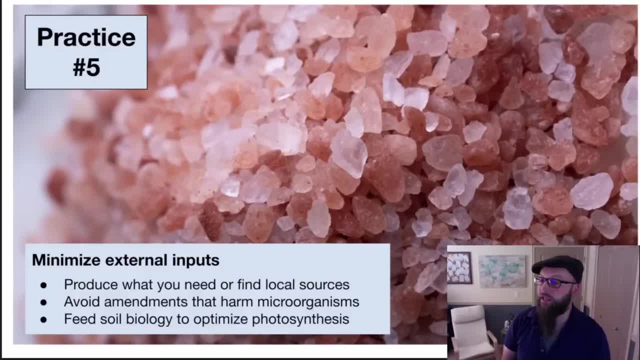 Getting something off a shelf- a synthetic fertilizer, a salt-based product, You know you don't want to go into that. You don't want to go into that. You don't want to go into that. These can be very harmful to the microorganisms. 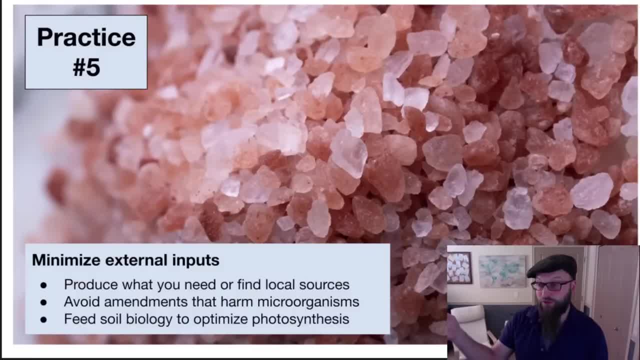 Those bugs in a jug, like I was talking about earlier- commercial inoculants. those can have harmful substances in them or they can just have not well-adapted organisms. So you spend all this money, you put this product on and then the organisms all die. 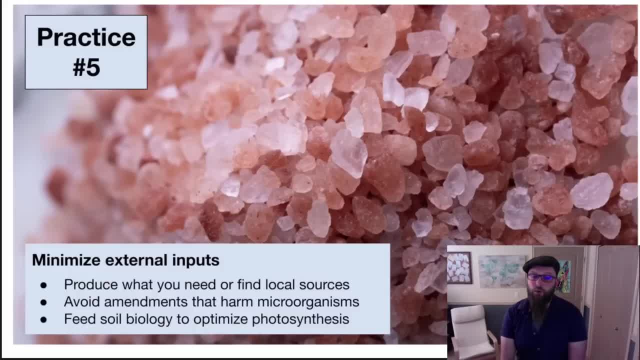 in a few months. right, What have you really done? So we're thinking of the soil biology as a way To also optimize photosynthesis in the plant. So the plant is not missing key nutrients and it's capturing a lot of sunlight, which 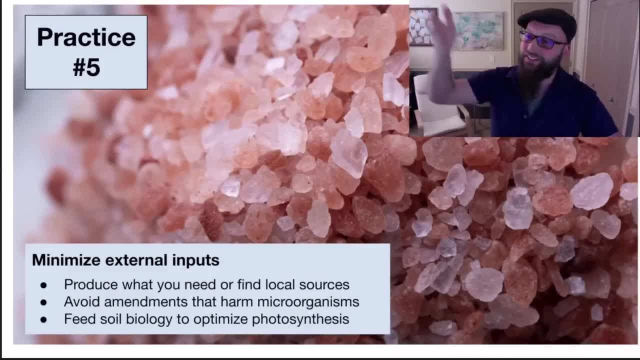 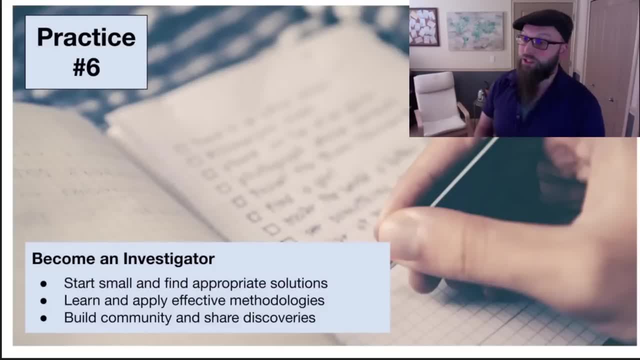 it turns into sugars which it feeds the microorganisms Again. it's the back and forth. So practice number six: become an investigator. We teach you these tools of microscopy because we are hoping to cultivate this curiosity in you where you say: I want to see what's happening. 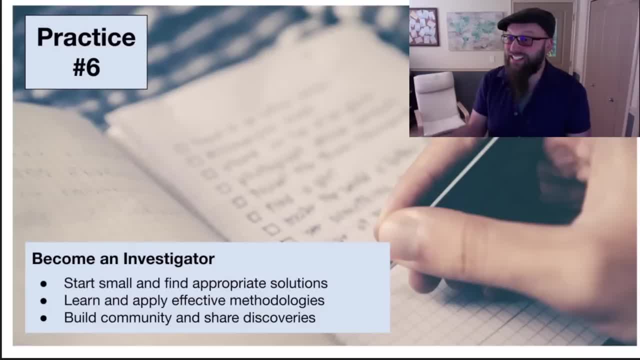 I want to see what's happening. It's a tiny world, It's hard to see, It's hard to even imagine sometimes, but it's so important- And then share what you know. We're trying to create a community here at the school where we can co-create together. 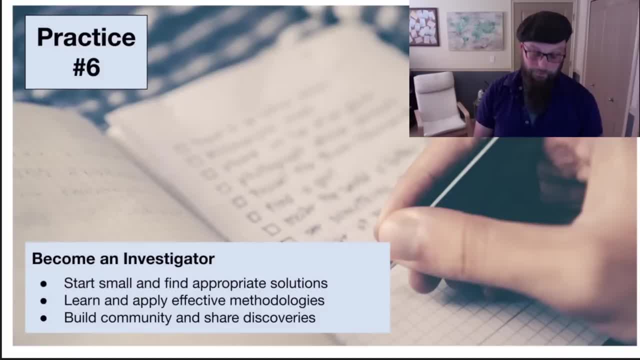 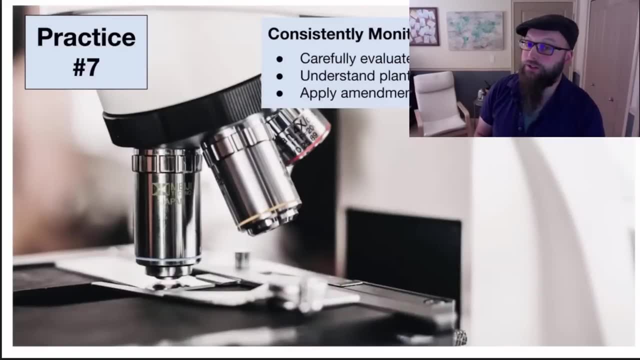 We can learn things together and share them. And finally, it's that monitoring of the biology where we would connect any of those practices that we're doing with their effect. on the soil food web, I like to say, you know, there's chemical and physical parts of soil. 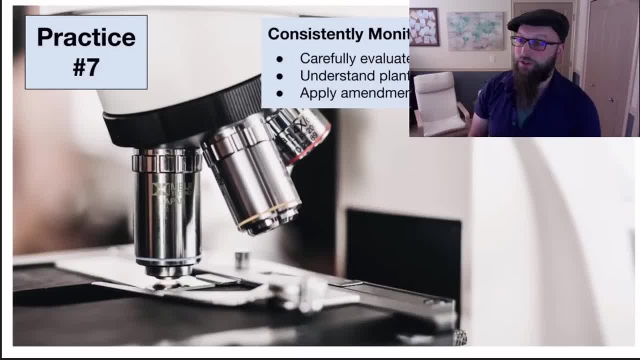 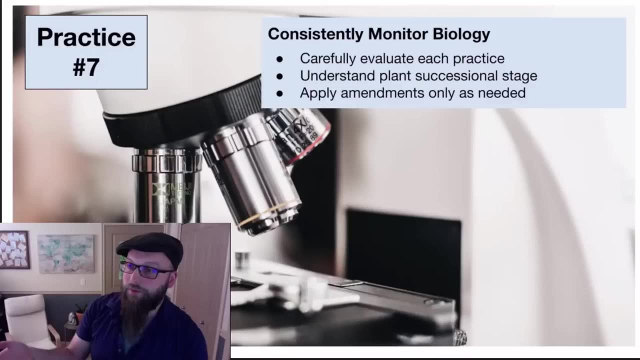 But the keystone that holds the arch together is the soil biology, And so if we don't get that right and see what's going on, you know, determine the influence on the, on the soil microorganisms, then we're really we're missing a step. 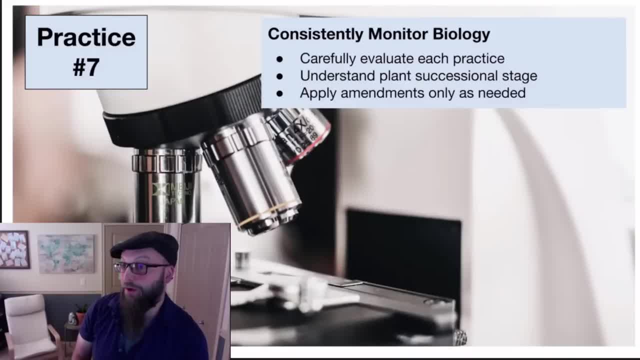 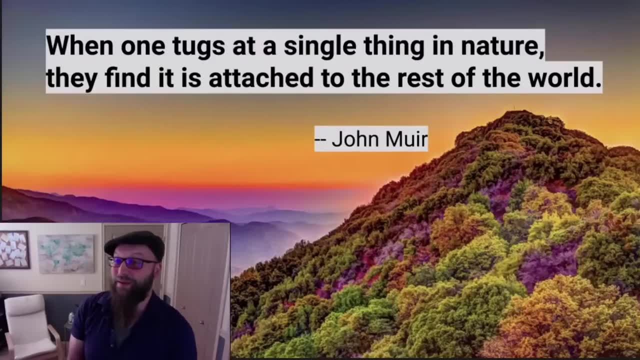 We can't answer, We can't come up with the right answer without without knowing how it affects the soil biology. So I'm going to end with this quote. coming back to fungi, It's one of my favorite from John Muir. It makes me think of fungi. 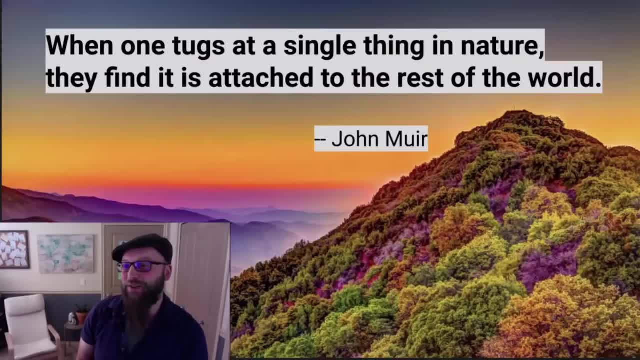 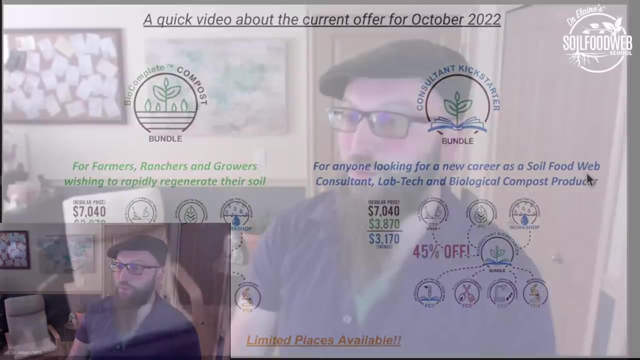 When one tugs at a single thing in nature, they find it attached to the rest of the world, And I think that the our fungal allies are tiny allies in the soil. They are one of the the strings that attach to everything. Okay, I think it's you, Brian. 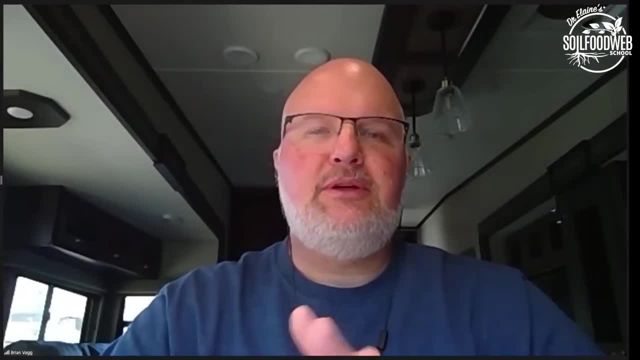 Hand it back to me. Yeah, Thank you, Adam. Thank you for your presentation. As always, you're very insightful in the way you present. This is just fantastic. I noticed a lot of comments in the chat. Kudos to you. 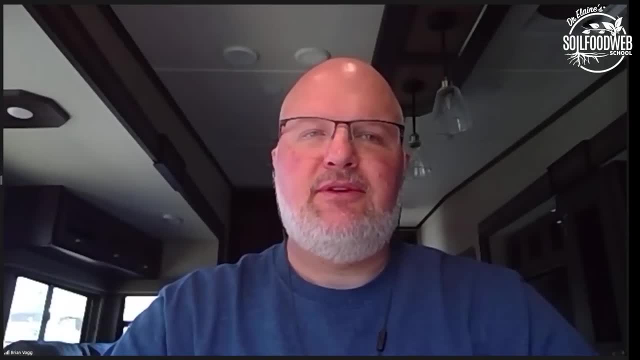 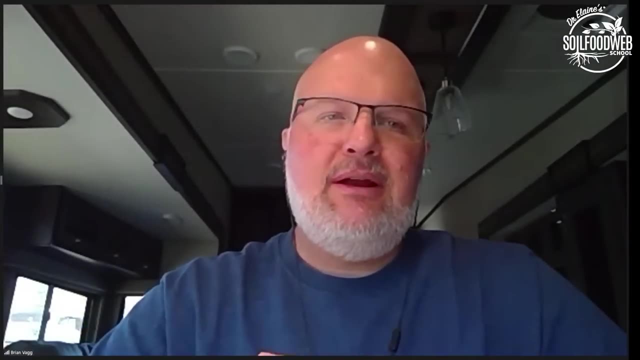 It's a complicated subject that I think you really were able to really distill down for folks. So thank you, Adam. Okay, so let's move on to our next part of the webinar And, before we get to Q&A, what we like to do is talk about our October promotion. 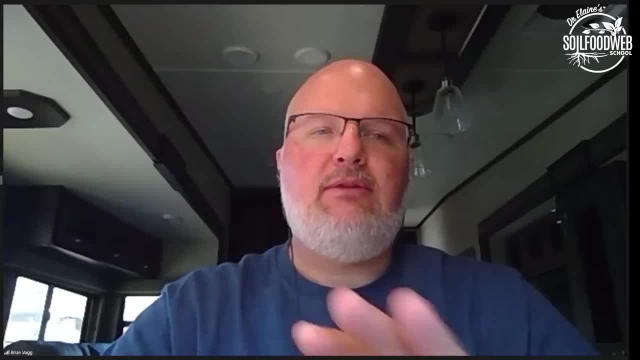 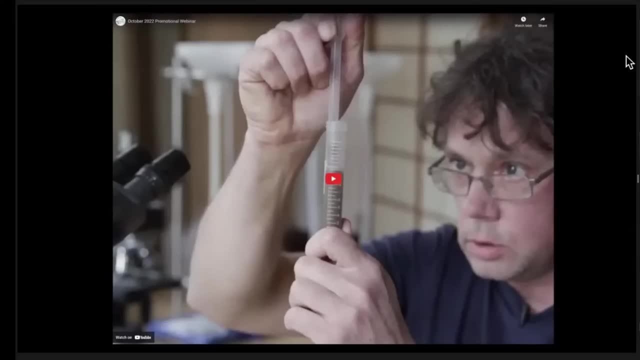 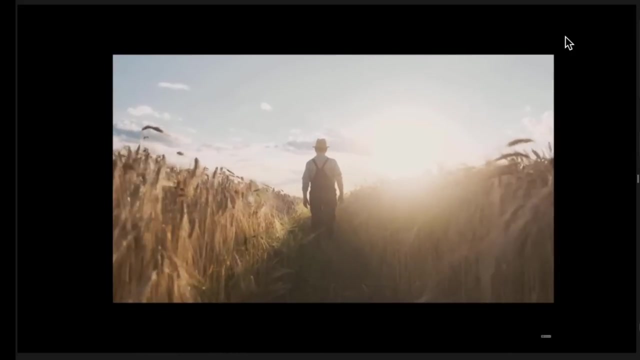 So we're going to watch a quick video that's going to talk about the two different bundles that we have going on In our October promotion. So, Adam, if you want to go ahead and start our video, If you're interested in joining the Soil Revolution, this is a great time. 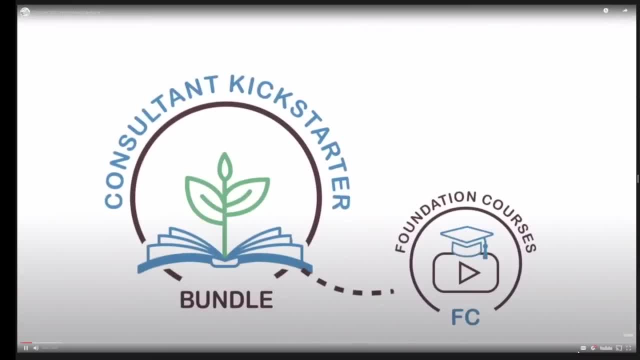 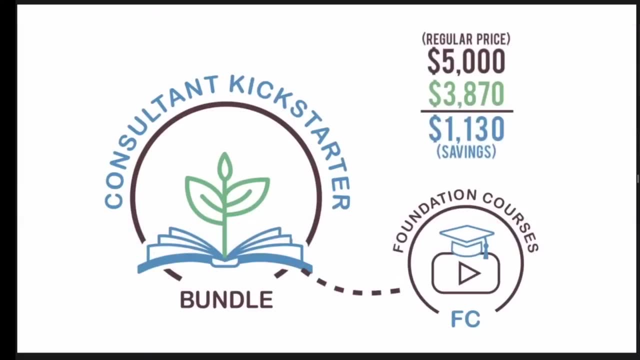 With a Consultant Kickstarter bundle, you can register for the Soil Food Web Foundation courses with Dr Elaine Ingham for just $38.70,, saving over $1,100 through October 20.. You'll also get stage one of the Consultant Training Program totally free. 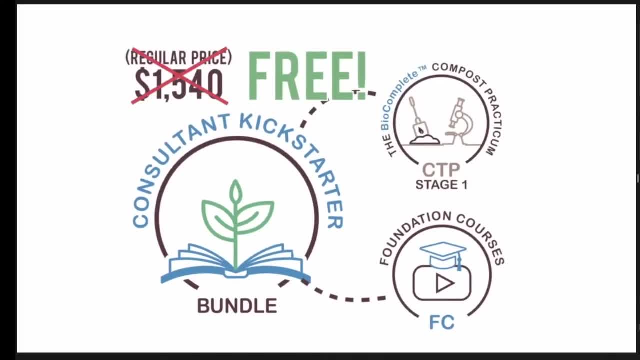 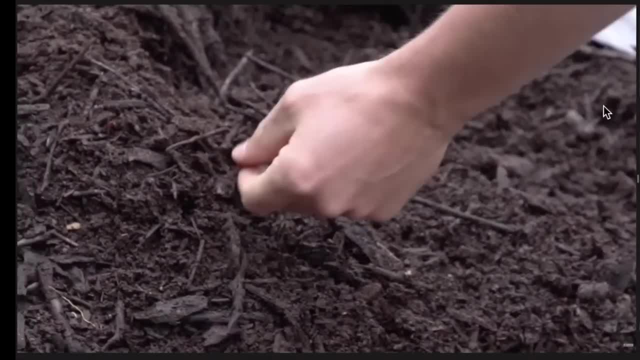 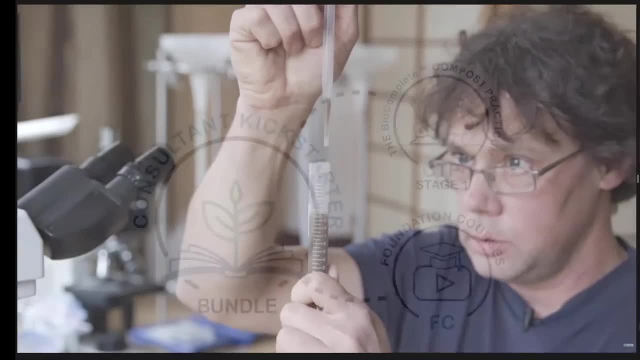 Thank you, Saving a further $1,540.. That's 26 hours of mentor time dedicated to helping you make your own biological compost and develop your microscopy skills to the standard required to qualify as a certified Soil Food Web Lab Technician. You'll also get two free bonuses with this offer. 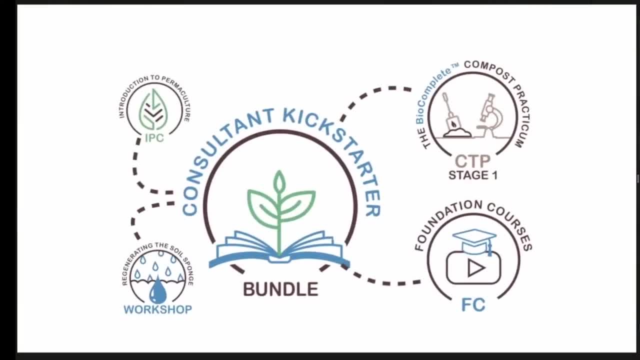 The Introduction to Permaculture course with Graham Bell and the Soil Sponge Regeneration Workshop with DeeDee Pursehouse, saving a further $500.. The total value of this bundle is over $1,500.. This bundle is also free for the first time. With the Consultant Kickstarter bundle, you'll save $1,400 through October 20.. The total value of this bundle is over $7,000.. For which you'll pay just $38.70, saving over $3,100.. That's 45% off. 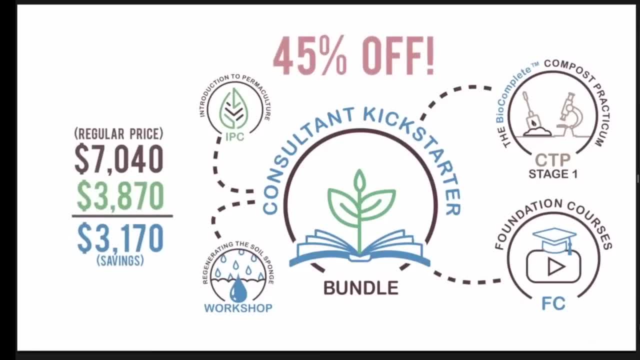 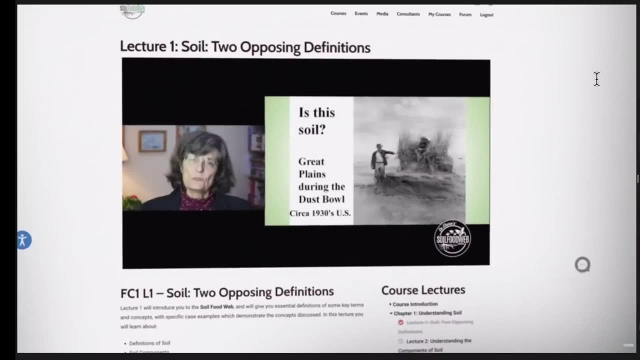 There are limited places available with the Consultant Kickstarter bundle, so please don't delay. In Foundation Course 1, you'll take a deep dive into the science and methodology that underpins the Soil Food Web approach, which was developed by Dr Elaine Ingham over the 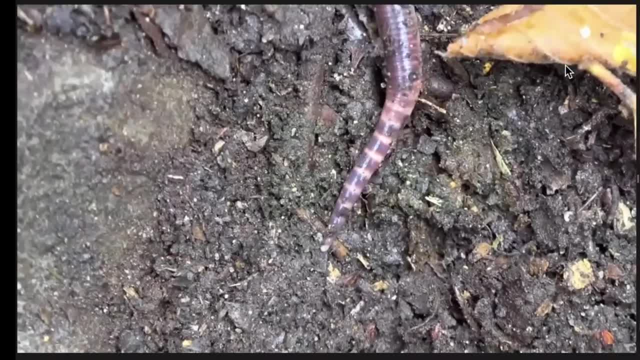 last four decades. This is the first time Dr Ingham has used the Soil Food Web to develop the Soil Food Web. This is the first time Dr Ingham has used the Soil Food Web to develop the Soil Food Web. how the agricultural practices we've been using in the last hundred years have degraded our soils. 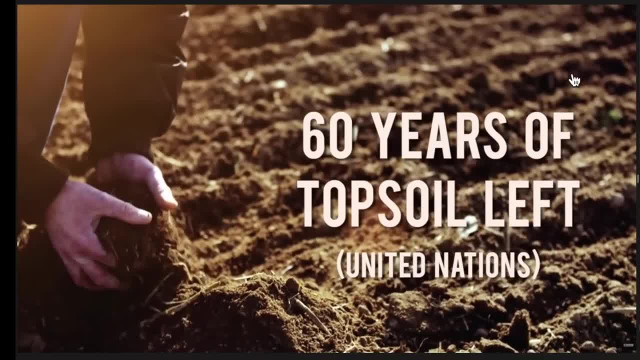 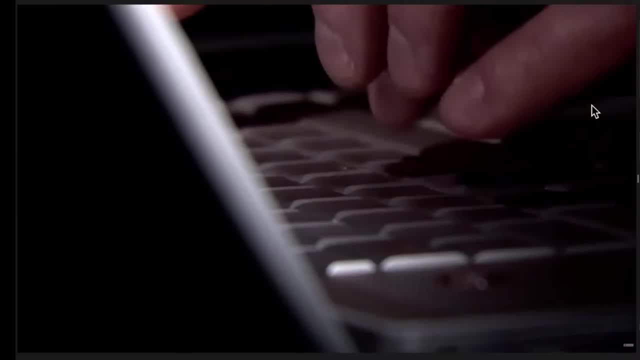 to the point where we now only have around 60 harvests left, according to the United Nations. You'll learn about the solution to many of the problems that are familiar to farmers all over the world today, Problems like diminishing soil fertility, pest and disease pressure. 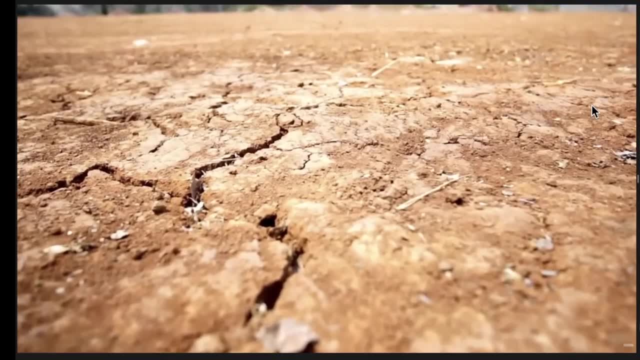 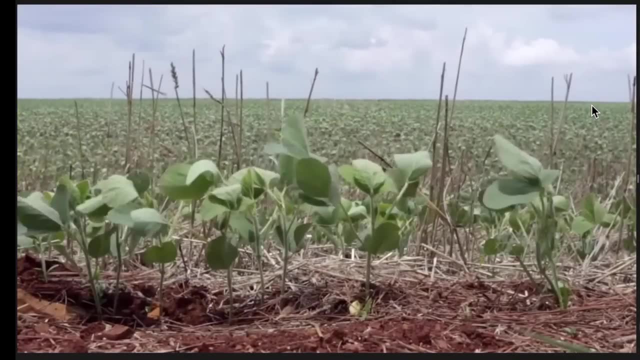 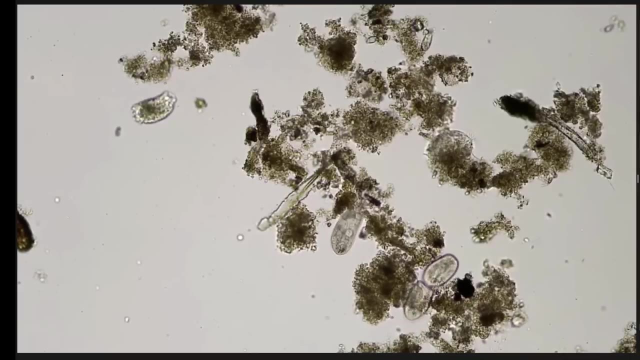 low crop yields, drought, flooding, compaction and soil erosion. Regenerative agriculture can address all of these problems. You'll be introduced to regenerative practices like no-till and the use of cover plants. You'll also learn about the four major groups of microorganisms that drive soil. 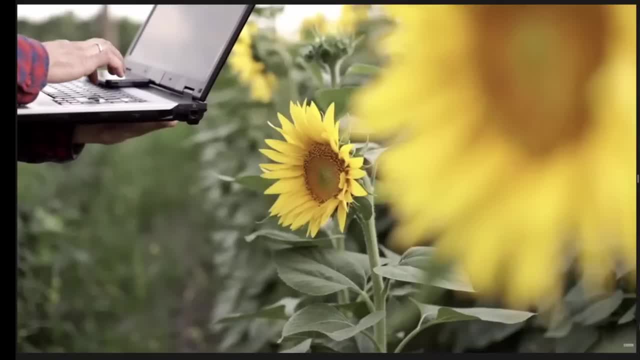 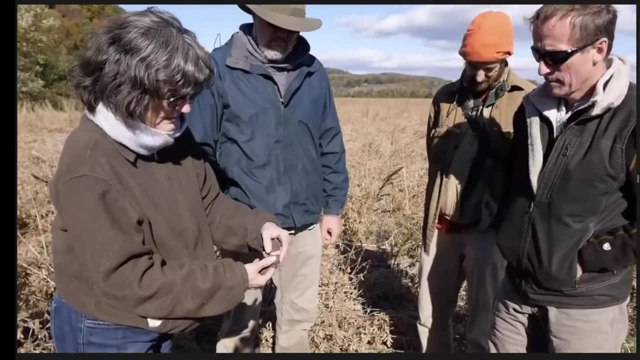 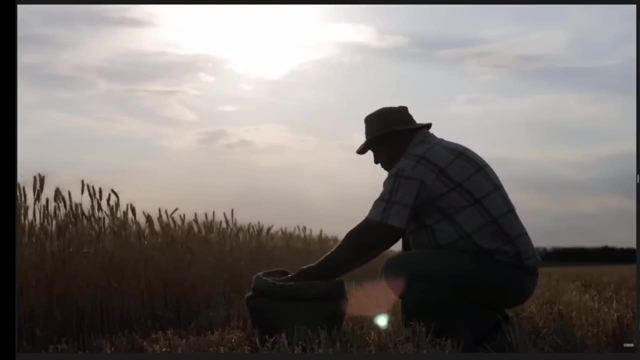 regeneration and how the process can be accelerated by restoring the microbial community, or soil food web, to your client soils. Dr Elaine will present a number of case studies from around the world that she has worked on personally. Here you'll see some of the amazing results that have been 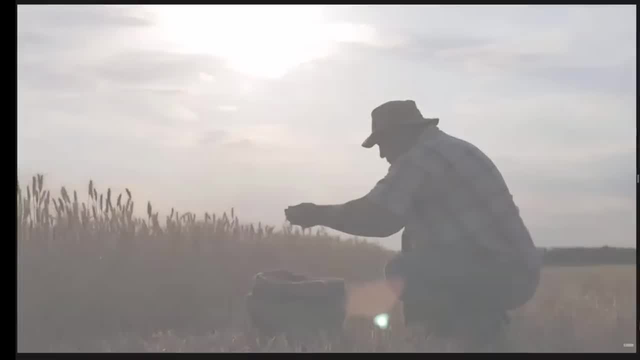 achieved using this research. Dr Elaine will present a number of case studies from around the world that she has worked on personally. Here you'll see some of the amazing results that have been achieved using this soil food web approach. In Foundation Course 2, you will learn all about the importance of 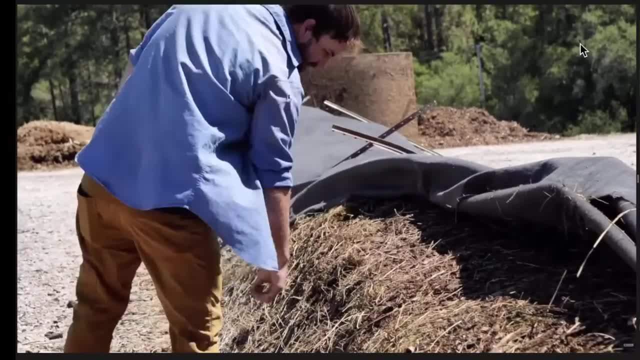 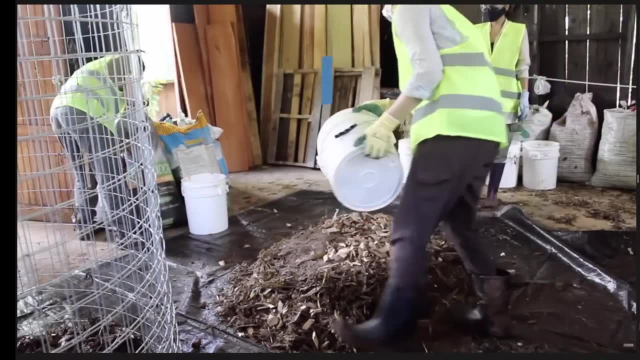 biological compost and how it's very different to regular compost. When most people look at compost, they only see a means of delivering nutrients to their plants, so they think about how much nitrogen, potassium, phosphorus and other elements are in the compost. 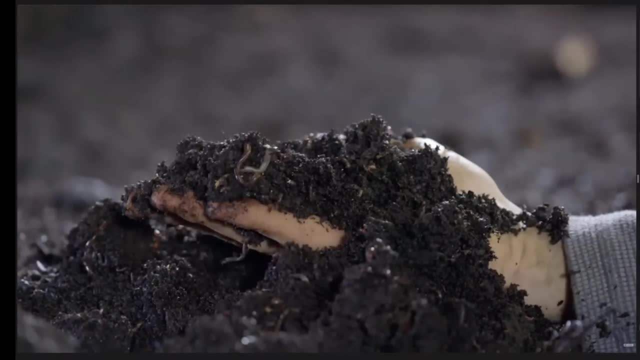 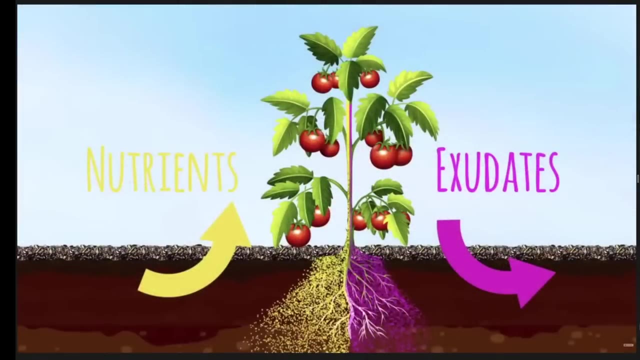 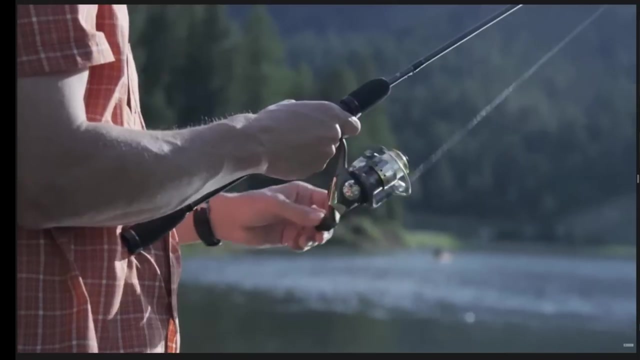 When we look at biological compost, we see a means of inoculating the soil with beneficial microorganisms so that the soil ecosystem can start to function again, Providing plants with a continual supply of nutrients. This is kind of like teaching someone to fish so they can feed themselves for life, as opposed to just giving them a single meal. 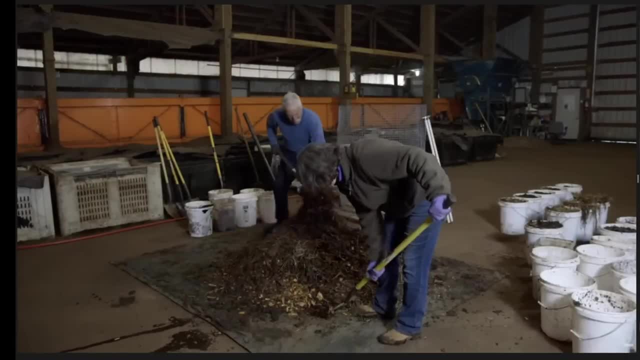 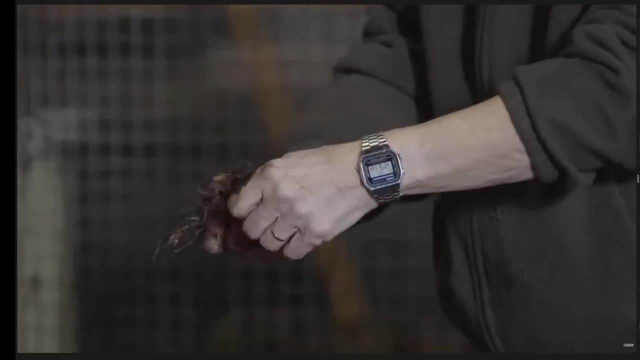 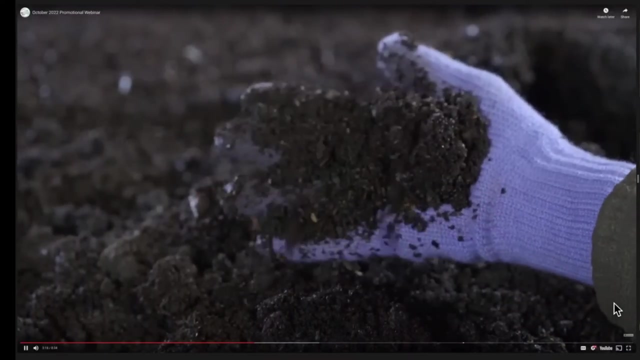 In this part of the training, you will learn how to make biological compost using various starting materials to create a recipe that will produce results. You'll learn how to monitor and control moisture levels, aeration and temperature in order to ensure that beneficial microorganisms are multiplied while disease-causing organisms are destroyed or. 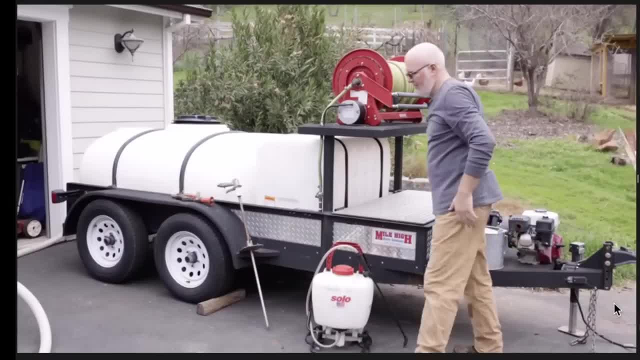 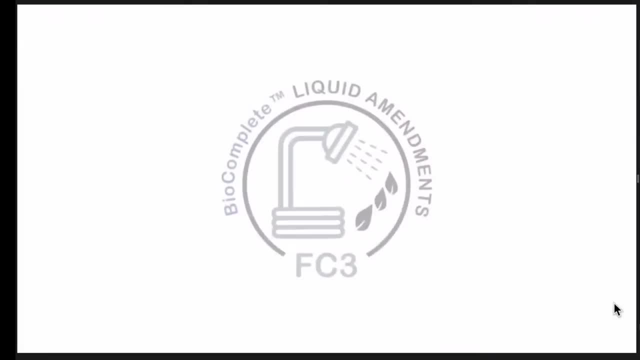 become dormant. You'll also learn about the various types of equipment that can be used at different scales, And you'll learn about the different ways in which biological compost can be applied to the soil. In Foundation Course 3, you'll study Dr Elaine's methods for making. 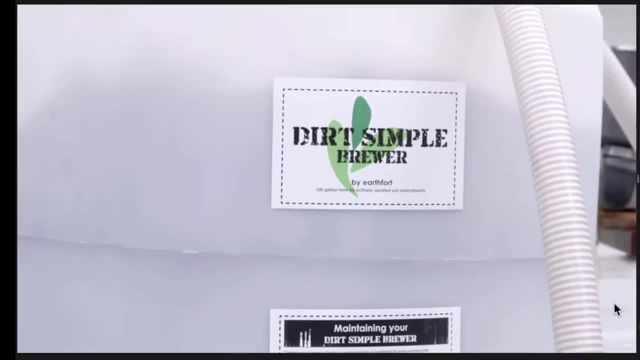 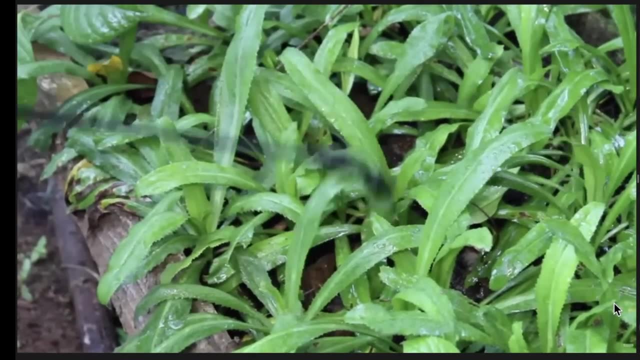 liquid biological soil- amendments. Compost extracts are used as a soil drench, delivering microbes deep into the soil profile, where they can interact with the plant's root system. Compost teas are applied to the plant's foliage where they form a protective barrier against the 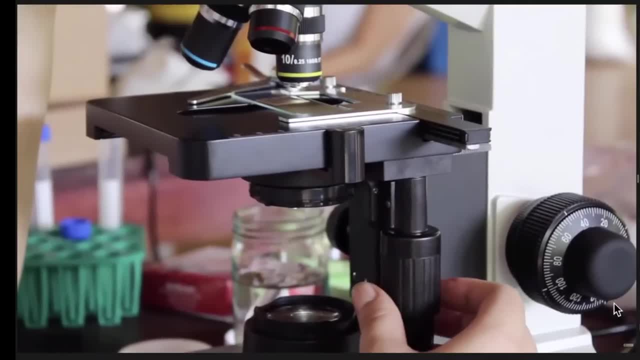 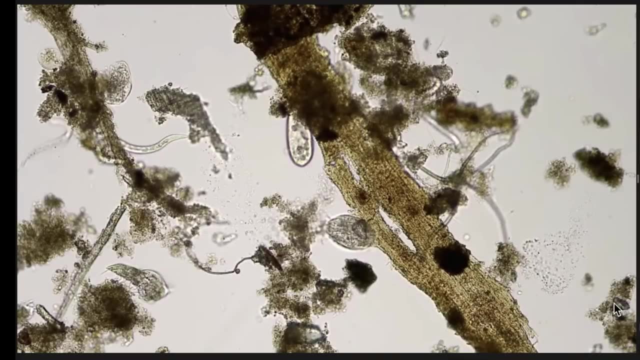 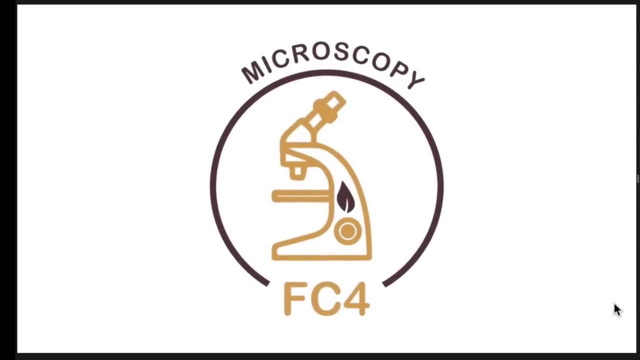 foliar diseases. In time, as your soil biome becomes more diverse and vigorous, your plants and trees may be entirely covered with beneficial microbes without having to continually apply them. In Foundation Course 4, you'll focus on four major groups of microorganisms in the soil food web. 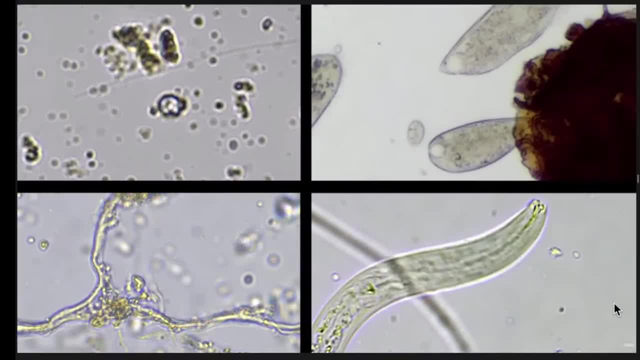 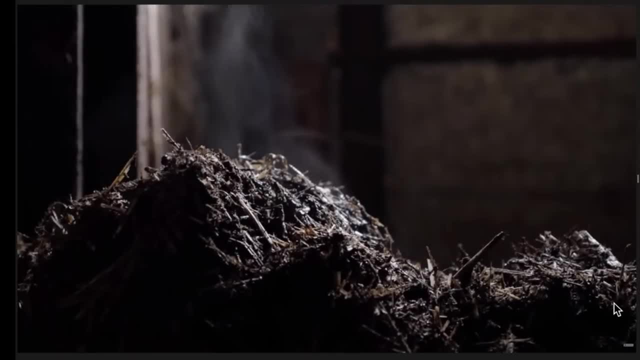 bacteria, fungi, protozoa and nematodes. You'll learn how to use a compound microscope to identify and quantify these microbes so that you can really see what's going on in your compost and in the soil. This can be done with a microscope or a microscope, and the other way around. You'll also 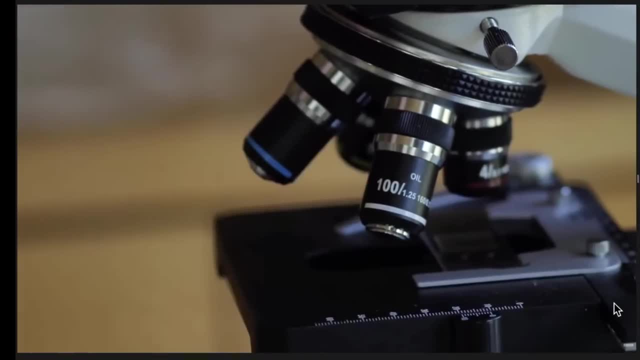 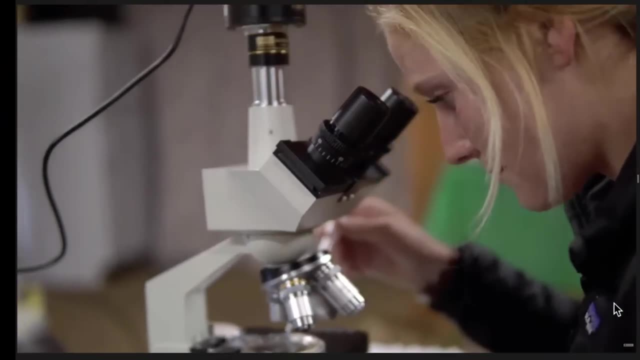 This will give you the ability to assess the quality of your compost and liquid amendments before you invest all the time and effort that is required to apply them to the soil. You will also be able to monitor the progress of the microbial community in your soil over 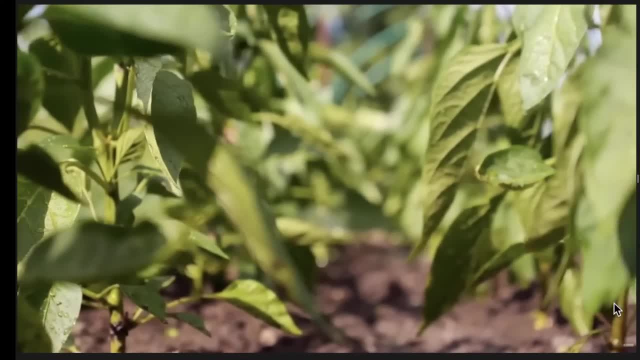 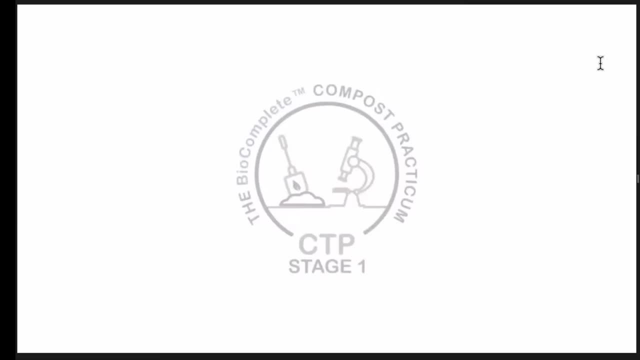 time, so if something is going wrong, you will know about it before the plants start to suffer. This gives you the opportunity to take remedial action early on in the growing season. In stage one of the consultant training program, you'll be assigned to one of our highly 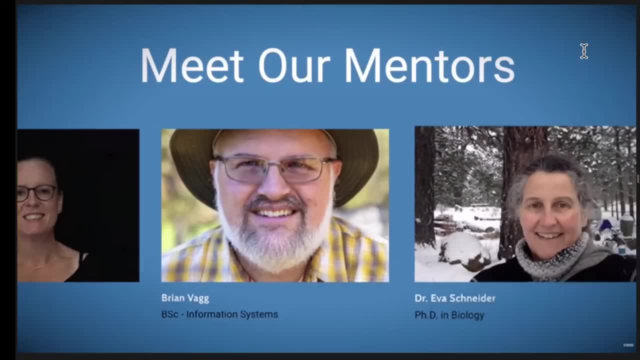 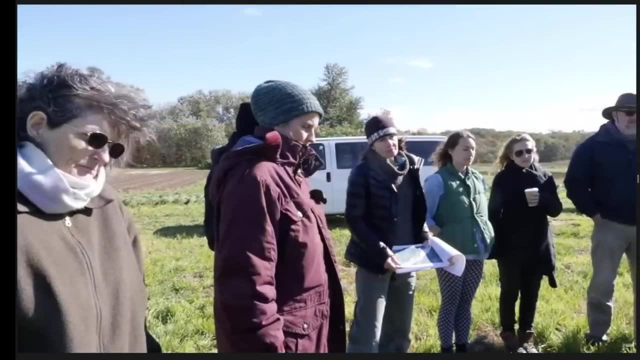 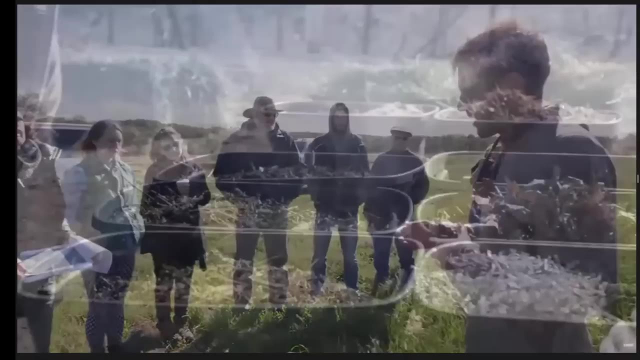 skilled mentors, some of whom are soil food web consultants who run their own businesses supporting farmers to make the transition to the soil food web approach, and others are PhD biologists who have been working closely with Dr Ingham for several years. You'll work one-on-one with your mentor to develop your compost making and microscopy. 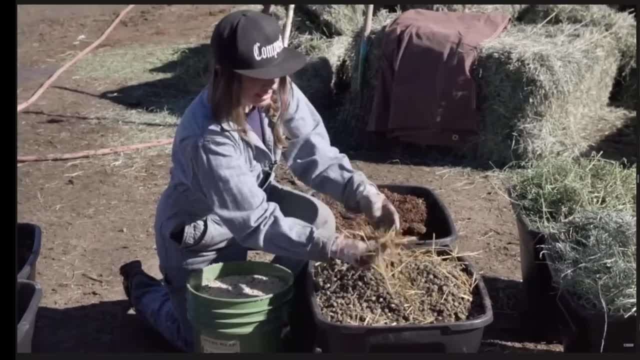 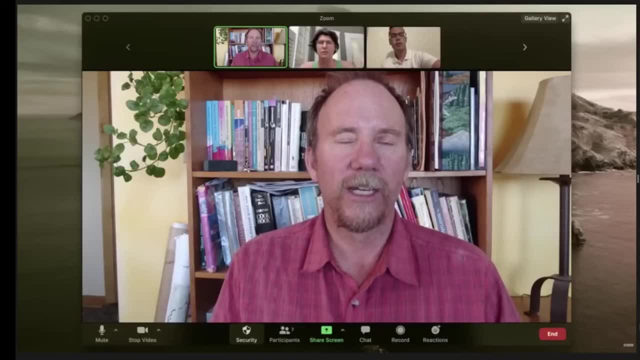 skills. When it comes to making great biological compost, there are many variables and every situation is different. Our mentors have worked with dozens of students making compost in many different conditions, so they'll be able to help you address some of these challenges that are unique to your location. 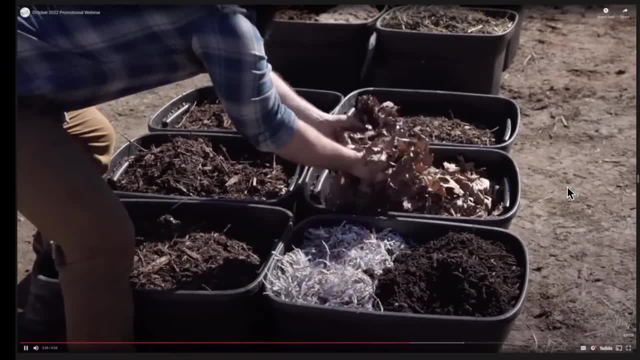 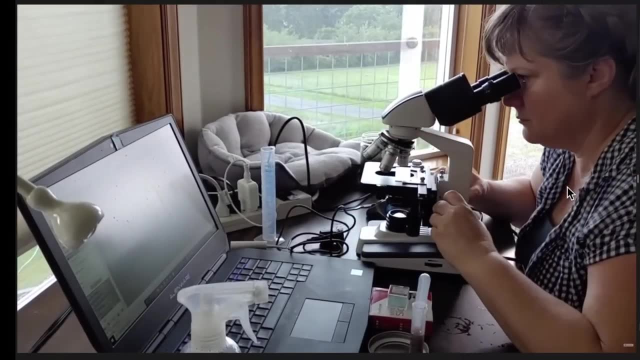 They'll also guide you to avoid making common mistakes that can cost you lots of time, money and effort. Your mentor will support you as you develop your skills to the required standard to pass the microscopy proficiency assessment. Achieving this standard will give you the confidence to really know what's happening. 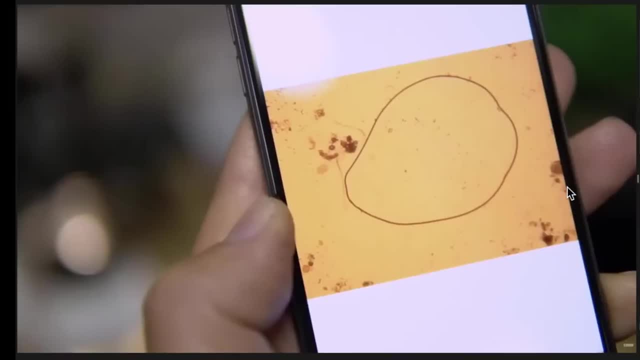 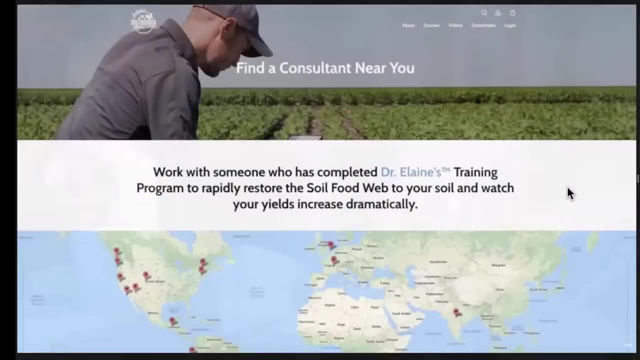 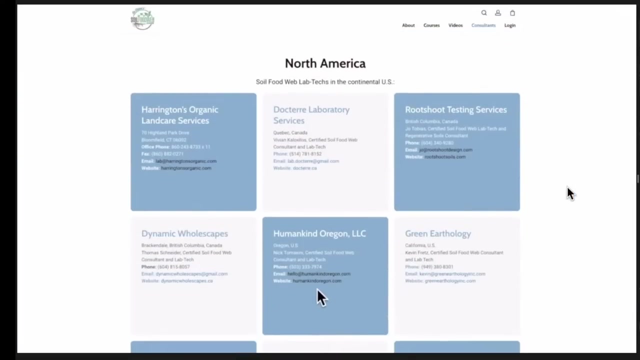 in the microbial community in your compost and soil. You'll be able to identify and quantify the four major groups of microbes in the soil in about an hour or less. Once you successfully pass the microscopy proficiency assessment, you can elect to be listed on our website as a certified soil food web lab tech, which means that you can. 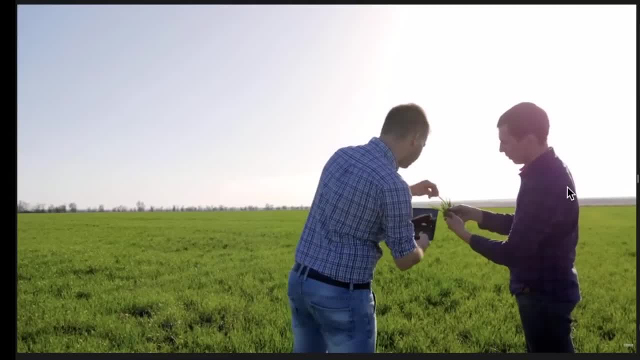 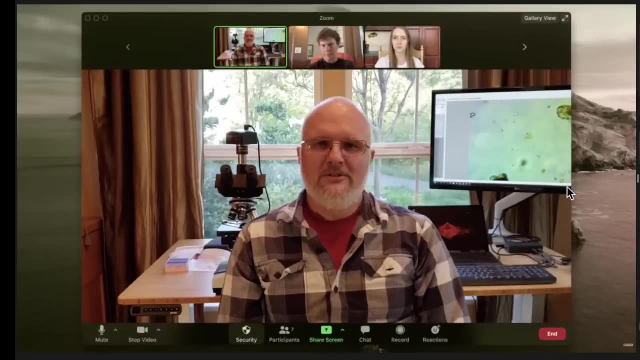 assess soil samples for other farmers and growers in your region. You'll have a total of 26 hours of mentor time so you can arrange Zoom calls and exchange emails with your mentor whenever you feel you need help. Well, that was abrupt. That was abrupt. 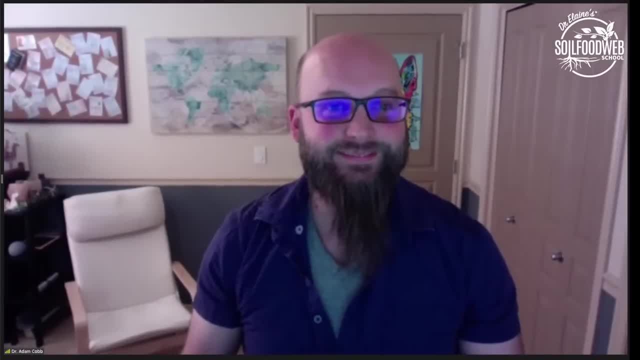 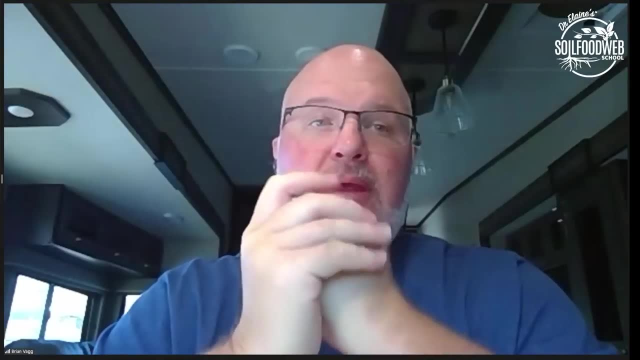 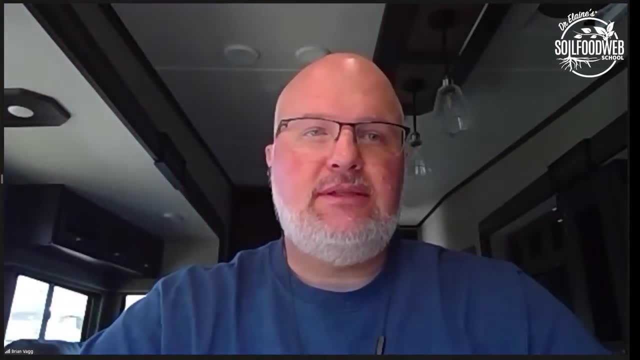 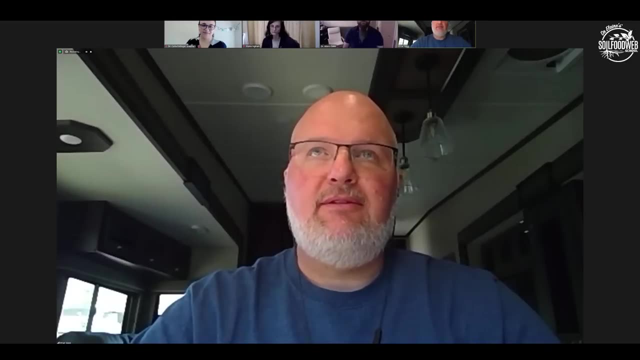 I know we have limited spaces available, but I highly suggest, if you're interested, go ahead and sign up. The amount of information that's provided in these classes is tremendous. I was very appreciative that I was able to get that education for myself, and it definitely 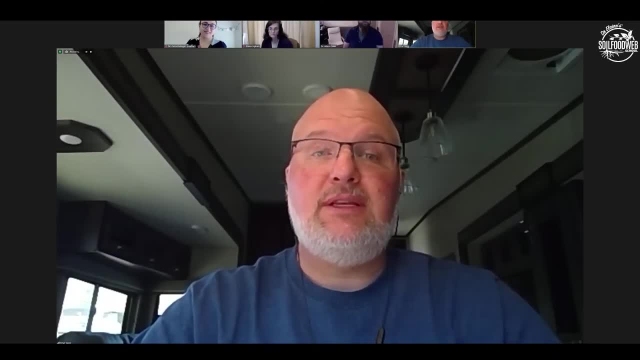 allowed me to be able to do the things that I do, that I do today. so, Okay, with that being said, let's move on to our Q&A section And, Adam, I think you're going to share that out, right? 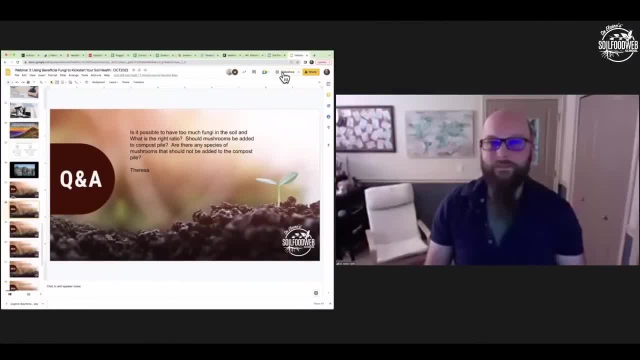 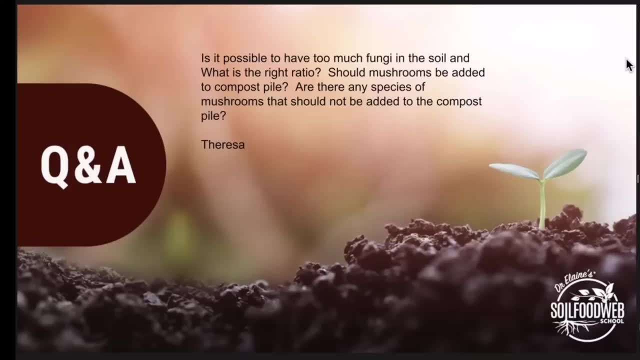 Yep, Perfect, Okay. so for the rest of the webinar we're going to be going through Q&A And I guess again are the questions that you guys posted in our Q&A section, And the first question is from Teresa. 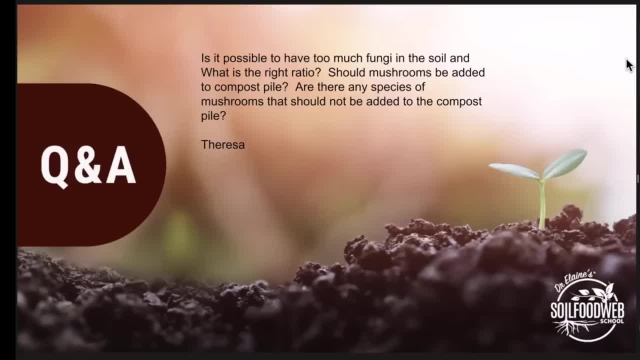 And the question is: is it possible to have too much fungi in the soil, And what is the right ratio Should mushrooms be added to a compost pile? Are there any species of mushrooms that should not be added to the compost pile? So multiple questions in this one. 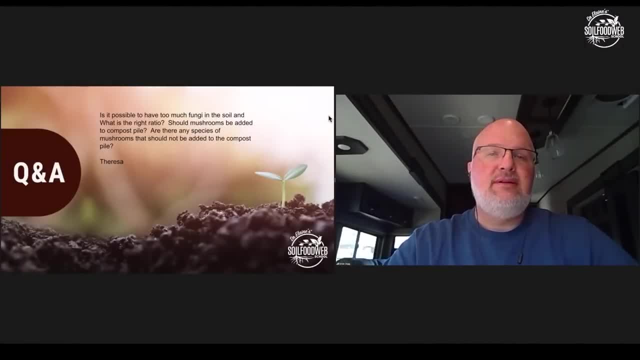 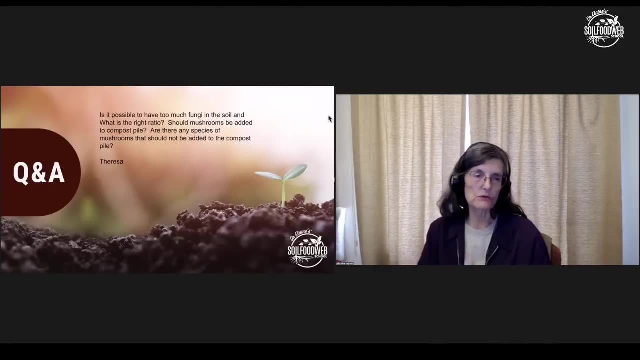 But we're dealing with fungi. So, panelists, what say you With the fungi and how much fungi you want in the soil? it needs to be linked to the plants, to the crops that you're trying to grow. So we know what's the proper ratios for most plants. 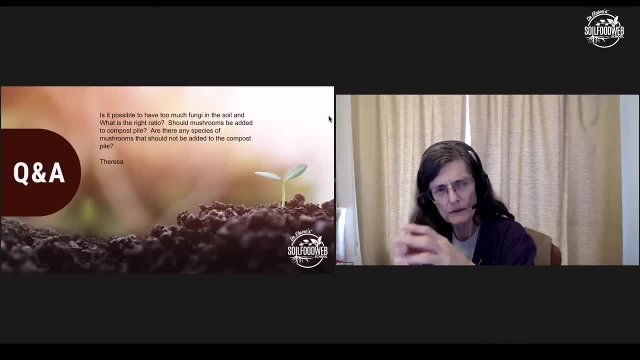 You know, sometimes you have to just think: well, the plant I want to know about isn't on their list, But you know it's an awful lot like a lilac or it's just like a tomato planter. So you would be able to figure out what that fungal to bacterial ratio needs to be and get that fungal to bacterial biomass correct. 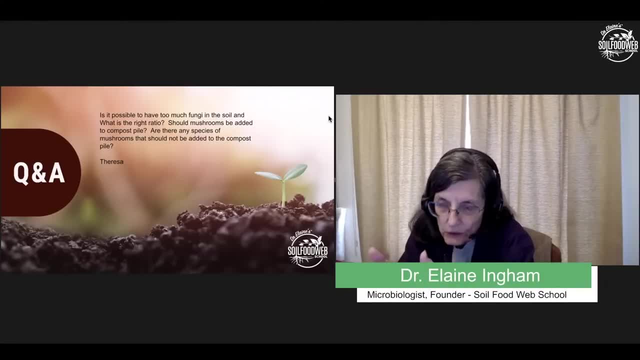 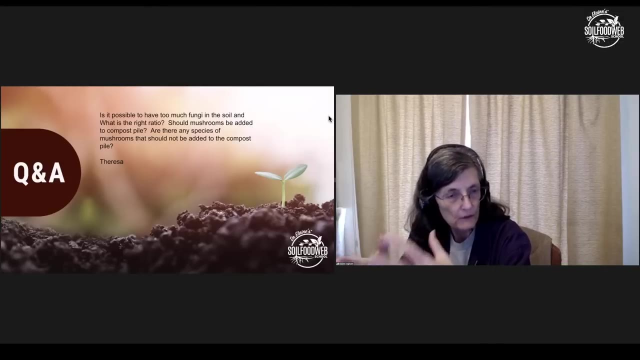 That's what we're really looking for. So if you're trying to grow kale and you've got the fungi of an orchid, An old growth forest, in that soil, things are not going to work out well. You want to make certain that. you might even have to. if you started with an old growth forest, you would probably want to disturb it a little bit to bring it back to the right balance of the fungi and the bacteria, protozoa and the nematodes. 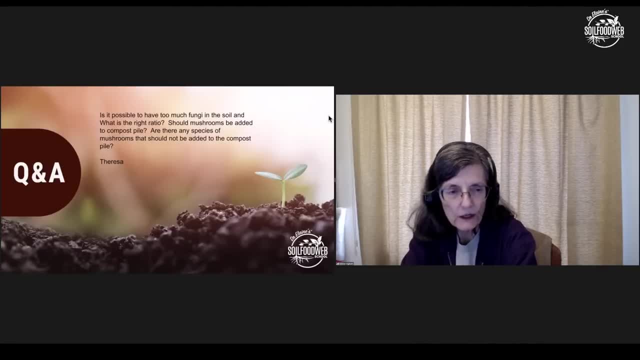 So what is the right ratio? It depends on what you want to grow, And here is where it's probably going to be best If you have a mentor. So you know, sign up, do the FC courses And then, when you move on to the higher level courses, you get a mentor. And lots of good discussions between you and your mentor. So should mushrooms be added to a compost pile? Well again, standard, ecological answer. it depends What are you trying to achieve. So are there any species of mushrooms that would not be added to the compost? Yes, the poisonous ones are probably not what you want in your compost pile. So you do have to learn a little bit about what the different kinds of above ground mushrooms are appearing, And I'm sure Adam can add a few more sentences about that. 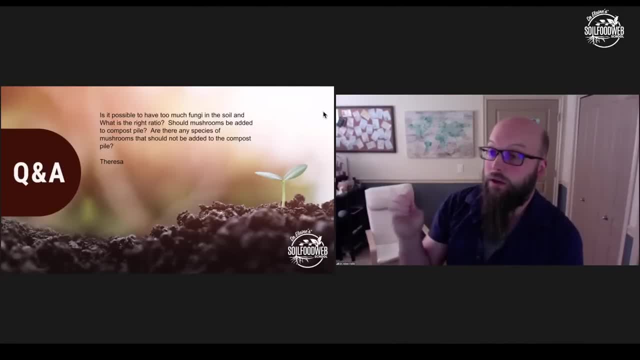 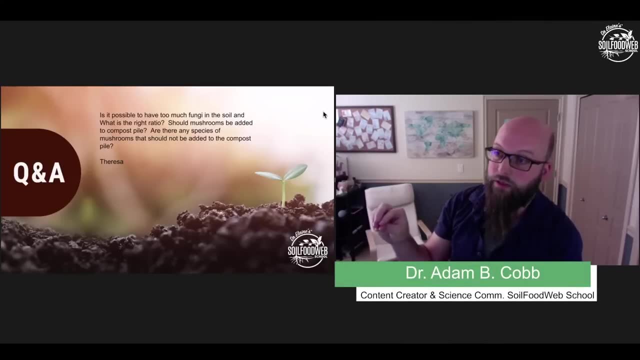 Well, I just want to point out that sometimes we tell people that they can go get a little bit of leaf, litter or other material from a really thriving ecosystem in their area That's already going to be full of fungal, hyphae or other things. 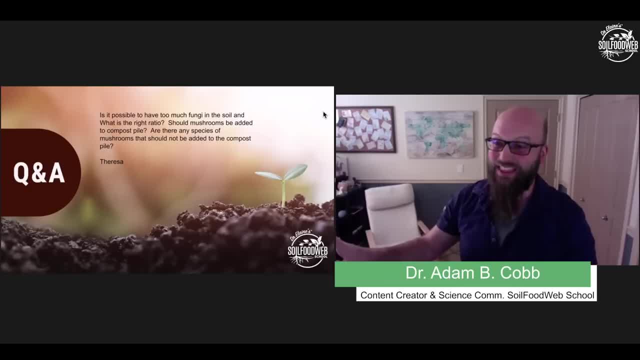 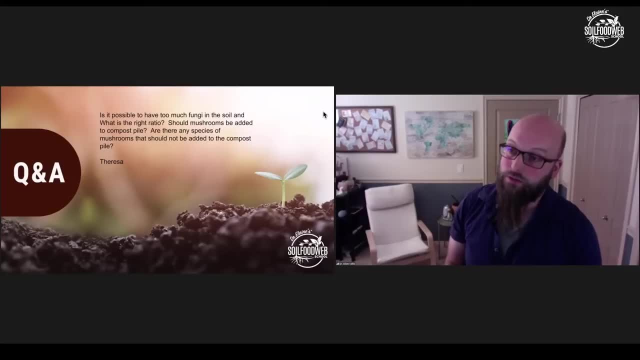 We just don't want you to go out and disturb massive areas with that right. So if you were growing a grain crop, I might say: well, is there a diverse grassland that you could go to and take a little soil and some of the you know plant material, maybe as well, to get those organisms in your pile prior to the composting process? 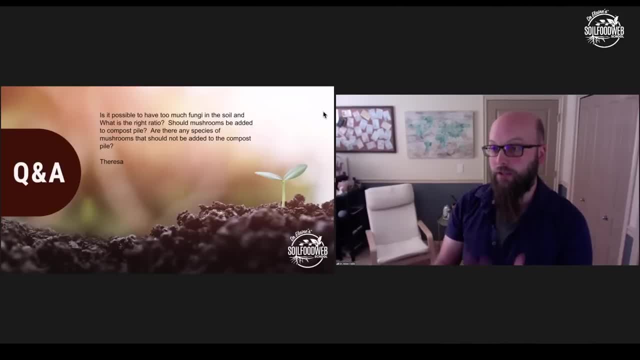 So that any pathogens that are in there will have the chance to be killed by the heat. But you know that can be a great way to get more diverse fungi into your compost pile. I've also made compost where I didn't do much of that kind of stuff and I found a lot of diverse fungi in there. 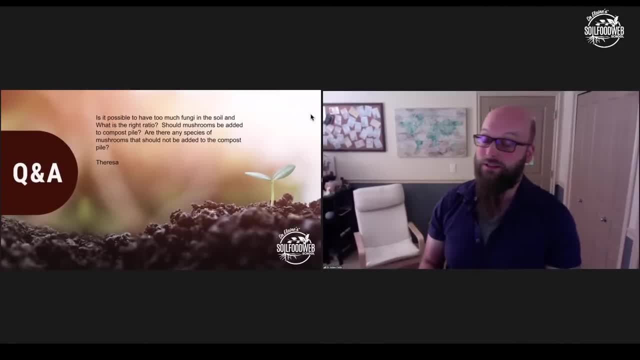 So they're coming in the air and other things. And yeah, I do know some people that like to go foraging. They know enough about the diversity, They know enough about the different mushrooms that they will gather some of the caps of non-poisonous mushrooms and add them to their compost pile. 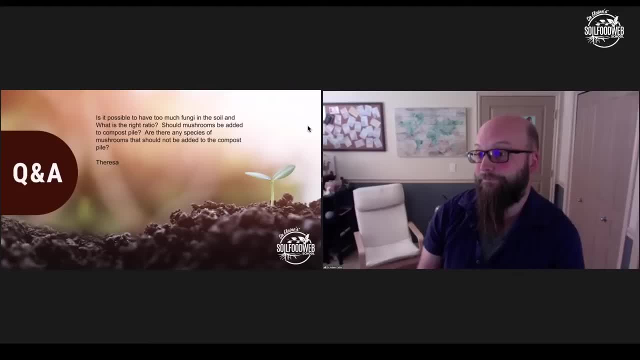 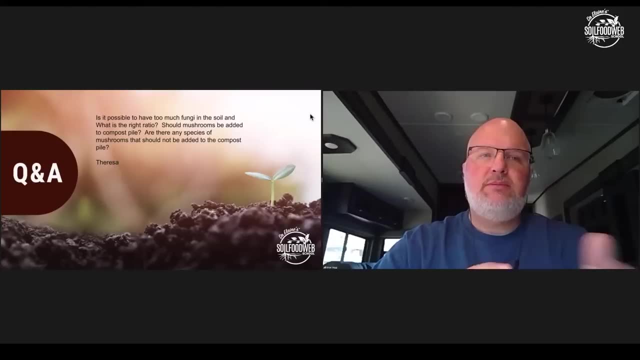 And that seems reasonable to me as well. You know, one thing that I get quite a bit too is people will ask me: hey, you know, I have access to mushroom spawn, you know, from a commercial mushroom operation. You know, should I add it to my compost pile? Well, I mean you can, but you also have to recognize that you're going to be adding just a single species of fungi. Yeah, When you take that mushroom, Mushroom spawn, those mushroom blocks, So don't rely upon it as being, oh wow, I'm really going to make this fantastic compost just because I added this mushroom spawn. No, it's fine to add it, But, as Adam and Elaine were talking about, go out and find those indigenous fungi in your area and add pinches of those into your compost. That's a much, much better way to get the diversity that you're looking for. 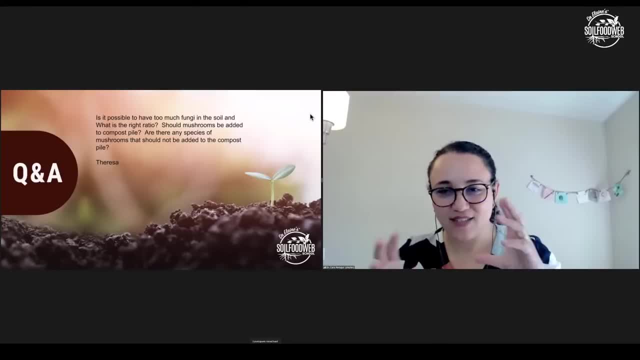 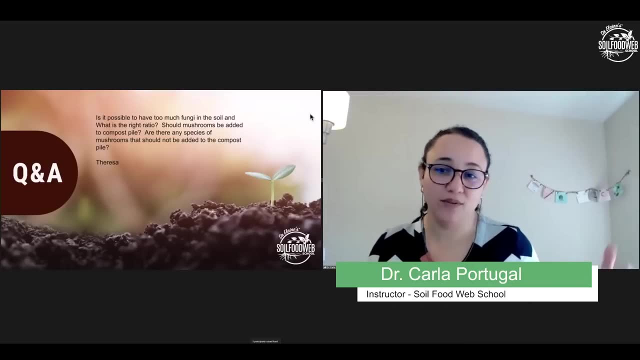 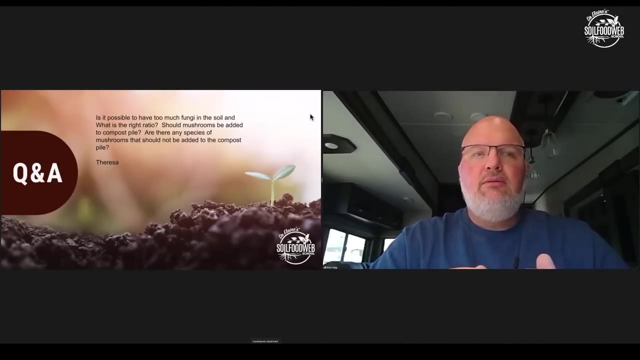 Yeah, Plus, ecologically speaking, you will avoid any exogenous species that can just like bring more damage. It doesn't benefit. So keep it local, Keep it simple. You know. one of the things I would like to mention too is Elaine was talking about. you know, you may not really be able to find for a particular plant. you know where does it fit in its F to B ratio? 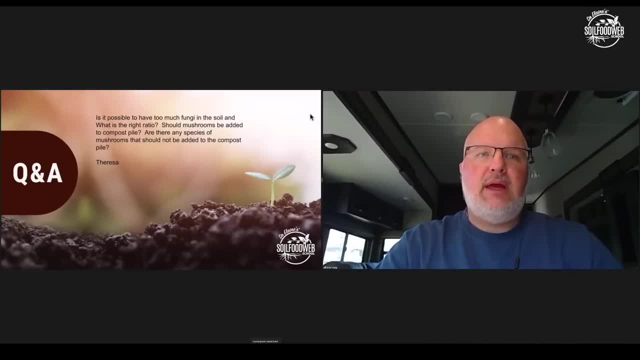 But all you need to really know is where it is its natural habitat, What is its ecological role, And that will give you a very good hint as far as what kind of F to B ratio are you kind of really looking for? And so those observational techniques, 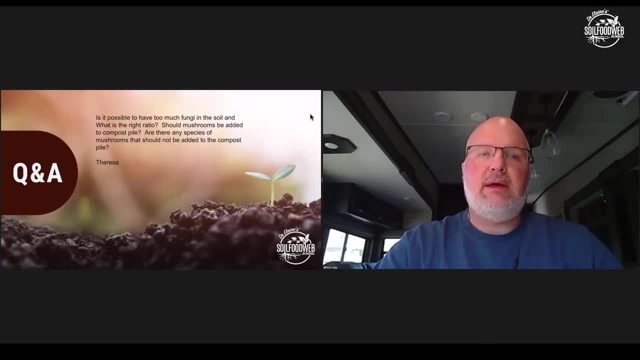 And just doing a little bit of research in that sense should kind of set you in the right path. Great points, Alice. anything else you guys want to add? Okay, Let's move on to the next question. Okay, So this question is from Megan. 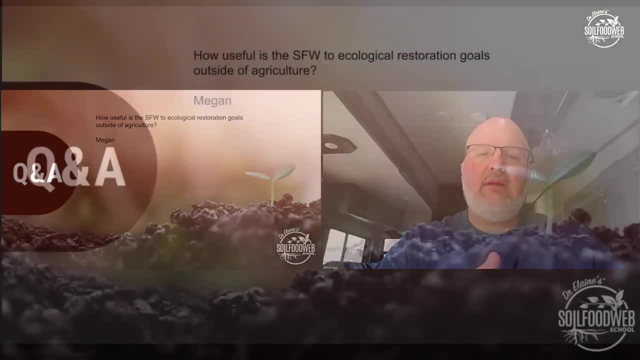 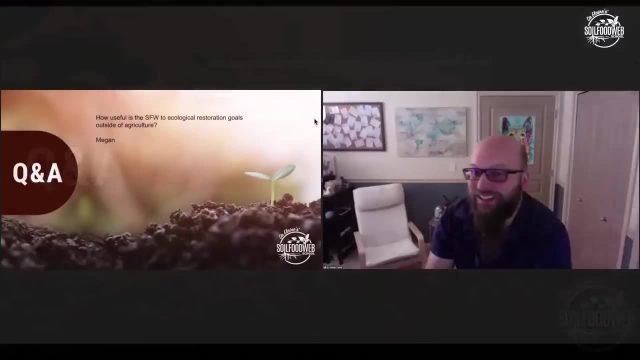 And the question is: how useful is the SFW to ecological restoration goals outside of agriculture? Alice, what say you? I'd love to take a whack at this one. Sure, Because I'm Super excited, as somebody who you know had formally taught ecological restoration at the college level, that we have this new relationship as an organization with the ecosystem restoration camp movement. 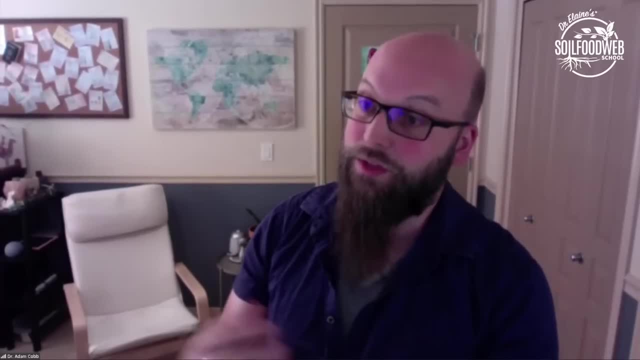 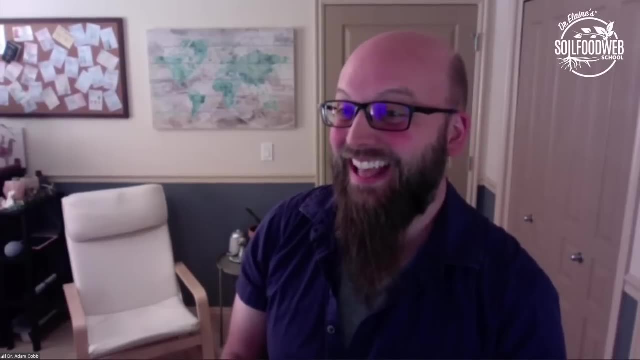 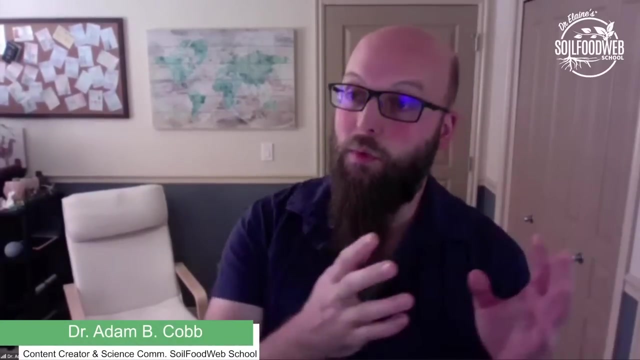 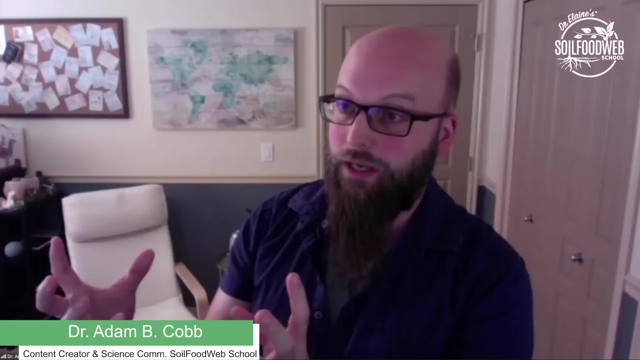 And I've been able to look at some of the materials that they're developing as courses on our website, And so the answer is there's a lot. There's a lot of crossover, Because in many ways, We are advocating for a style of agriculture which is more similar to the natural state of soils, right, 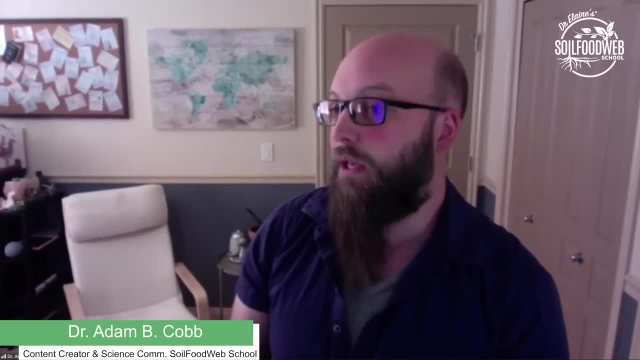 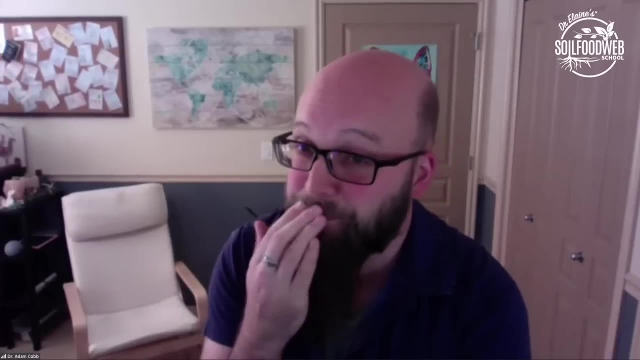 And so some of the tools that you might use could be different. with ecological restoration- And really when I hear that term, my ears tuned to you- have a specific target in mind, that you're trying to go to some kind of reference condition or site. 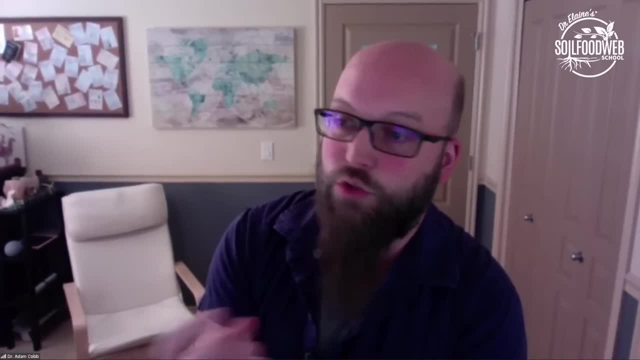 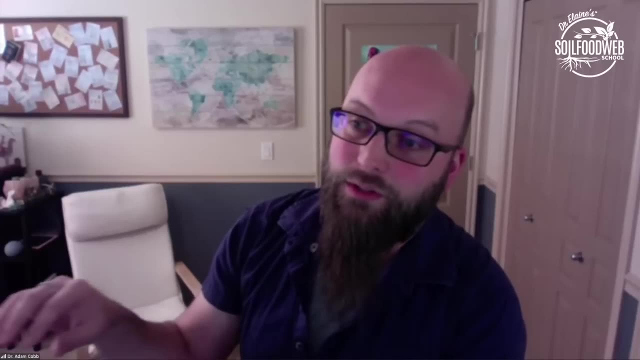 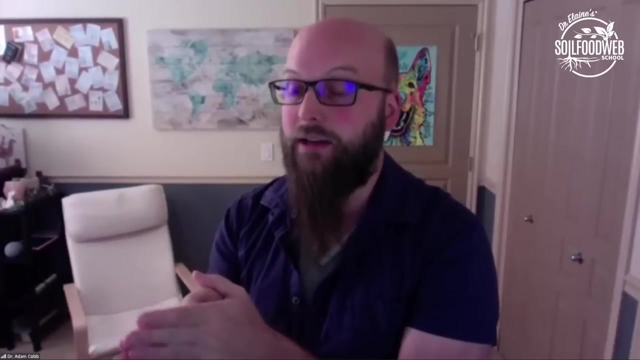 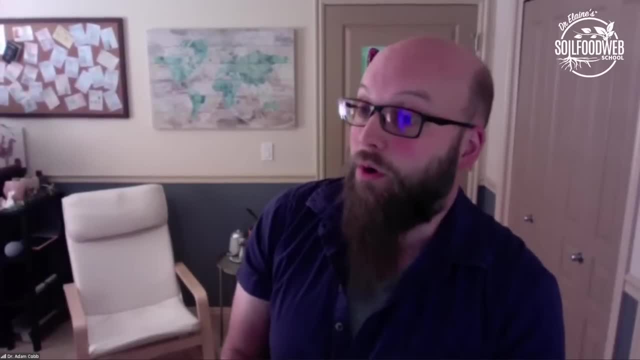 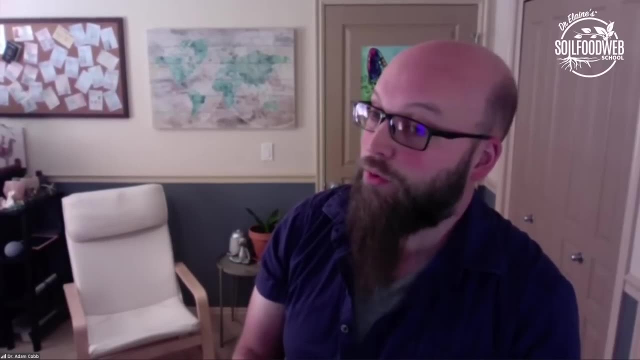 That's going to be. the main difference is what your overall goals are, But the soil ecosystem is going to be very similar between what we're advocating for in an agricultural setting and what you would want with a grassland, And so it's going to be very similar. 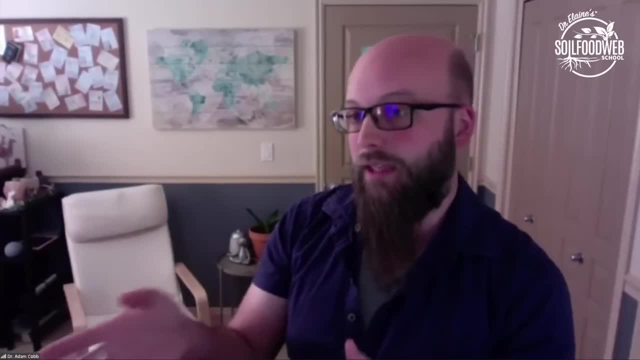 But the soil ecosystem is going to be very similar between what we're advocating for in an agricultural setting and what you're wanting with a grassland Or a forest. It's just going to be about fine-tuning things like that F to B ratio. 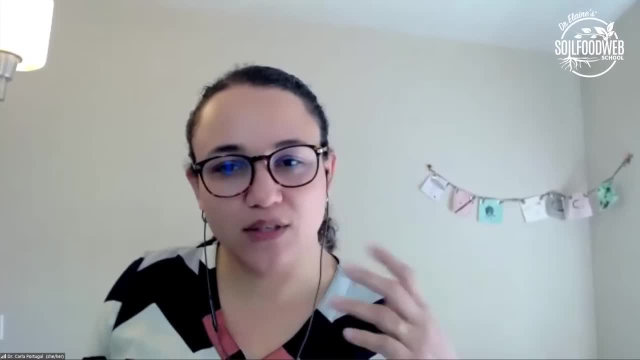 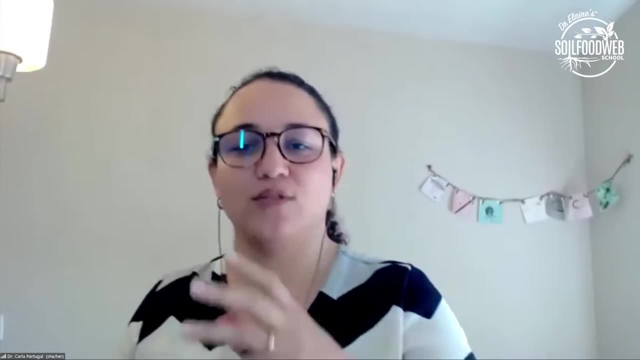 Yeah, if I may just compliment something, It's really about understanding what was the disruption on that path And have to deal with that first and then walk through to the restoration stages. So in a sense it might look like a longer journey. 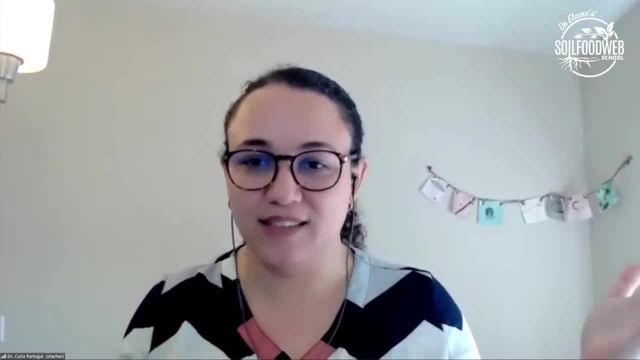 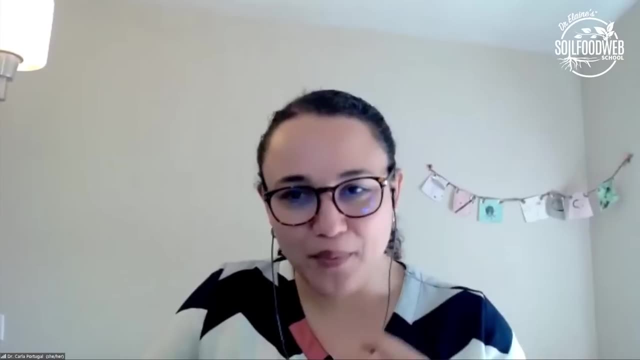 But it's possible And, like Adam said, it's a teamwork. right, And it's a team work. And it's a team work. It's a different set of tools, But the logic, the food web approach, is basically the same. Just different plants in different successional stages. So when we're dealing with agricultural plants, they all tend to be on the earlier side of the balances between fungi and bacteria, And so when you're doing agricultural crops, especially annuals, we're going to be able to restore that. 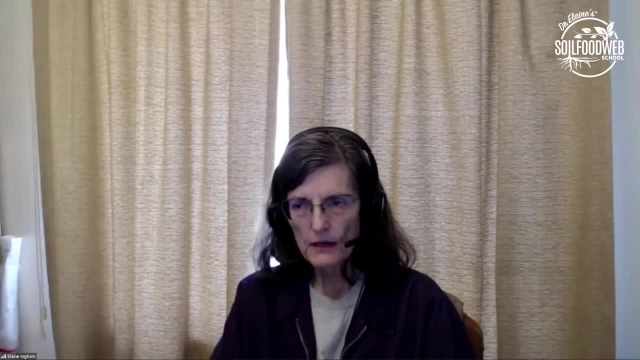 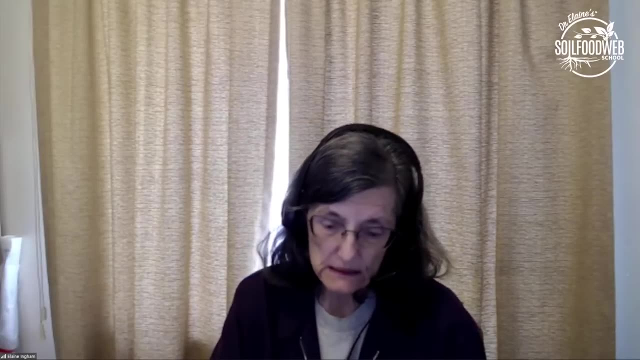 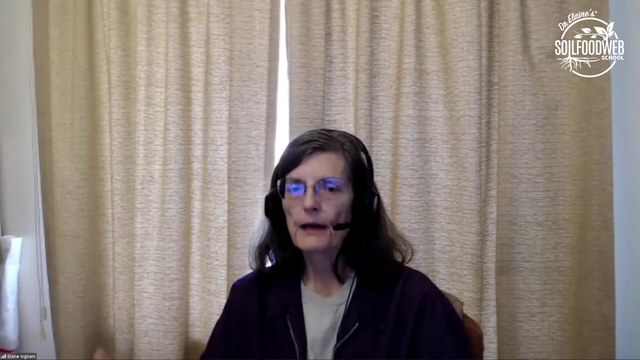 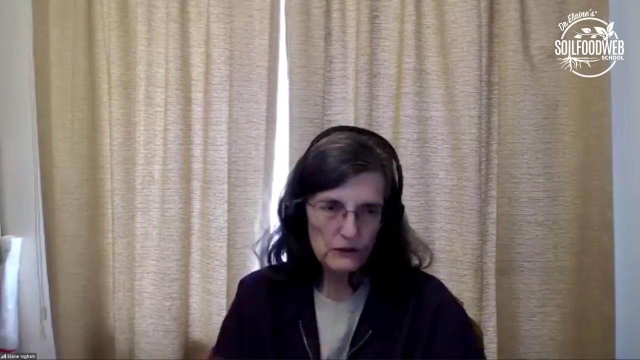 And fungal to bacterial ratios, the different kinds of predators and what are the balance with their prey. that can get done in the first growing season And, if you pay attention and you do the steps properly, get the biology back into your compost so you can inoculate that on your property or wherever you're growing your crops. So when we get into forest systems it's going to take a little bit longer, Because getting the fungi up to the level that you know, say, an oak tree, requires- or you know, fir trees or something- most of the when you have a group of trees. I love it when my brain goes on holiday. So orchard, there we go. So in an orchard situation, those aren't quite as fungal as some of the other plants, Those other trees that I just mentioned. So it might take you a year, year and a half, to get your orchard soil up to speed. 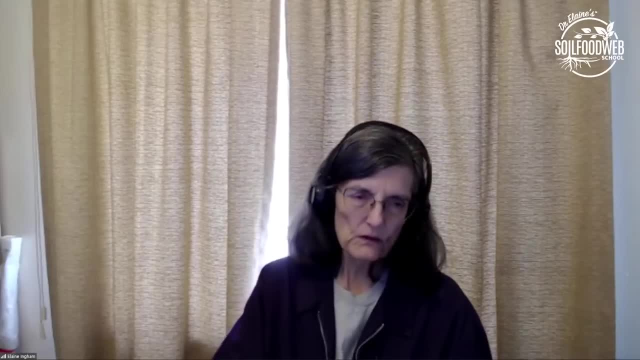 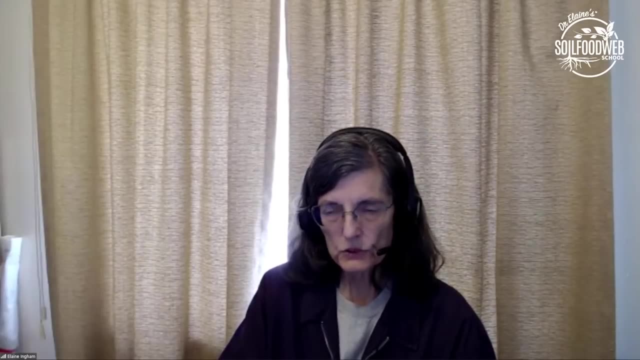 Same thing with vines and shrubs blueberries. It can take a little bit of time to get there, But in general it's not going to be too long And if you really pay attention to what you're doing, you will be successful. 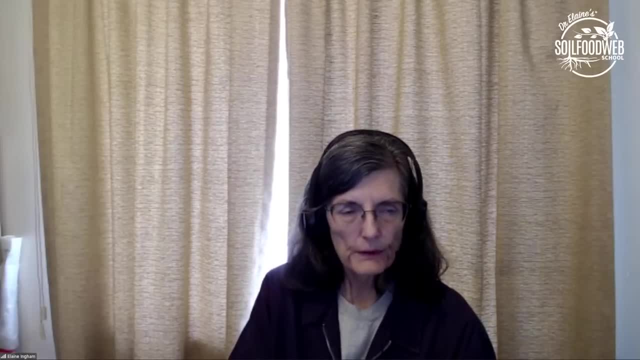 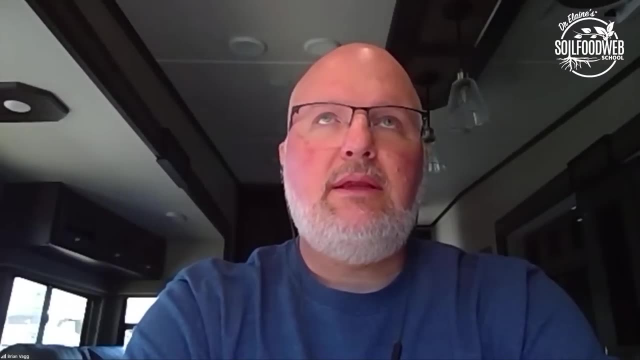 And even in your first year, when we're growing grapevines or blueberry Orchards. Yeah, You know, I've actually had to think about this question quite a bit lately, because I'm working on a forest restoration project right now And you know it's one of these things where fire was a challenge. 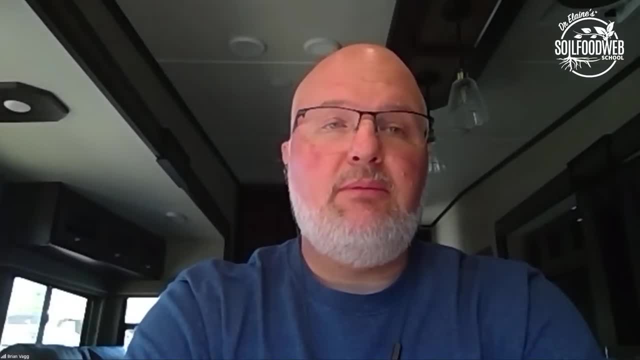 Where you know, fire suppression had been in play for quite some time frame And very, very hot fires with some frequency. multiple fires coming through this land had killed the pinyon pine, juniper, sagebrush ecosystem, And it's very difficult. 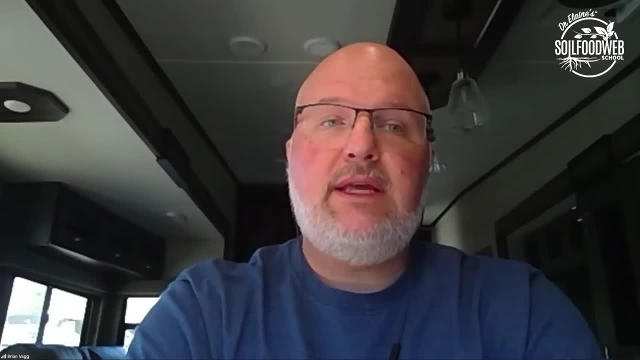 It's very evident when you drive through there. the forest land that had not burned, very few annual weedy types of species. It was a very set: pinyon pine, juniper, sagebrush, bitterbrush, you know everything was. it was kind of an ecological balance. 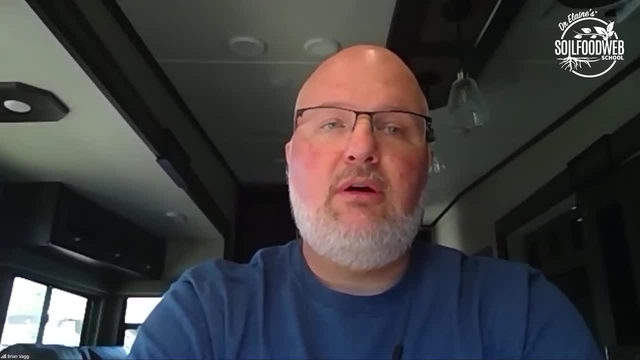 And then just across the road is where the fires had come through, And it was all cheatgrass and mustards and these very early successional plants And eventually, in Mother Nature's timeframe, it will restore itself Back to that pinyon pine, juniper and so forth. 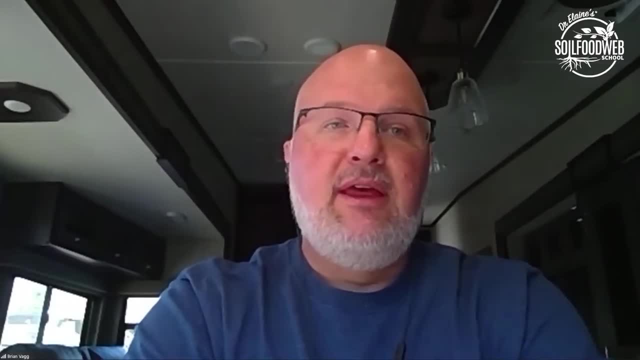 But from a human scale or time scale, that's a long, long, long ways away, And so our role is to come in there and try to restart and jumpstart that, that restoration, as fast as we can so that we can re-establish that ecosystem that's in there. 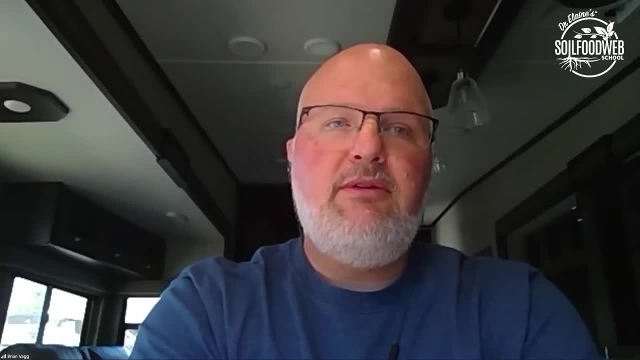 And so I think it's really important, especially you know that there are some of our practices that we do that will cause these significant damage. And so I think it's really important, especially you know that there are some of our practices that we do that will cause these significant damage. 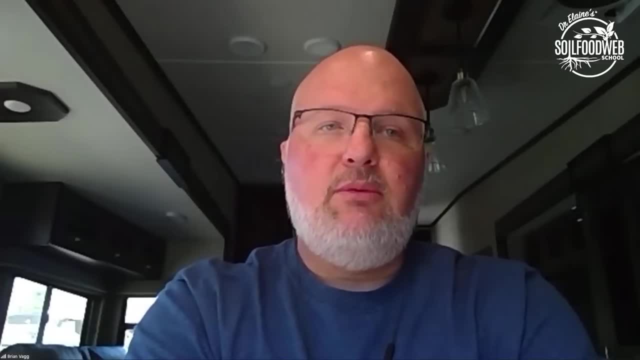 to happen. you know, because we eliminate fire and we stopped doing prescribed burning and you know cultural burning and things like that, It'll allow for these very, very hot fires to come through and destroy that ecosystem. So I think it is upon us to be able to be able to restore those…. 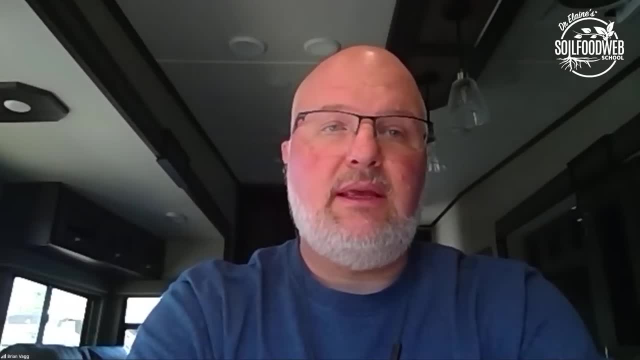 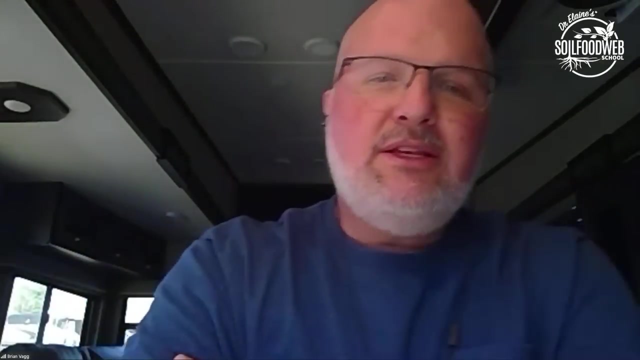 those environments as fast as we can, because I think it was our negligence that helped cause those issues. Okay, panelists, anything else you guys want to add? Oh, we could go on for real, Just one second and on, but let's go to the next question, you bet? okay? so the next question, um, and there's a lot of. 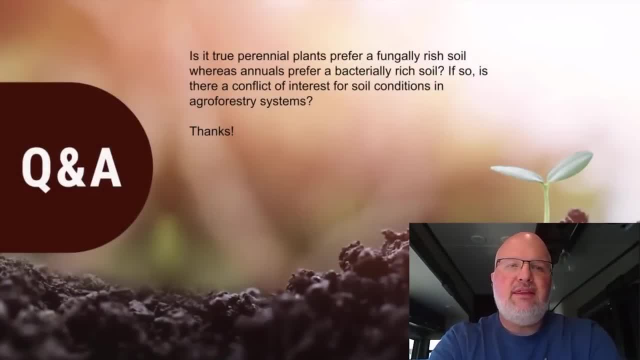 questions that seem to be very similar, so i'm glad that we're there's a theme or a thread to this um, and the question is: is it, is it true, perennial plants prefer fungally rich soils, whereas annuals prefer a bacterial rich soil? if so, is there a conflict of interest for soil conditions in? 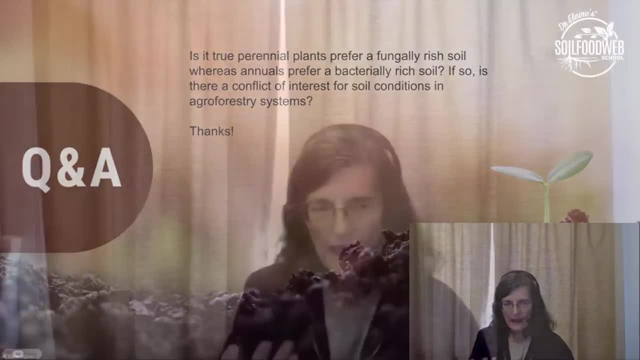 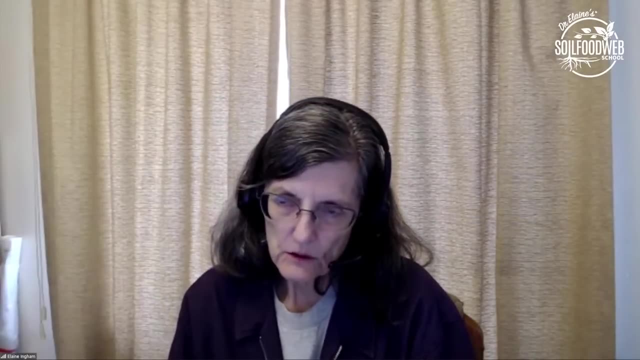 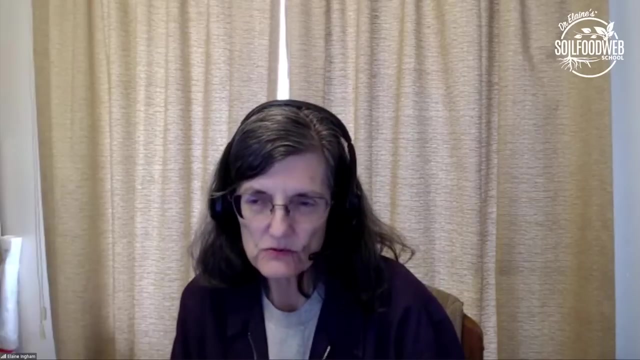 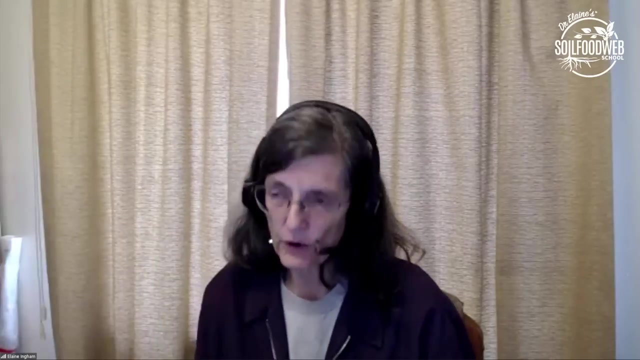 agroforestry systems. well, agroforestry systems are still going to be growing this, the same basic crop, the trees, and so we're just doing agricultural practices to those forests, some of which are really not very intelligent if you want a good, healthy forest system. 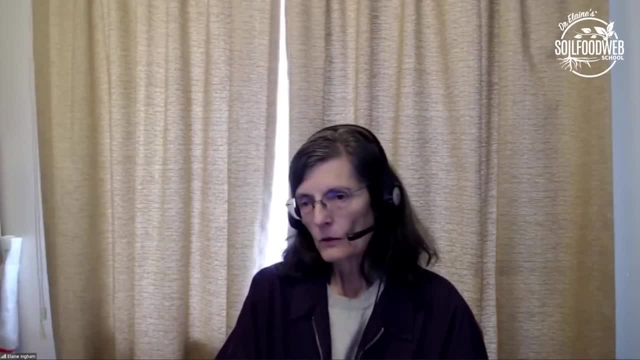 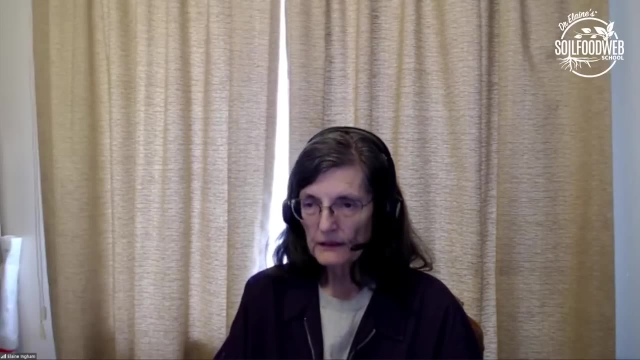 so there's some training that has to happen with with people to make them understand that you can't be destroying, you can't be disturbing the soil, you can't be going in there and pulling out all of the dead trees and all the dead logs and things. 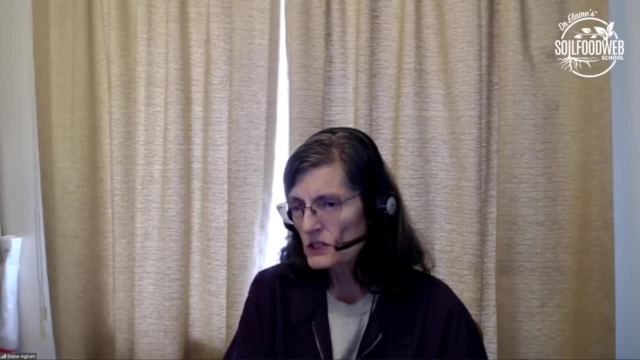 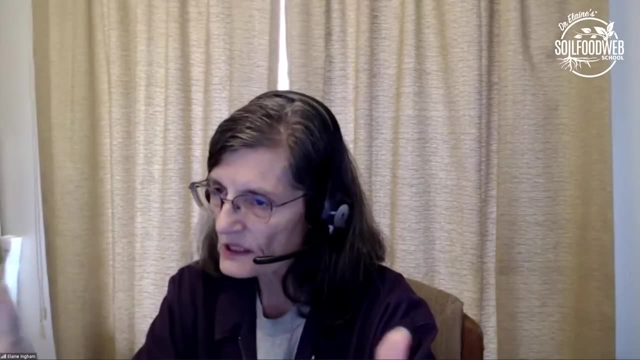 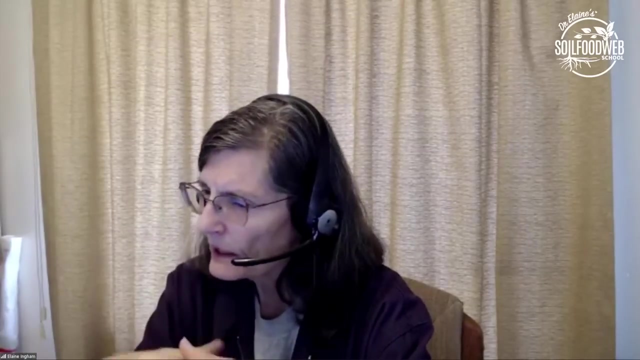 because you're so disturbing that situation. but then of course, you've got the fire danger. well, why aren't all of those logs decomposing? why isn't all of the woody material, wide seed n ratio material- getting decomposed and then you're able to do things that you're doing? that's not going to be. 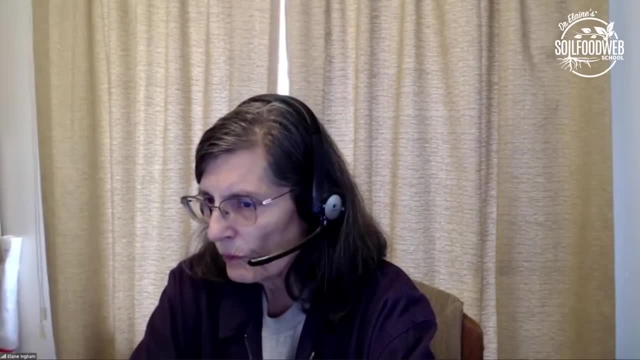 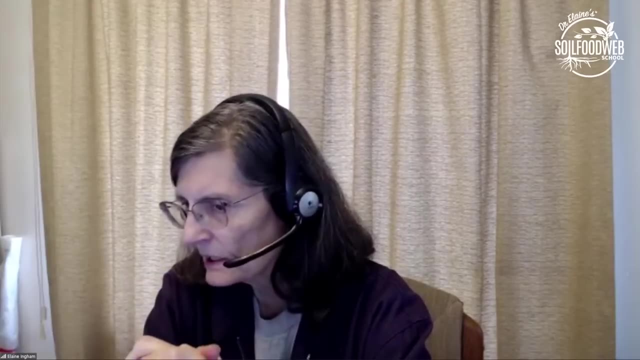 that's not going to be the same thing if you don't have all of your soil together and you've got to decomposed by the bacteria and the fungi. What's going on there? Well, you know that's a really slow, takes a long time to decompose these kinds of materials. No, it doesn't. Where'd they come? 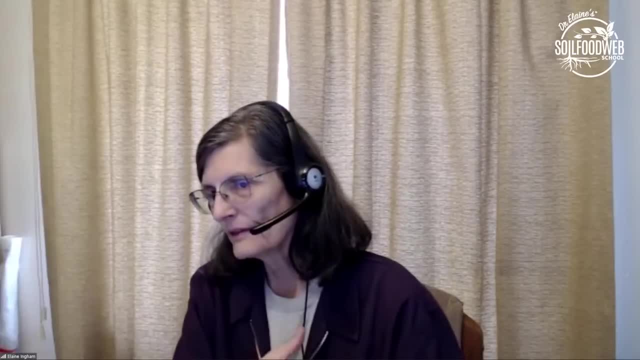 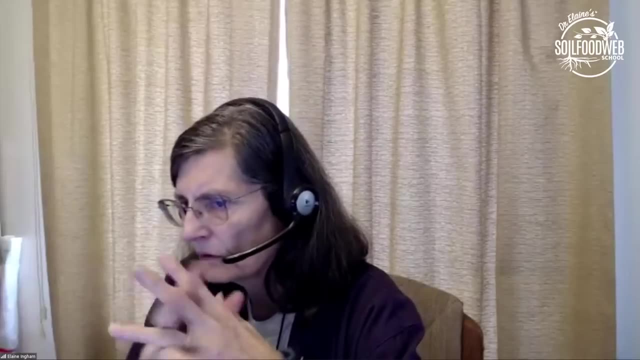 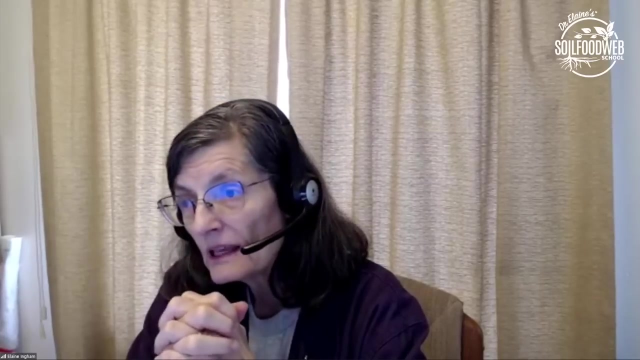 with up with the idea that you, the organisms, the fungi that work with really wide seed in ratio materials, would not be able to decompose those wide seed to N ratio materials. It's because we're out there spraying things and we're trying to keep the weeds down, So we're going to go out and 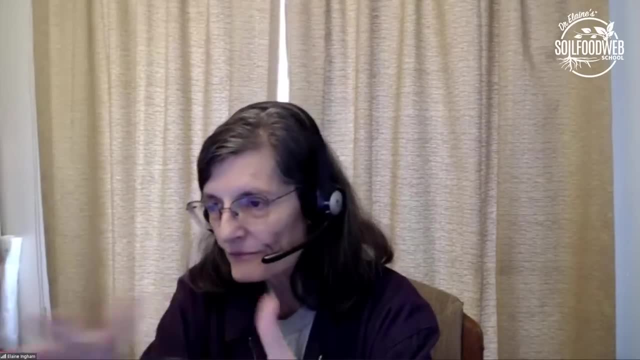 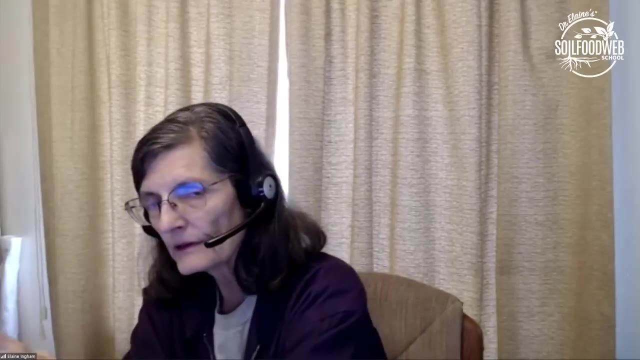 spray glyphosate. We're going to do all kinds of practices that disturb the system, when what we need to do now is because we've been disturbing those four systems. What we need to do now is to do all kinds of practices that disturb the system. What we need to do now is because we've been 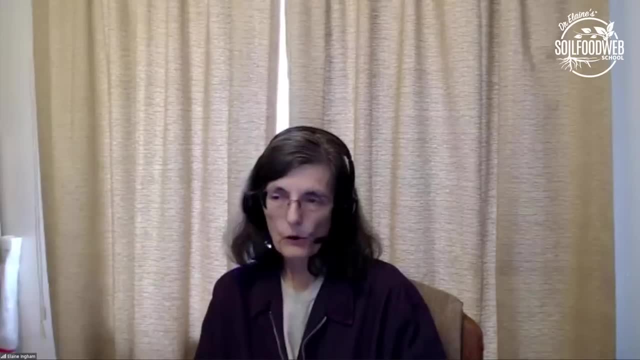 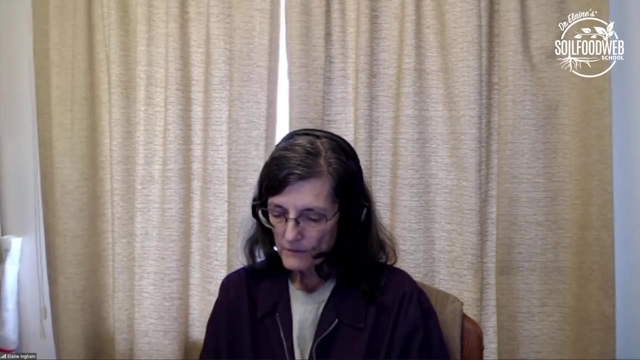 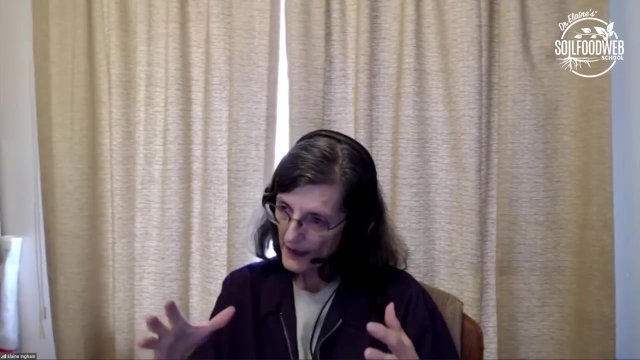 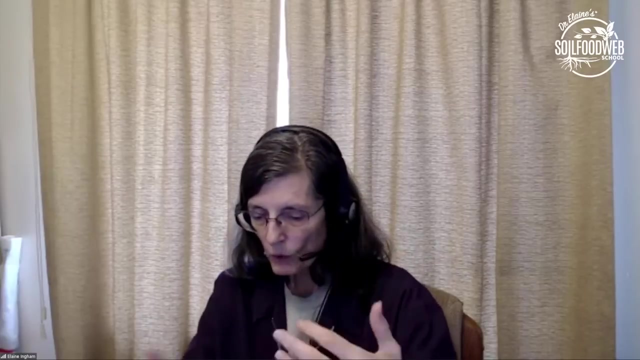 is go out and apply the missing micro microorganisms. When we look at old growth forests in the United States, we have data from, say, 1995 to the year 2000, where they had normal ratios of fungi to bacteria: 500 times more fungi than bacteria, a thousand more times. 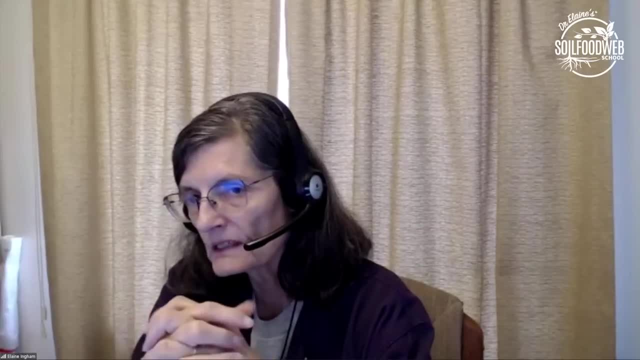 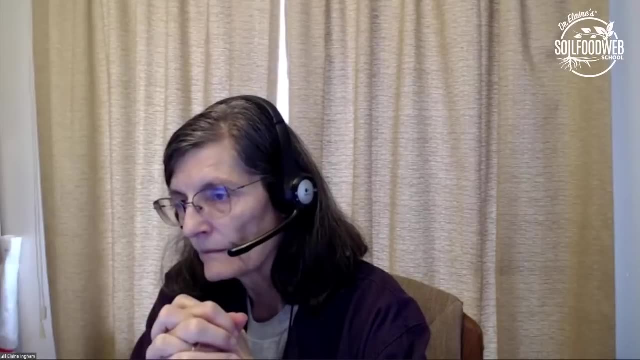 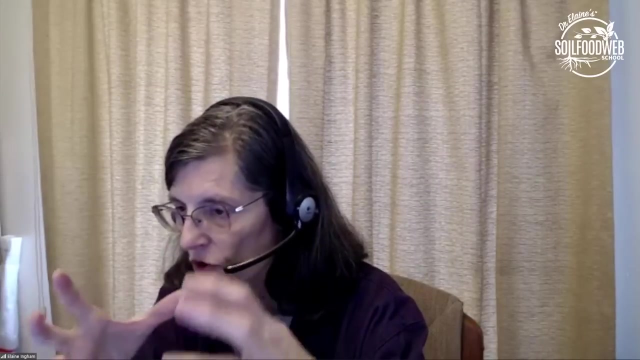 more fungi than bacteria. But you go out and you look at the same forest- SNAP- and it's almost equal fungi to bacteria. And of course you look at the trees and they're all sick, They're unhealthy, They're struggling to get through. I don't know how many of you know. in the Pacific Northwest, for example, that we've really seen that decline in the soil around oak trees. There are several very well-known parks close to San Francisco where they've lost all of the oaks just this past year, And so we have to. 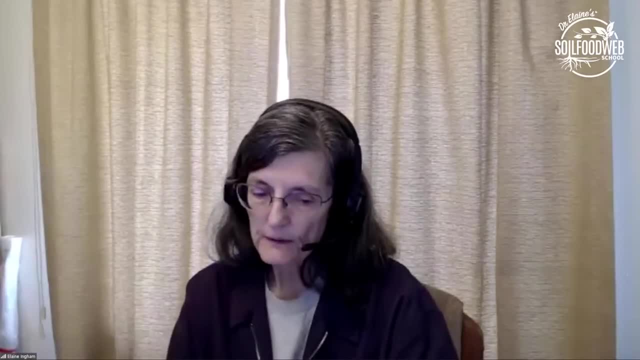 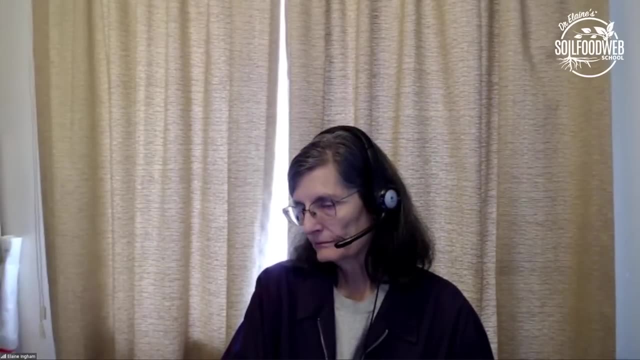 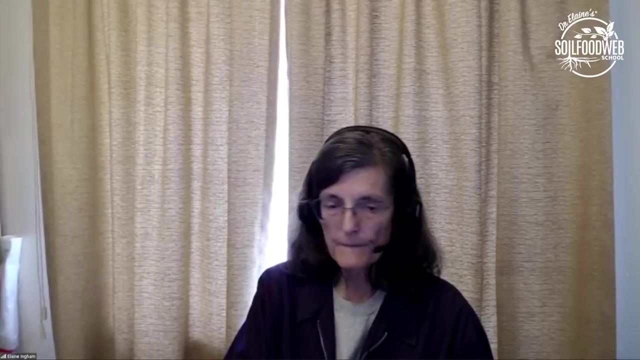 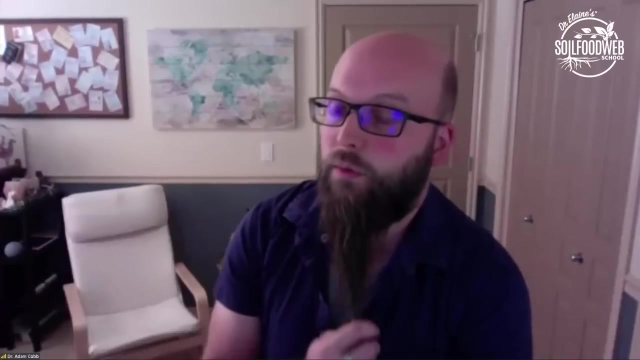 get that biology back into the soil if we want to keep these trees in the system And you can't be disturbing the soil. if you expect to get the biology back into that system, that will support the trees that should be there, I guess. I would just like to pick up on one aspect. Going back to the slide, I mentioned biodiversity. 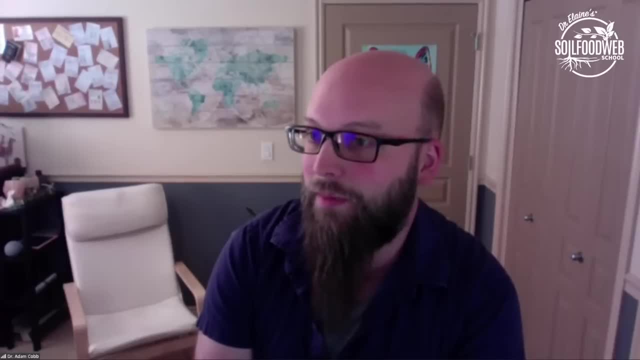 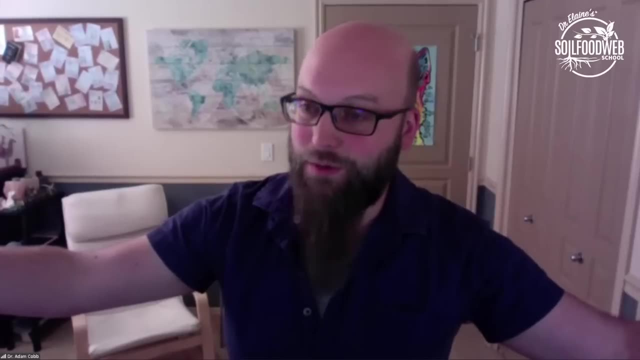 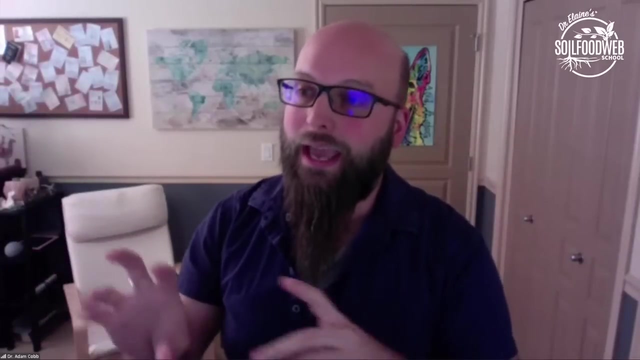 I didn't use this term, but I think about it all the time. It's patchiness right In a landscape. you want a patchy set of ecosystems In the soil, even though it's on a different scale. you want patchiness in the soil Areas where you know, because there's- you know there's- a lot of. 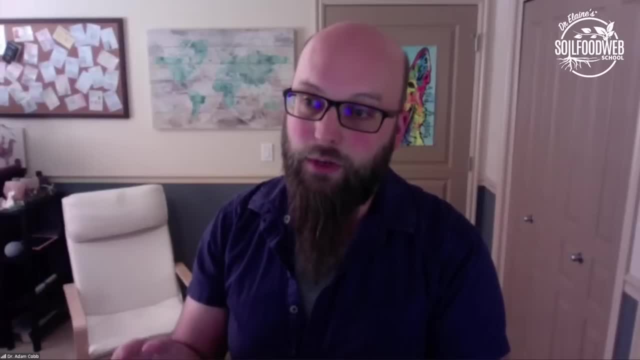 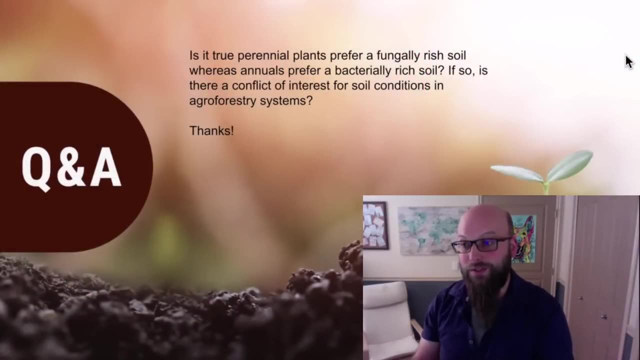 trees there, and because you created a more fungally rich compost, you get this proliferation of fungi in that area. But right next to it in a forest system might be a patch that's more bacteria-dominated and it has different plants in it, And so we're not trying to make it all the 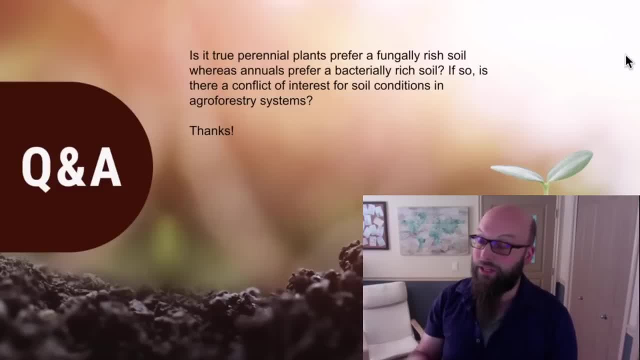 same, And in an agroforestry system, you're very intentionally setting up these different kinds of plants, And so your compost piles might have different objectives. right, You might make an amendment, a liquid amendment- to spray on those trees. that's very different from the one you would spray on the nearby grass. 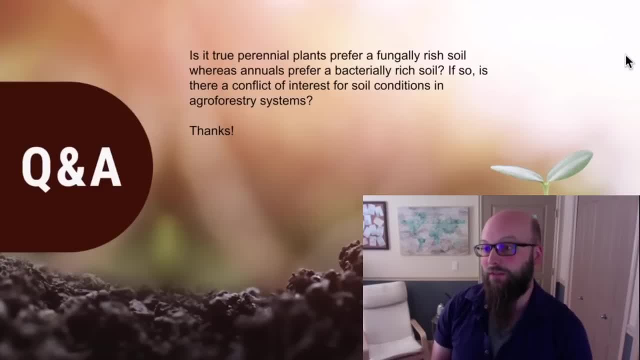 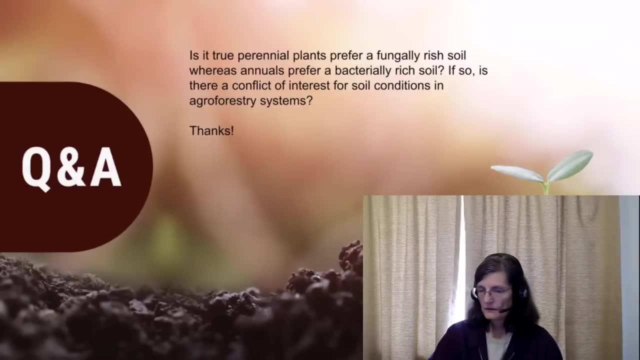 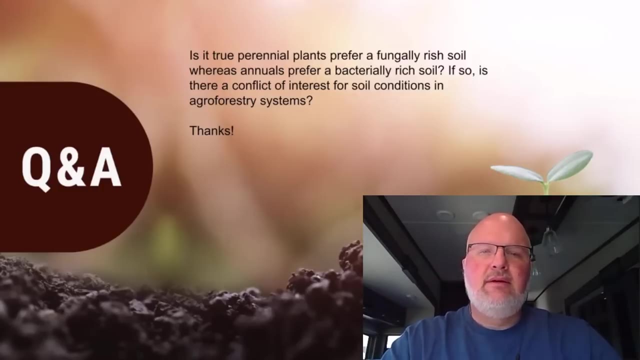 because that patchiness is part of biodiversity. Good point, Jenna. Excellent point. Thank you, Okay. Anything else you guys want to add to this question? I think Elaine and Adam nailed it out of the park. All right, Okay, Thank you. 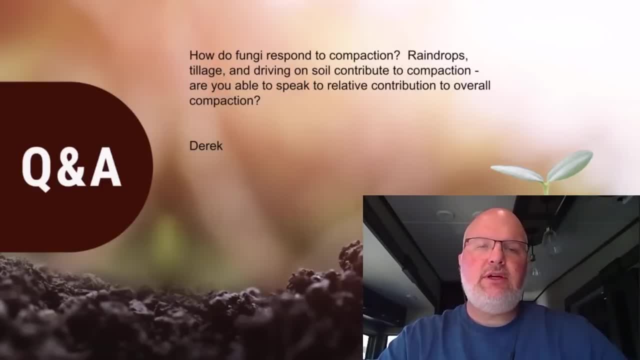 And so I think it's time to turn over to the next question, Adam. This one's from Derrick, And the question is: how do fungi respond to compaction? Raindrops, tillage and driving on soil contribute to compaction. Are you able to speak to relative? 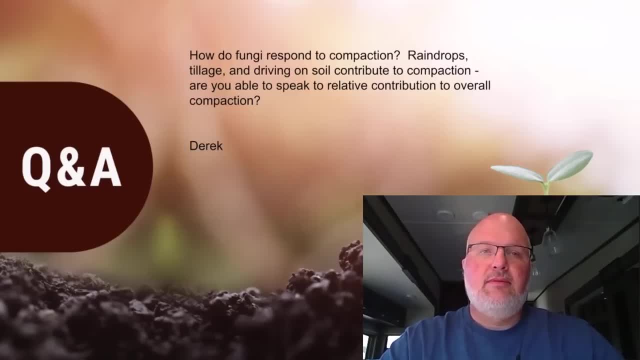 contribution to overall compaction. So fungine compaction- I'll go ahead and start with this one- And you know fungi again are going to be good allies for us to be able to help reduce those compaction issues, because they are the ones that help us create those macro aggregates that allow for us to create that soil structure, to get the pore space. 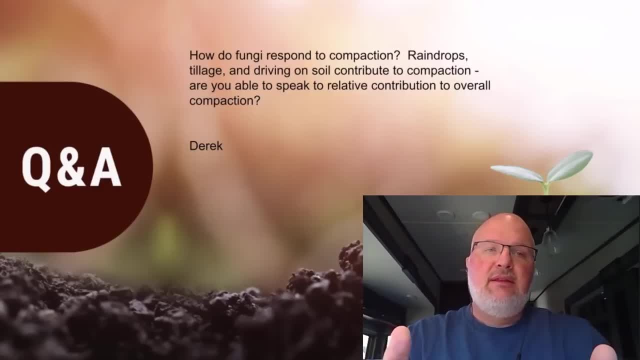 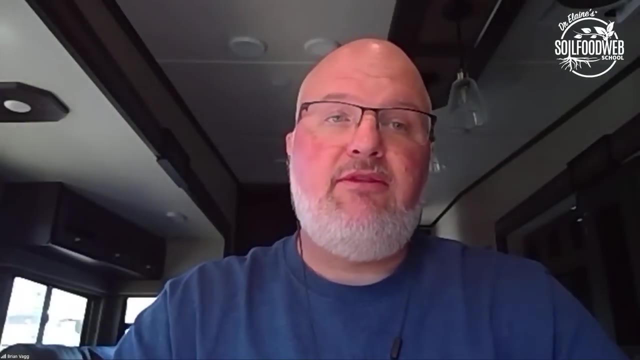 And they also will help with the chemistry. You know Adam talked about the biology being kind of the keystone to the physical and the chemical. That's for sure. They are going to impact both of those properties of soil, And so fungi can be great allies for us to one change the chemistry in the soil to help flocculate our soils. 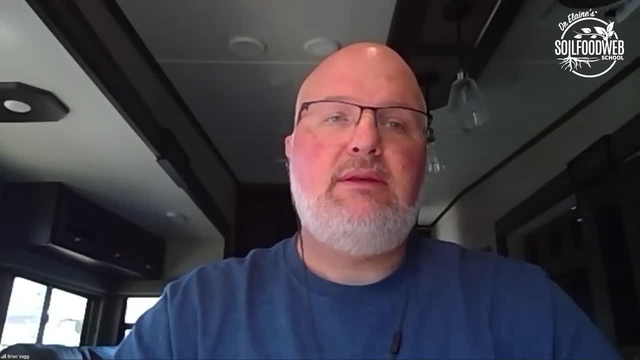 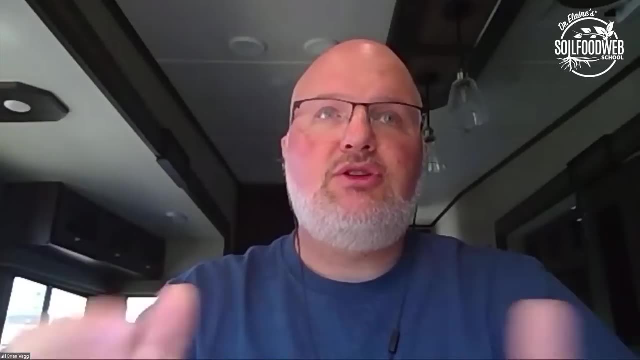 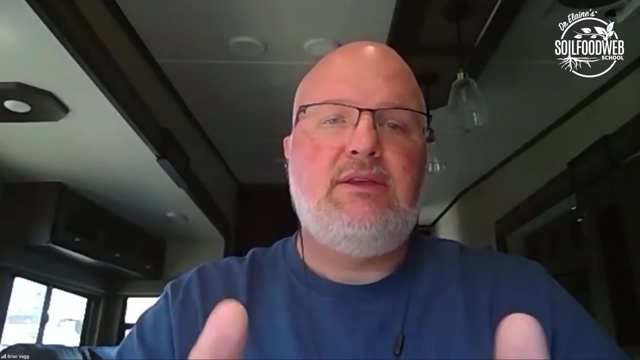 And again, it's just going to set the right balance of certain nutrients so that the clay platelets, you know, repel each other versus actually stack upon each other, And then creating that structure in the soil to allow for the aerobicness to be able to, you know, keep that ability of water holding capacity inside the soil. And again reducing compaction in that sense as well. Now a challenge: you run into you till You may decompact for a very short period of time frame, but you've just destroyed all of that structure and that soil will compact through raindrops and driving on the soil. 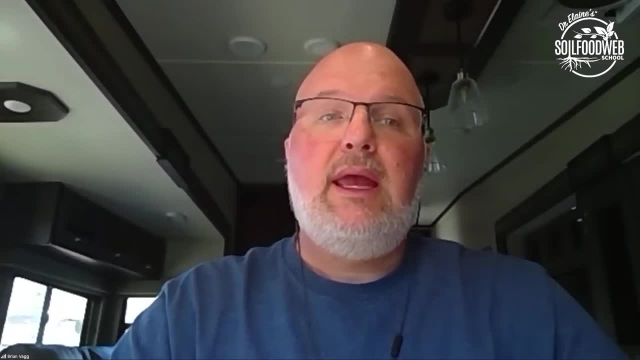 And if you keep on tilling you're going to lose that soil structure And this can be really hard, I think, for those fungal communities to rebuild back into that, because you're starting again from a compacted environment. So anybody else want to add to that. 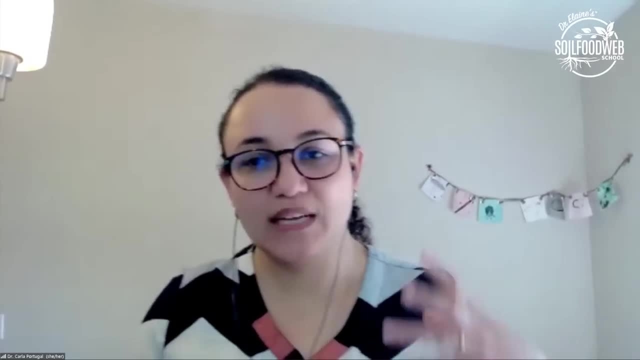 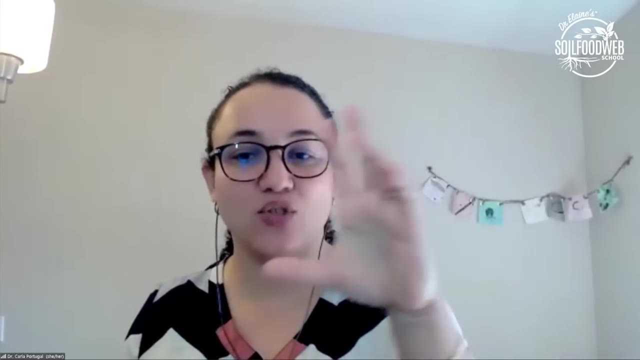 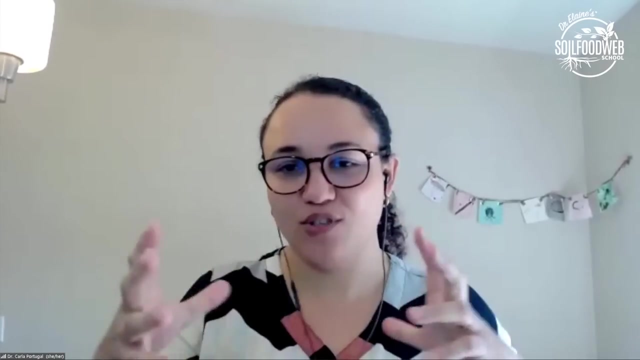 Yeah, like you said, it's just about the structure: right, Right, Right, Right, Right, Right. So really pay attention in the process of how each event or action is affected, this soil structure, and reapply what we need to help heal that structure, put back in place, put the biology back in place. 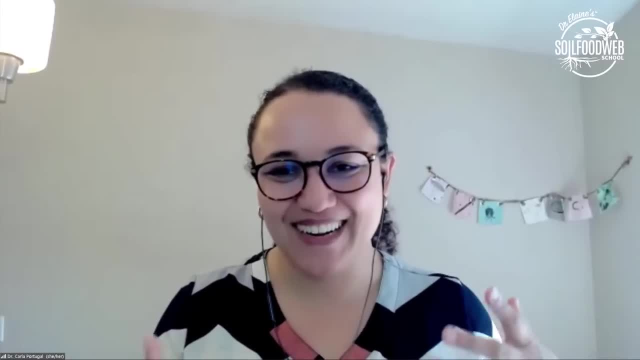 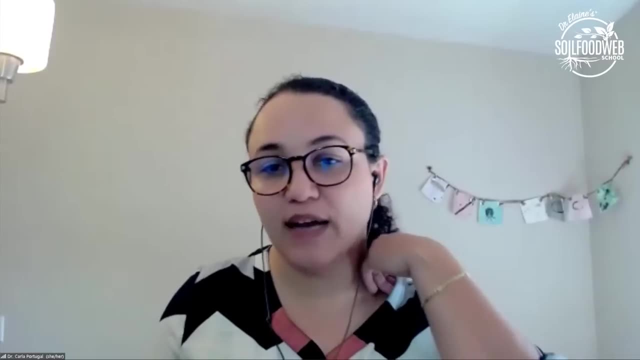 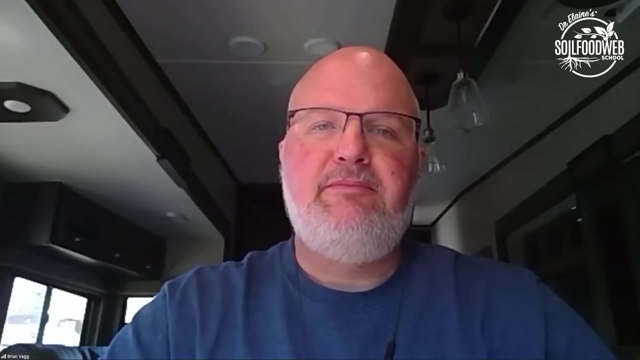 So it's always this detective job, right, Really pay attention to what nature is telling us, how each action or rain or storm or whatever is affecting your area. But, Brian, you summarized very, very good, Thank you. Yeah, And there's one more term that goes with compaction. I'm not sure I heard which was the plow pan. Yeah, So if you have tilled previously many times, you'll tend to get however deep. your implement went right under where it was chopping up the soil. That's where you tend to get a pan, a crust of really compacted soil. 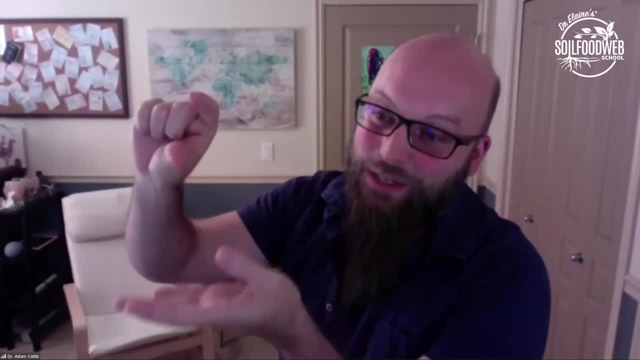 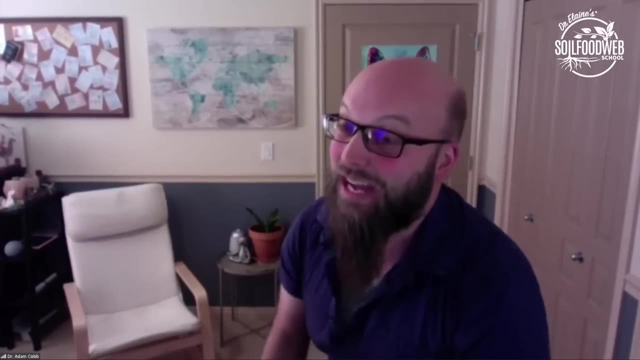 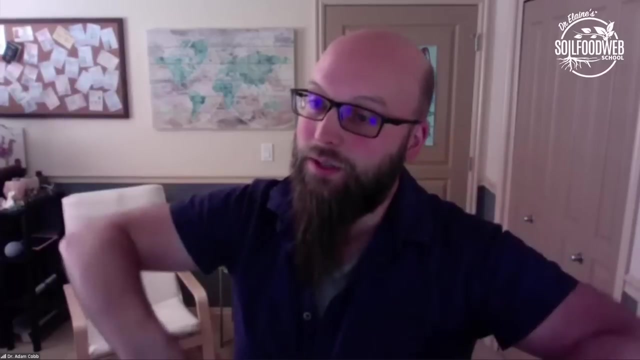 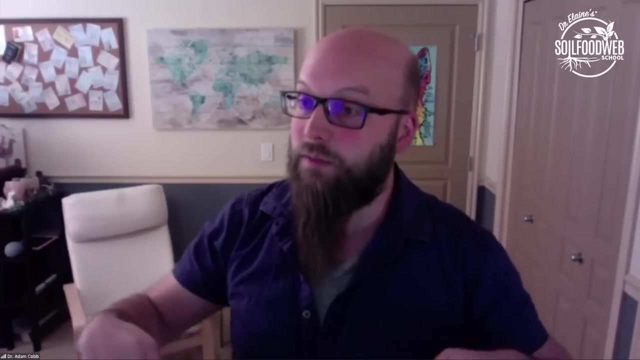 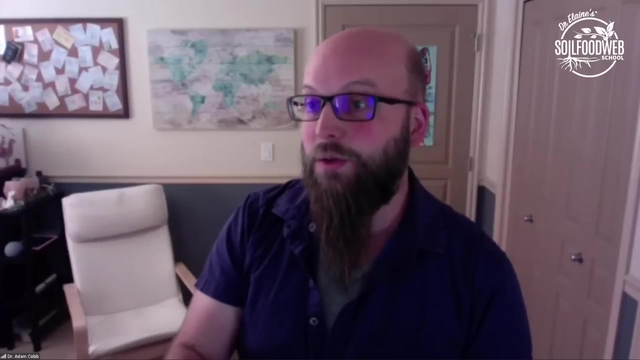 And just under that is often A really anaerobic soil environment where a lot of nasty pathogens might be building up, And so sometimes we advocate for the last tillage event right, that you go in with something that can rip really deeply like a key line plow, maybe disturb the top of the soil as little as possible, but have something that goes down to where that plow pan is, tears it apart and then get the biology in there right away so that it can start to change. 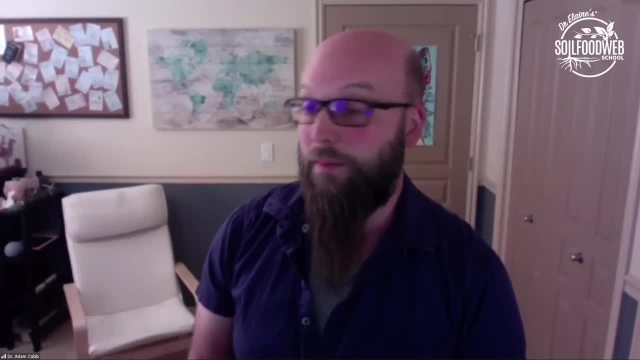 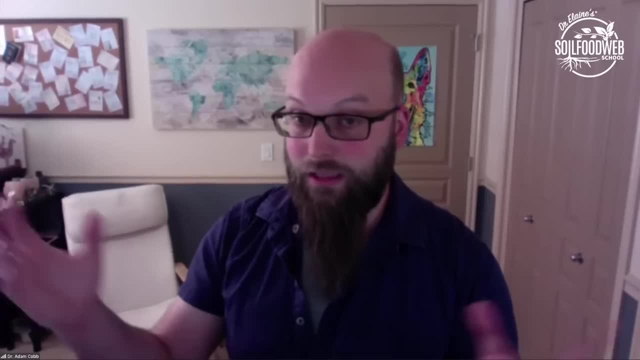 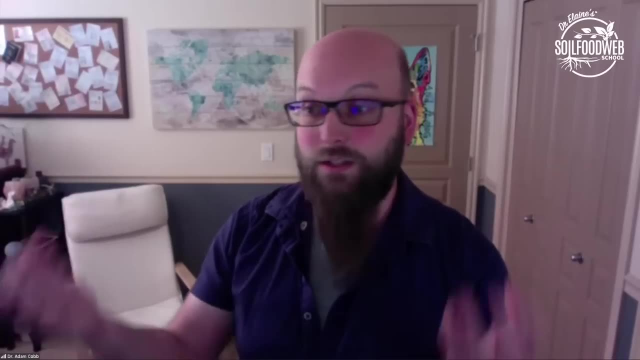 You know- we had someone in chat talking about that- they've been inundated with lots of rain, But if you have a spongy soil, that rain is not a problem. It's going to soak deeper and deeper and deeper. There's not going to be layers of compaction. 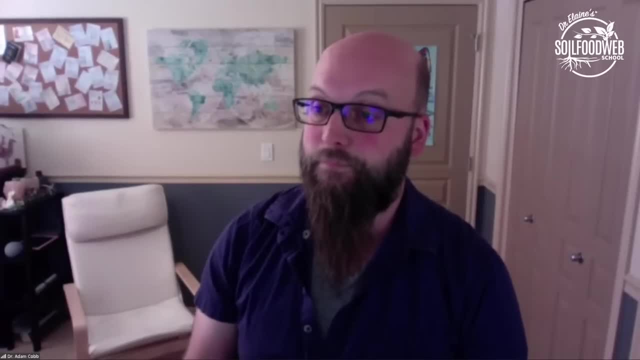 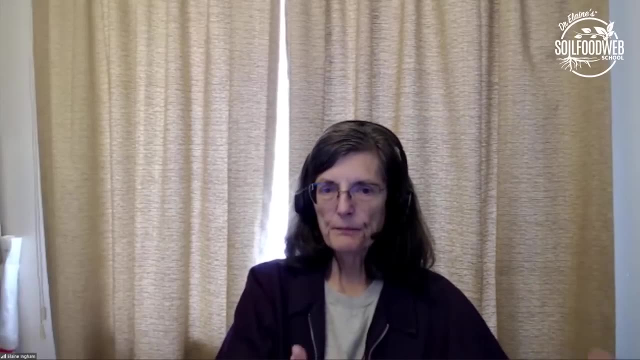 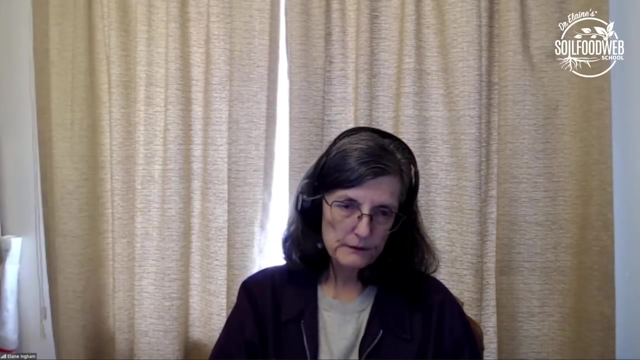 Right for it to hit and pull up on yep, and one of the things to always remember is if, if you're getting things physically fluffed back up, you have to immediately get the biology back in there as well, and then, as rapidly as possible, you want to have plants in that system that will intercept. the raindrops falling from clouds, because the most compacting thing, probably in most people instances, is going to be that raindrop smacking into the soil surface and causing compaction somewhere around four to six centimeters. so you may have slightly different things, but please monitor constantly to see if things are coming along as they. 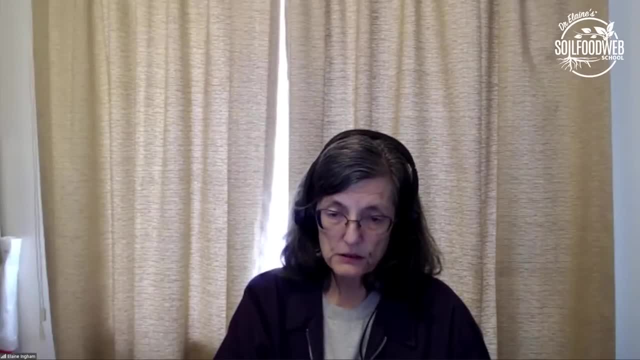 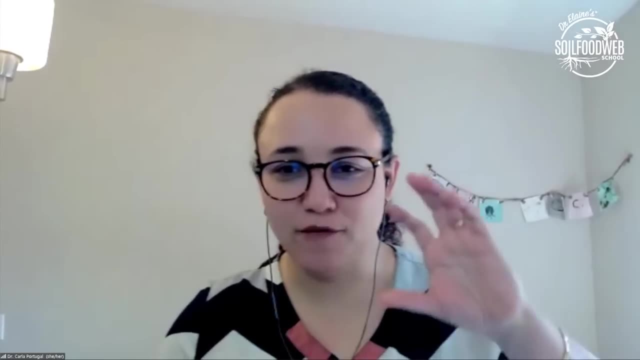 shift, and if they're not, then you're going to have to get the biology back in there as well should be, and if they're not, get out there with another application of the right biology. and may i just like there to say that we have to sometimes put ourselves under the micro. 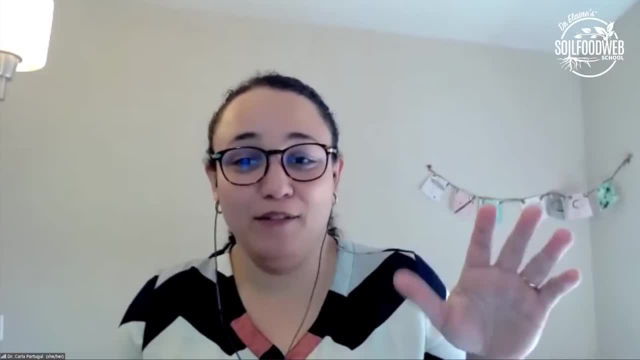 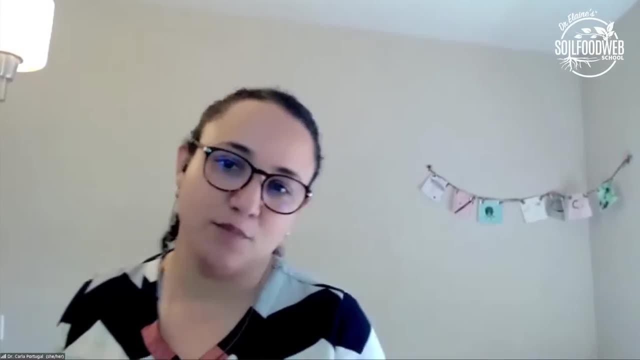 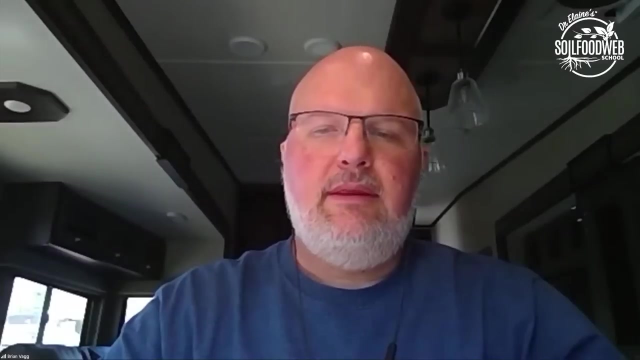 perspective right, because raindrop for us is nothing. for these tiny little creatures it's everything. it's like a tsunami. so put ourselves under their perspective to oversee the actions as well. yeah, okay, anything else folks you want to add? yeah, all right, i think we we got this one done. all right. next question is from kathy, and kathy asks: how long will fungi and other microorganisms survive after the soil has been tilled and left barren, and how long will it take for a new colony to establish itself naturally on tilled soil? do you want to take that one? oh boy. um, how long will fungi and the other and other microorganisms survive after the soil has been tilled and left barren, and how long will it take for a new colony to the soil has been tilled? well, tillage is going to take out about 50 percent of the beneficial. organisms that you need to have, and so if there's no new plant growth going into that system, then those organisms are going to go dormant and the dormant organisms will often be able to survive for quite a few years. so hopefully you would, you would get at least the things that would come in. and establish, you would get the weedy species, all those wonderful thistles and things, and so food starts being put back into the system. it's just that it's food for the wrong critters. if you're trying to grow something, in a year or two you're going to put in something that requires a very high fungal domination in that soil. so how long will it take for a new colony to establish itself depends on how big the area was that was damaged. so if you have just a little garden and you you know 10 feet by 10 feet and you till all of that up, it's going- the organisms. 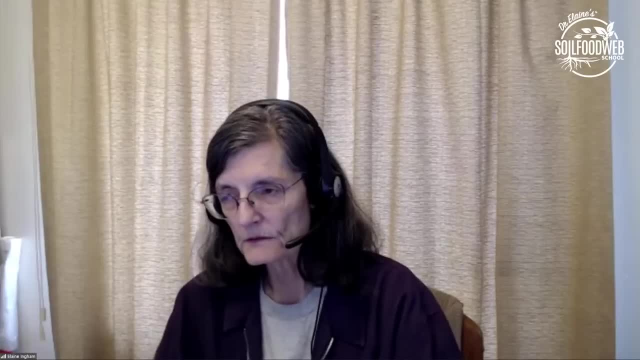 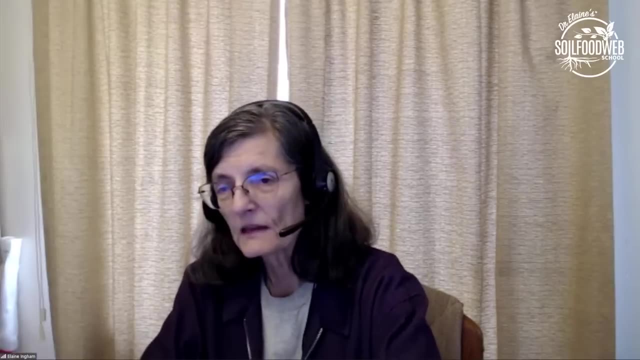 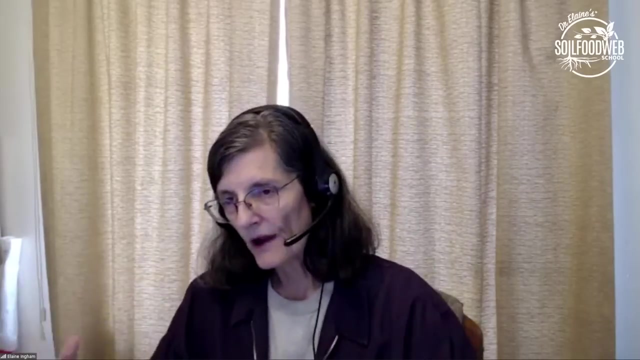 from outside that weren't harmed, that weren't destroyed, they're gonna sneak in and go: oh, look at this nobody's home. it's a great place to live, especially that they've put vegetables in or saw. you know, now there's something growing there. if you disturb a larger size- and we've did this- these are experiments that we did in the peninsula in washington state, in some of the mature forest systems there where they would clear, cut 10 acres and we would see that it would take a year, maybe two, to get the biology to even start coming back. so think of all the time there was for erosion to happen and loss of the soil. we figured in an especially rainy year, there was three inches of soil that was washed down the hill, gone from the system and causing damage in all of those ecosystems where that water flowed to. it was going to be harmed by the erosion that was happening in that area. that wasn't, you know, wasn't? 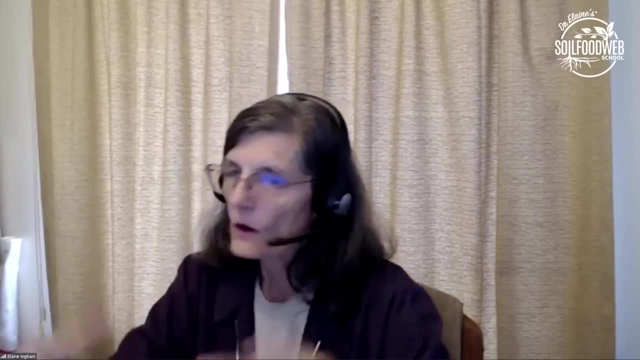 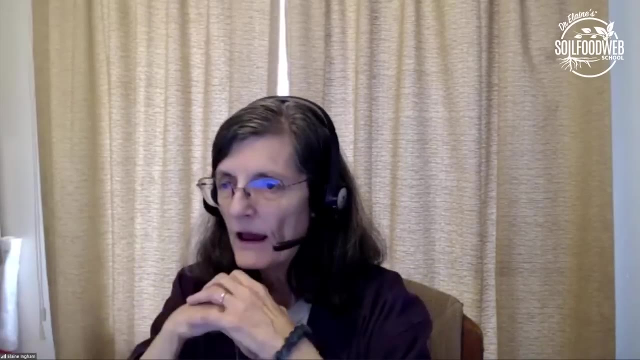 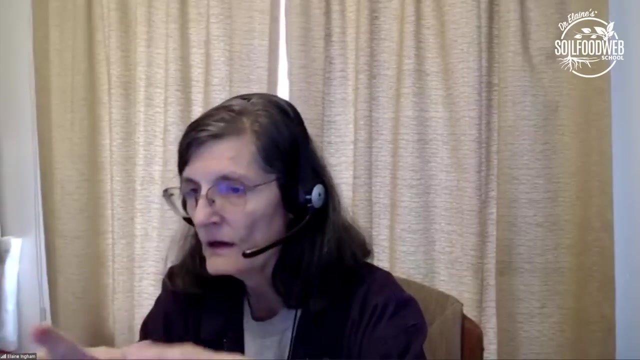 fixed in any way. after it was clear cut, go out and even larger, even bigger. clear cut. you know, several a mile or two across, and there are places where the only plants that are growing in those soils, in the center of that disturbance, are still the same weeds. 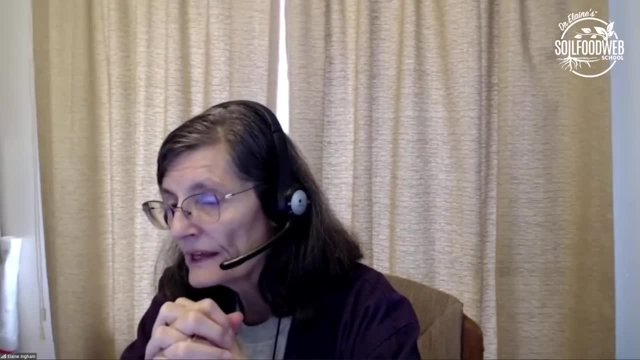 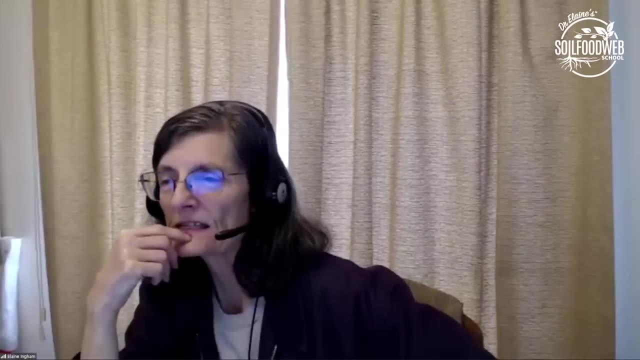 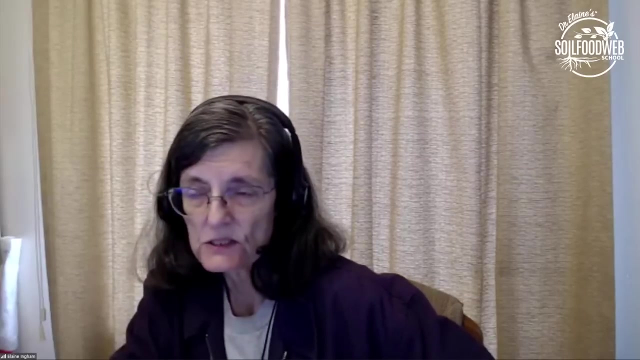 there's been no recovery at all and something like that's the last time i adding, got to add on the year since we i was working on that system, probably about 40 years. um, where there's, it's still in a weed situation. it hasn't improved at. all. so everything depends on those organisms coming back. what's bringing them back? well, if you've, if that animal, the bird's got to fly two miles and it's going to have to fly two miles. and it's going to have to fly two miles to the center if the deer have to traipse over out in the middle. 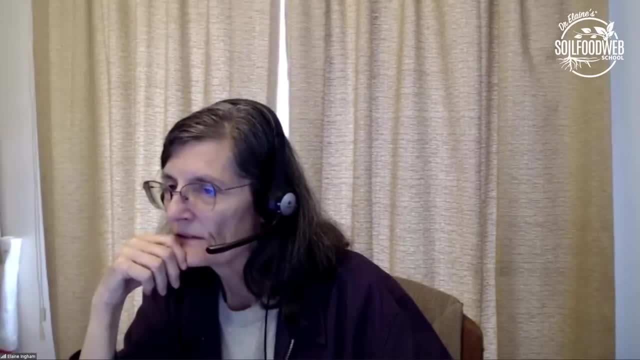 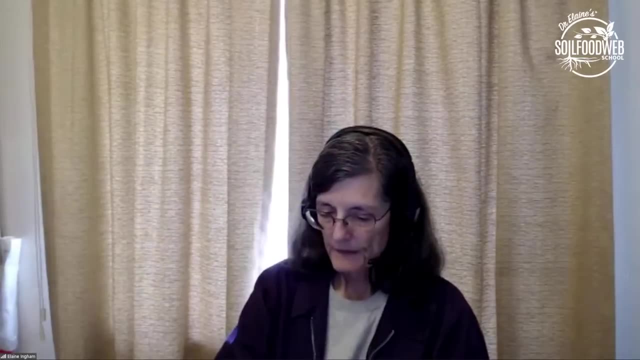 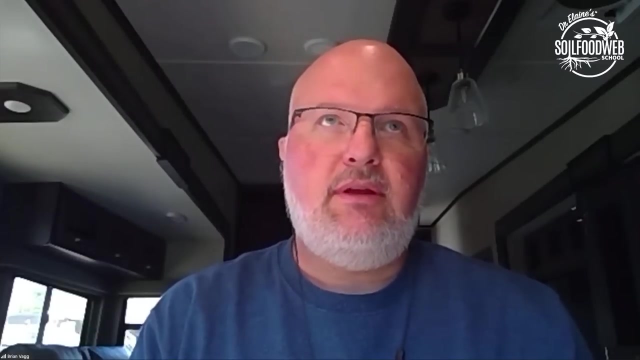 of a clear cut. there's no way they're not going to be there, so it's kind of critical for us to get these organisms back into the system. yeah, i think of an analogy of you know, like a natural disaster from a human standpoint, um, a very small disaster. it's very localized. um, it was probably much faster. 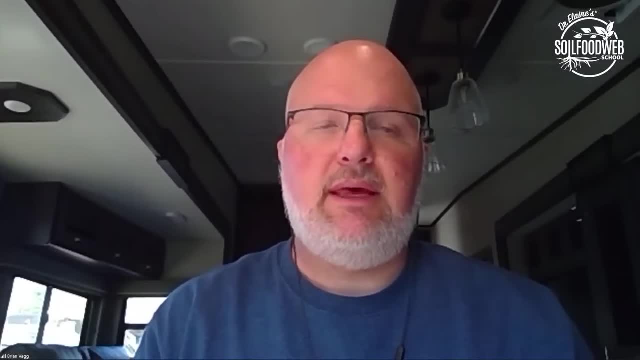 to recover because there's a lot of infrastructure around to help, you know, rebuild that environment. but if you have a massive natural disaster, that it impacts a huge swath of land, um or area, it takes a while to be able to try to rebuild in that and, and if you don't put any investment into it, any energy to try to improve the system, it may take a very long time for for the roads and the buildings and everything else to kind of get rebuilt back up. but if there's a lot of investment where we're intensively going back in there and 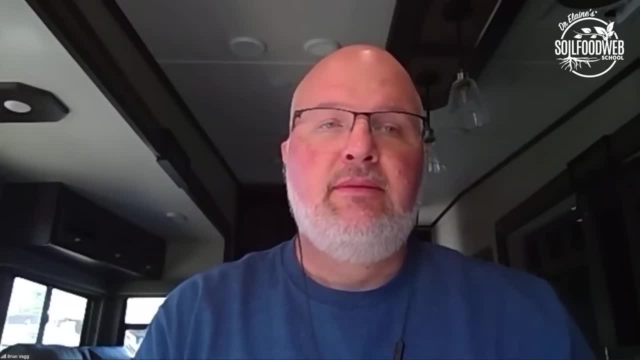 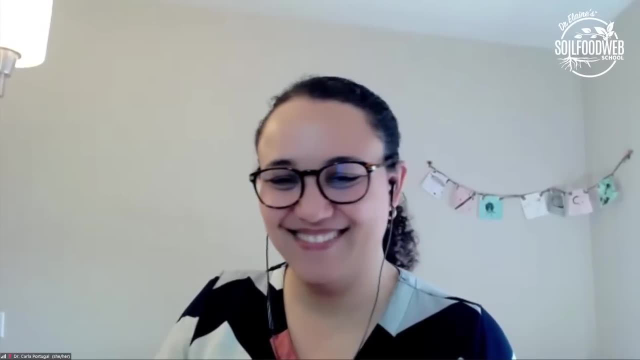 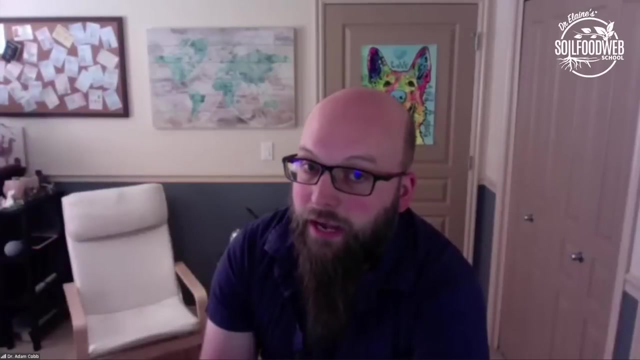 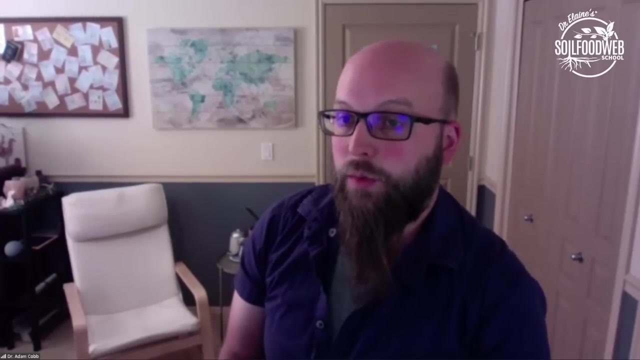 trying to rebuild, it will happen in a much faster standpoint. so, um, hopefully that analogy made sense. yeah, totally, yeah, all right, uh, panelists, anything else you guys want to add? i mean, okay, the question about natural reestablishment. i, i know that with our muscular mycorrhizal fungi, which is what i've primarily researched, that the spores for those can. 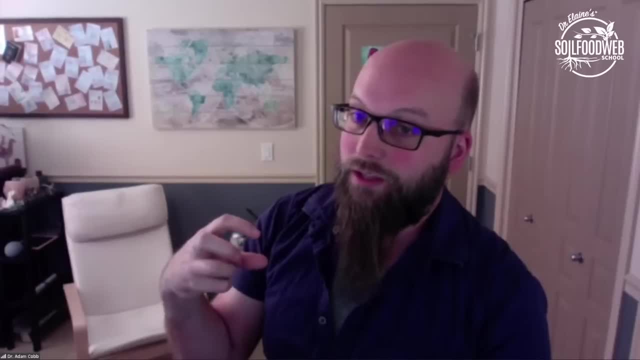 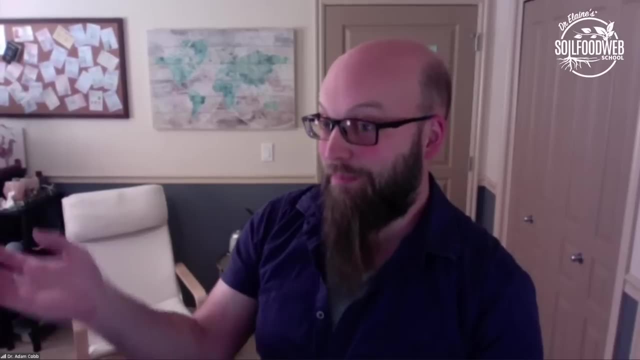 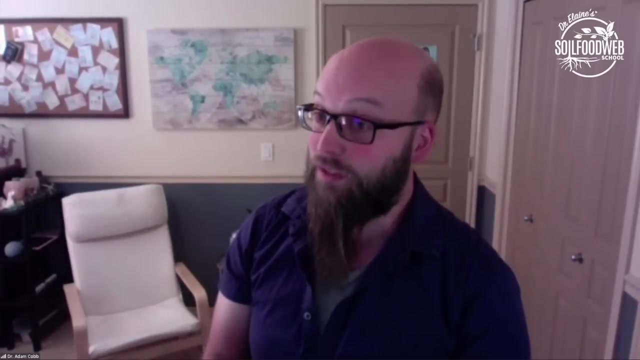 blow around in the air but, much like elaine said that plants that are earlier successional can be more aggressive and some of those spores that blow around in the air we think might be the more weedy species, the more aggressive they might be. less beneficial to plants, especially later successional plants. more beneficial to maybe early successional plants right, and so natural establishment, the do nothing approach. you can- really you could- be talking about decades before you're getting back to any kind of soil function, which is one of the reasons why we're so focused on helping people find locally adapted diverse microorganisms and speed that process up. 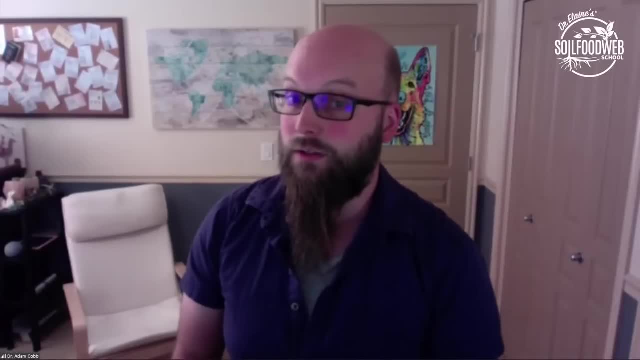 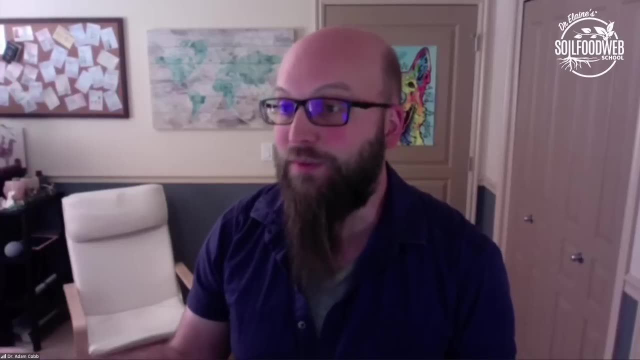 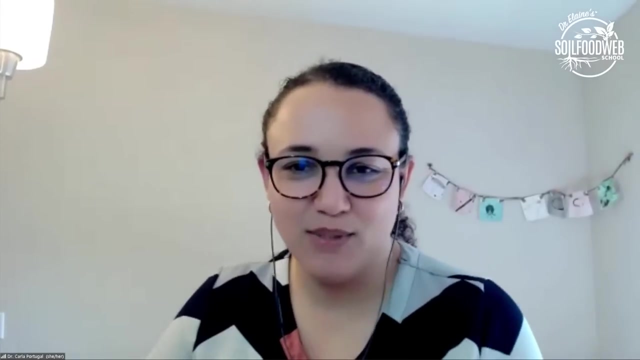 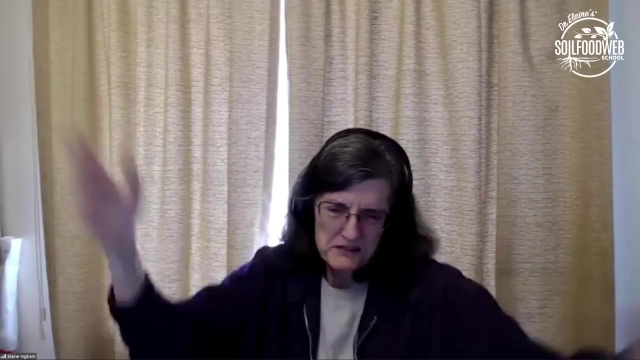 by inoculating that soil with good compost extracts and peas, because that natural reestablishment can be like half of a human lifespan. right, mother? earth's time scale versus human time scale- two totally different things. we are just dust in the wind. yeah, exactly, mother goes. ah, you know so. it takes uh, 50 years, 100, 150. well, who cares? i'll get it there, don't stop. 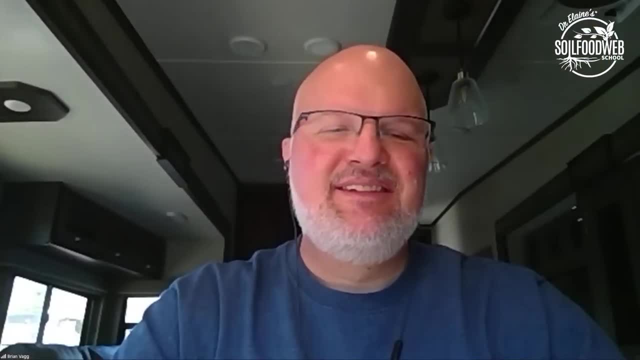 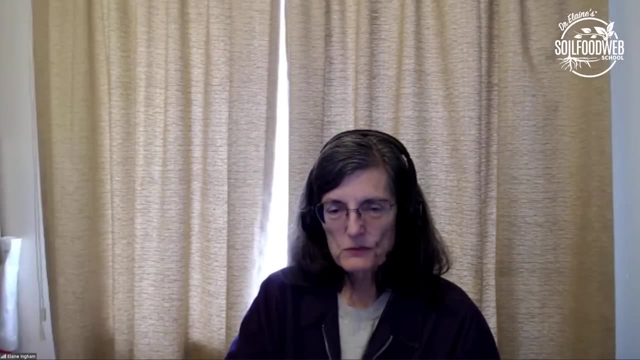 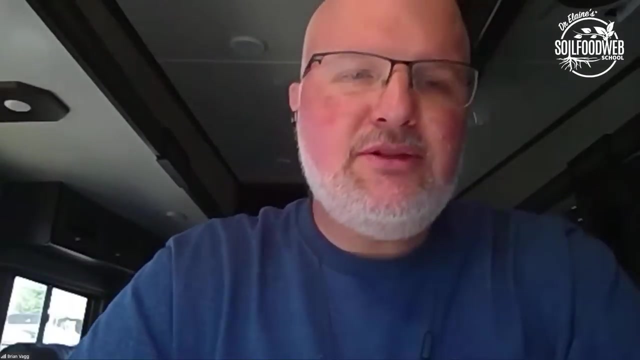 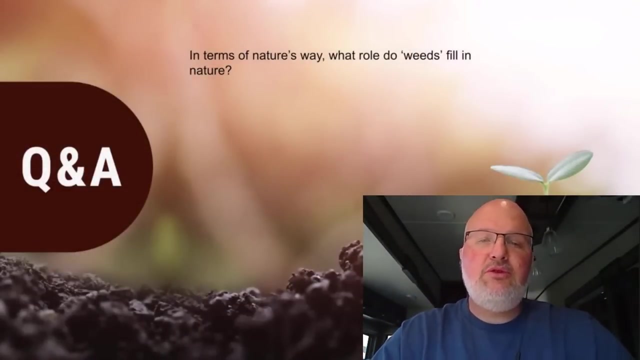 fussing exactly, but if we want to live downstream from that ecosystem, from that disturbed system, we better start getting those plants back in as soon as possible. yep, okay, let's move. next question: um, i love this question and we've had a lot of discussions around weeds and in terms of nature's way. what role do weeds fill in nature? 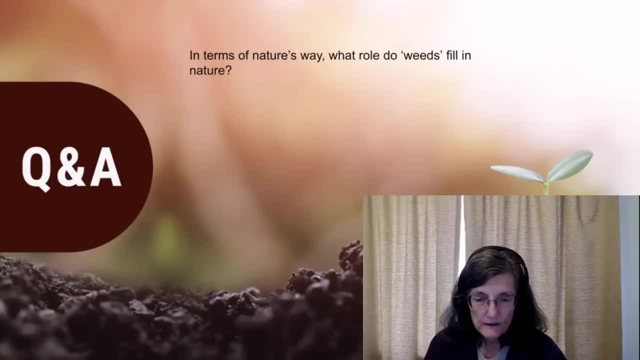 it gets things started again. you know it's uh going from bare dirt where there's no biology really, you know, getting stronger, getting more numerous where they all that you know, and uh, no. so with no, um, no plants in the system, all those organisms in the soil are just gonna. get more and more dormant or die. they have to have food um, and if it takes 20 years for plants to really come back um it, it's going to be really hard to recover that area. it's going to take a very long time. so weeds start the whole process. how important is it that you've got thistle starting up over? 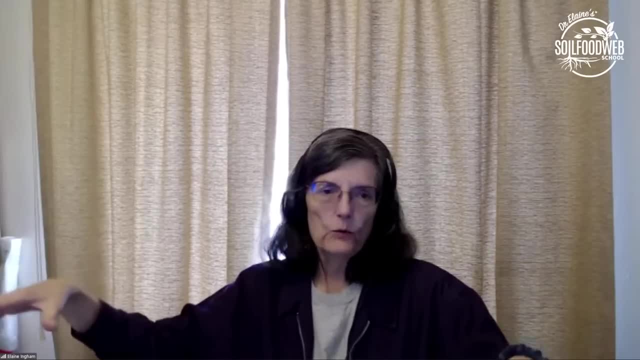 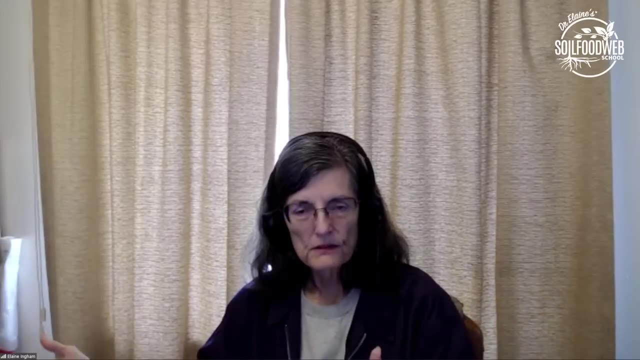 here and over here you've got, uh, ragweed, and over there you've got the predominant plants and you've got the predominant plants and you've got the predominant plants. and is something else. it changes the course of the plants that are going to come into the system. so even there we want to. could. could we get the fastest um set of weed seeds to, uh, get in and have a highly diverse set of weeds so that you can pick what you want? or does mother nature picks what she wants? well, interesting conundrum, isn't it? 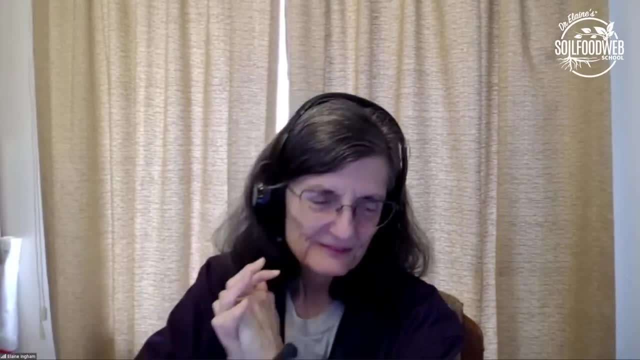 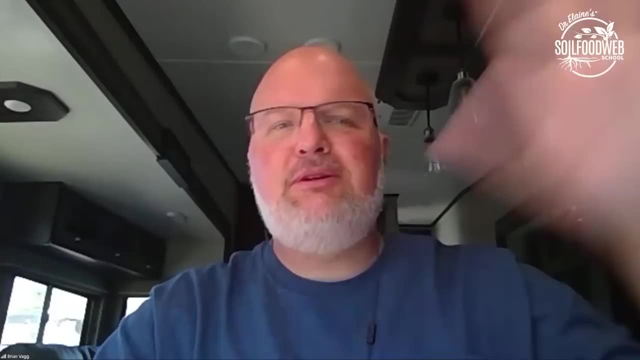 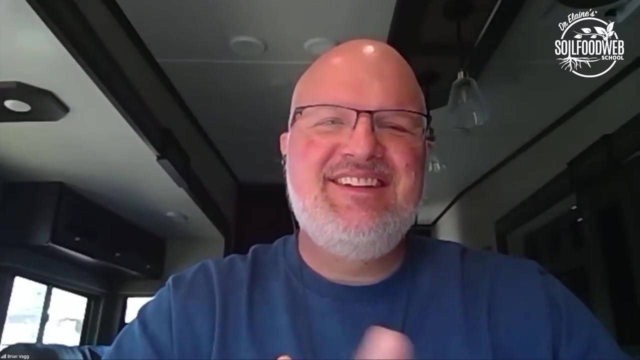 yeah, it's. it's funny because people- oh, weeds, the dreaded weeds, you know what purpose they have. the question always comes out: are mosquitoes? we should just get rid of mosquitoes completely. i don't know what else is behind there. yeah, exactly, i mean, everything has their role in the 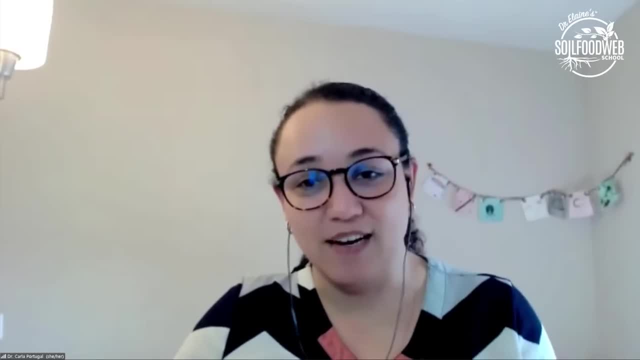 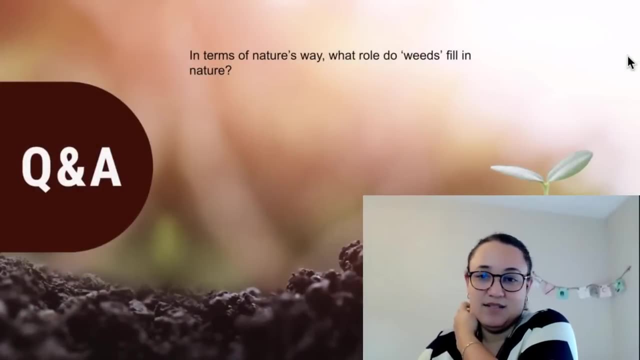 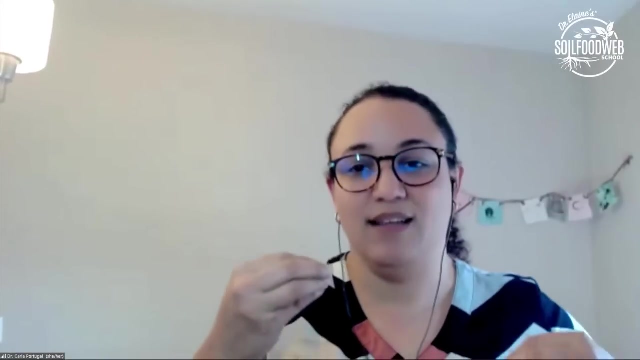 nature. we might not like, we might not understand, but if we take them out we're gonna see the effect of things going sour. so, uh, like elaine said, weeds are pioneers. they are the first one you're going to break down and really initiate this interaction of the food web and the root. 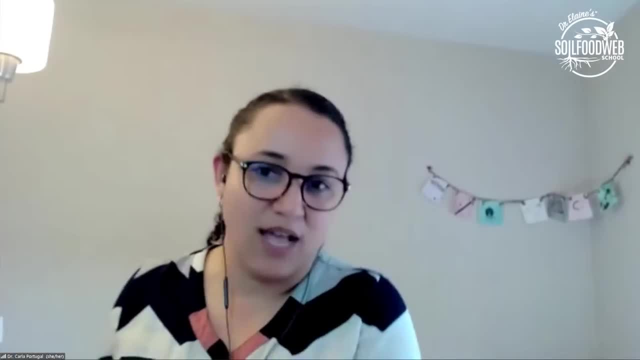 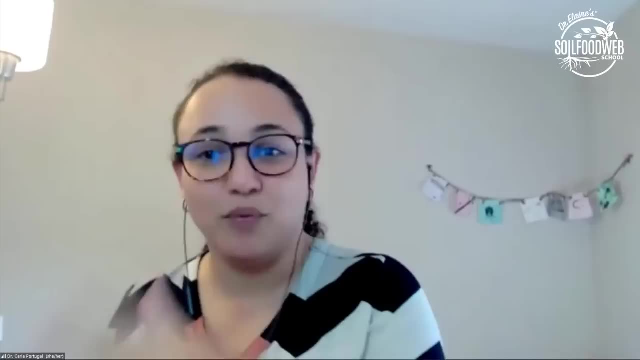 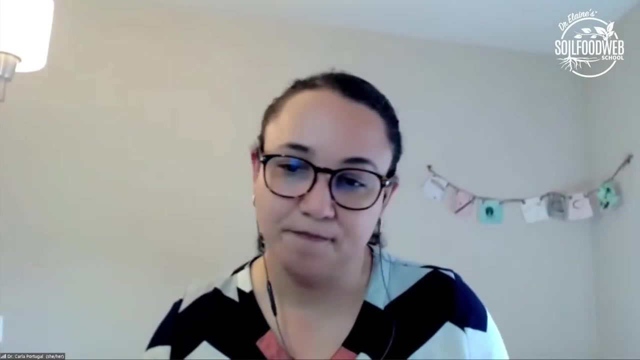 system, then allowing the succession stage to happen. so it's a step by step, like with we when we are babies, we don't learn how to run first, right, we run, we learn how to sit. then we go step by step. so it's the same logic. yeah, you know one thing: exercise like a logical exercise i like to do. 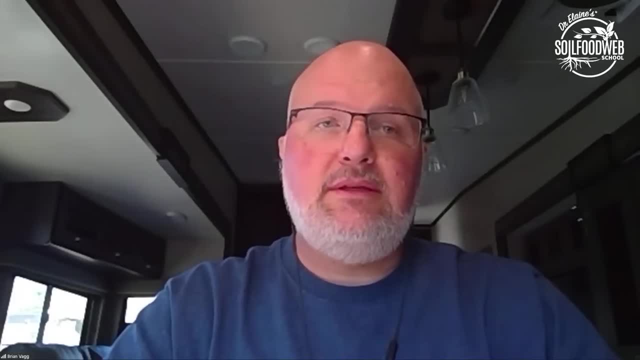 with some of my clients as well, when they're dealing with a lot of weeds, is to tell them about what's the ecological role of weeds, where do they typically fit? and then to describe to them well your fields are essentially in a highly disturbed environment. it's not necessarily where. 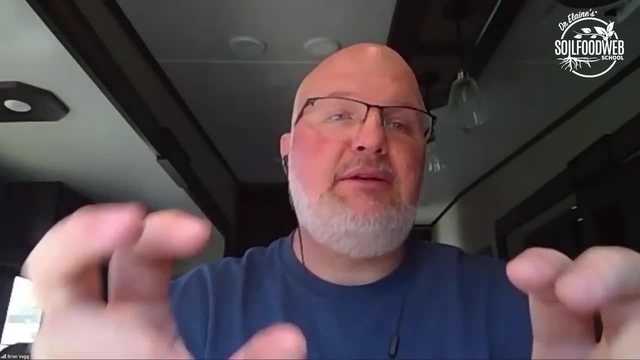 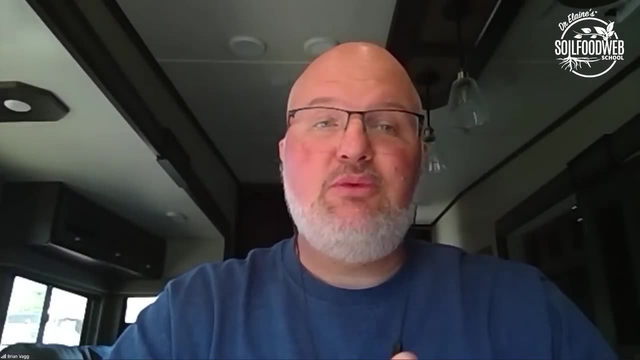 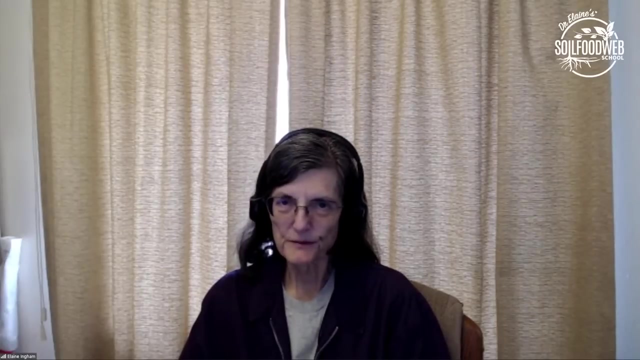 the plants that you want to grow would typically grow in that highly disturbed types of soil. so the weeds are telling you something. uh, they are a very good messenger to you, saying you're not really treating your soil. it's considered to be really highly disturbed environment and you're keeping it disturbed, so no wonder it's not. 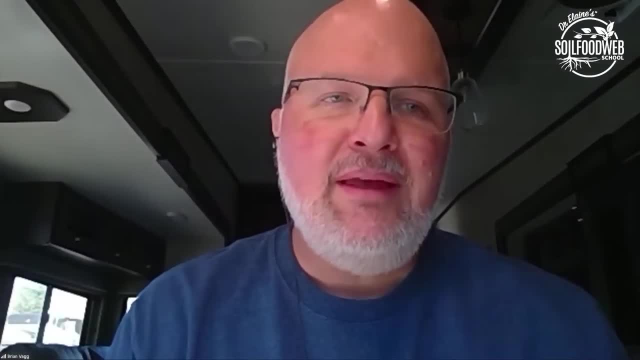 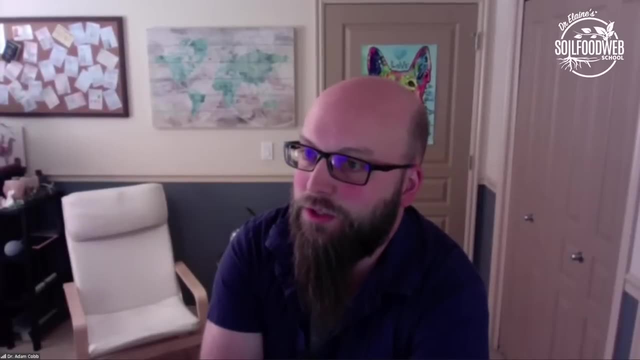 productive, exactly okay. oh, go ahead, adam. i have a friend that i spoke to that said in their native language, which i believe was german, that they don't have the concept of weed like a pest heap, a pesky plant, but rather that it's a showing plant, that it's a telling plant, that it gives. 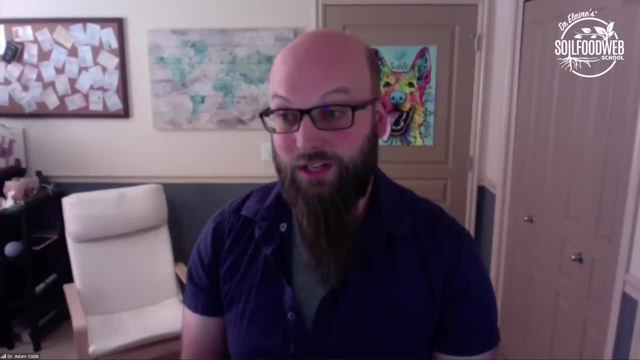 you information about your soil. That's really interesting to me And I think a lot of this indigenous cultural knowledge is on the cusp of being lost around the world in different systems And because of the biases of the scientific worldview, which is great for many things. 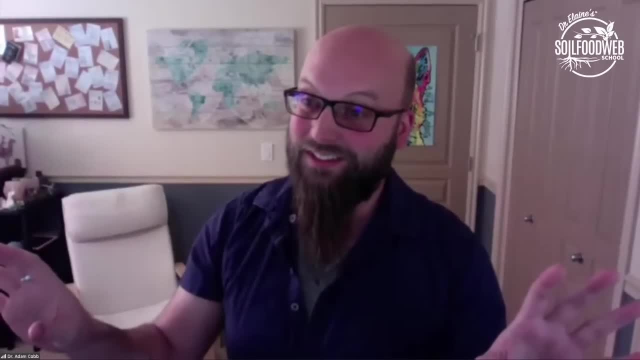 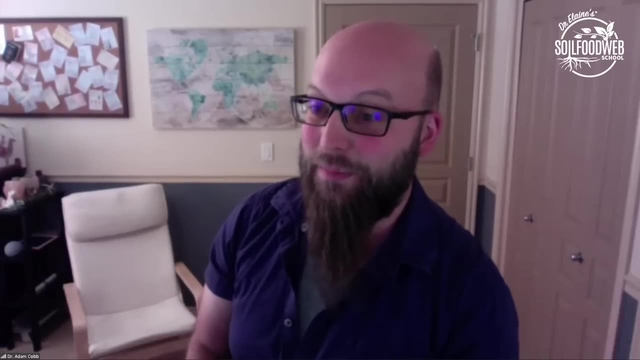 don't get me wrong, but because of the reduction, focus, bias and all that, it's sort of like: well good, what good was that? anyway, It wasn't done through a scientific period paper And I'm like: no, there's deep wisdom, There's deep wisdom. that's there where people have noticed that. 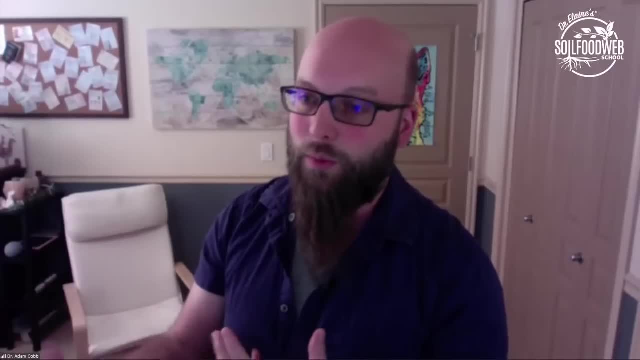 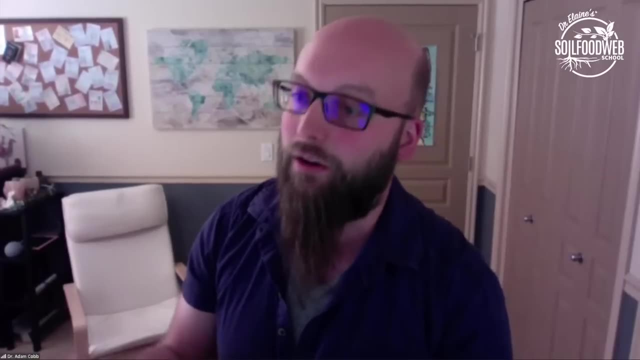 certain plants grow on this soil when we can't get it to grow this crop And you know, it might be that those plants indicate that there's not enough iron in that patch of soil or that it's not bioavailable to plant. 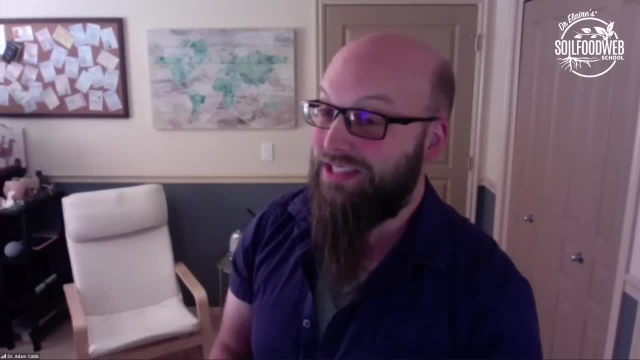 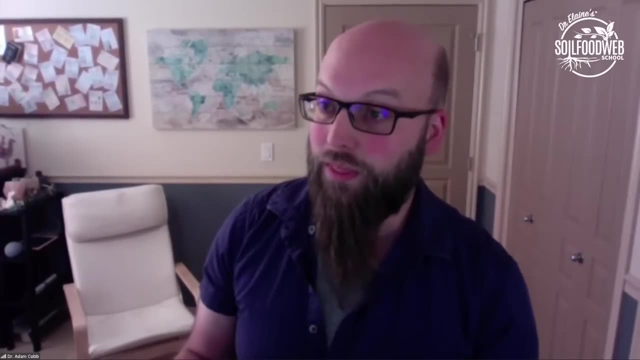 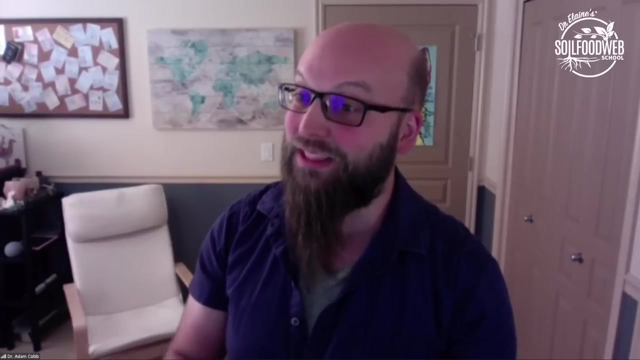 Right is really what we're saying. So weeds have the potential to be more than just an ecological role that they fill, But we can have a relationship with the weedy plants as well. Right now, I get it. we don't want to let the weeds take over and destroy all of our yield capacity in an area. 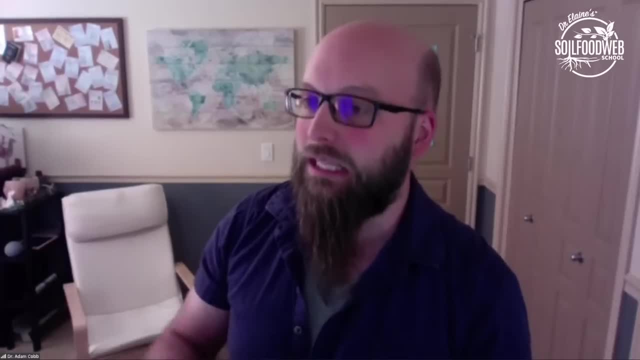 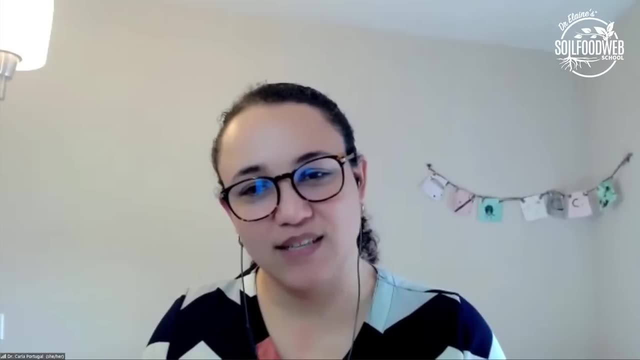 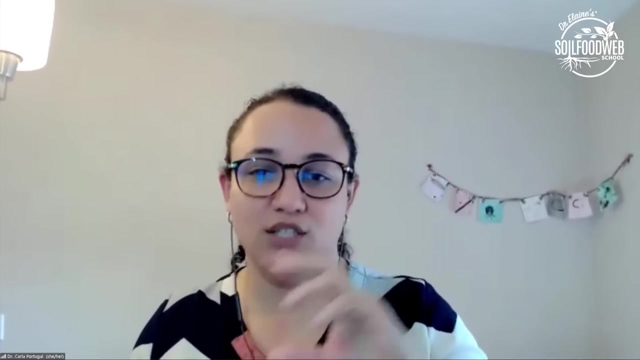 But there's, there's something about bringing these different lenses together To say what is this weed telling me? And I like to see that. I'm happy to see that some universities are already bringing this traditional ecological knowledge as line of research and classes. So I know, Adam, I agree. 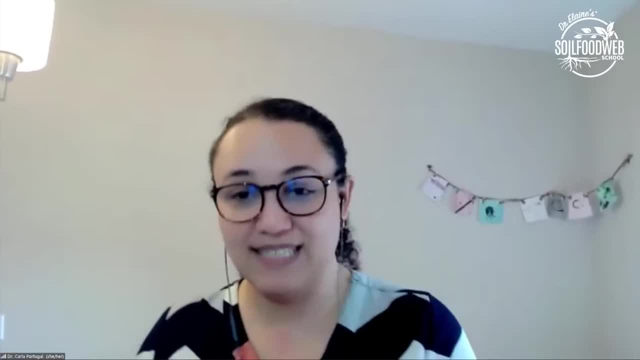 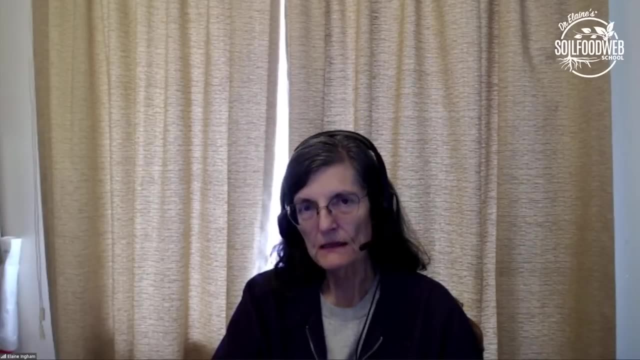 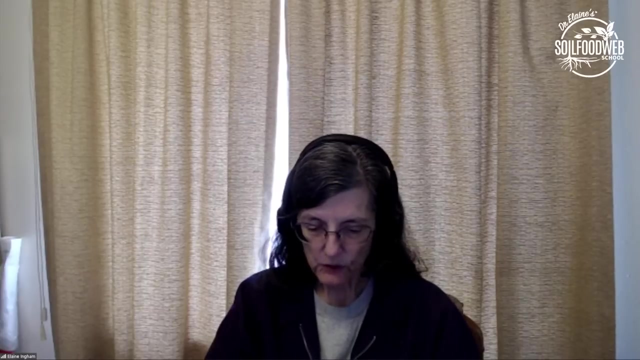 with you. we're far away of the ideal, but finally it's happening. So, but we cannot lose that. I totally agree with you. One of the things we see in the soil food web is that very early in succession, where there's just a lot of weeds that are, you know, very. they're sucking nutrients out, they're sucking water out. they're not putting a lot of organic matter back into the soil, but at least it's better than nothing. Those bacteria aerobic conditions will take the NH4 produced by the bacteria and fungi in the soil being eaten. 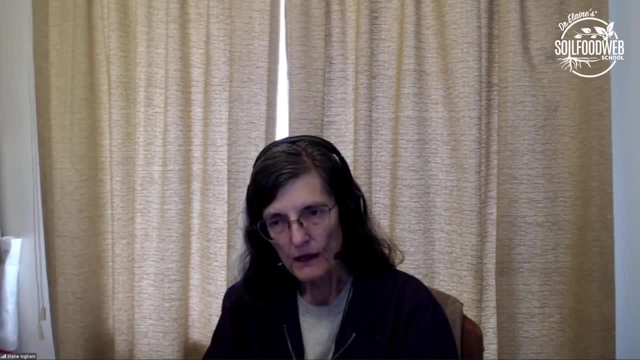 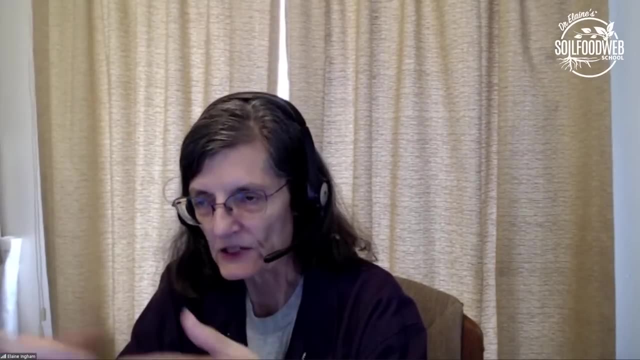 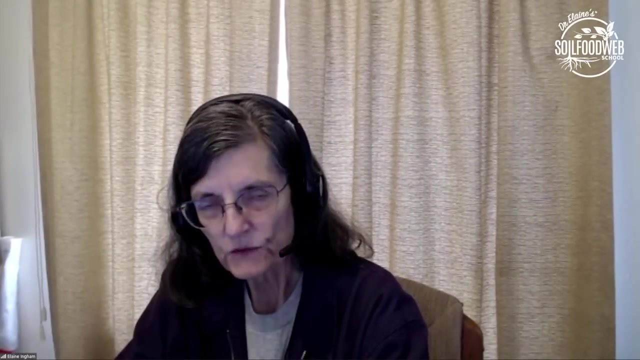 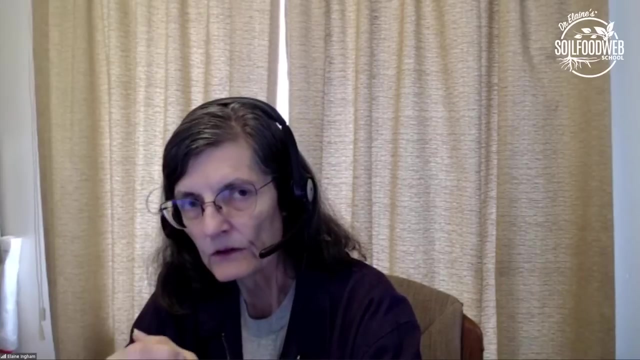 by their predators And those bacteria- the aerobic bacteria, those very early successional individuals, are kinds of species- will convert all of the NH4 into NO3.. Weeds require nitrate, And there's a set of papers out of the University of- I think it's- Tokyo in Japan. 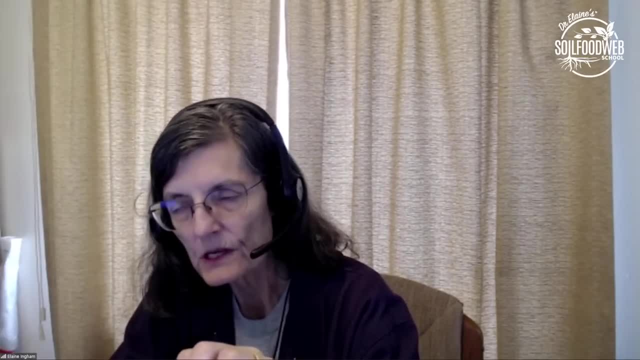 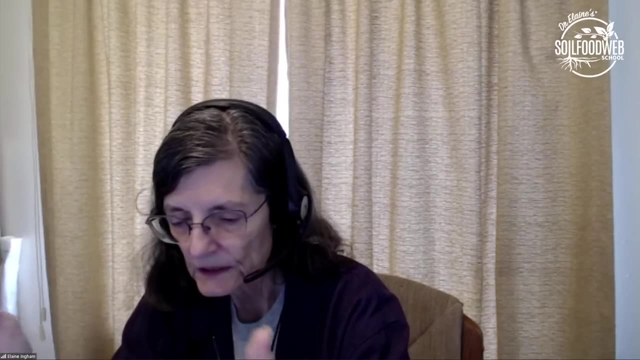 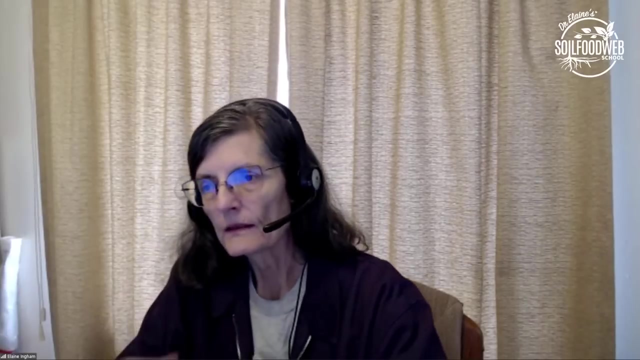 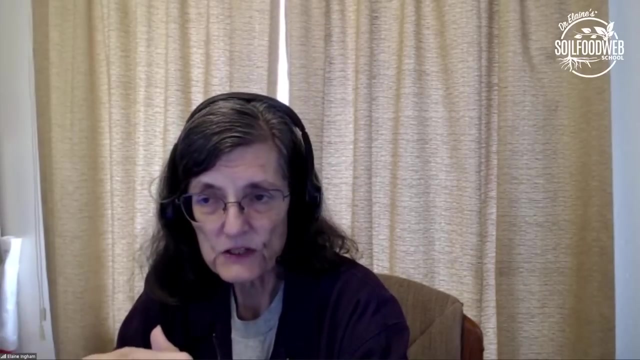 And it's on our reference list. If you take the FC classes, You get the manual with the references and you can access those papers and read them yourself about this ratio of ammonium to nitrate. And so, as the bacteria have to now start sharing a little bit more with the fungi, a little bit more with the fungi because of the cellulose that's been produced by those weeds. And finally the fungi will overcome that limitation, and when the fungi get going they'll drop the pH down to 6.5, so definitely further down that the nitrifying bacteria can tolerate, And so NH4 starts becoming an important component of that soil. that's doing work in the soil. So, as time goes on, the mechanism for why we go from just bacteria present bacteria and plants, early, very early successional plants that require just nitrate, And then finally fungi come in and now they start competing with those bacteria. And so the weedy species die off, because the high level of NH4. In the soil prevents those weeds from being able to compete, because they cannot take up. the weeds can't take up the NH4.. There's certainly a lot more research that needs to be done on this. 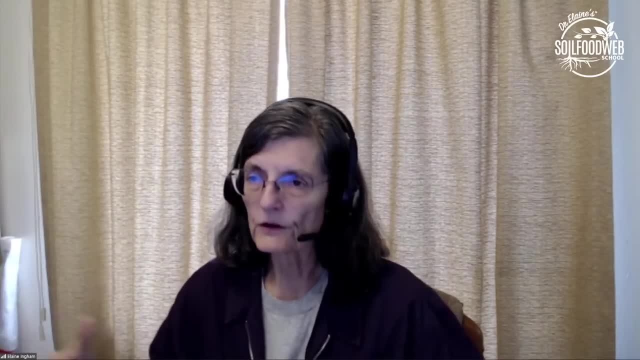 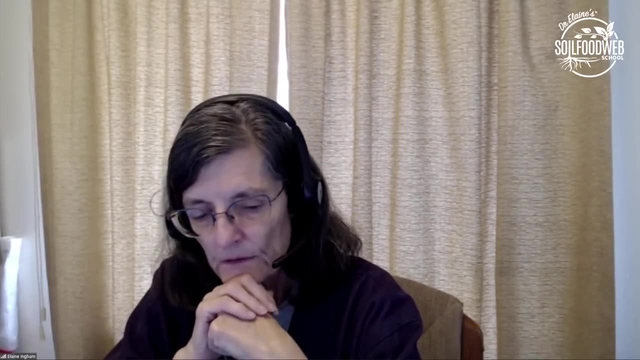 And so you know, those of you want to come and join us and learn all of this with us. And then, coming out the other end, you start doing some of these things. you know, listening to nature, doing the things. And then, coming out the other end, you start doing some of these things. you know, listening to nature, doing the things. 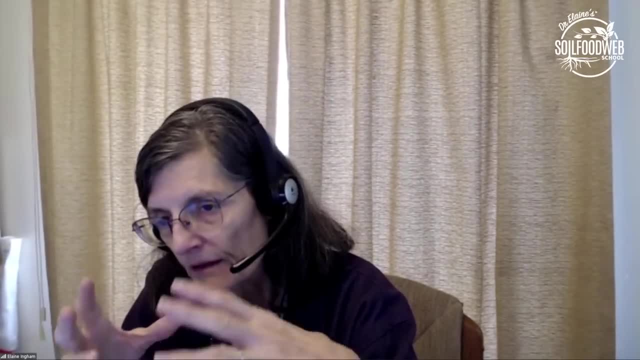 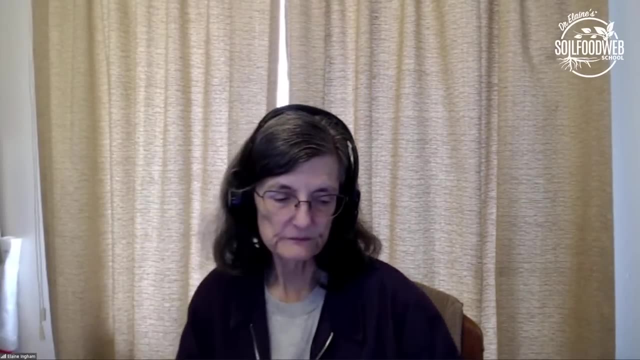 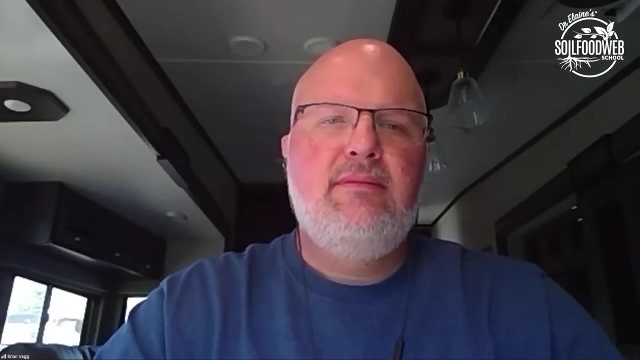 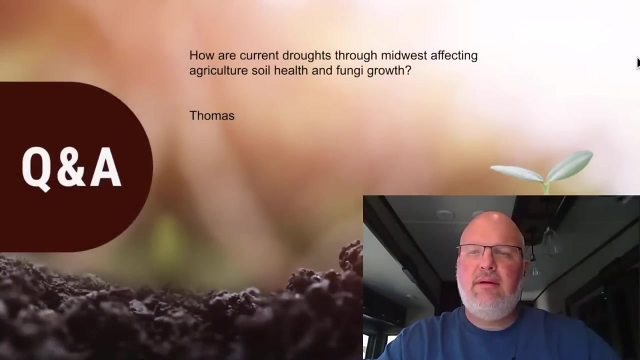 There are things that nature does to prove that working with nature instead of against nature is the proper way to go. Well, certainly, All right, Adam. this is the next question. My internet view bill is slow. Okay, I got it. 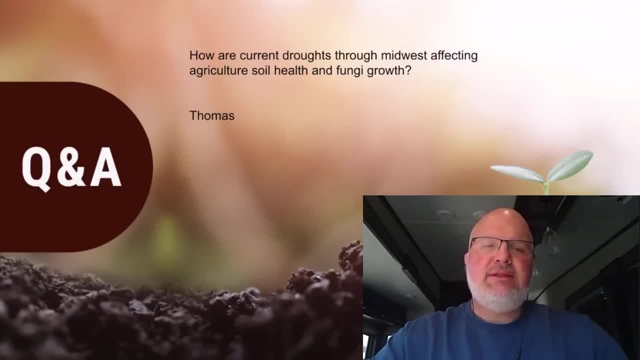 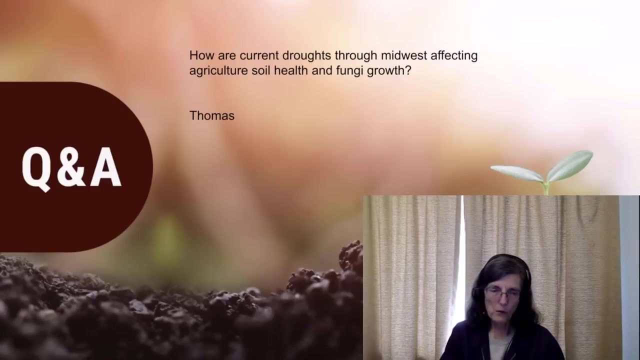 Yeah, Here we go. The question is from Thomas. how are current droughts through the Midwest affecting agricultural soil health and fungi growth? They luckily all have dormant stages that if the lack of moisture is really killing all of the plants and maybe lowered production. so there's not as much food for the bacteria and fungi, protozoan, nematodes et cetera. they're not going to be killed, They're not going to be done away with. They will hang out. Some bacteria and fungi don't have very long-lasting. There we go again. Dormant stages. Thank you, Dormant stages. I think I haven't had enough sleep. So those dormant stages. But as soon as the water Comes back, or as soon as you start putting the compost teas back out, the X dates going into the soil. those guys wake up and start doing the proper things to rebuild soil structure, to hold water in the structure of the soil. So we really need to do that. You go back in history and you look at some of the data about water And how much rainfall they've had. And we're calling these terrible droughts When a hundred years ago there, it wasn't a drought. If you got that really low amount of rainfall, that's not a drought Back then. Why is it a drought now? Because we've destroyed the structure in our soils. 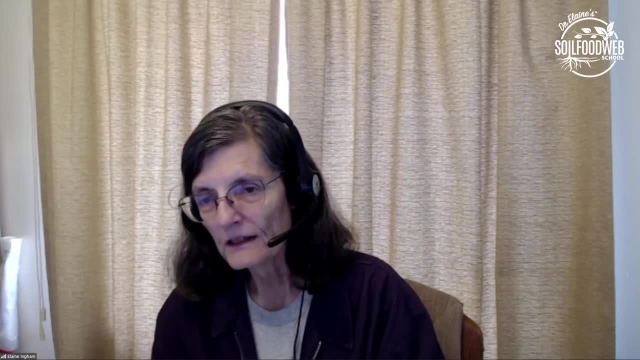 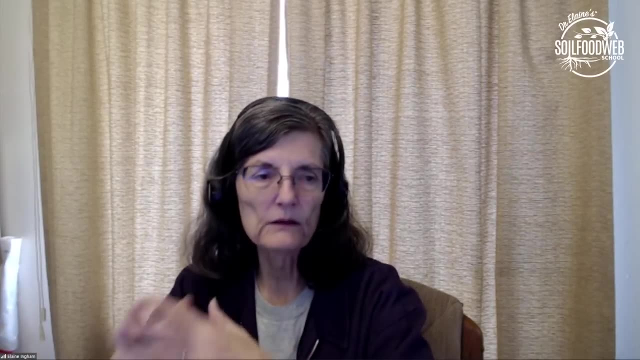 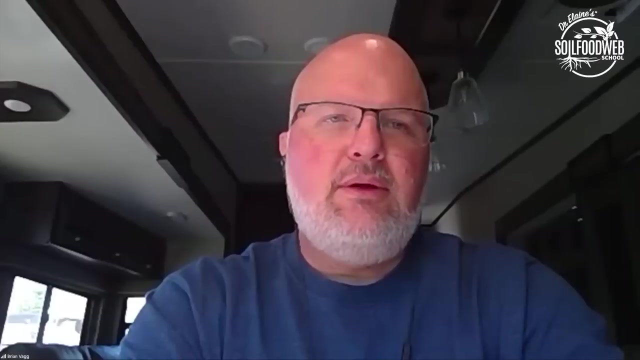 We aren't farming on soil, We're farming on dirt, And so this huge difference between then and now- And it just goes hand in hand with all of the other problems We've done this to ourselves- Get the fungi back there. For me, you know it's- there's a resiliency aspect to the work that we do. 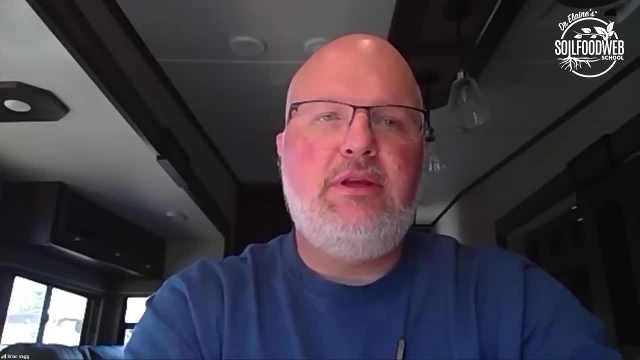 You know one of the things that we are. you know we're always trying to help our farmers with this. How do we reduce their input costs and, and you know, make them more productive and all the other kinds of things? 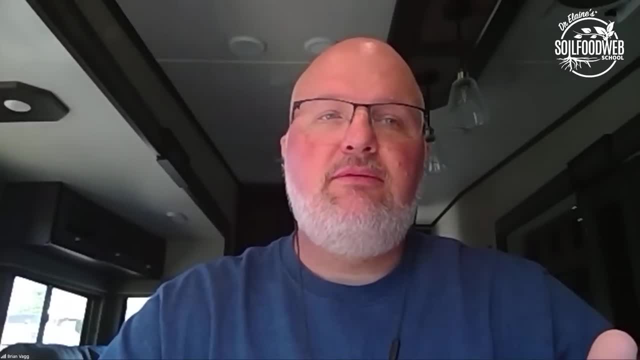 But I also think one of the really true benefits of- You know, of Establishment a good soil, food web and a functioning ecosystem is the resiliency. You know the bookends of issues where you have too little water or too much water. those 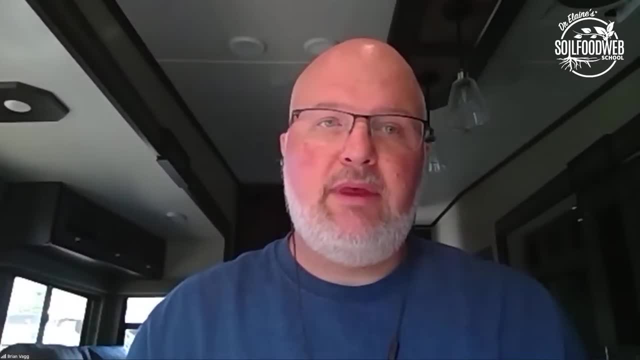 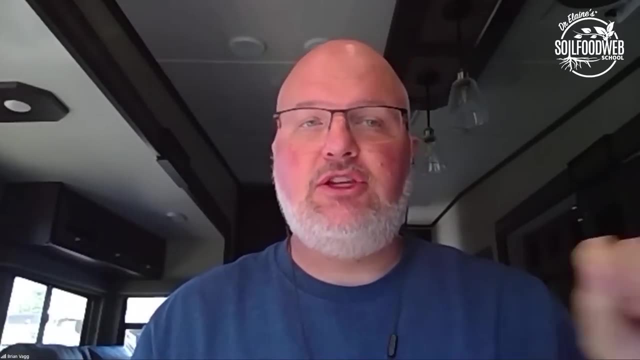 soils have the ability to either too much water, absorb that water, don't cause erosion and have all the runoff, Too little water. well, we're holding onto that water for a much longer period of time frame from that dirt, from that soil that has no structure. 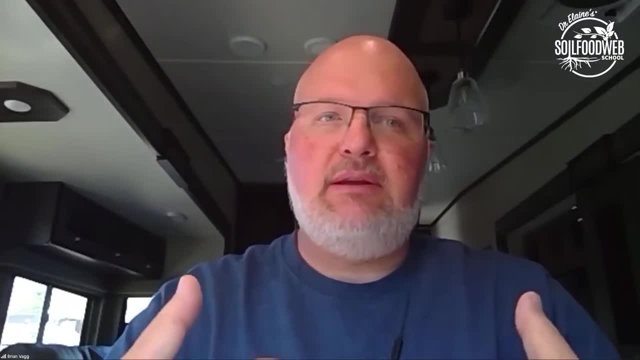 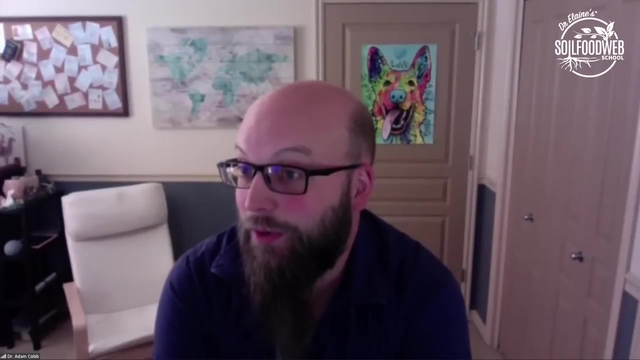 And so the farmers themselves have a resiliency battery kind of built into their operation, which is really really huge. All right, panelists, anything else you guys want to add, I think it's been really well covered. And you know, one of the things in the promo is DD. 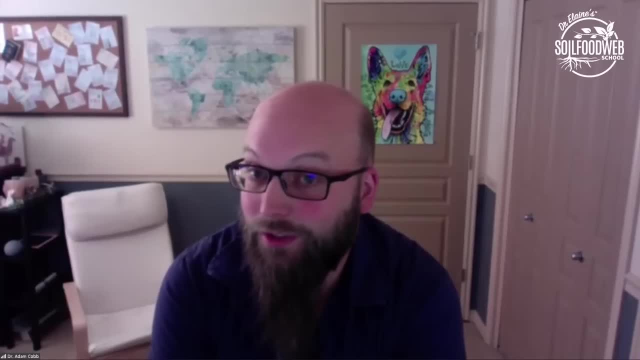 Pursehouse's Soil Sponge Workshop, which I recently took and found to be amazing, which really goes into this whole link between soil health, the microorganisms which she calls the essential workforce of the biosphere, and the way that they can create you know. 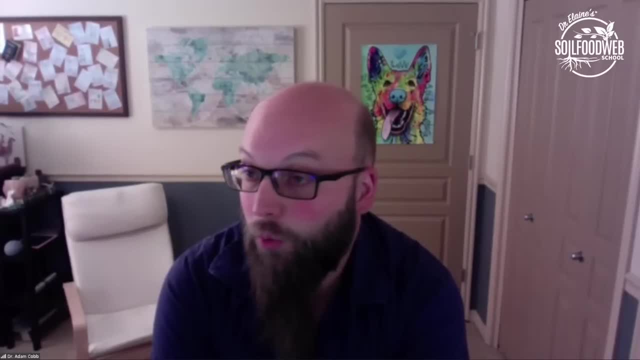 create soil which is capable of holding, absorbing and holding deep pools of water, And Elaine talks a lot about. when you have soil which is truly soil, nice and fluffy, with good structure, the roots can go hundreds of feet deep. on some of these trees, 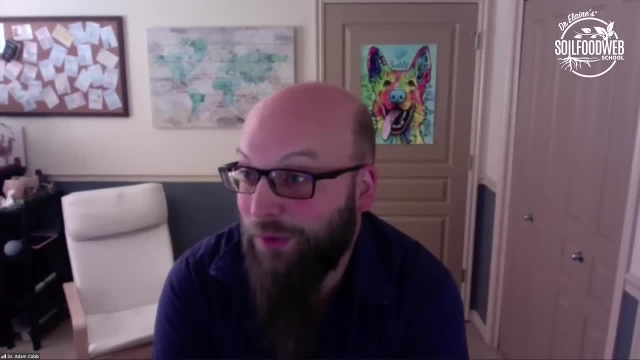 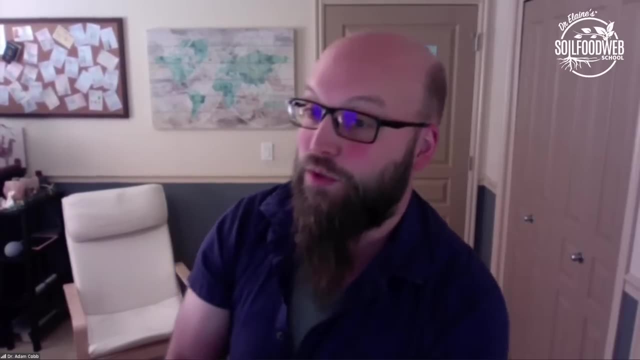 And then you're talking about it. you know what's rain for 100 years to something like that that can go down there and get water from that deep Soil layer. All right, All right, let's move to the next question. 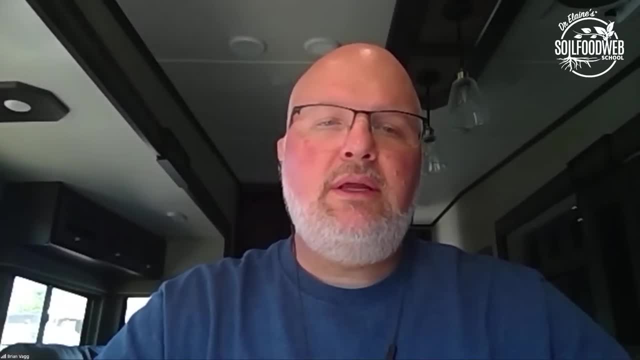 This question is from Nicola and the question is regarding killing off fungi due to tilling and chemicals. would there not be fungal spores in the damaged soil that would regenerate when conditions are more favorable, rather than having to make their way back from afar? 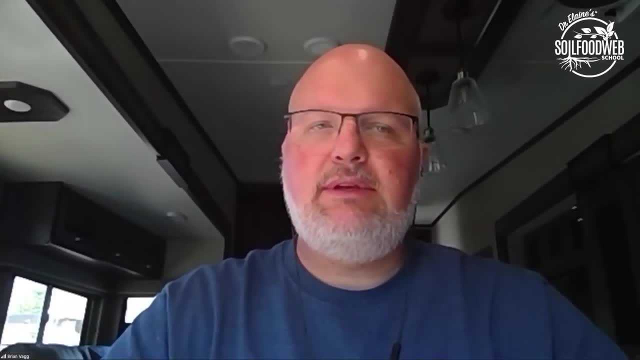 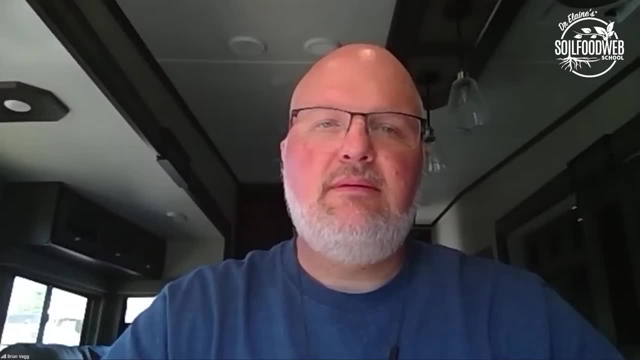 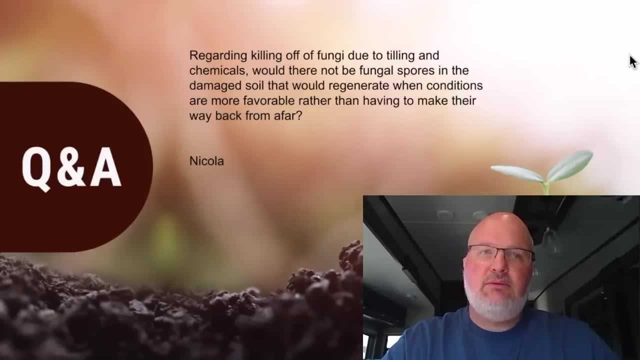 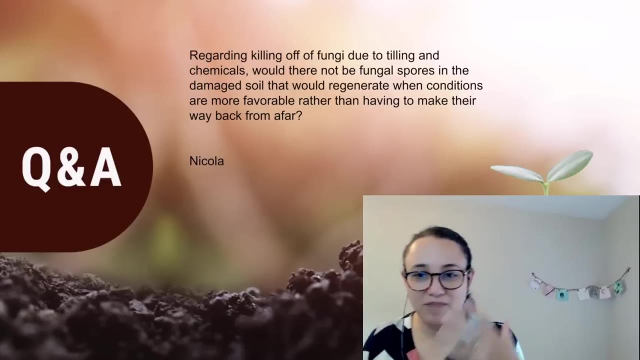 It will take a while for those species to recolonize and restart, to build that structure, And it just takes a while if we're not intensively trying to manipulate that. Okay, Yeah, again, it's go back to the depends. how deep was the damage? how much of this? 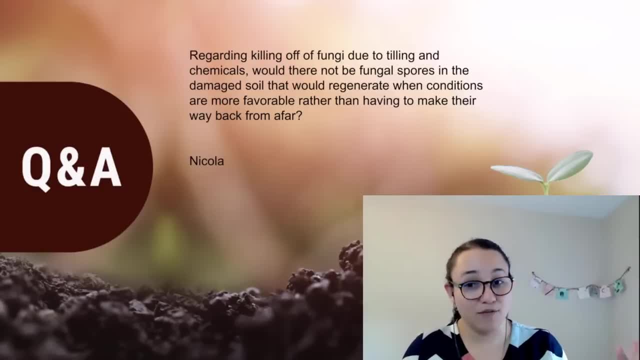 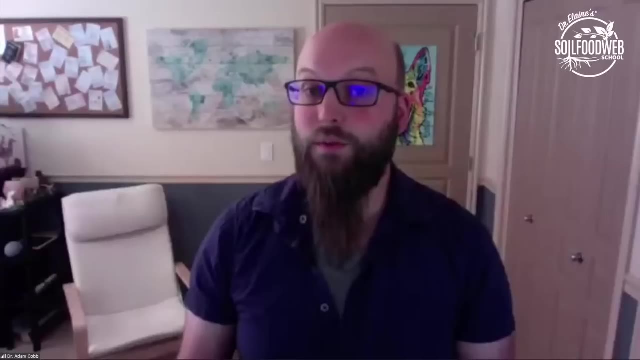 fungi biology was lost. how much of spores do you have there and when reached the perfect condition? So it's again: observe and reassess your actions constantly, And often we're not talking about a single disturbance event which you know. I don't. know what the spores might be able to, you know, recover from, but an annual disturbance event, or two or three times a year with something like this. And so if you, if you have spores, a population of spores in soil, they keep waking up and connecting to, say, corn, but then getting chopped up again after the corn is harvested. How long does it take before you have depleted that spore population? because the organisms aren't able to recreate To reproduce right. It takes a while for the fungi themselves to have the resources to establish themselves. 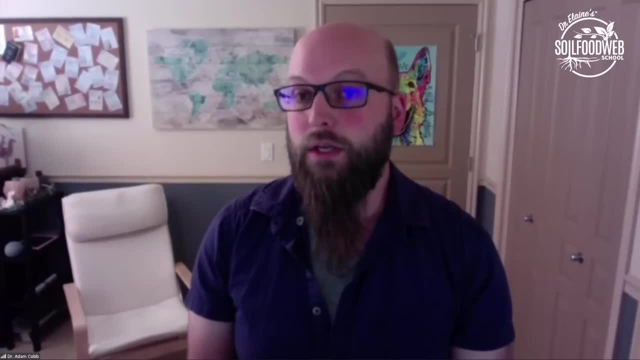 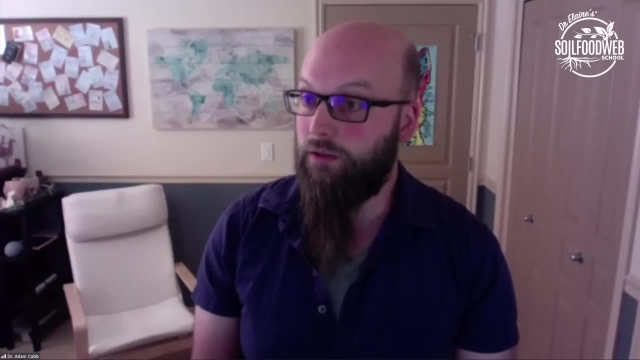 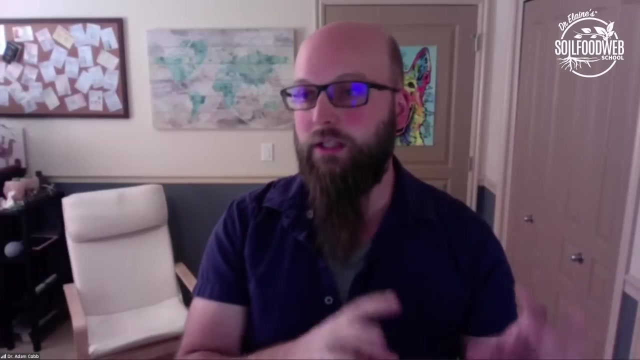 and to really be in a reproductive phase. So in Eastern Zambia I did some research among different farming styles, even things like agroforestry and conservation agriculture- but those have been taught to these villagers relatively recently- And the historic damage from tillage and fallow and fertilization. I went in and assessed. 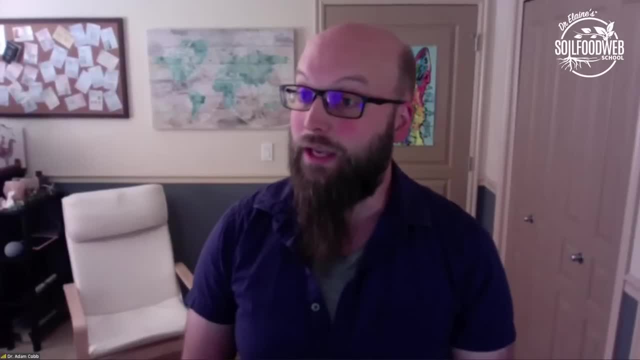 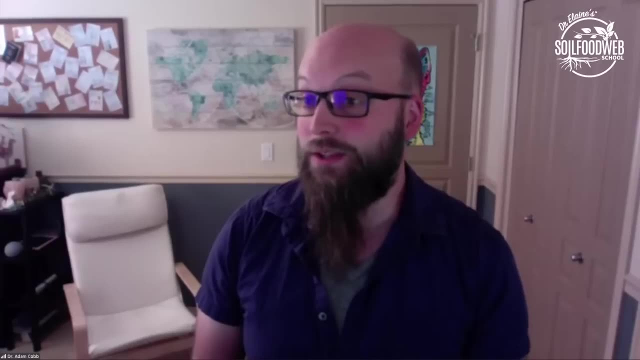 the fungal biomass, comparing it to like a local nearby grassland, It was still half the level of biomass And there's a good chance that the species in there had also shifted. It was less diverse And so, and that's, that's one of the papers. I'm sorry I don't have access to my Google. 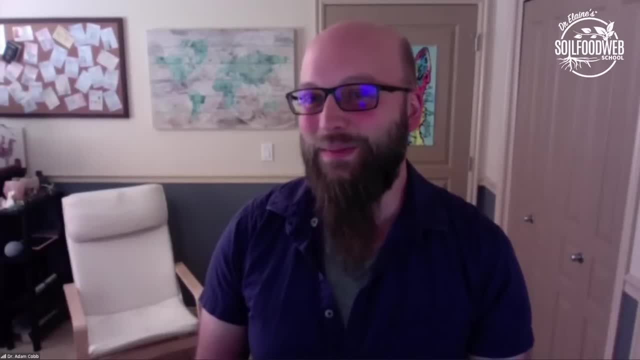 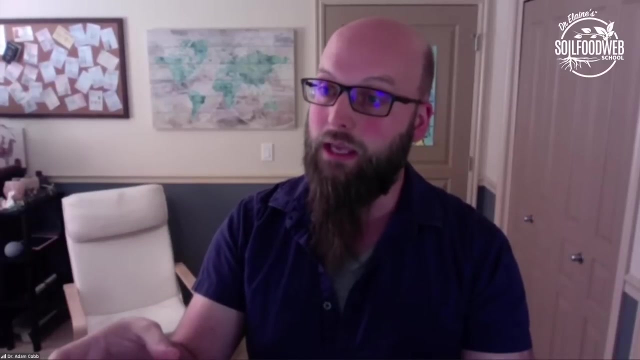 profile. I'll link that somebody asked for because I can't leave the screen just yet. But one of my papers was in Zambia and it and it showed that that there was deep damage from historically that even when they started farming in a better way, the soils had not. 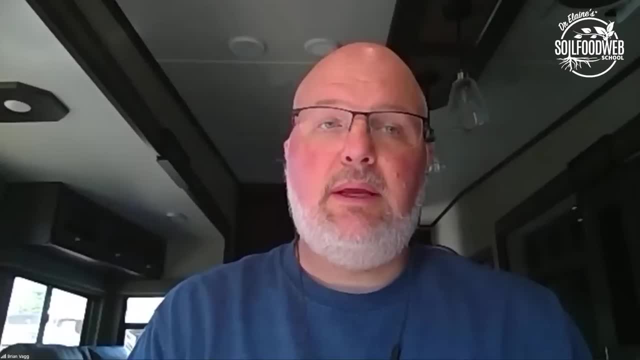 recovered yet. Yeah, I mean I deal with a lot of agricultural systems that are severely damaged. I mean this is multi-generational potentially. Yeah, I mean there's this one in a small country where they've been tilling adding chemicals. 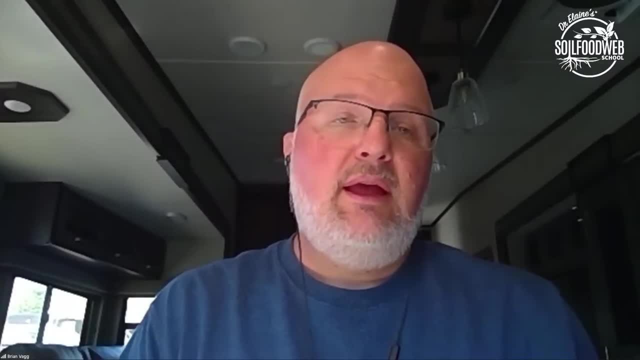 both fertilizers and herbicides and sterilants and so forth, And you get. you look at it, soil. I mean there is no structure. organic matter is down in the 0.2, 0.3% organic matter in the soil. 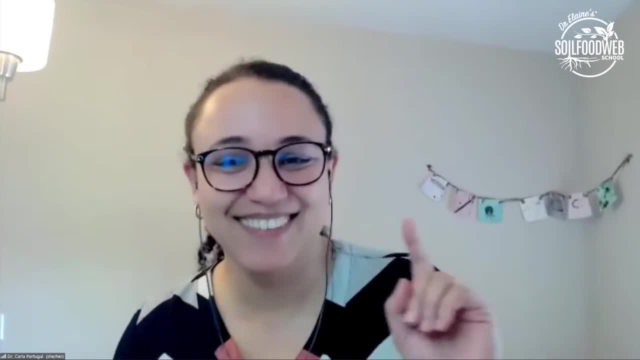 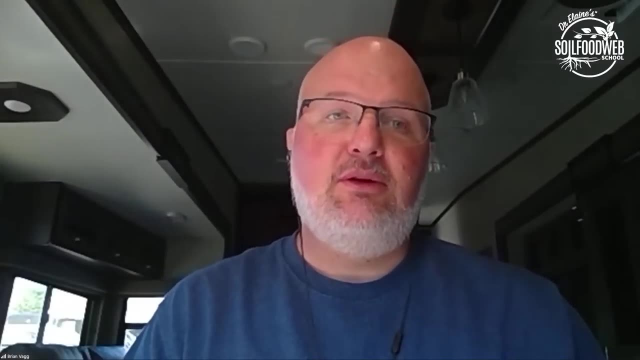 Should we call that dirt and not soil? Exactly, Really, It is dirt And there's just. it's not a favorable condition for the organisms that we want to to live, you know, to thrive in that system. It's not very favorable for them. 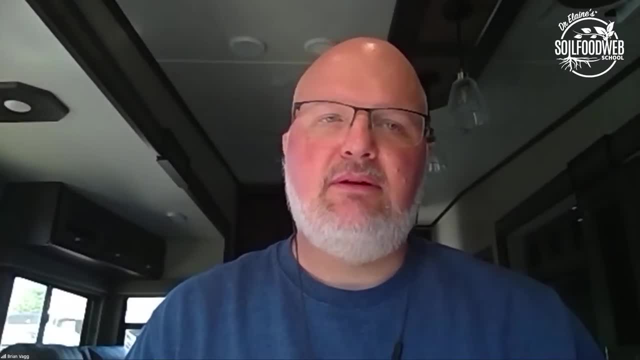 know we're trying our best to to get them back in there. have them start building some structure. do the things we can do, you know, like the breaking up soil compaction by mechanical means, if we can, to help push it along, to become more favorable for the biology, to establish and, and for me, you. 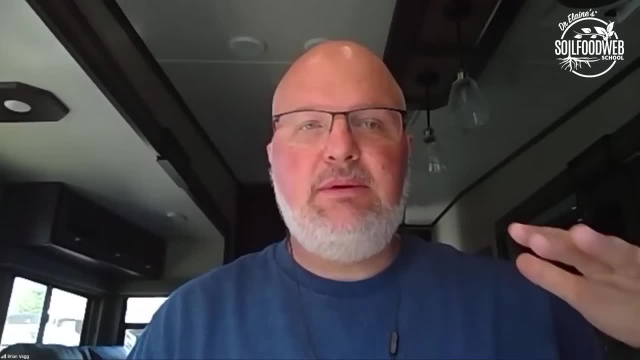 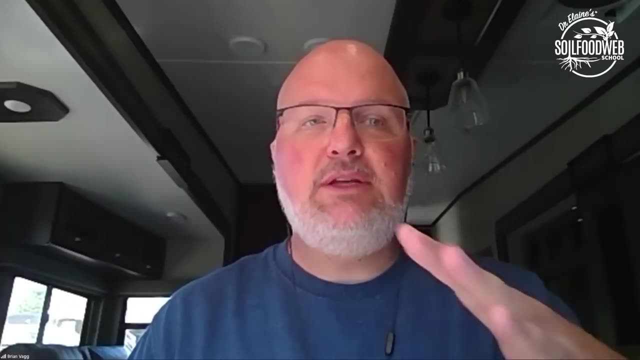 know, when i look at soils, when they're really, really degraded, it's a little bit of a slow start. but once we start, you know, intensively managing it and really changing those practices, it's a little bit exponential curve. you know they start to build more structure, and when, more structure. 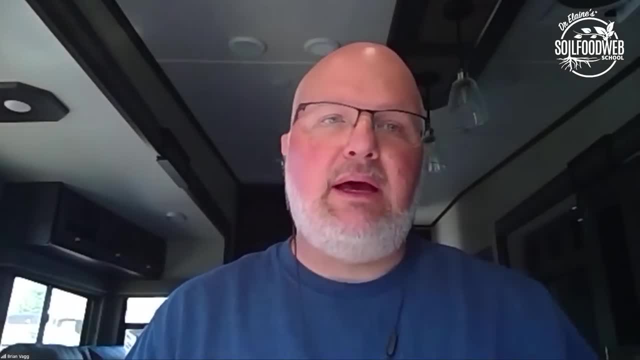 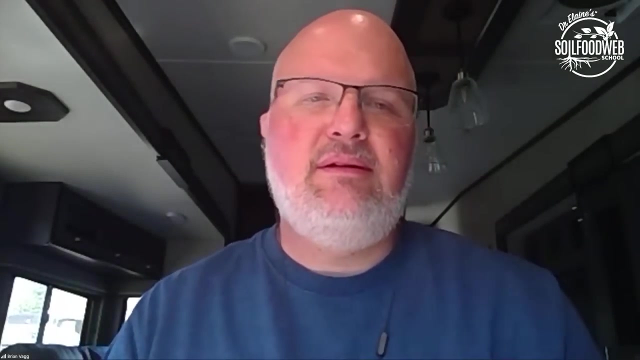 gets built, more organisms are able to to survive and then the biology starts to take off, and that's that's what we're really trying to hope to see. all right panels. anything else you guys want to add? okay, let's move to the next question. oh, wait a second. i think i had some more questions in there. 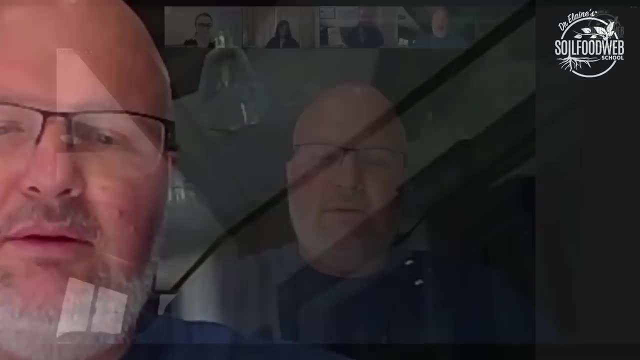 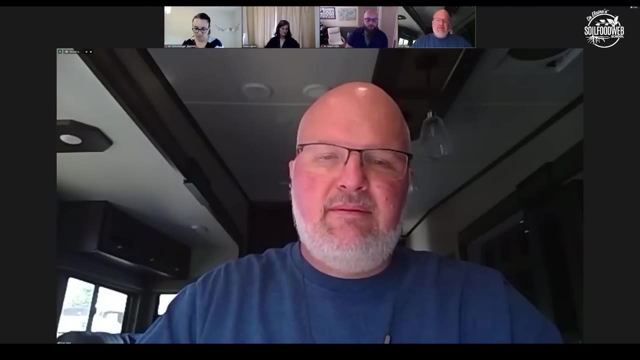 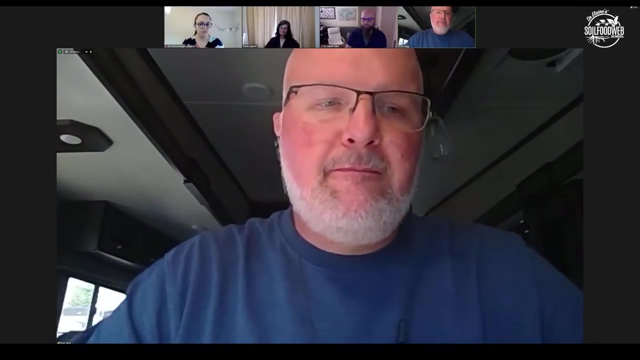 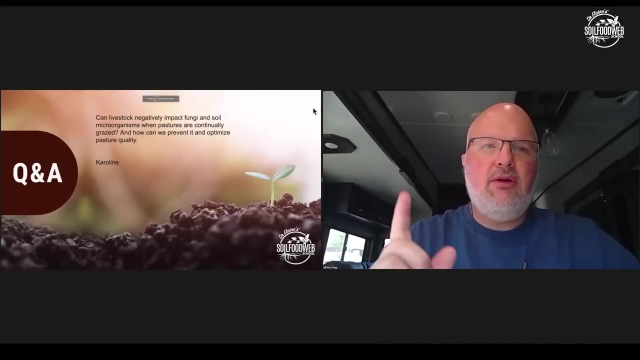 um, yeah, we go ahead and refresh there, adam. i think there may be a few more. that got added. all right, i think you can go back up. uh, i think there's a few more just previous to that. oh, maybe not, okay, so let's go to that one from from caroline. um, the question is, can? 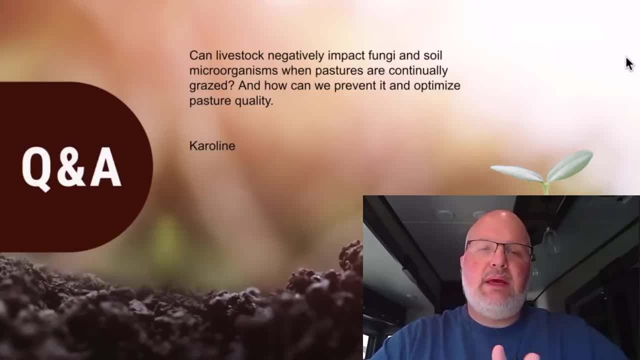 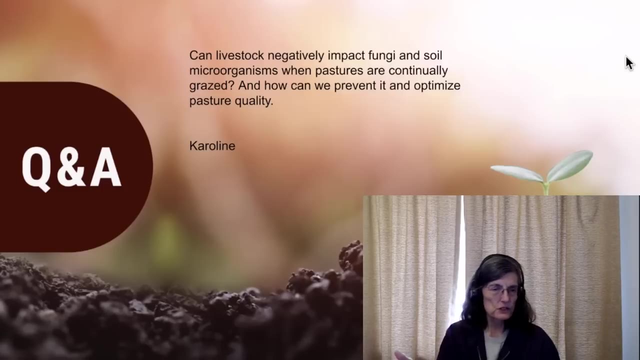 line stock negatively impact fungi and soil microorganisms when pastures are continually grazed. and how can we prevent it and optimize pasture quality? definitely, the livestock are going to negatively impact the fungi and other soil organisms through compaction, mainly when pastures are continually grazed. that's a problem because you don't get the flow back into. 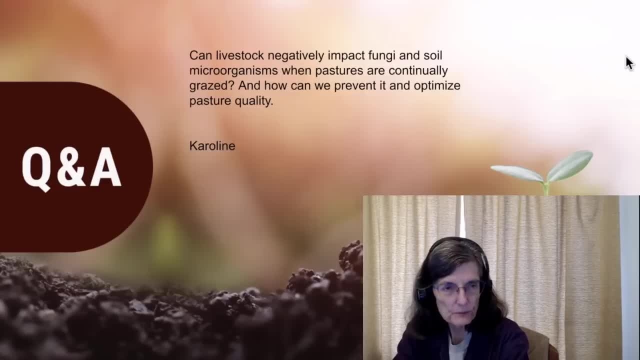 the soil, that would have been possible and the the grassland wasn't heavily grazed and that's why, uh, you know, having the rotations of the livestock on the on the um farm is a really good idea and you want to see that the plants have recovered back to some level where you know that they can. uh, those plants can tolerate that. 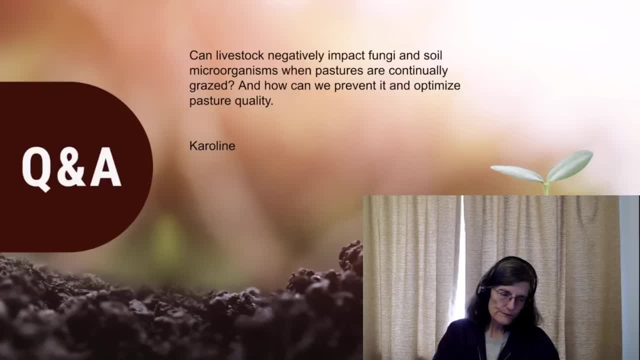 disturbance of being grazed once again. so um compaction, that's the biggest problem there, and if you've got continually grazed pastures, how do you get out there and apply the biology we do have? um, we've done some work in australia, quite a fair. 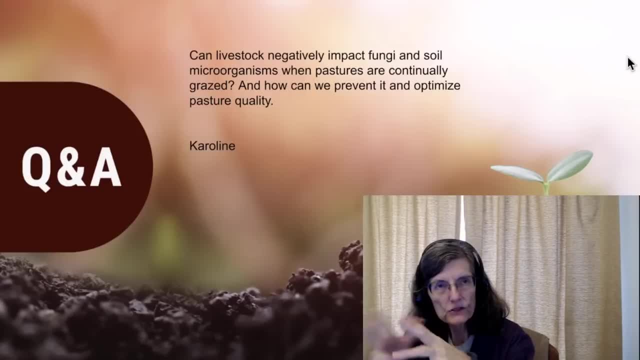 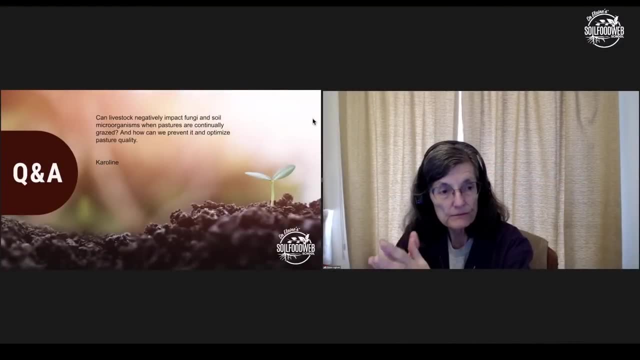 amount of work in australia, where we actually dropped bales of hay that we had soaked in compost tea, and so when the animals came over to eat the con, the um plant material that was dropped in their field, all of their hooves got covered with this. really, 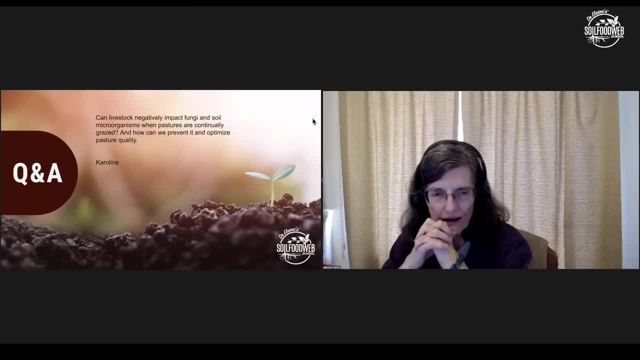 good biology up to the knee. um, they got covered in this really good biology. and of course, their mouths and um, cows are not, um, very, um, tidy eaters. they, they spread it far and wide and we could see that over time, the kind of the circle that where we dropped the 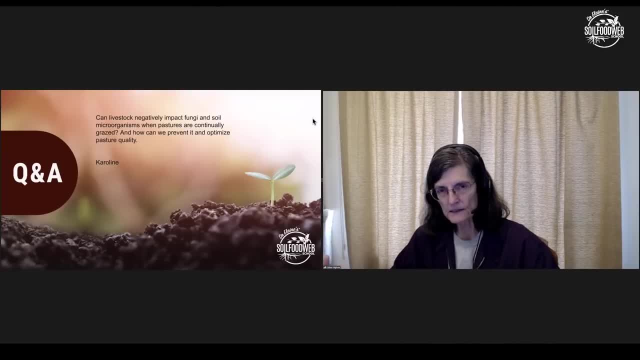 rapes on over the meant to go. nasıl w dry practice was in might work in a short interval, like when the mixed vegetables were blown away at night, for example. Murphy, why would we need to go upokay, so rich and healthy and flaky? it was a matter of sort of a. 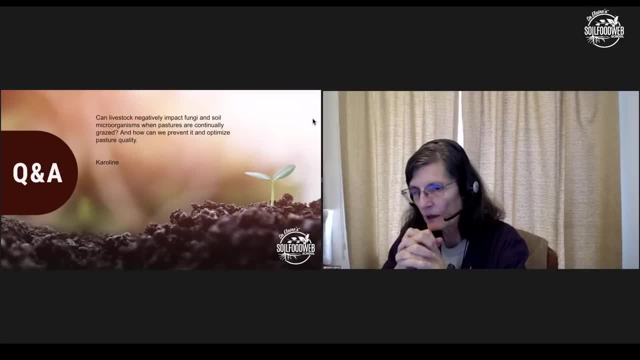 down-ici sort of sort of action um process that led them to we're looking for return. and then we took a. they spread that biology and we could show where all of those trails that the animals were following were in that pasture, so clearly lacking a whole set of those microorganisms in their 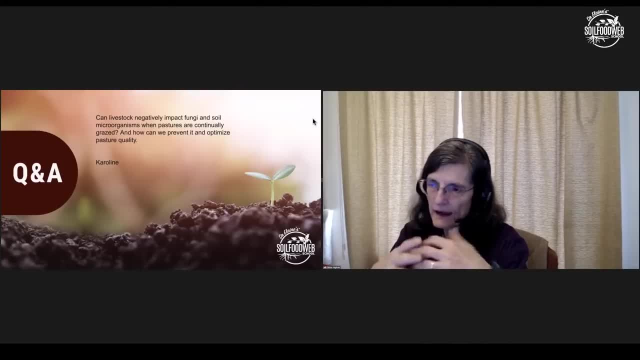 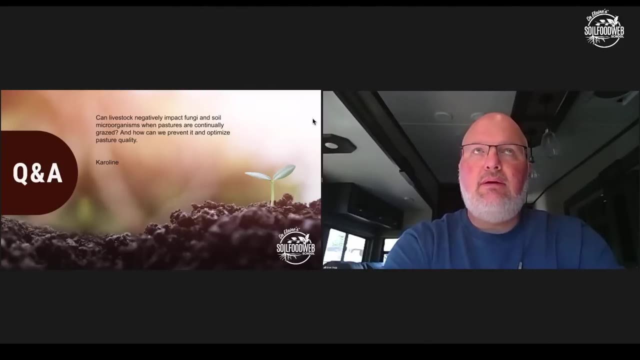 pasture systems and the only way to get back that kind of um, that kind of growth response was to get the organisms back into the soil. yeah, for me- you know i look at pasture land- and just in any agricultural system is you need to really review your management practices and- and as elaine was mentioning, your grazing practices are. 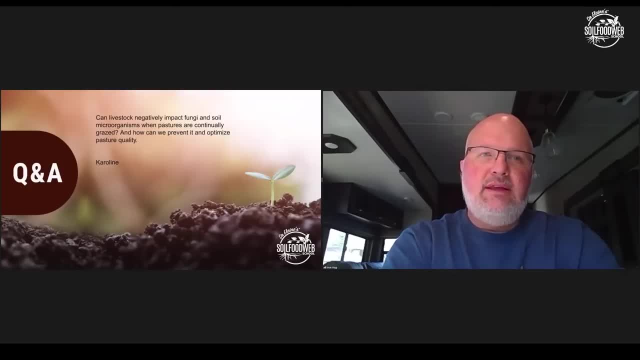 huge determinant as far as the health of that particular pasture. they're going to have in stocking densities too, making sure that you're not running too many animals on a land that can't support that. um, you know, i know, adam and i, we. we did a, i did a talk at a local grazing group and we went out and 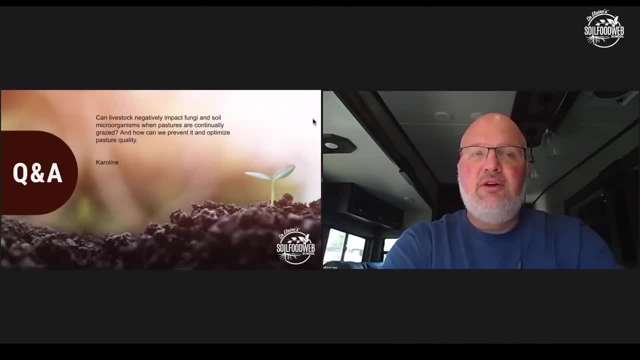 walked some of these pasture lands and they were fabulous. their management practices were really good as far as how they were moving their animals about in that system and you could just tell the diversity of grasses and forbs and all the plants that were growing in that system and the amount. 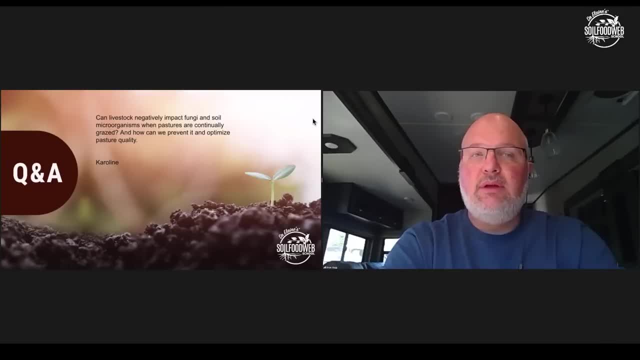 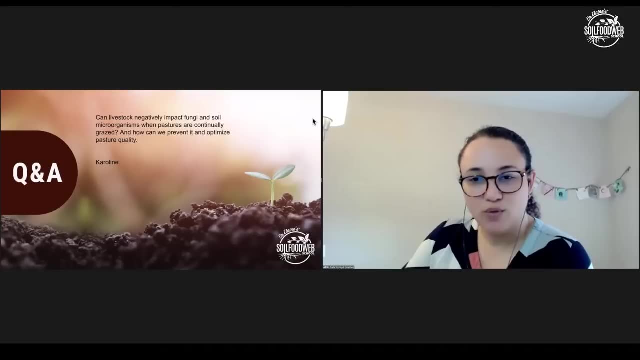 of growth response was was tremendous and that really, i think, spoke to the management practices that that particular rancher had. yeah, one of our recent consultant graduated my student, kevin kraus. his final project was exactly that: he combined the soil food web approach plus management and rotation on grazing the areas. 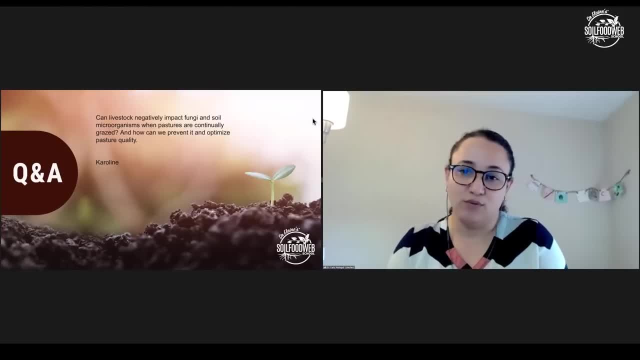 and the results are impressive. so if you want to get a hold of him as well, he's on our website, so don't feel shy to chime in and message him. sure, we need to get all of his data and put it into the. you know the case study and the 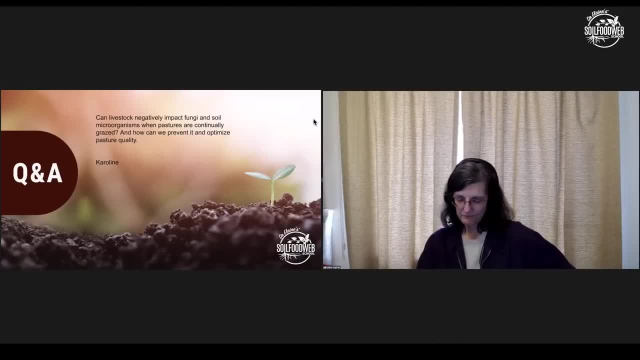 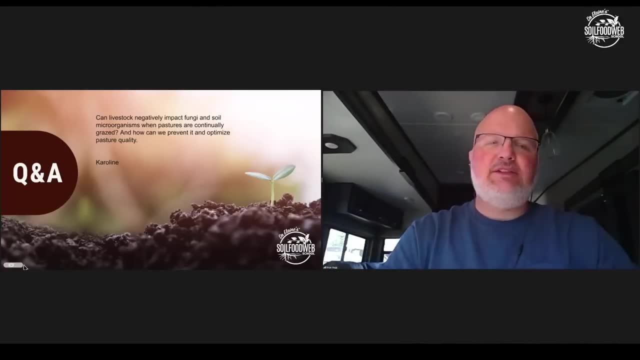 s? well, if it is, the methodology will go over it, but as far as sava pense, the answer is absolutely right, absolutely yes, so that what you're trying to do actually is. we have this one question here, that is, use alol, which i think it's an obvious one. 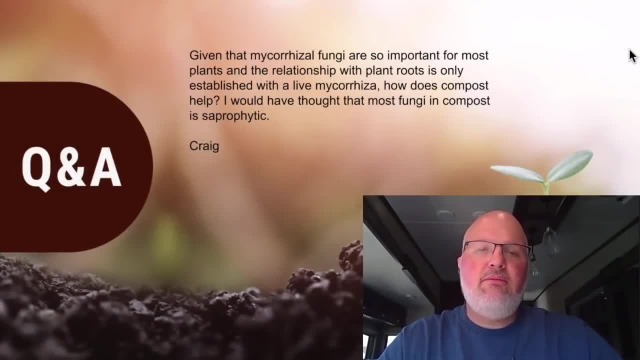 um, do you want to throw something at this? i would like some feedback on this. first, i would like to ask you a couple of questions. i'm not sure of what the problem is with our asking for cork vienen. i would like to'd you know the fact that products like this are in Grandpa's groves. do you think it's going to help? but we're not going to talk about all of this to the final talk. i would like to know some things at the context of the question that we're going to talk about. this question based on that great, perfect. I would have thought that most fungi in compost is saparitic. Craig is exactly correct. Mycorrhizal fungi are not going to arbuscular. mycorrhizal fungi are not going to be reproducing in a compost pile, because they need a living root Now. 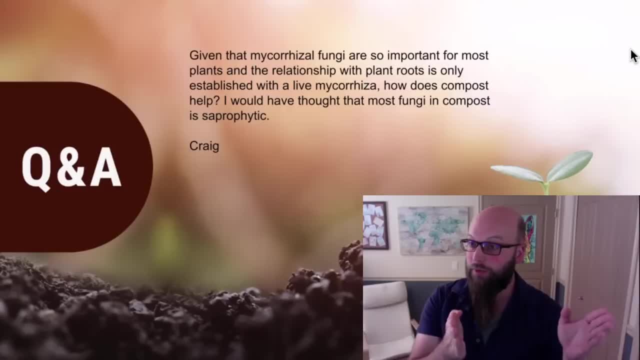 the word mycorrhizal means the relationship between fungi and plants. There are saprophytic fungi that form mycorrhizal relationships. A very famous one is the Amanita muscaria mushroom, That's the red one with the white spots. that connects to birch trees and a few other hosts. I believe. But it's a basidiomycete and most arbuscular mycorrhizae are in the phylum glomeromycota. They have a different lifestyle. They cannot get food without a host that they're connected to, So 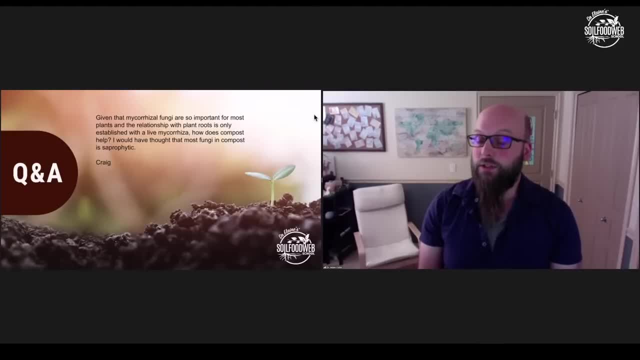 when we're talking about arbuscular mycorrhizae. there are some different methods that have been explored, especially by the Rodale Institute- is one that I like to help propagate: those with living plants in a special area on a farm, so that then you could spread those as well. 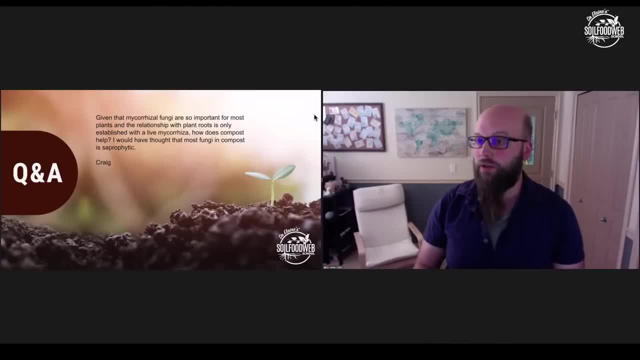 or potentially add them to compost tea prior to using it, But probably the most effective thing would be to spread them to compost tea. But probably the most effective thing would be to spread them to compost tea prior to using it, But probably the most effective thing would be. if you could somehow get it on living plants prior to transplant in terms of the mycorrhizae really surviving and thriving, which is something that we did in my lab at Oklahoma State. Oh gosh, we did thousands of nurse plants with just a little bit of whole soil inoculum. so that they would become colonized, and then we transplanted them out and it was very effective. They spread the mycorrhizae very quickly that way. But yeah, keep your eyes peeled for the second part of a blog that I'm writing on mycorrhizal fungi. 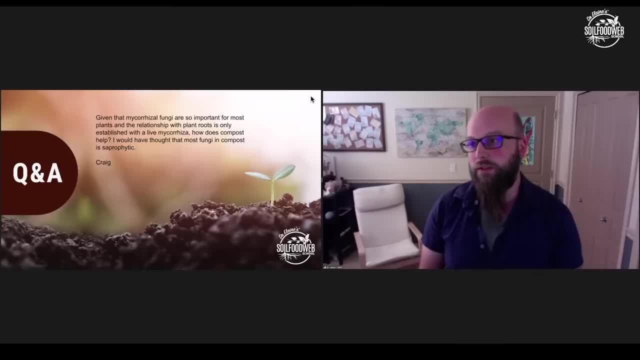 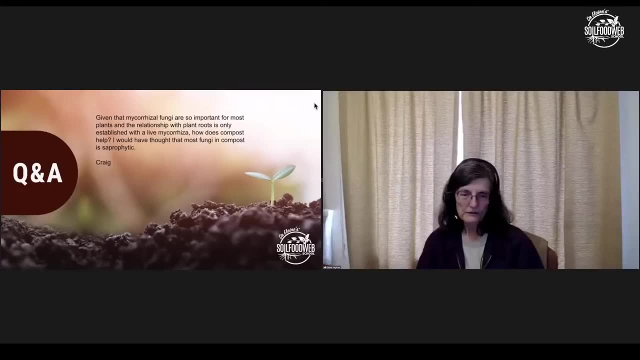 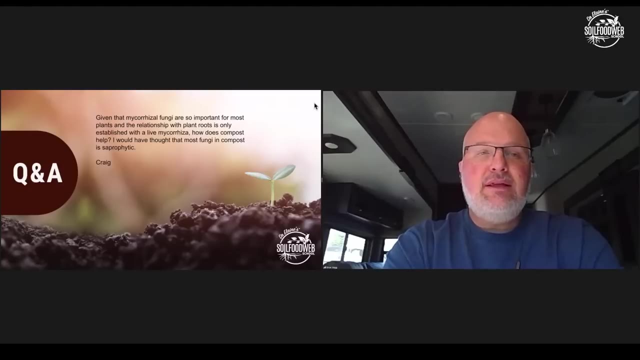 where I want to go more into these other application methods that are an alternative to just buying these commercial products that I don't really believe in. You need local indigenous Yep- Very important. It's funny, you know, because the biological marketplace is expanding rapidly. In fact, I have clients who constantly come to me and say: 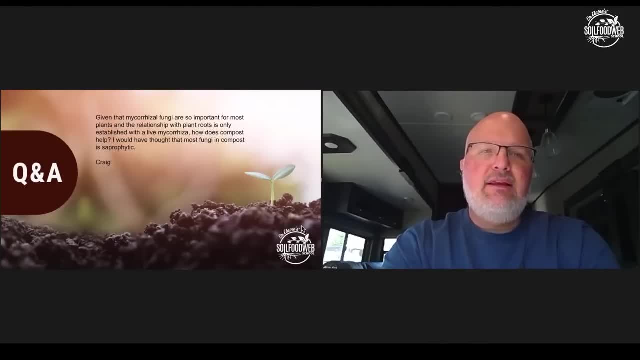 hey, what about this product? What about that product? What about this product? And you know a lot of those are kind of bugs in a jug or you know they're made in some bioregion that's way away from the bioregion that you're trying to grow in. And, yeah, there'll be a 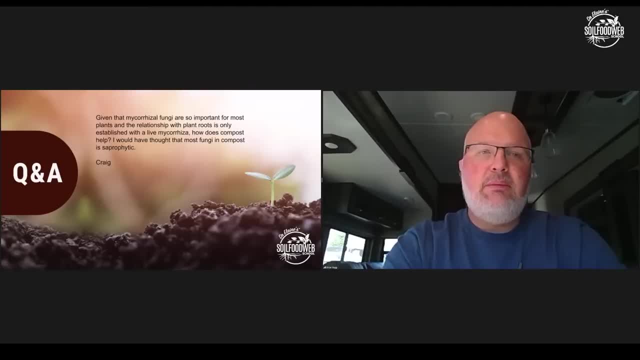 few of the species, organisms, that will provide you benefit, but there's gonna be a lot of them that won't, And diversity is going to be a big part of that And I think that's going to be a very, very low. And that's the other part of our paradigm, which is we want biomass of those. 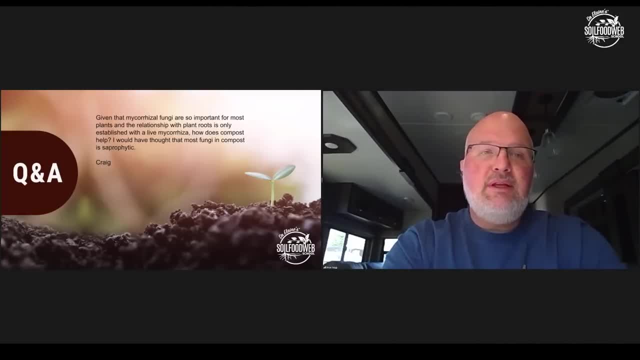 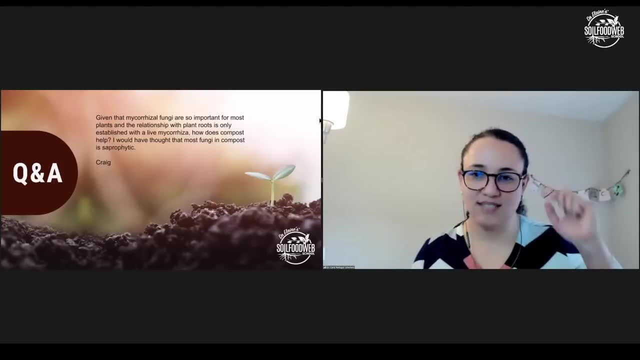 organisms, but we also want high diversity, And locally indigenously grown organisms is the way to go. Yeah, this whole movement of selling magic dust is dangerous And you have to be very aware that you should not shift from industrial agriculture to biological. 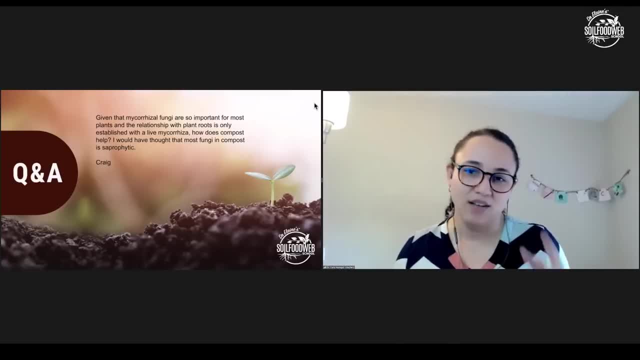 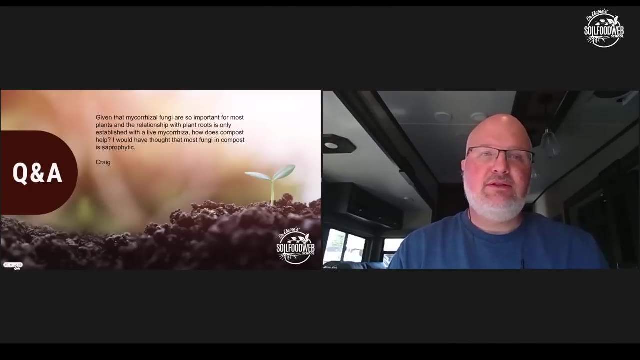 boxed agriculture in the same way. It's just changing the name, but also promising one application only and you're done. So be aware with these easy solutions. Sure, Okay, you know what? I think we have time for one more question. Let's go for it. 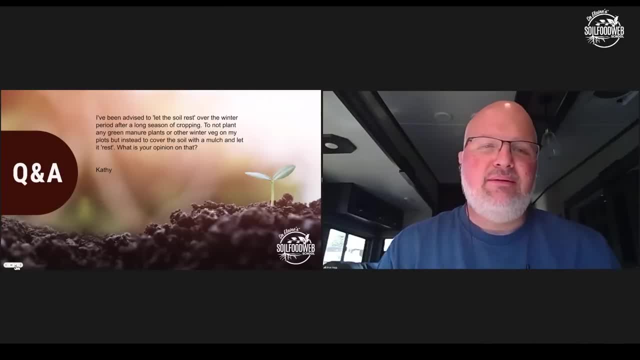 Adam, I think we got one last one here. Okay, so this one's from Kathy, And Kathy said I've been advised to let the soil rest over the winter period after a long season of cropping, to not plant any green manure and to not plant any green manure and to not plant any green manure. plants or other winter veg on my plots, but instead to cover the soil with a mulch and let it rest. What is your opinion on that? Yeah, even in the wintertime your microorganisms are going to benefit from the roots that are still left in the soil or the mulch that you left from just. 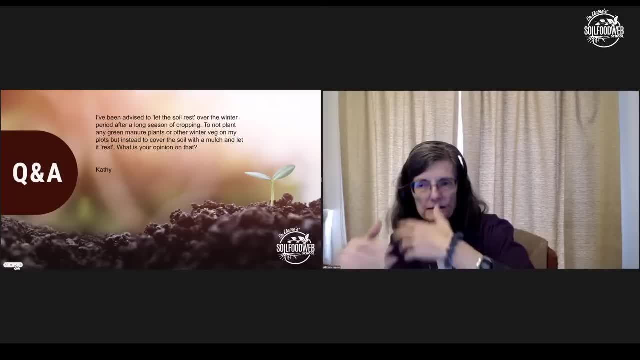 cutting the above ground part of the annual plant and dropping it. So I think that's a good question. Yeah, I would agree. I think that's a good question. So I think that's a good question. So I think that's a good question. So you want those bacteria and fungi? 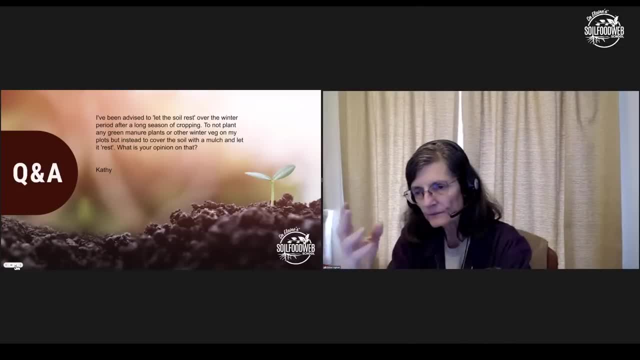 protozoa and nematodes to continue to cycle nutrients. to be building that soil structure, You had to come across your field with heavy equipment, probably to be able to harvest your crop in time. So there's some reconstruction that has to happen in that soil Now, the only time. 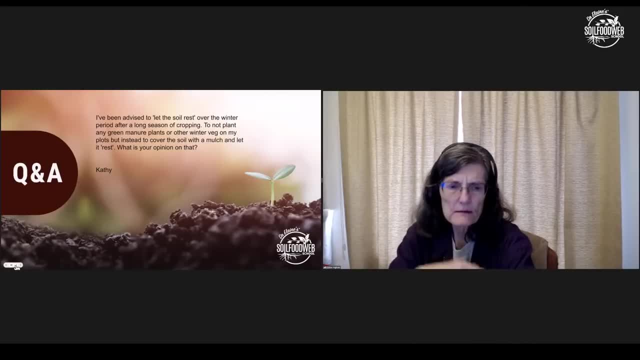 I could see, you know, planting green manure plants or other winter veg That's probably going to be killed in the winters I've encountered in my life, And so that dead material in the soil provides food for the bacteria, fungi, protozoa, nematodes, et cetera. And it just keeps things going. The most rapid rates of decomposition ever encountered on this planet was from a study that we did up in the mountains in Wyoming, where the most rapid rates of decomposition occurred in the winter under the snow. You have to have a layer of snow to prevent rapid freezing. 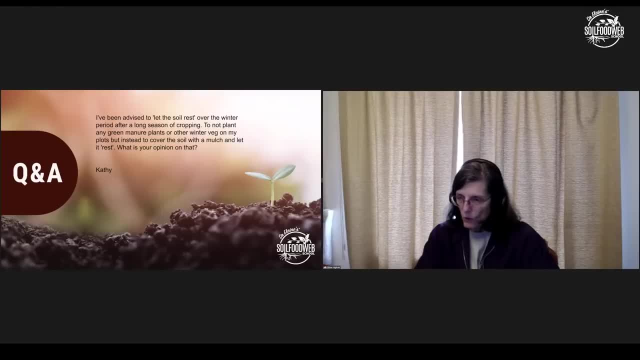 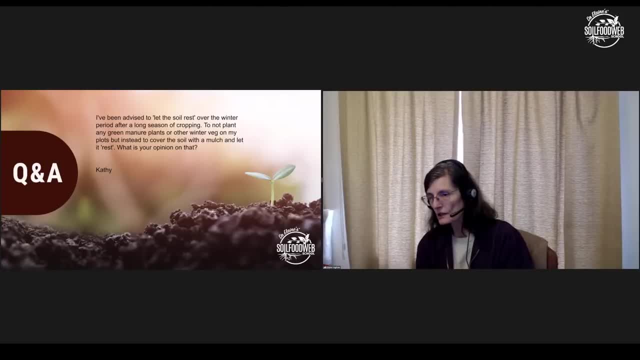 Now, if you don't have snow and you don't have a mulch layer out there, you're not going to get these benefits. So if you can remember that, you're going to get benefit from these organisms even through the wintertime. 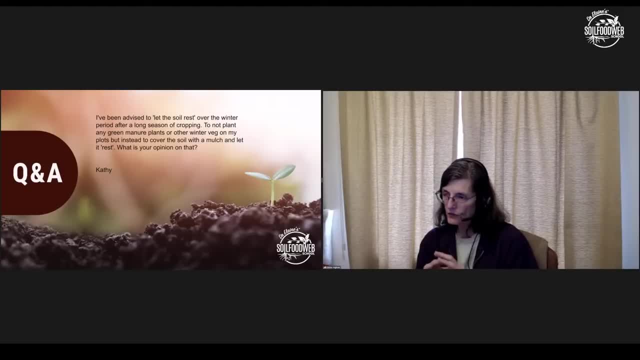 they're ready and raring to go. the instant that soil thaws, as soon as it can possibly get back up to the surface of the soil, you're gonna have those organisms building all that structure, doing all this good stuff for you. so this attitude towards don't plant anything, don't let any, 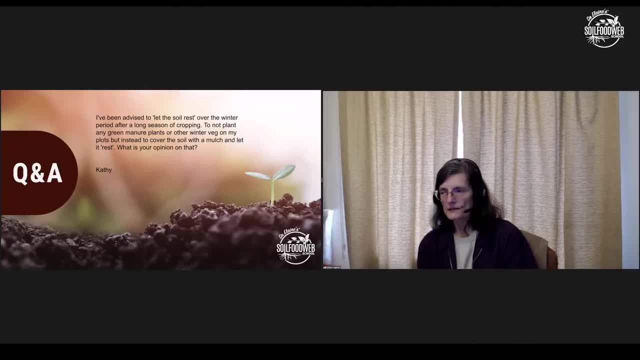 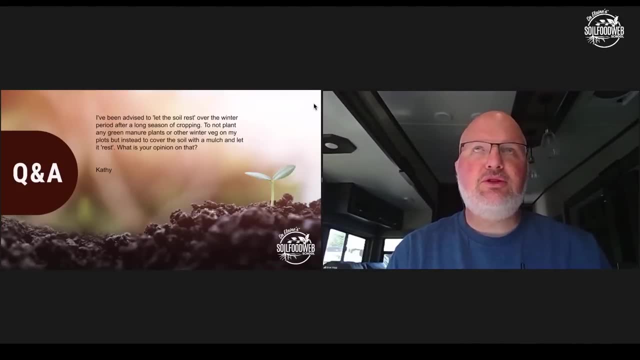 living thing loose because they're all dead down there. nope, not true. i remember um at the soil summit last year- soil summit i think his name is richard clark um- and he does a lot of different crop rotations so that he will plant in a late fall, planting that will not get winter. 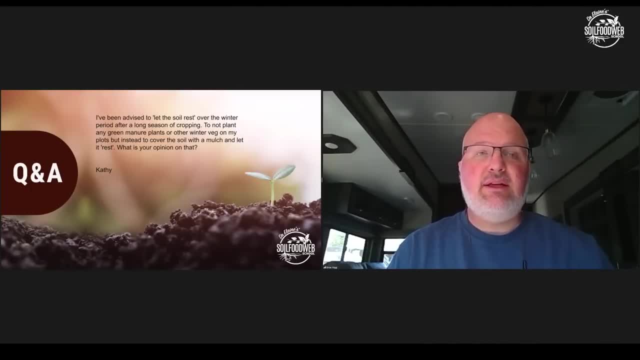 killed or or at least will provide some amount of cover. and if it does get killed in spring time frame- you know you've already got a lot of biomass is going to break down and decompose. you know, for me the most egregious thing you can do is to leave a field fallow with nothing on it. i mean, if you 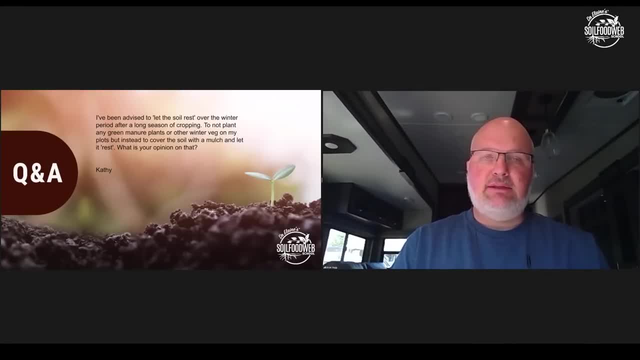 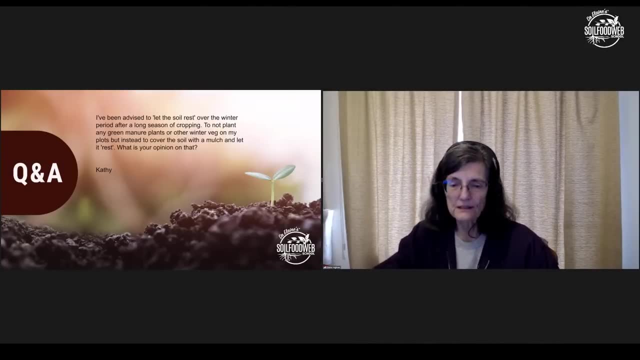 just left it bare soil over the winter time frame. that's just madness, in my opinion. yep, but you know it's like: uh, they don't want to leave that mulch down because that mulch has a weed seed in it, and so they pull it off, thinking they're doing the best, and in fact they're not. um, you want to? 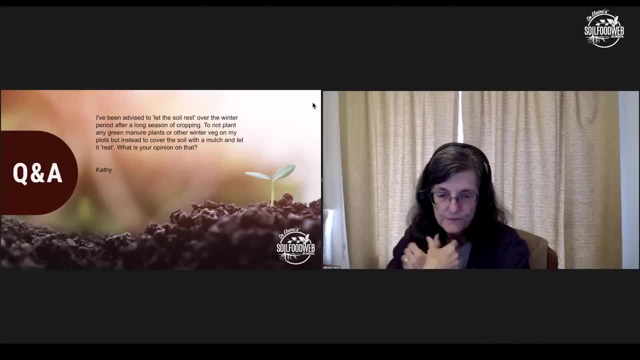 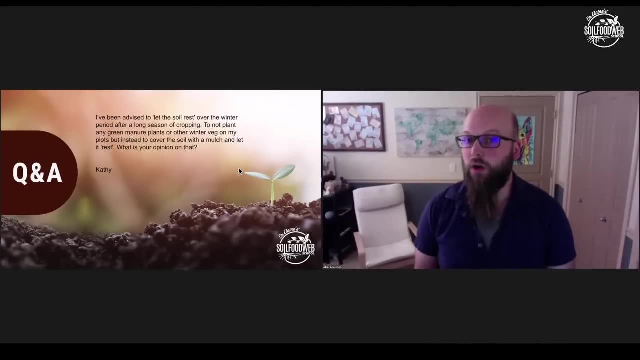 see that decomposition occurring through the winter time. i am really curious, like, um, what the goals were or the thought process was, and what the goals were and what the process behind this advice. um, i think a lot of times people have that leave the soil rest thing because they're monocropping the same crop and they want to actually 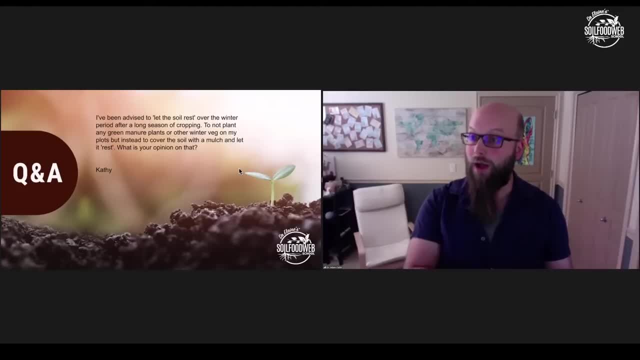 decrease the population of potential pathogens to that crop, and so it's that sterile world view right that go in and do something that will, you know whatever, but i think increase the diversity of your cropping system. don't grow the same thing and the same space. don't grow the same thing and 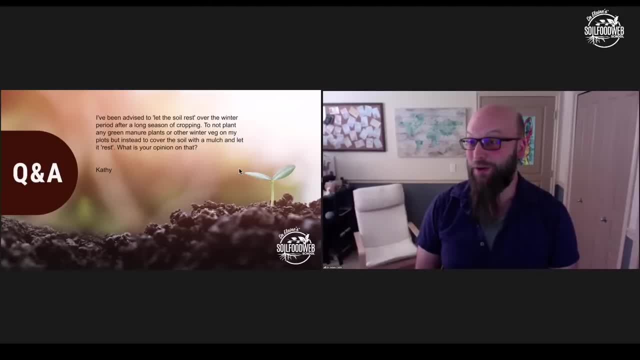 the same spot, year after year after year. um increase the the number of crops if you can integrate other processes. there's lots of. there's like legumes that can survive in a lot of winter conditions, and then they could be adding nitrogen to your soil, like austrian winter pea is one that 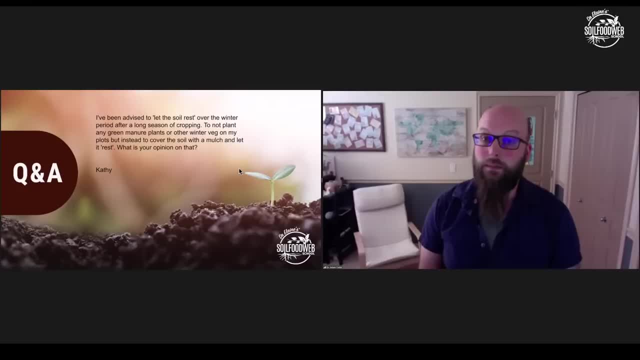 i've used in the past certain vetches um in my garden system. over winter i got some oats growing and all of that is like. ultimately, we have to be able to grow the same crop and the microbes, most of them and most of the animals in. 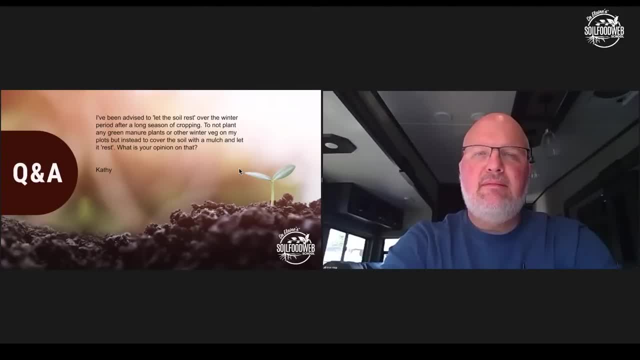 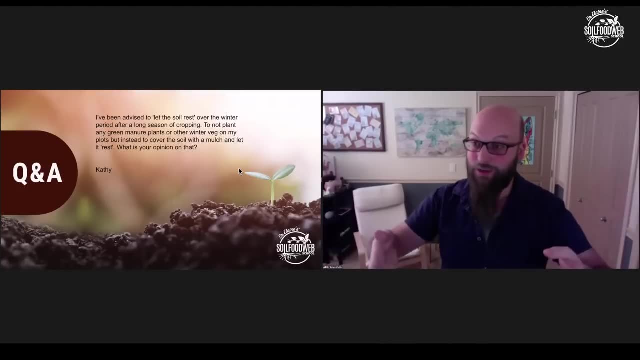 this world. ultimately, we're all eating sunlight right, and the plants have fixed for us into sugars and other carbohydrates, and so if you don't have, if sunlight is hitting your field but it's not hitting a plant, that's a wasted opportunity to grow food for the microorganisms. 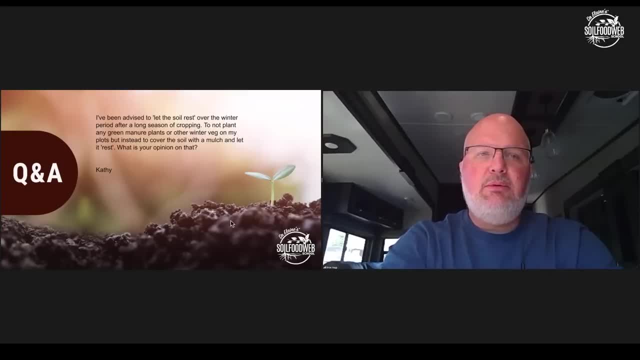 yeah, a common misconception that i end up coming across quite a bit is that people think of the, the nutrients in the soil, like a battery and the fact that there's only so much of the soluble nutrient and then, once you deplete it, you have to add it back into the system. so if i plant plants, over the winter time frame. they're just going to draw down that battery and take more soluble nutrients out of that system. it gets all the time too in, you know, like plenty understory plants in orchards or vineyards and things like that. oh, they're just going to steal the nutrients away. from, from those plants and unfortunately that's a very wrong way to look at it. the, the plants, are going to feed the microbes, which are going to continue to keep on understory and keep on growing, unlocking the nutrients that are in that soil. it's not like you're drawing down a battery, in fact. 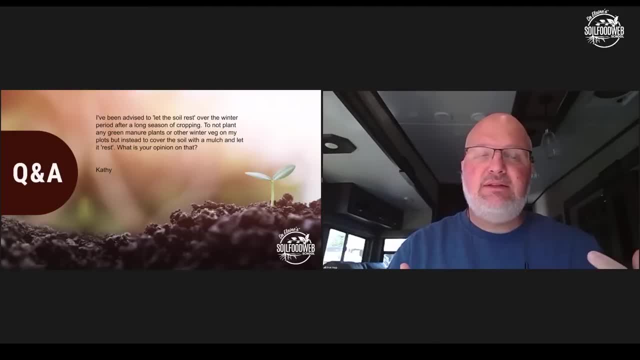 having a multi, diverse set of species or plants in there are going to drive different types of microorganisms and really allow for you to unlock those nutrients. so it's not a negative, it's actually a really big positive. okay, anything else you guys want to add before we close this. 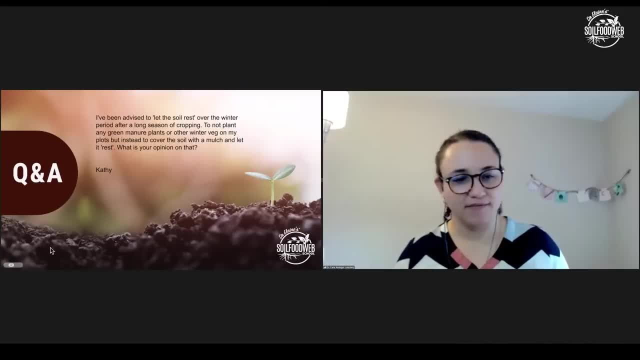 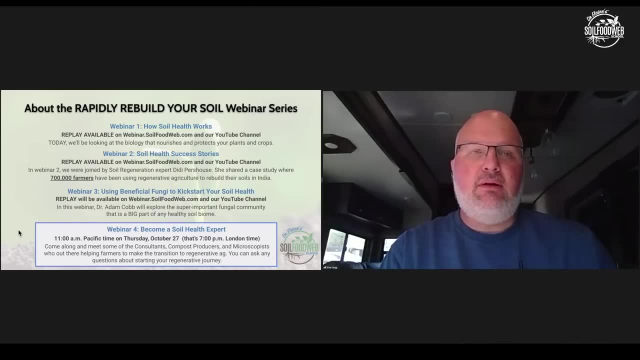 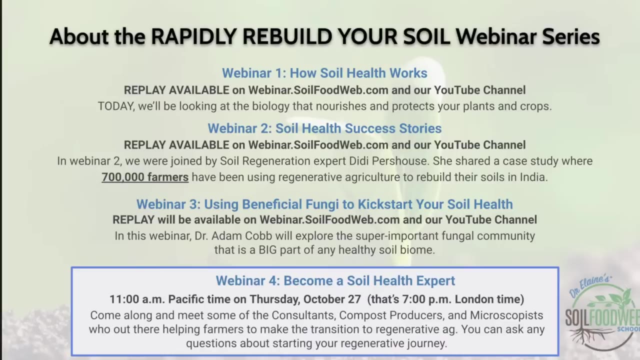 nope, all right. so, uh, let's go and move to the next slide, adam, and let's talk about webinar four. so we have one more webinar in our october promotional series and this is going to be on thursday, october 27th, and it's going to be, uh, talking with the soil, health experts, people that. 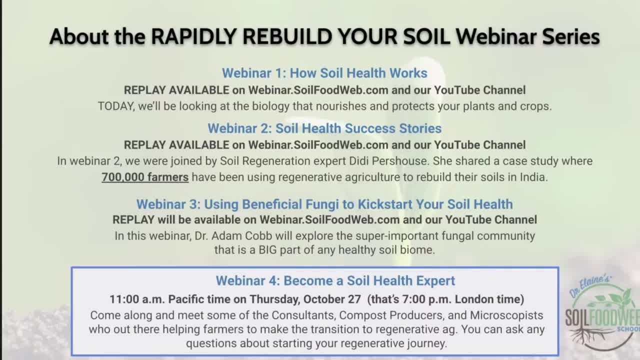 are consultants and compost producers and lab techs doing the work out there to help transform those growing systems and it's a great way to be able to hear from, from you know us, the folks out there doing that work, and then ask questions. you know what's. 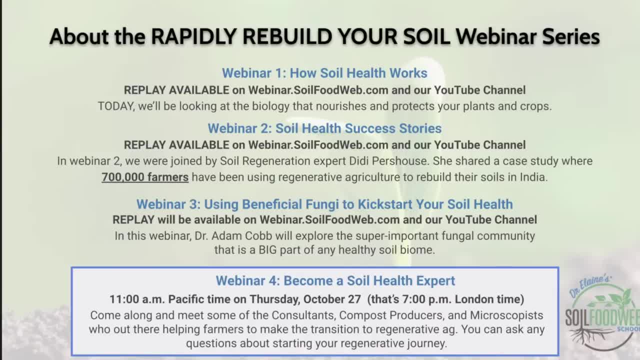 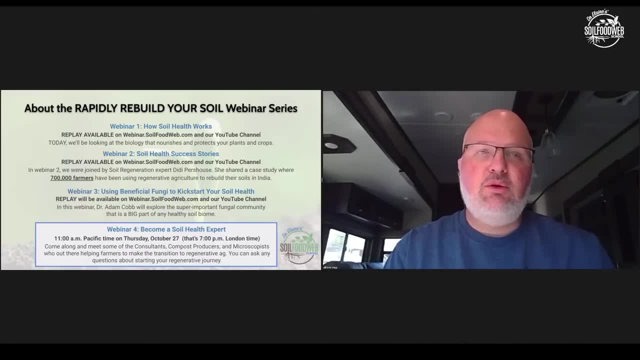 it like on the day in the life of being a consultant or something similar to that. so we look forward to seeing you folks on webinar four and before we close, i'd like to be able to get some thanks. um, so we have an amazing support staff. there are a lot of people that are behind. 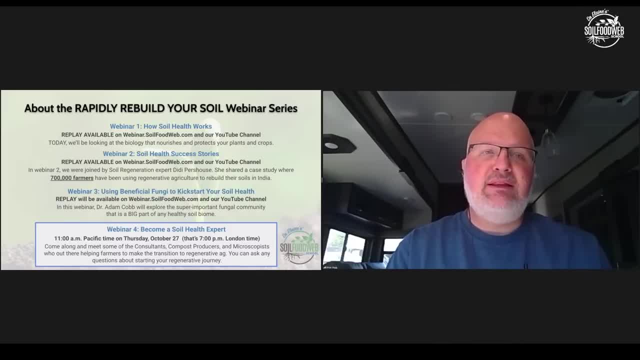 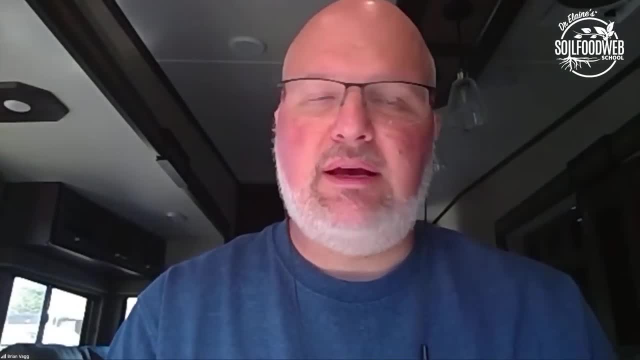 the scenes that really, really do a good job at making these uh webinars seamless. it takes a tremendous amount of work to be able to put these things together, so i'd like to really thank our support staff, and then i really like to thank our panelists today. um, you know your knowledge that you guys 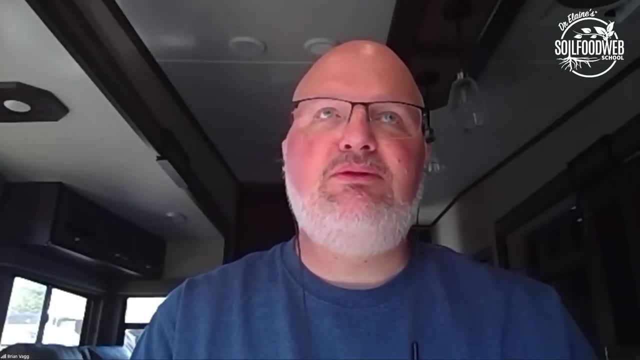 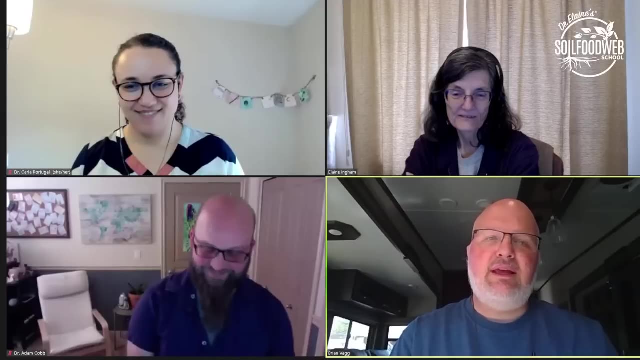 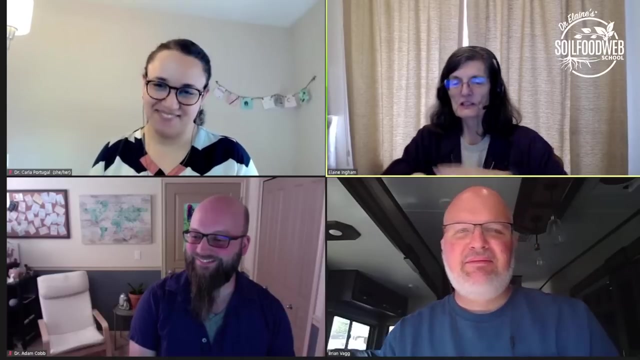 are sharing and the experiences that you have to be able to to really enlighten and infect minds uh with this information is fantastic. so so thank you elaine, adam and carla uh for all the work that you guys do and, of course, thank you brian for being the facilitator of everything, and david 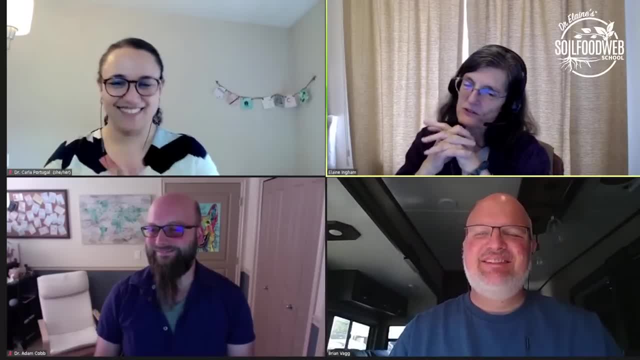 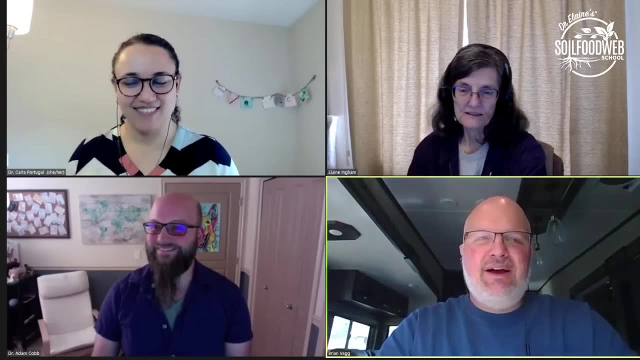 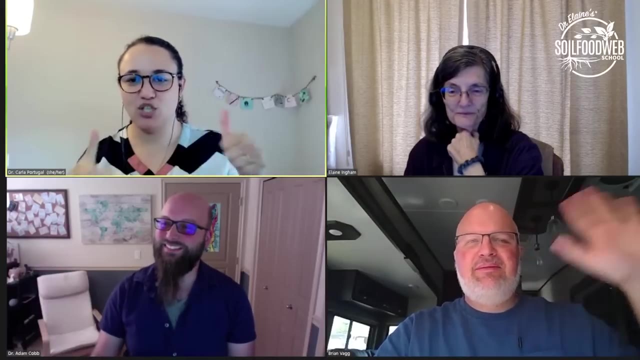 and sammy, and behind the scenes. thank you so much. we couldn't possibly do this without your help, exactly. all right, everybody. um well, we're going to put this uh webinar in the books and we will see you guys in a week from now. thank you so much for joining us. 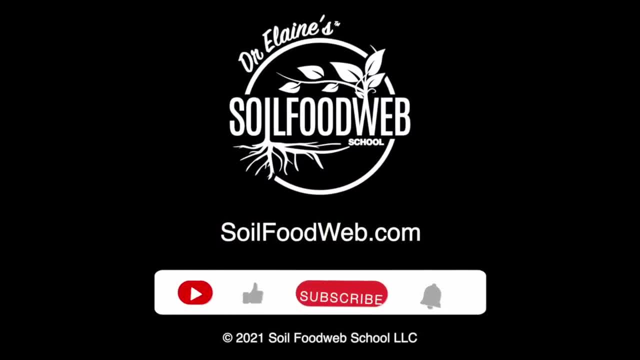 today. see you everybody, ciao. don't forget to click that like button, subscribe to our channel and ring the notification bell to stay updated with all our new videos. you. 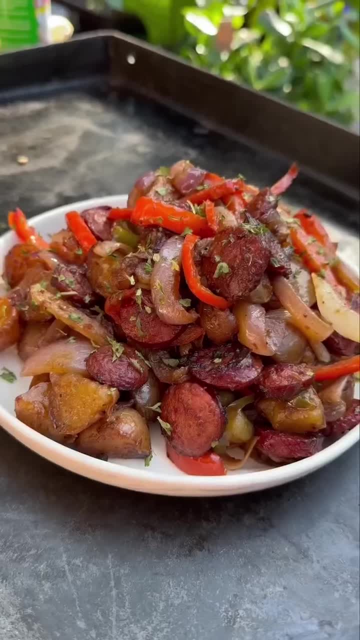 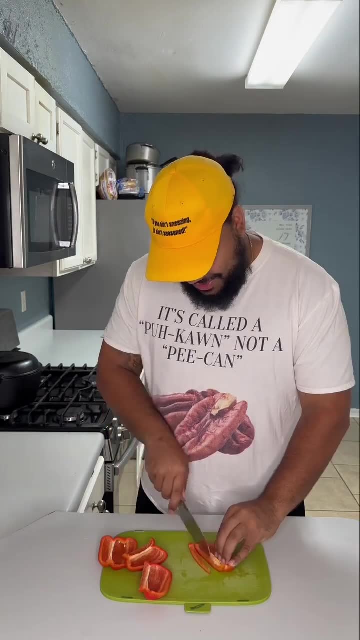 This is one of the best meals you can make for your family for under $10. And I'm telling y'all, it's pressure, Let's get into it. So boom. all you're going to need is some bell pepper, onions, sausage potatoes and Tony's spices and herbs You're going to cut your bell peppers into. 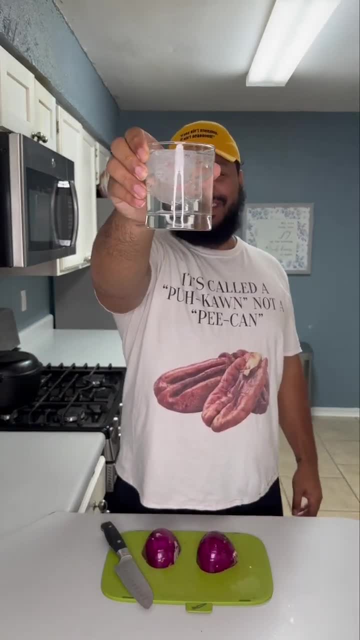 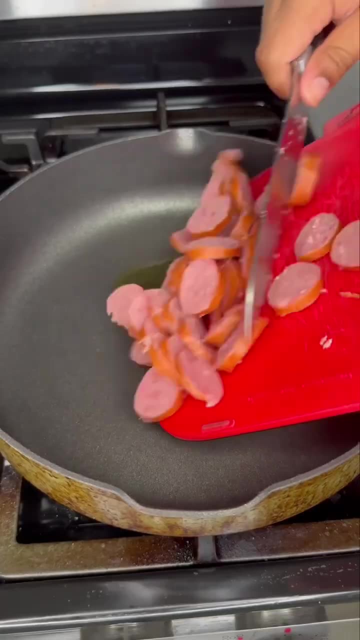 strips and get a glass of ice cold water to help absorb all the gases from your onions and you won't get teary eyed. Slice it up, Then we're going to take our baby red potatoes and cut them into quarters. Cut your favorite sausage in the rounds, Then we're going to brown it in the pan. 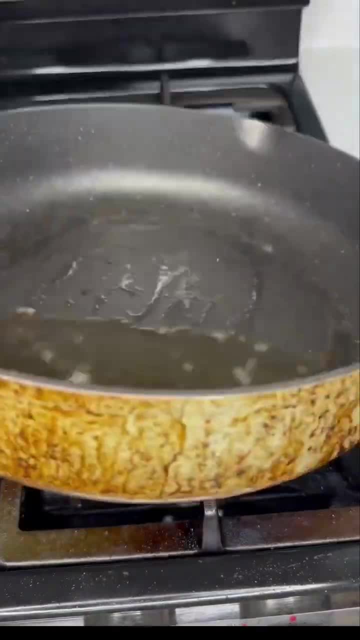 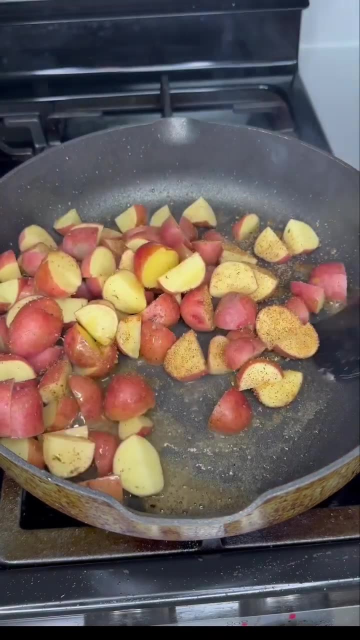 and render down some of that fat. Remove it with a slotted spoon. Then we'll use that rendered fat to cook down our potatoes. Season your potatoes with the Tony's sachery, spices and herbs And remember, if you ain't sneezing, it ain't seasoned. We're going to let it develop a nice little color. 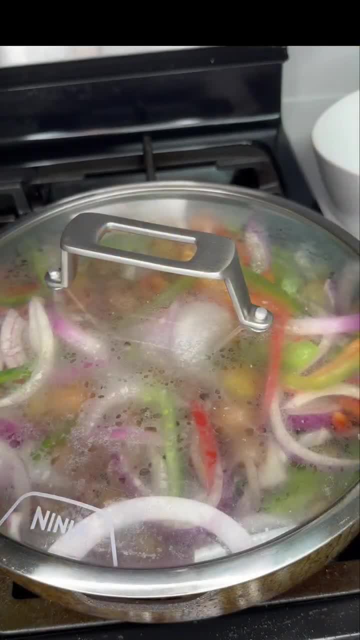 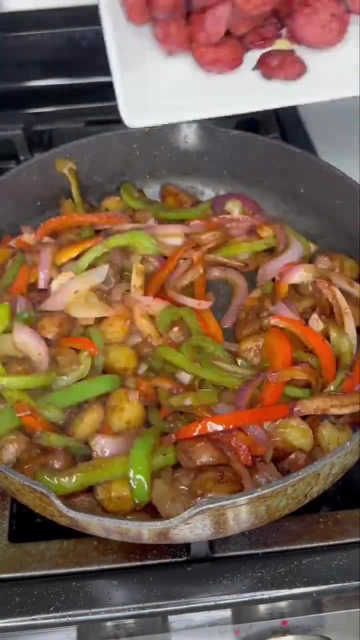 on it. Then we'll add in our vegetables, Cover it up and let it cook for about five minutes. The moisture from your vegetables will help tenderize your potatoes. Mix it up and cook it down for another five minutes or so. Once it's nice and tender, we're going to go ahead and add. 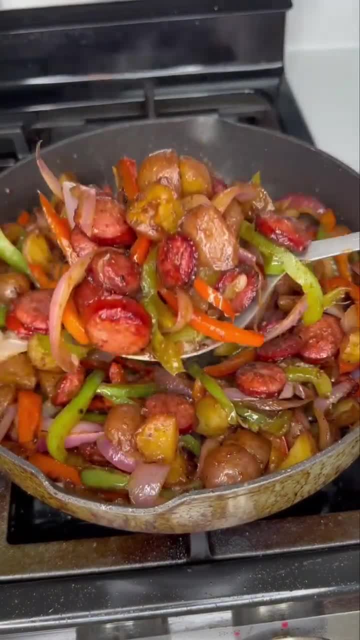 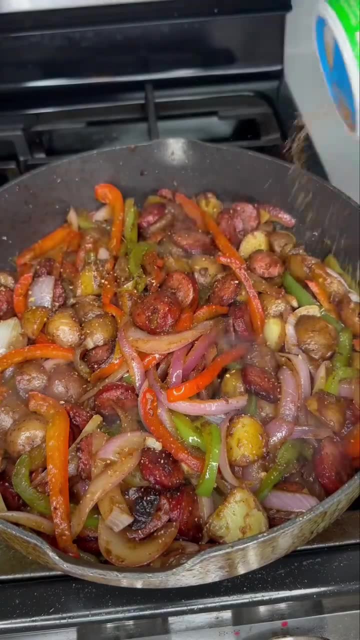 in our sausage with the drippings. I need all that. Mix it up and look at that. Yes, Lord, At this point your potatoes should be fork tender. Go ahead and adjust the seasoning to your taste, Plate it up And just like my name. 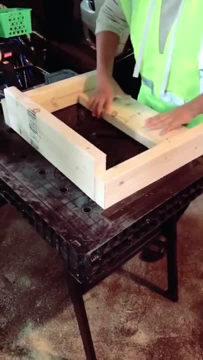 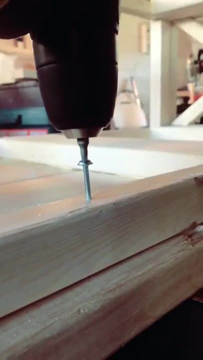 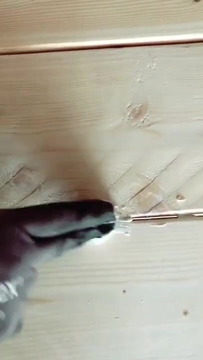 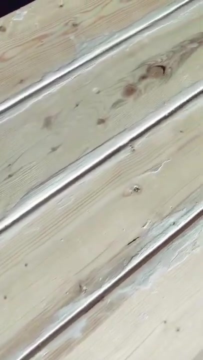 There is a large amount of information in the video. There are many people who have not watched the video. There are many tips and tricks. Please note that there are many videos that do not use punctuation. You can watch the video in a wide variety of ways. I was surprised and surprised.